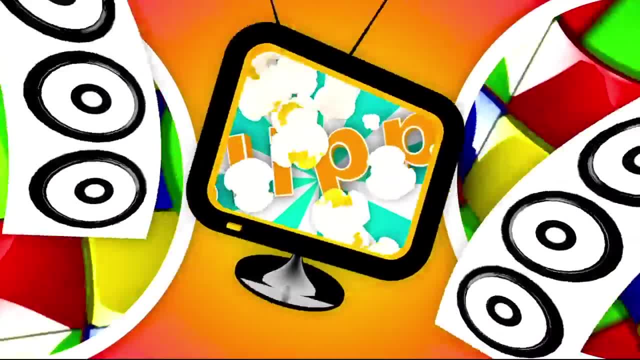 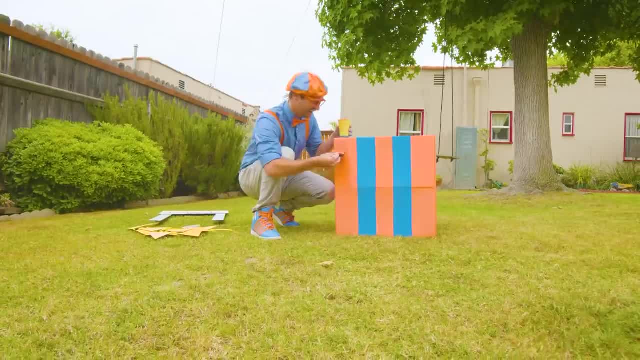 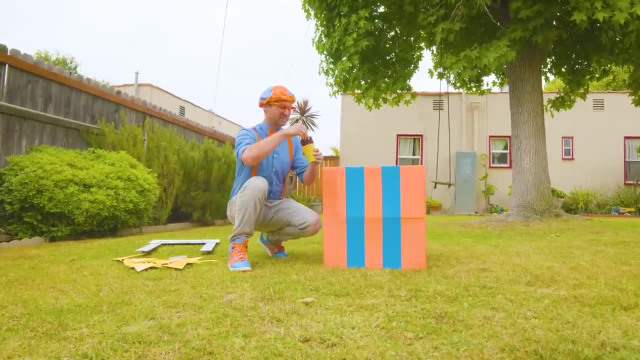 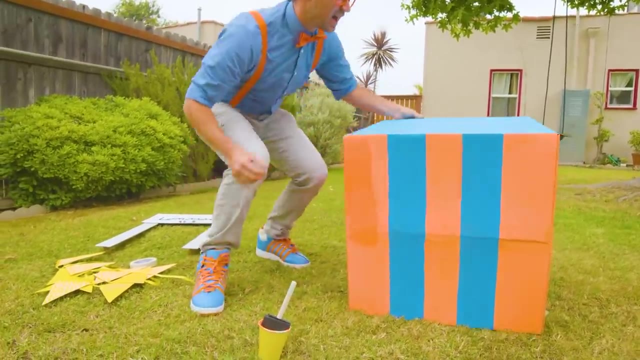 So much to learn about. It'll make you want to shout Blippi. Oh hey, It's me, Blippi. Do you see what I'm doing? I'm painting. Yeah, I'm actually painting just a regular cardboard box. Check it out, See, I took this cardboard box and I'm painting it. 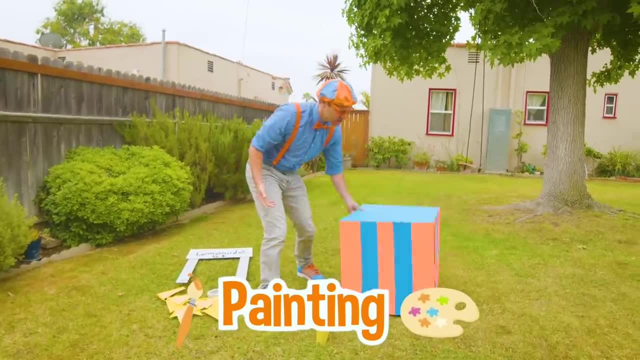 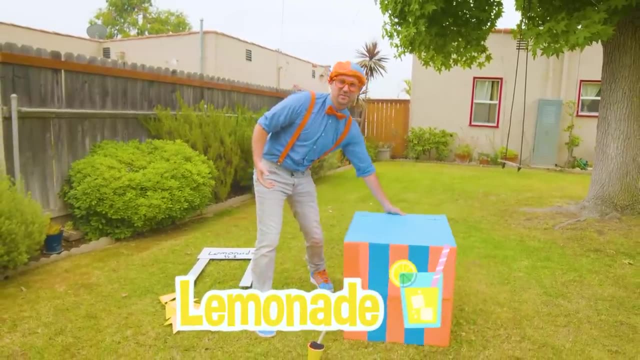 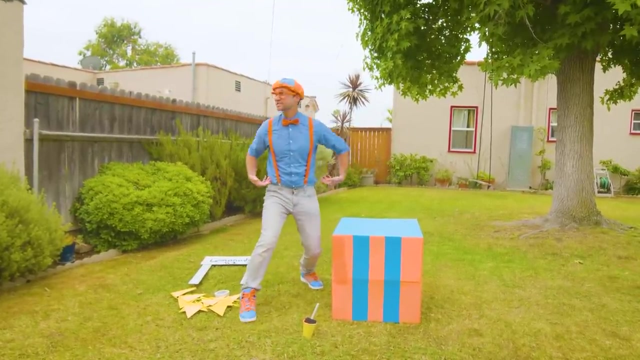 Do you know what I'm painting and making? I'm actually going to make a lemonade stand. Yeah, I love lemonade, It's so yummy. But a lemonade stand isn't used just to drink your own lemonade It's, so then you can sell lemonade to others. Yeah, So the first thing that you have. 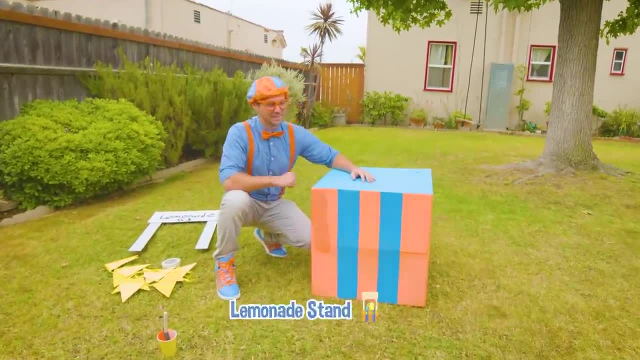 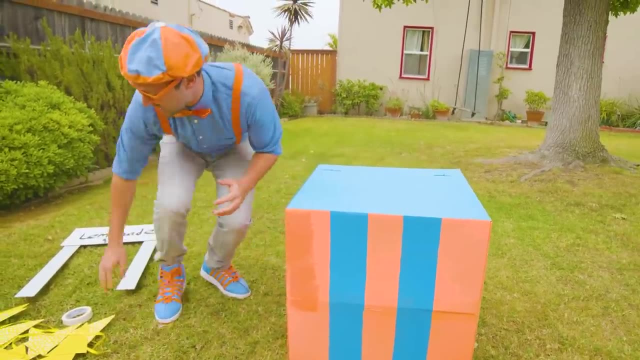 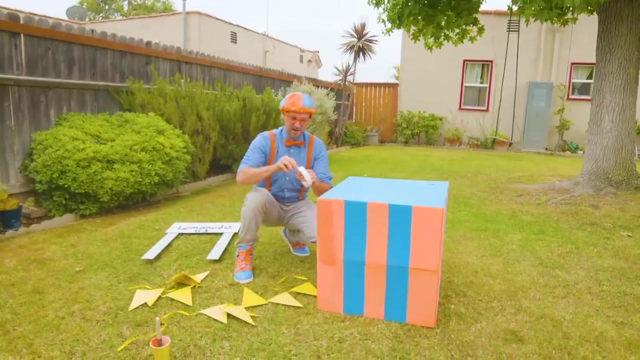 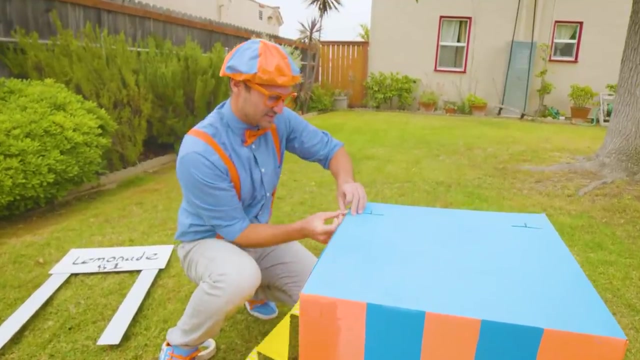 to do is make a very good looking lemonade stand, So then everyone will want to come try your lemonade. So now that it's all painted, I have these yellow triangle ribbons And if I put them on here on the top it will spark some more customers. Okay, let's put some tape right here. 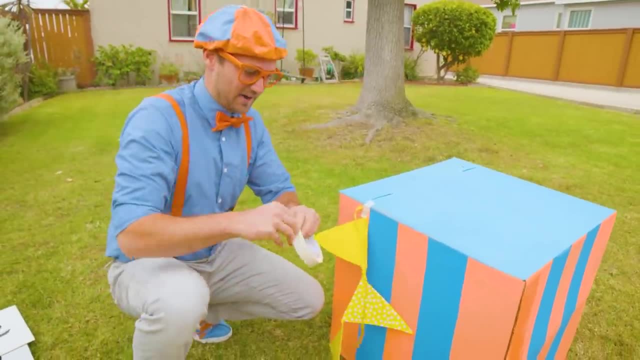 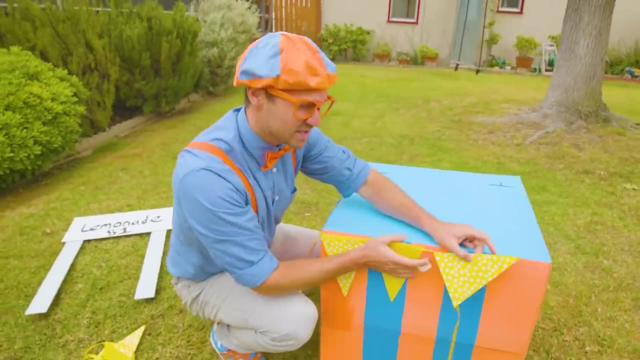 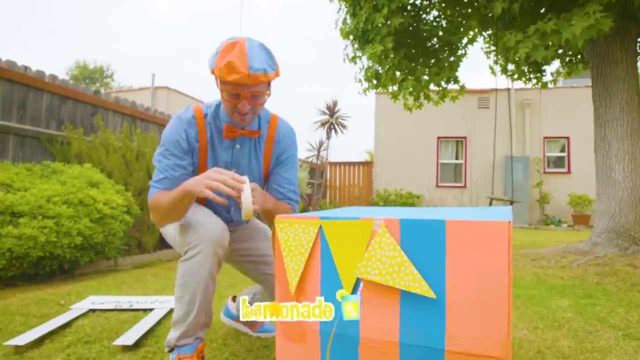 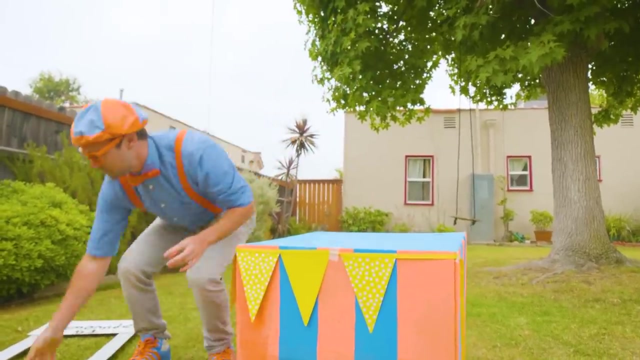 There we go. Wow, All right, You see these yellow triangles. Yeah, What? This is the color yellow that you can think of. Lemonade Also. the sun is the color yellow. Okay, here we go. Then we actually have a little bit more of this. Wow, Have you ever tried lemonade? 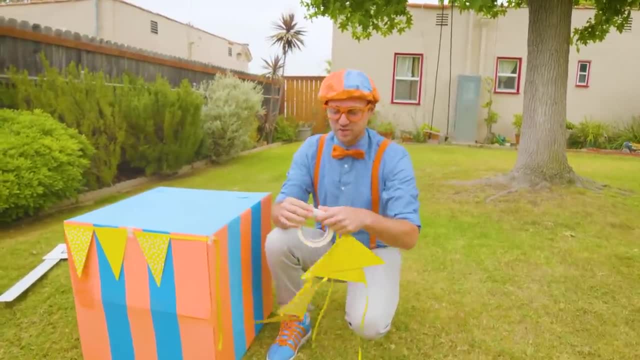 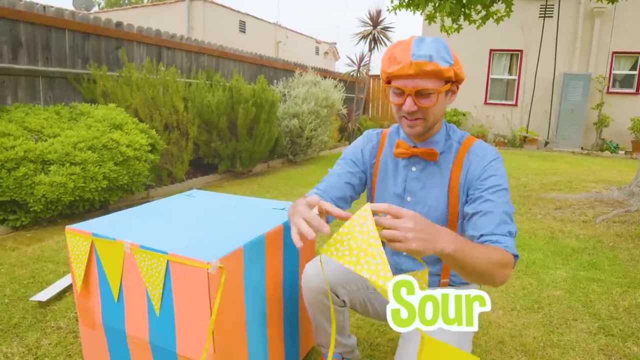 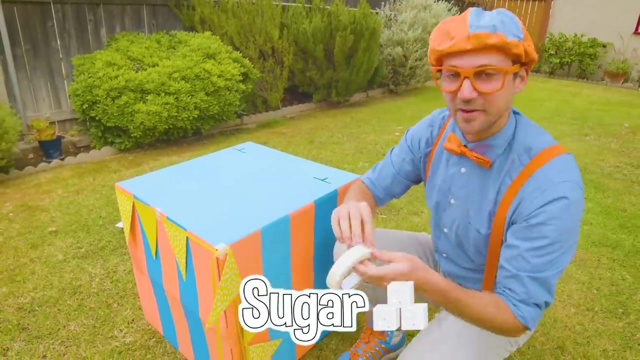 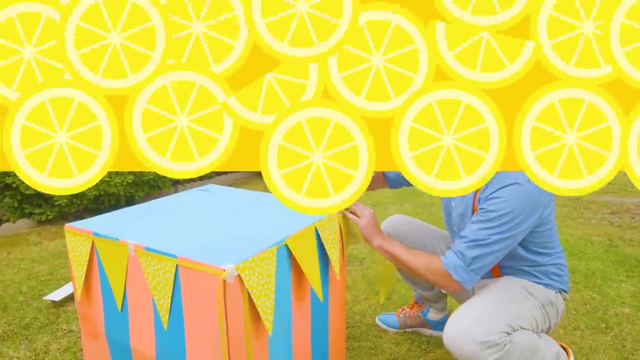 before It's really tasty. It's weird because if you just eat a normal lemon, it's really sour. Oh, So then we add a lot of water and then some sugar. It'll sweeten it right up and make a nice refreshing drink. Okay, How about right there? Whoa, It looks so good. All right, We have. 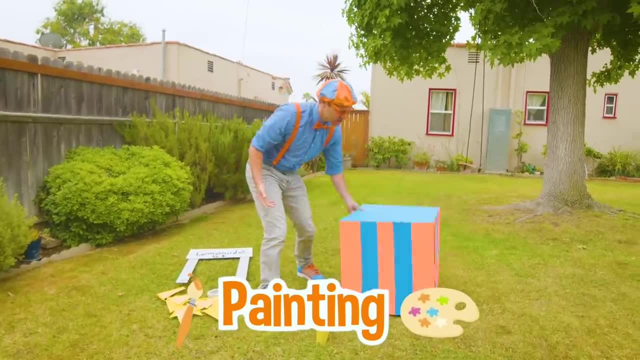 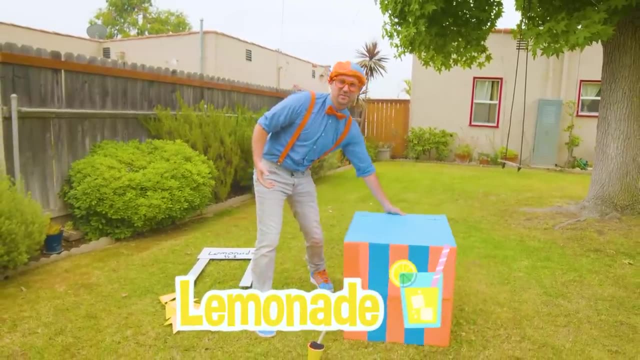 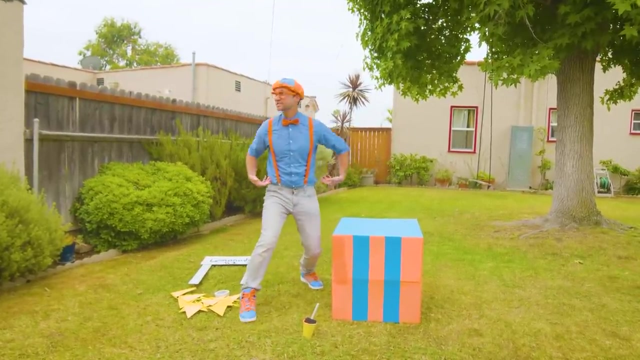 Do you know what I'm painting and making? I'm actually going to make a lemonade stand. Yeah, I love lemonade, It's so yummy. But a lemonade stand isn't used just to drink your own lemonade It's, so then you can sell lemonade to others. Yeah, So the first thing that you have. 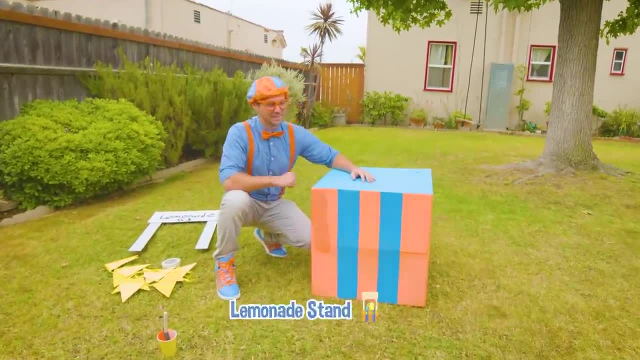 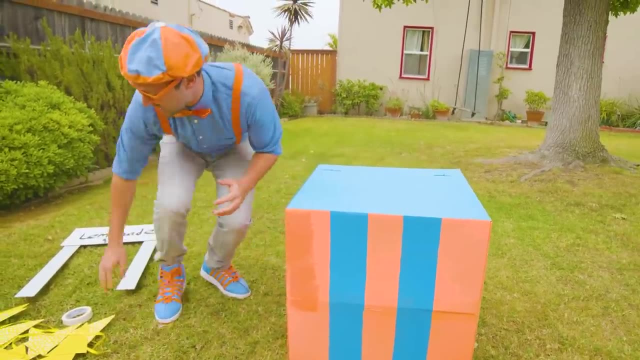 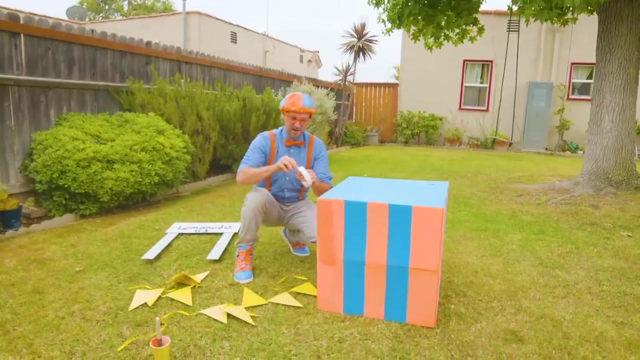 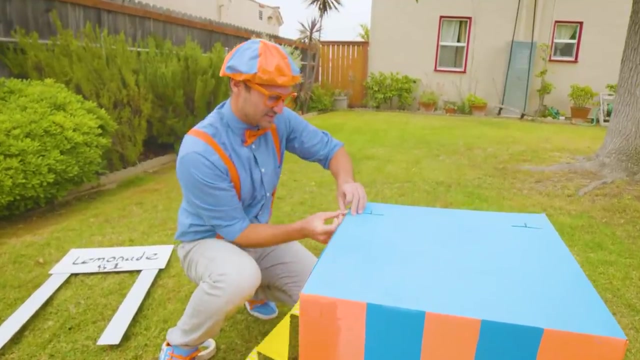 to do is make a very good looking lemonade stand, So then everyone will want to come try your lemonade. So now that it's all painted, I have these yellow triangle ribbons And if I put them on here on the top it will spark some more customers. Okay, let's put some tape right here. 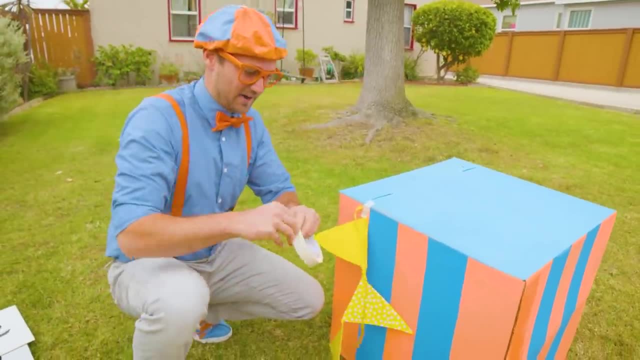 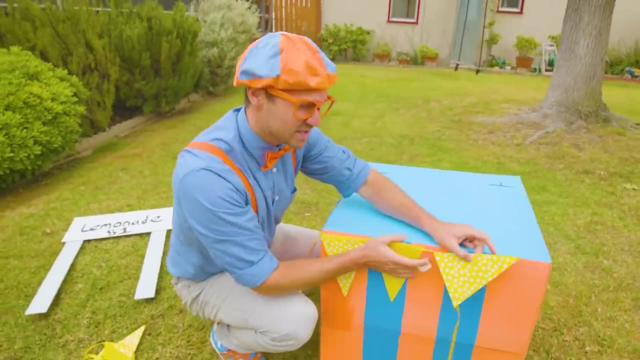 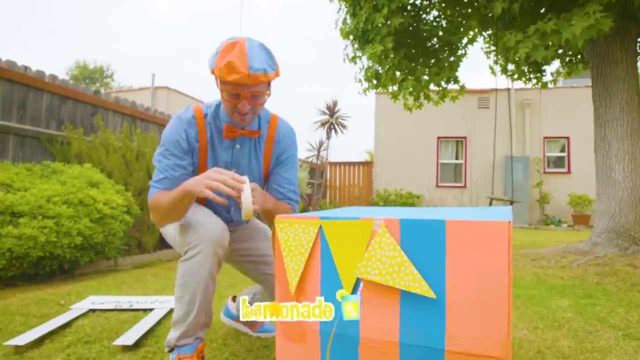 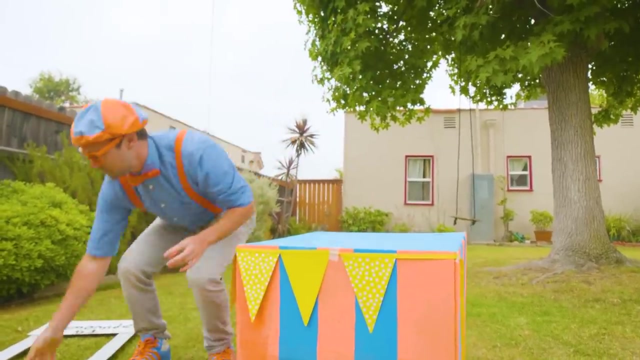 There we go. Wow, All right, You see these yellow triangles. Yeah, What? This is the color yellow that you can think of. Lemonade Also. the sun is the color yellow. Okay, here we go. Then we actually have a little bit more of this. Wow, Have you ever tried lemonade? 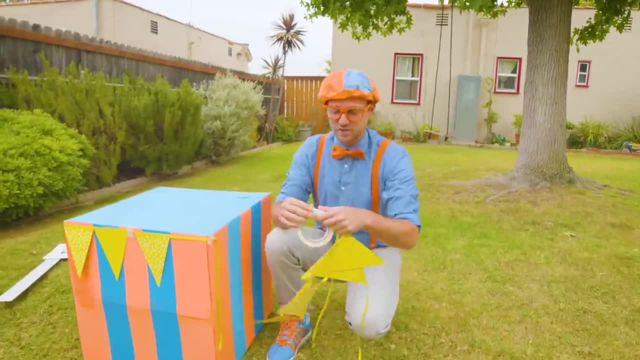 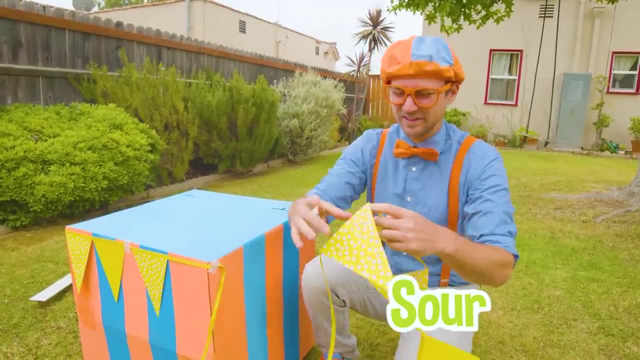 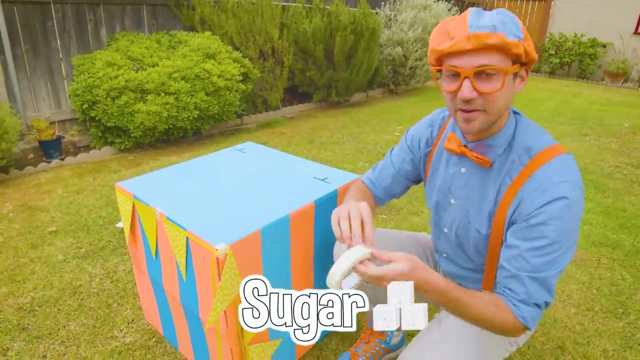 before It's really tasty. It's weird because if you just eat a normal lemon, it's really sour. Oh, We add a lot of water and then some sugar. It'll sweeten it right up and make a nice refreshing drink. 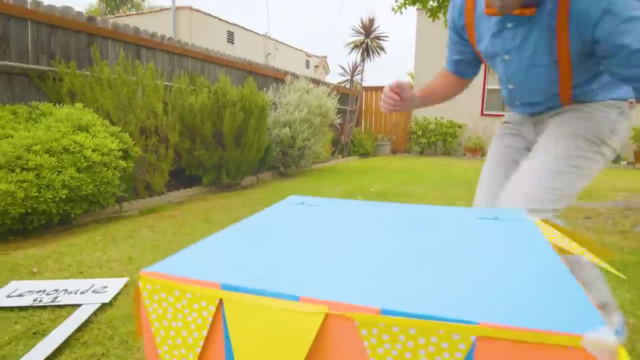 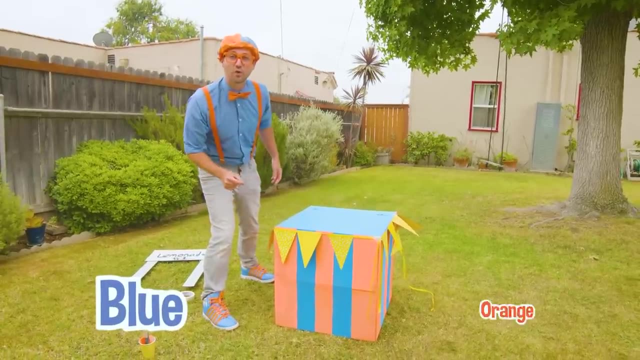 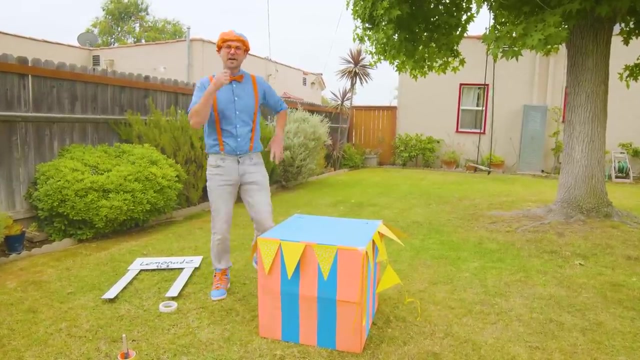 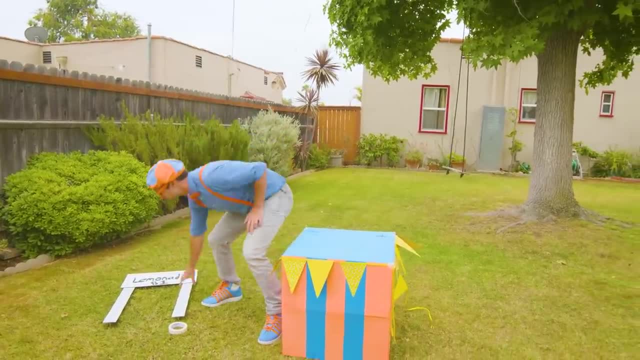 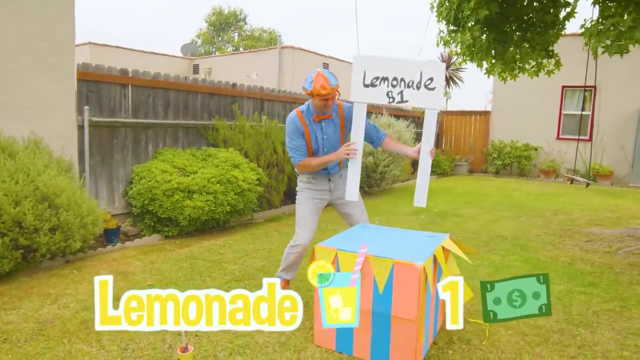 All right. So we're going to be like what's Blippi doing? So we need to tell them what we're doing. We're going to be selling lemonade one dollar, So let's put this right here. Perfect. 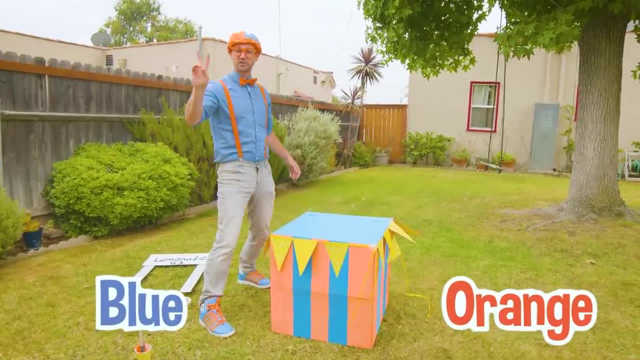 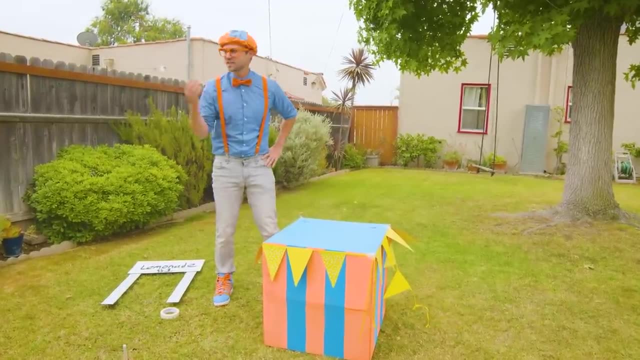 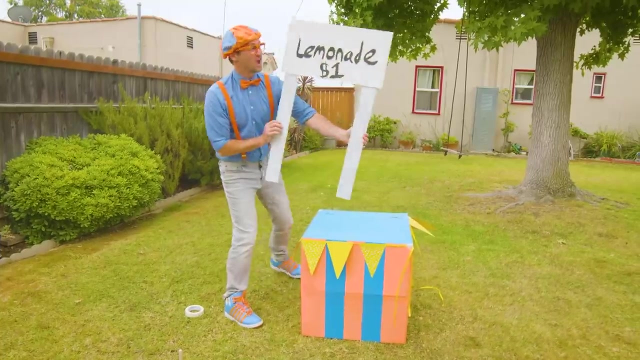 our lemonade stand blue and orange- My two favorite colors. We added the yellow banners to bring in more customers, But all these customers are going to be like: What's Blippi doing? So we need to tell them what we're doing. 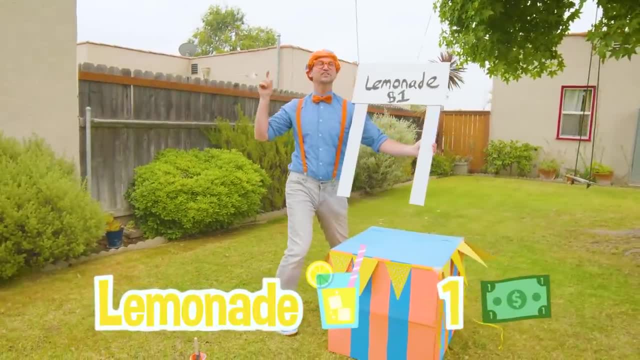 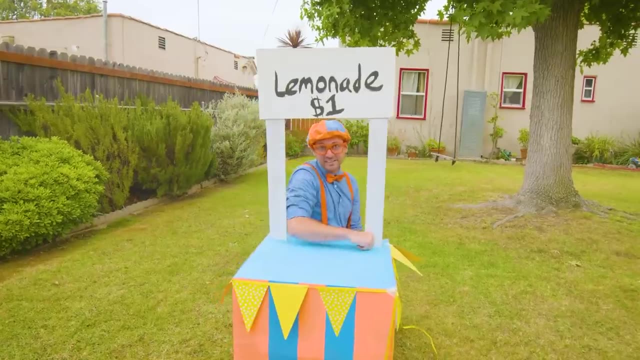 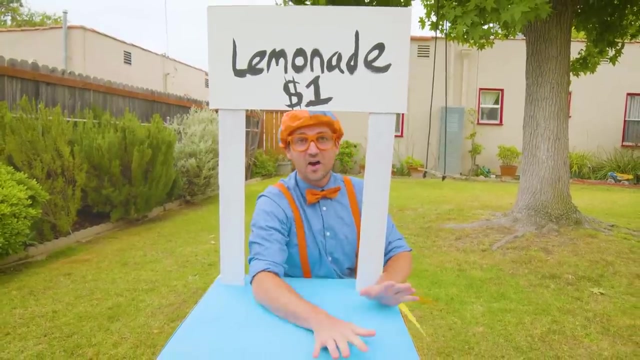 We're going to be selling lemonade- one dollar, So let's put this right here. Perfect, How does this look? Can you tell what I'm here for? Yeah, to sell lemonade. All right, now that we built the stand. 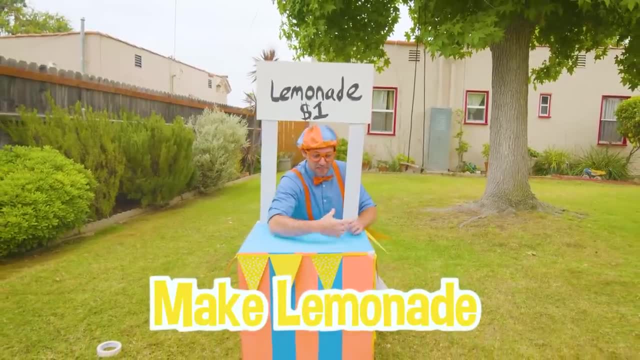 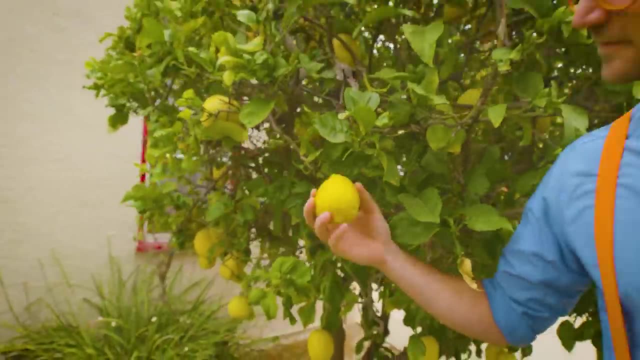 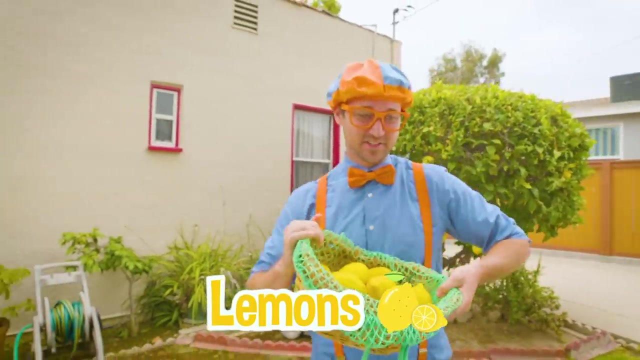 now we need to make some lemonade and then we can sell it. Yeah, let's go. Yeah, the first ingredient to lemonade is lemons. There we go. So great that our friend has their very own lemon tree. That definitely saves us a lot of money. 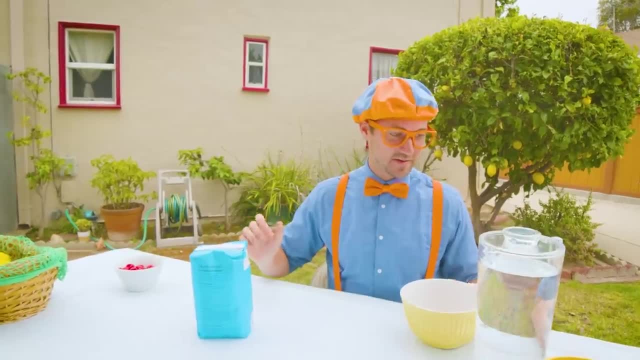 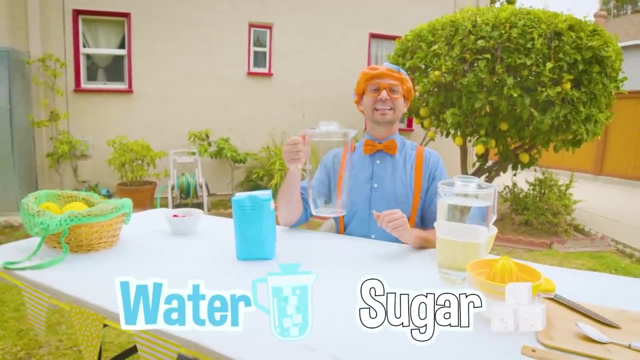 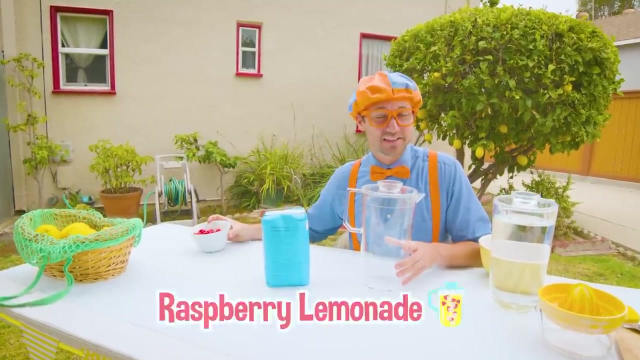 when we calculate how much this lemonade cost us to make. Okay, all right, see this picture. We're going to put a lot of water, sugar lemons and we're going to spice it up with a little bit of raspberries to make raspberry lemonade. 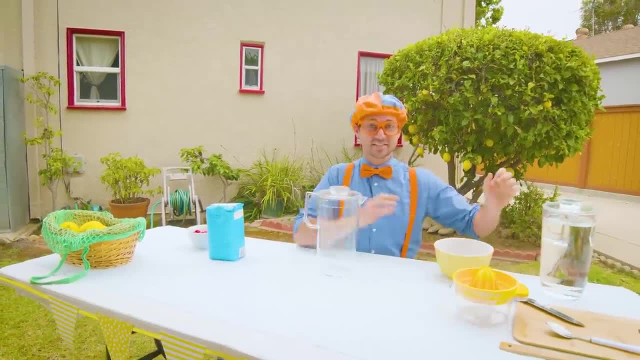 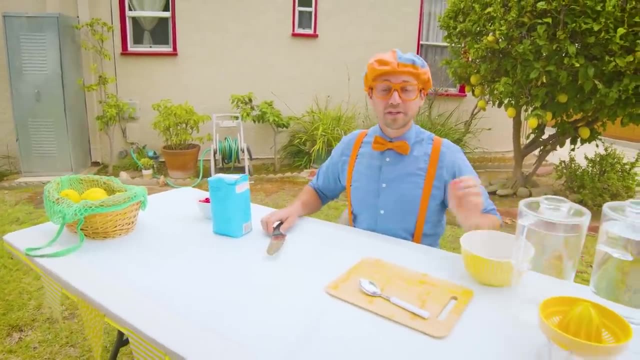 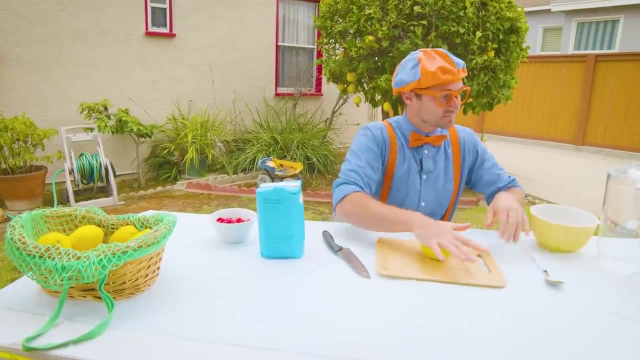 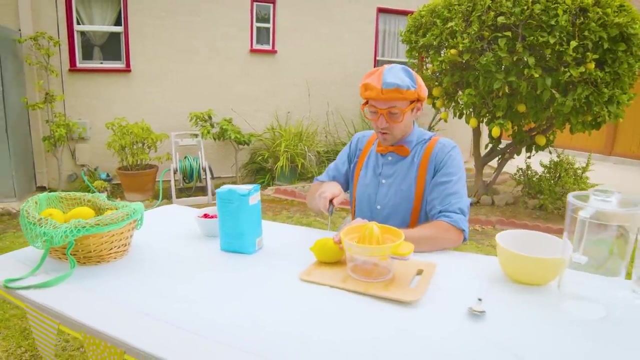 So the first thing that we need to do is to grab our lemons. Yeah, all right, And only grownups should use a knife. So we're going to first take a lemon, We're going to cut it in half And use this device to squeeze out all of the juice. 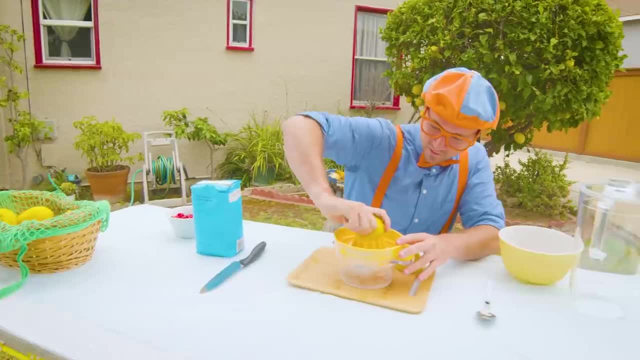 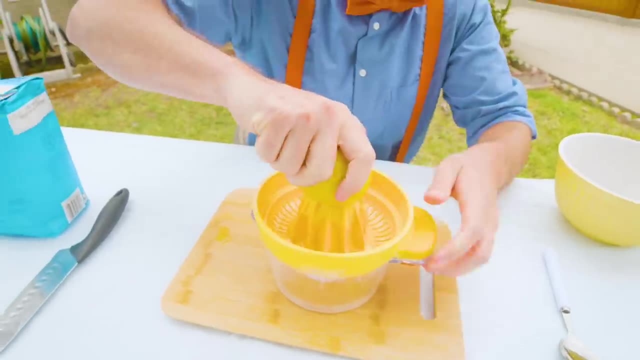 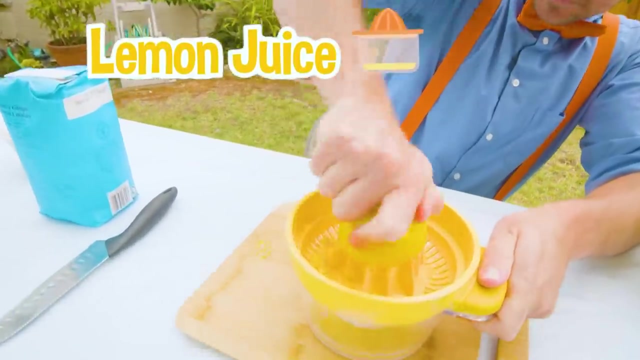 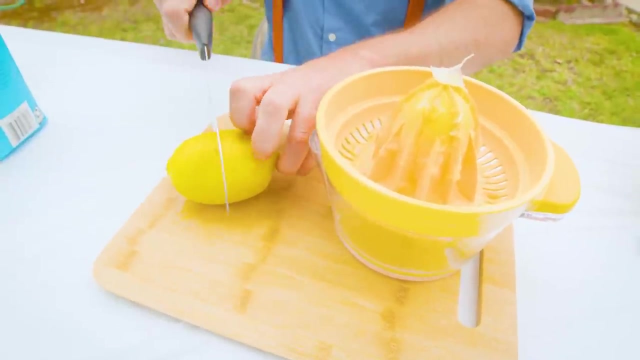 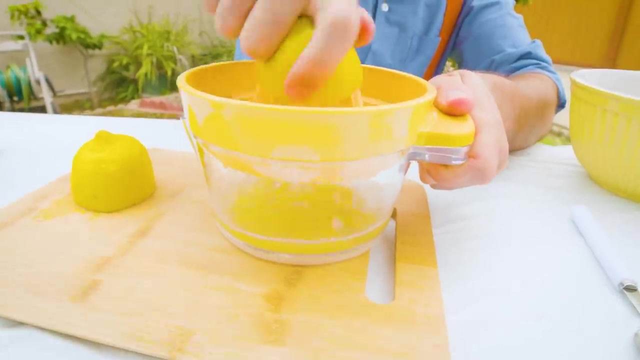 just like this: Ready, Wow, Yeah, do you see all that lemon juice down there? Okay, let's do another One, two, three, four. There we go. Whoa, This thing is just pressing out all of the juice. 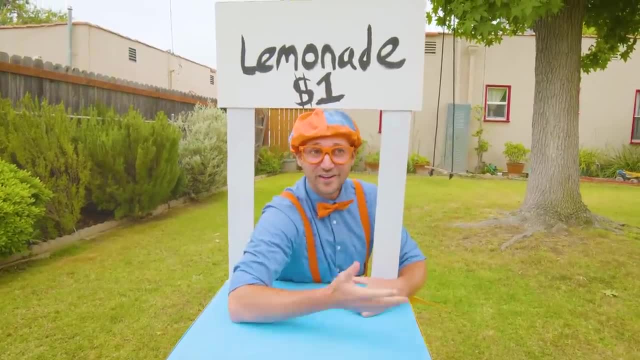 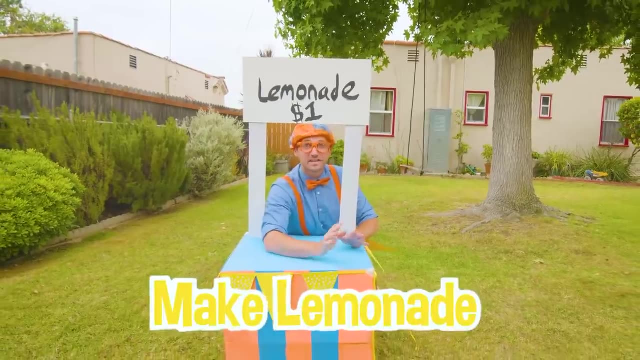 How does this look? Can you tell what I'm here for? Yeah, To sell lemonade. All right, Now that we built the stand, now we need to make some lemonade and then We can sell it. Yeah, let's go. 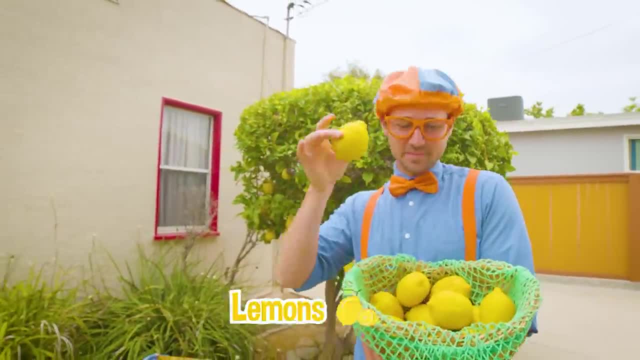 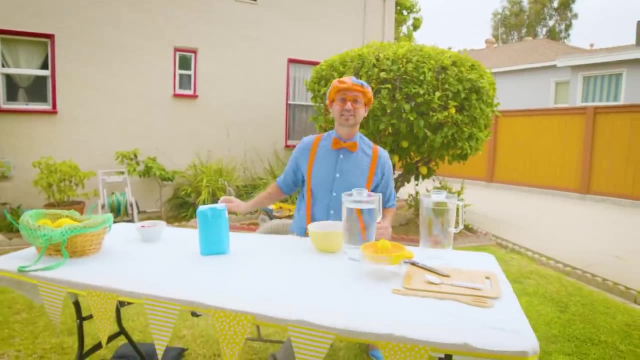 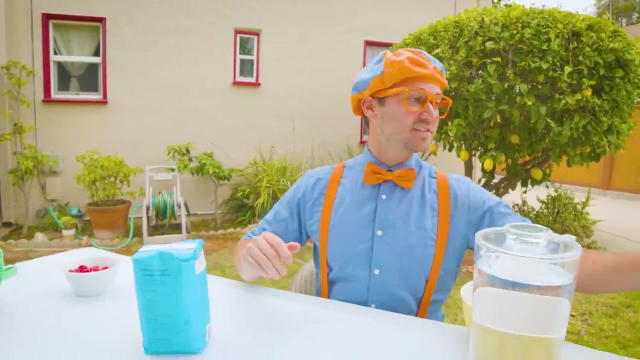 Yeah, the first ingredient to lemonade is lemons. There we go, So great that our friend has their very own lemon tree. That definitely saves us a lot of money when we calculate how much this lemonade cost us to make. Okay, all right, see this picture. 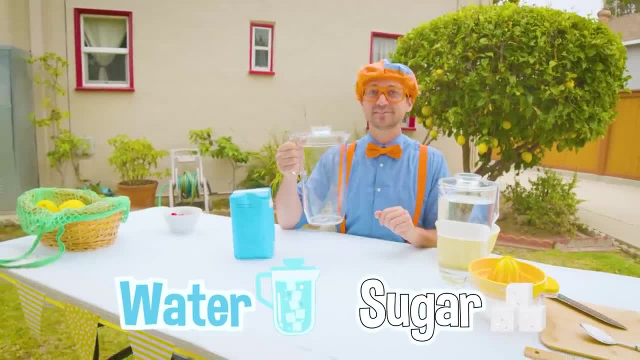 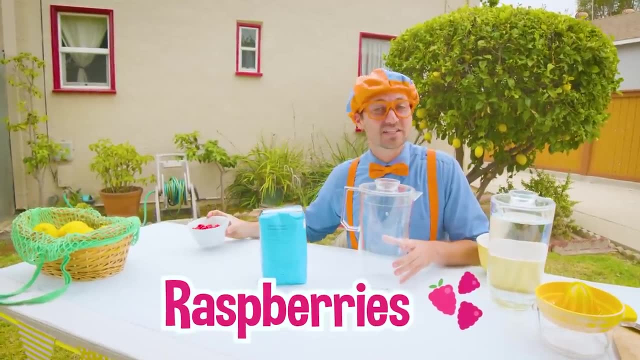 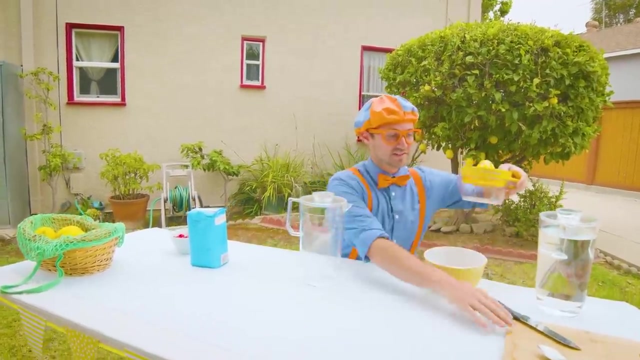 We're going to put a lot of water, sugar, lemons, and we're going to spice it up with a little bit of raspberries to make raspberry lemonade. So the first thing that we need to do is to grab our lemons. 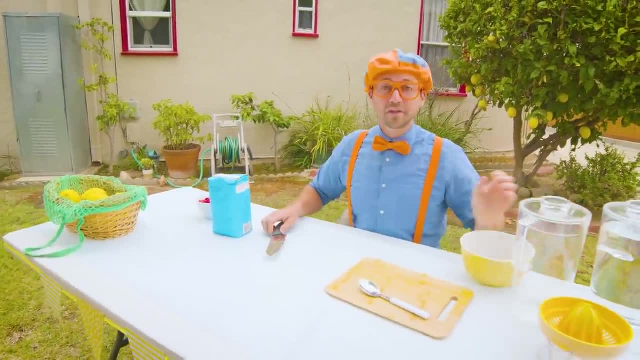 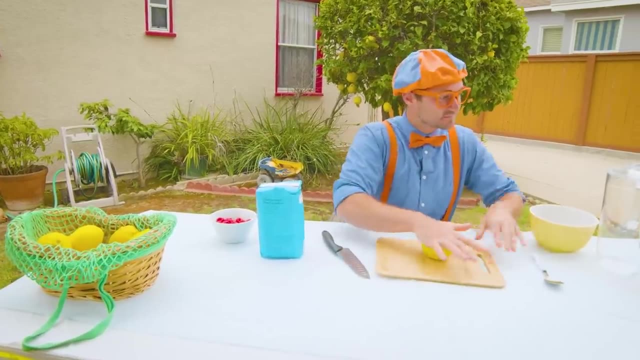 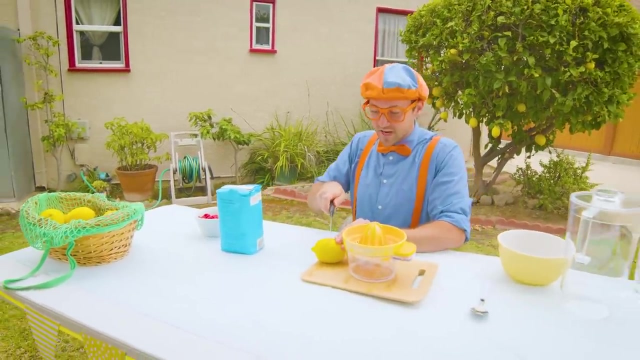 Yeah, all right, And only grown-ups should use a knife. So we're going to first take a lemon, We're going to cut it in half and use this device to squeeze out all of the juice, Just like this Ready. 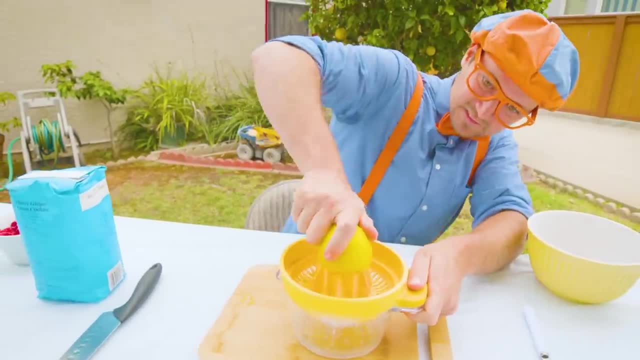 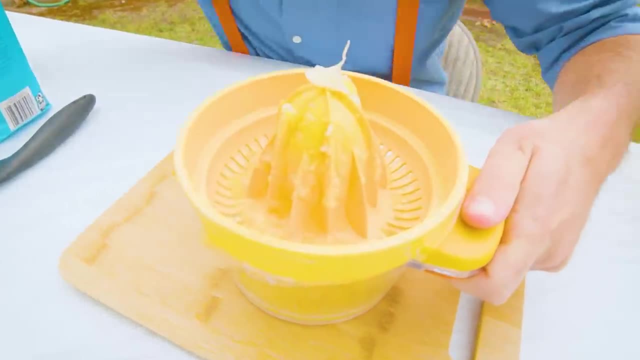 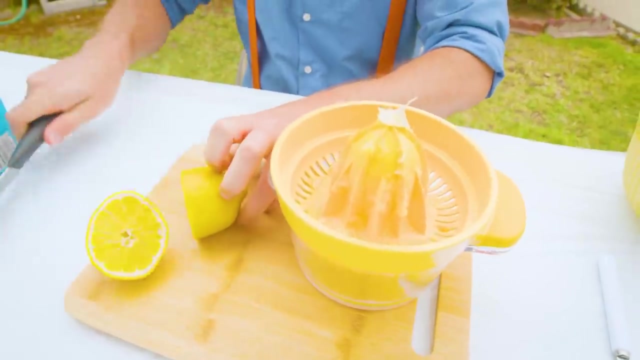 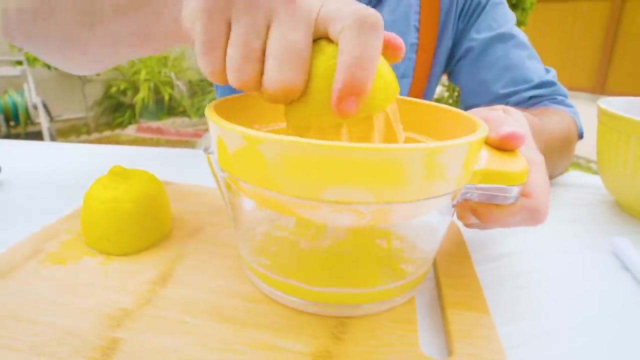 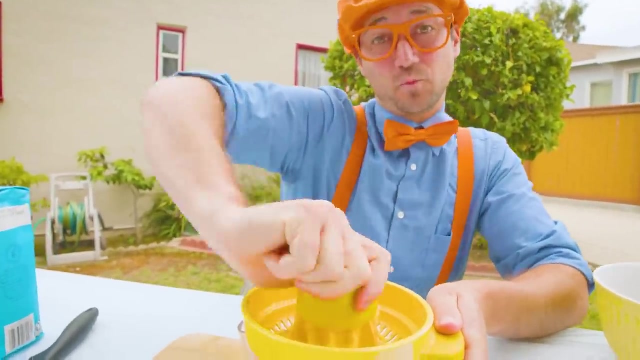 Wow, Wow, Yeah. do you see all that lemon juice down there? Okay, let's do another. Here we go. Whoa, This thing is just pressing out all of the juice. It looks so yummy. I bet it'd be really sour though. 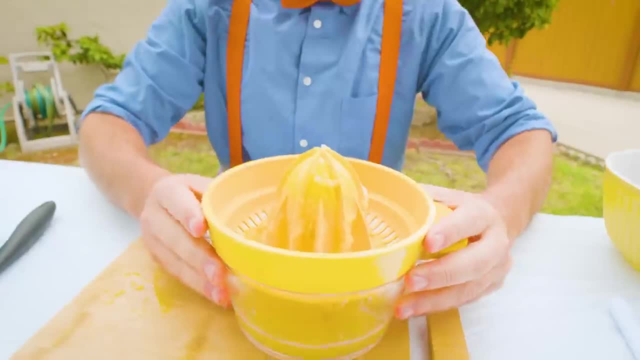 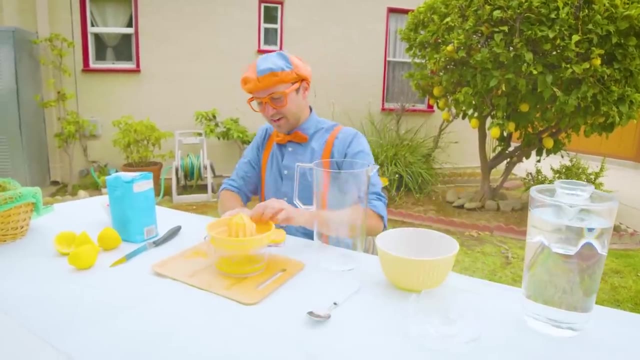 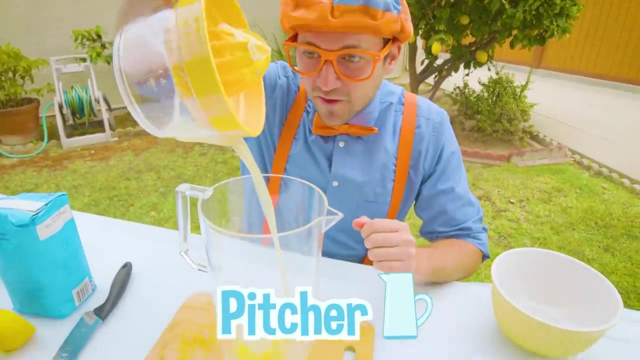 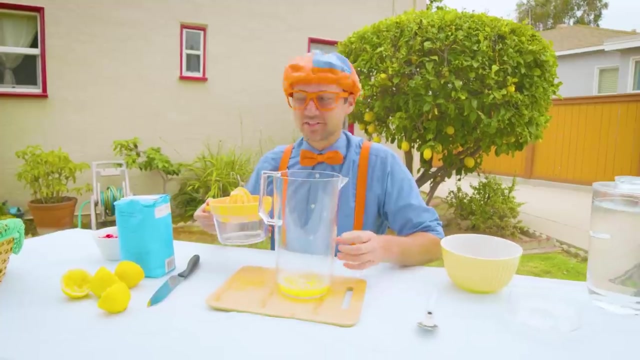 All right, I think that is plenty of lemon juice for our lemons. All right, So we need to now pour this in our giant pitcher. Oh, there we go. All right, it has a little bit of pulp, but that's okay. 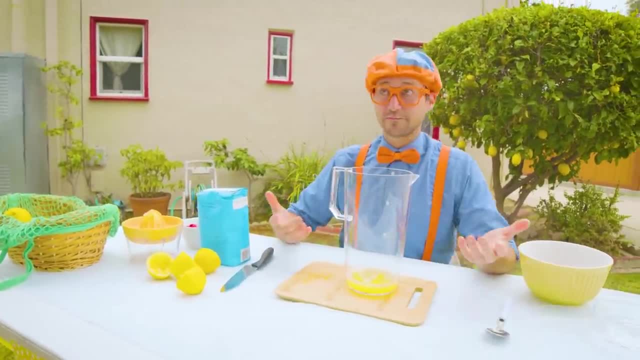 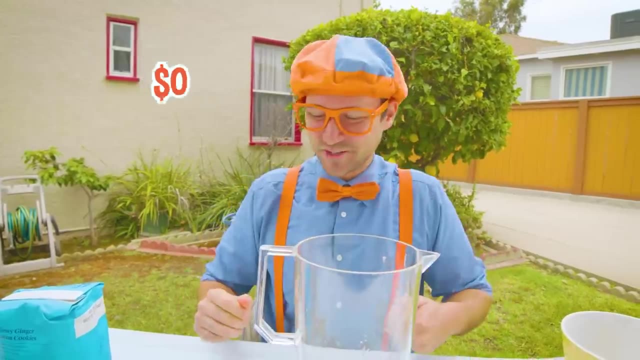 Okay, So the lemons were free, So this cost us zero dollars to make. We're right on track. Okay, The next thing let's get into our lemonade, And the next thing let's add our water. Okay, 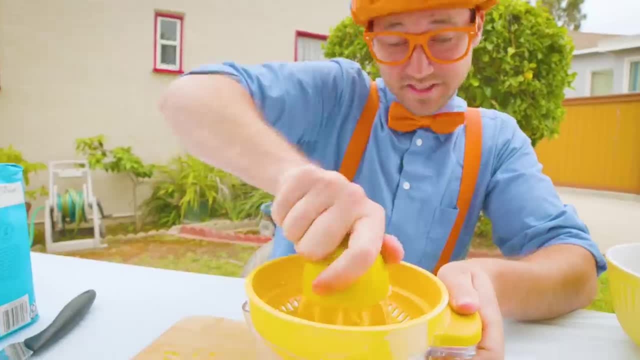 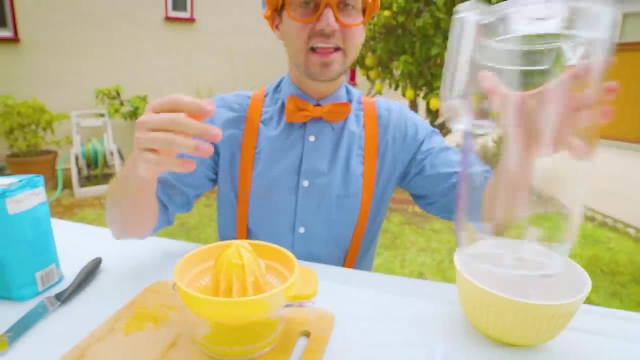 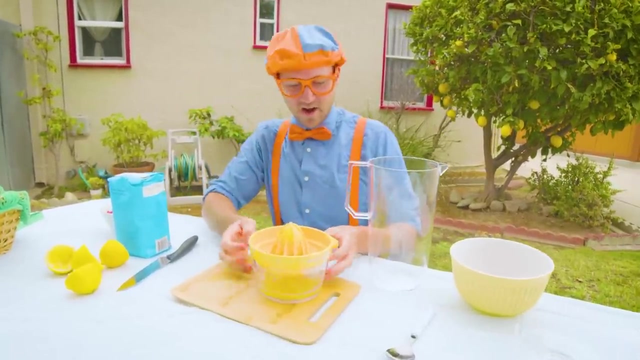 It looks so yummy. I bet it'd be really sour though. All right, I think that is plenty of lemon juice for our lemonade, So let's take a sip. All right, so we need to now pour this in our giant pitcher. 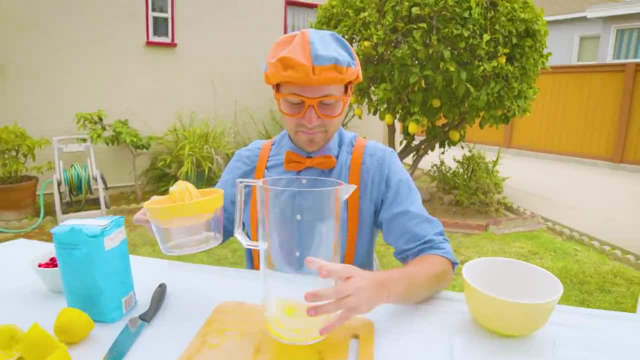 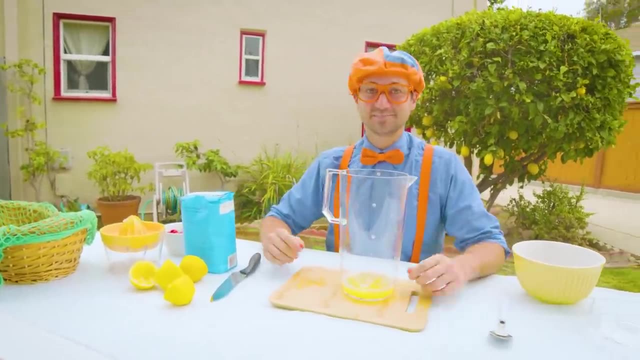 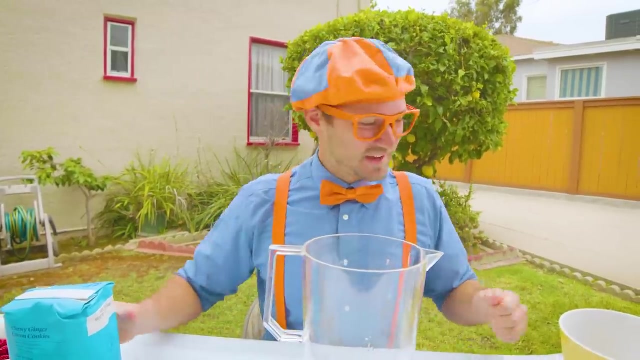 There we go. All right, it has a little bit of pulp, but that's okay. Okay, so the lemons were free, So this cost us zero dollars to make. We're right on track. Okay, the next thing: let's add our water. 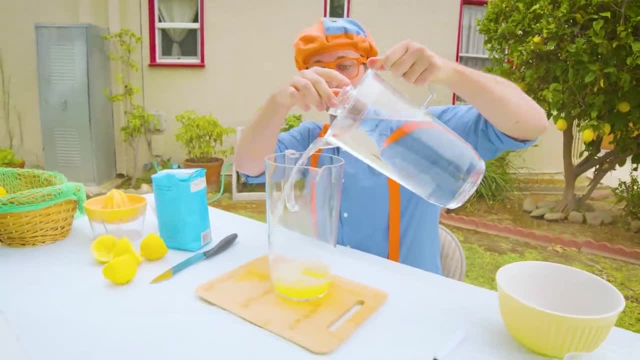 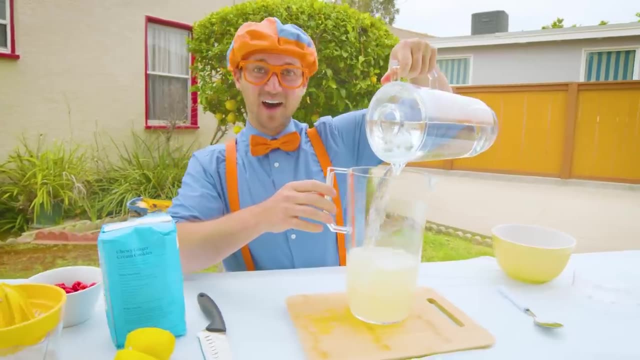 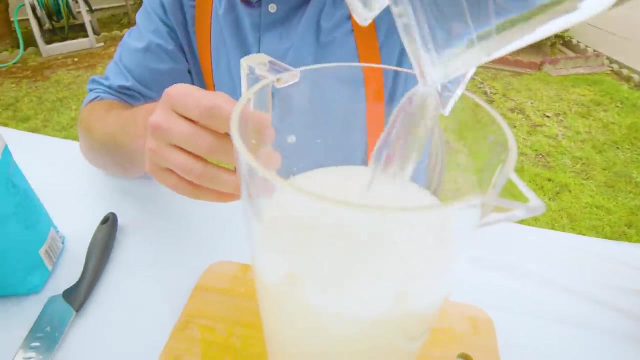 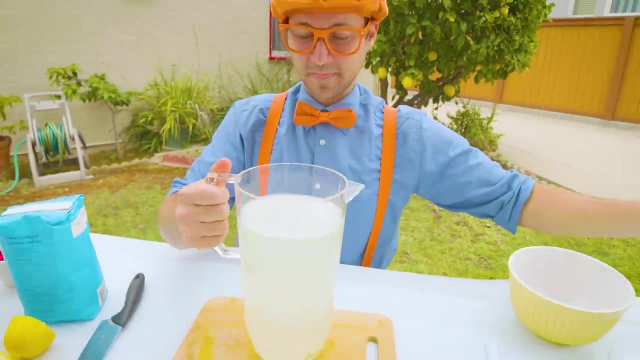 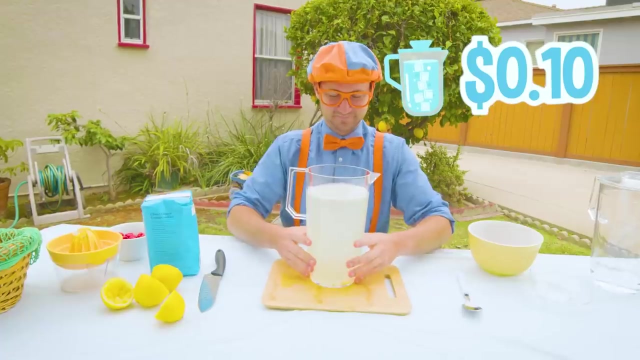 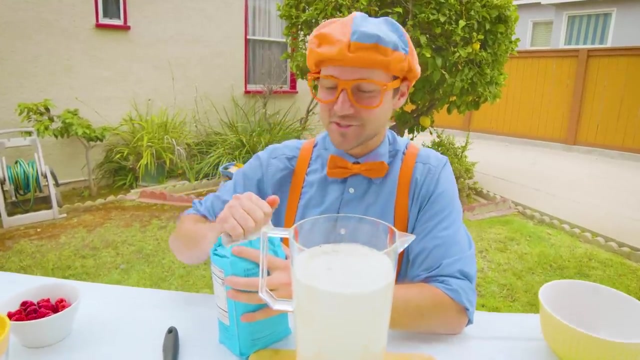 Okay, Whoa, Whoa, Whoa, Oh, that's a perfect amount. Okay, So the lemons were free, The water was 10 cents, Yeah, And now we need to sweeten it up, because this is basically just like watered-down lemon juice. 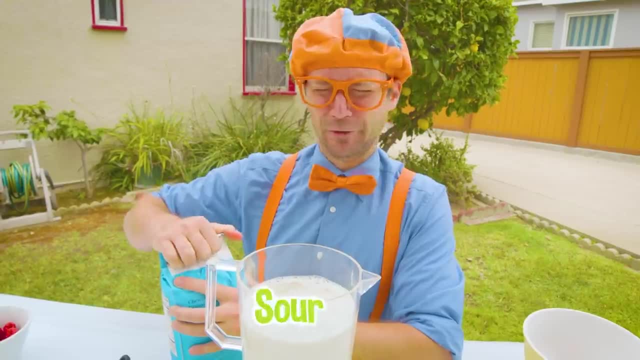 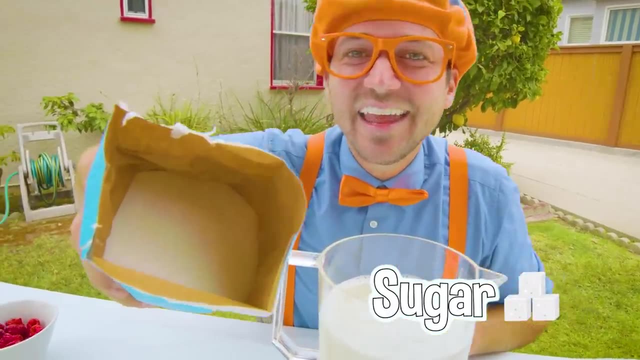 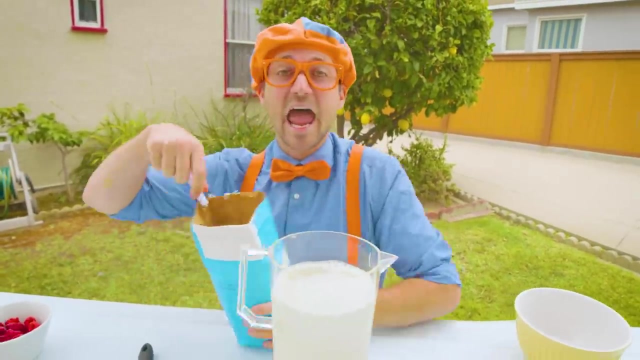 which would be really tart and sour. So what we have right here is sugar. Yeah, That's a really tasty ingredient. You don't want to eat too much sugar, though, But for the lemonade we're going to add six scoops. 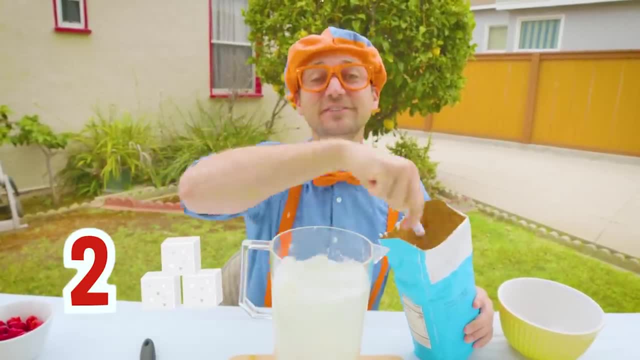 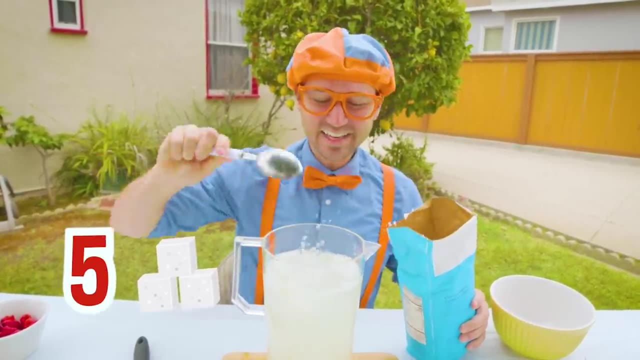 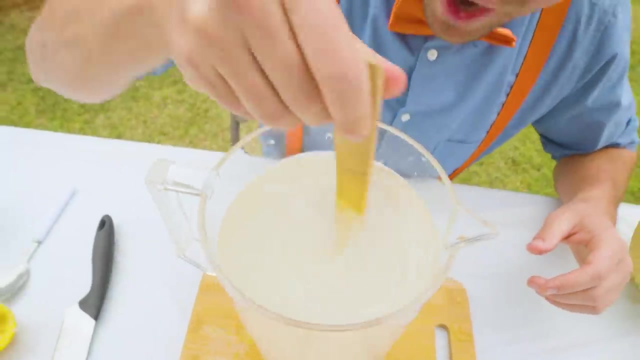 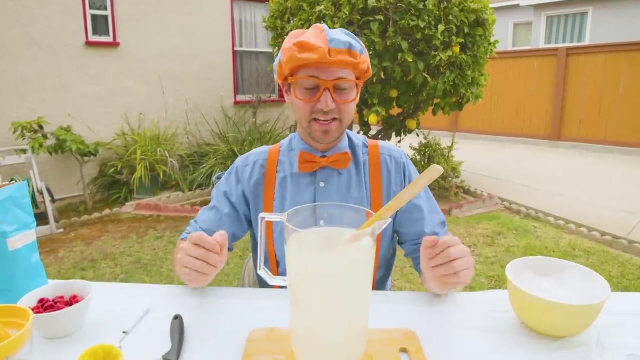 Ready. One, two, three, four, five, six. There we go. Let's put that aside. Here we go. Woo-hoo-hoo, This lemonade is complete. All you really need to make lemonade are lemons, water and sugar. 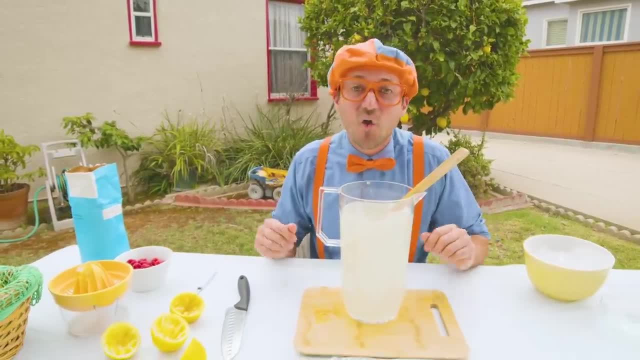 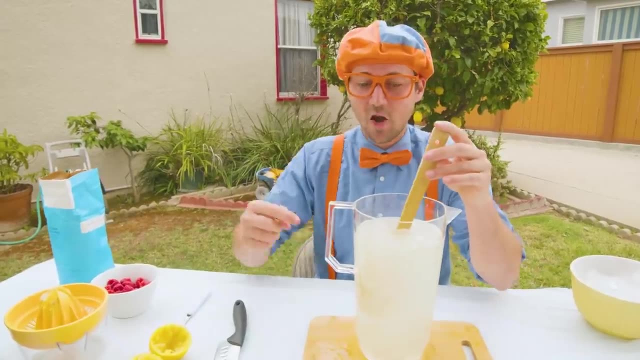 But we have that extra ingredient from earlier, remember Raspberries? Yeah, we're going to make raspberry lemonade, But before we add those, let's calculate how much this lemonade has cost us thus far. Well, the lemons were free. 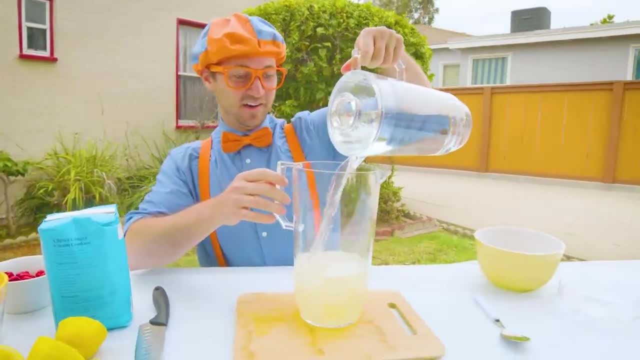 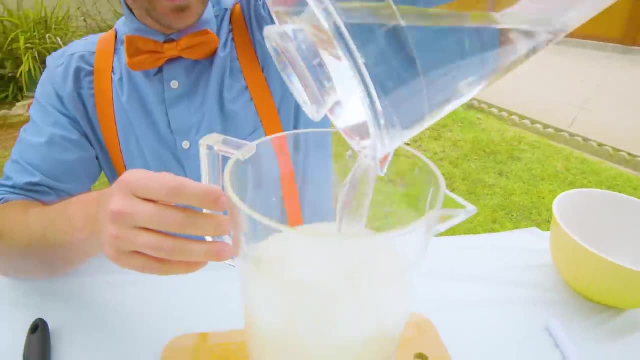 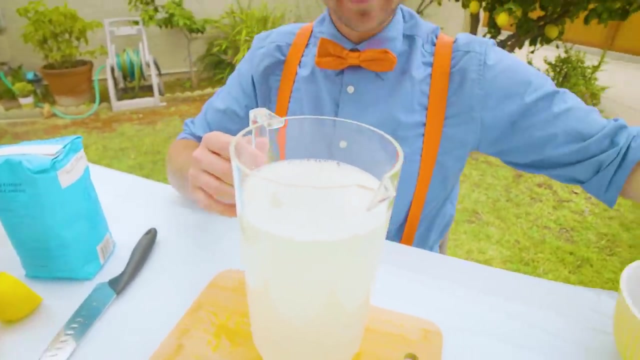 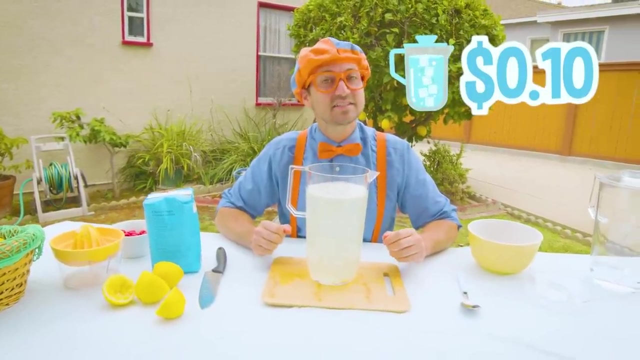 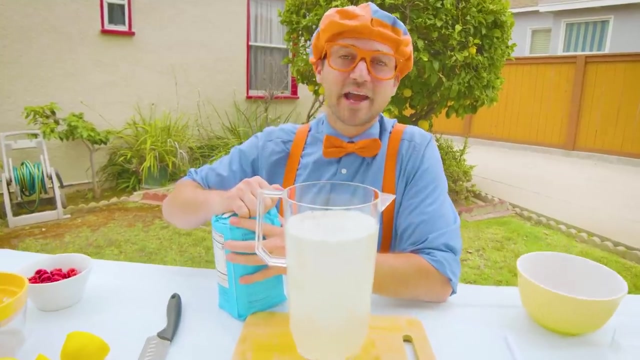 Whoa, Whoa, Whoa. Oh, that's a perfect amount. Okay, So the lemons were free, The water was 10 cents, Yeah, And now we need to sweeten it up, Because this is basically just like watered-down lemon juice. 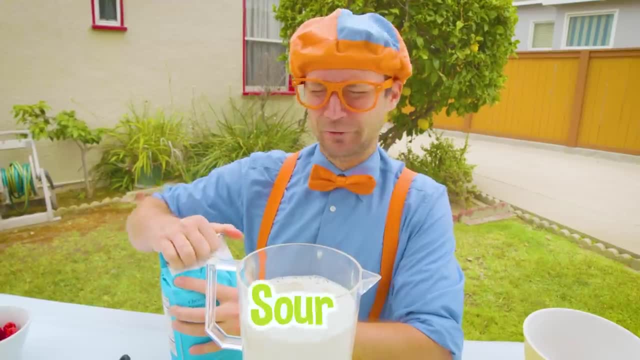 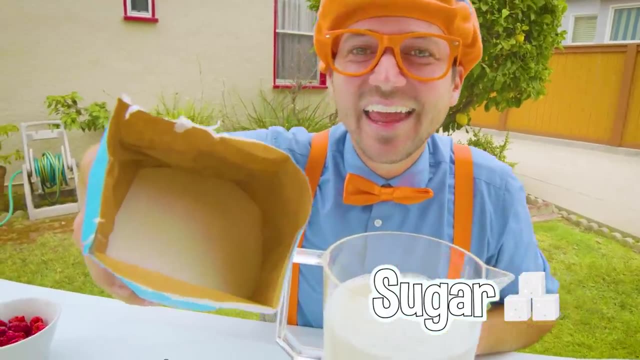 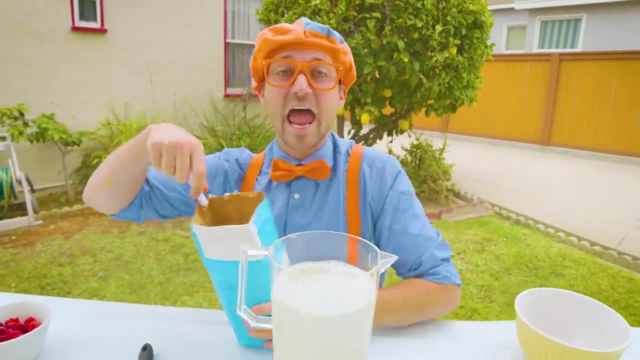 which would be really tart and sour. So what we have right here is sugar. Yeah, that's a really tasty ingredient. You don't want to eat too much sugar, though, But for the lemonade we're going to add six scoops. 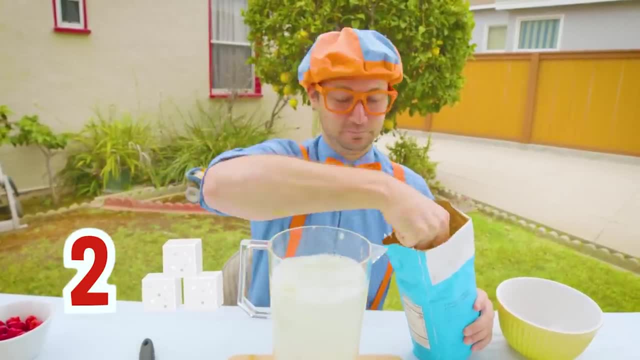 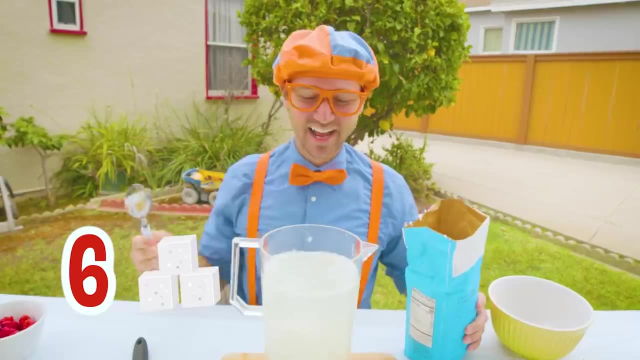 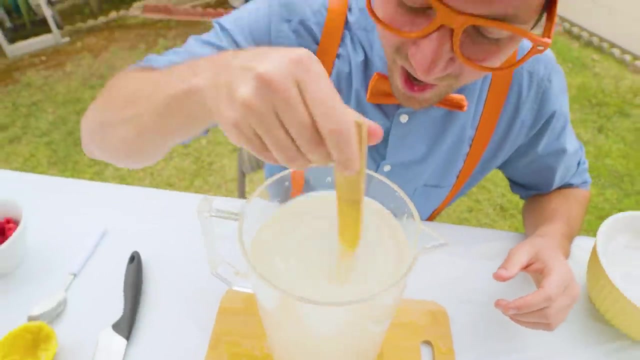 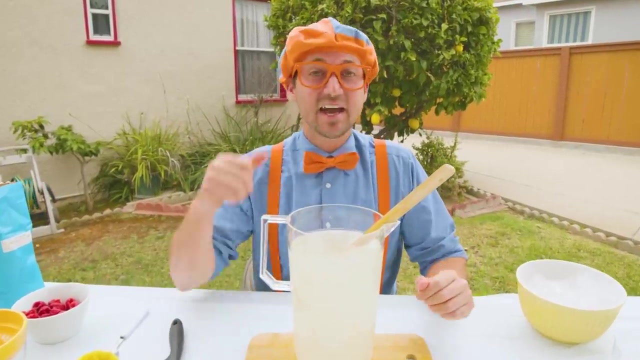 Ready. One, two, three, four, five, six. There we go. Let's put that aside. Here we go. Woo-hoo-hoo, This lemonade is complete. All you really need to make lemonade are lemons, water and sugar. 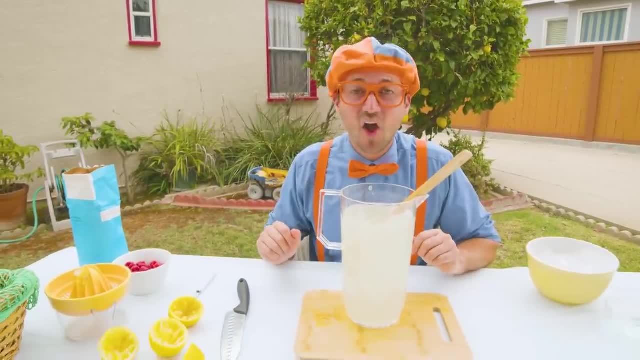 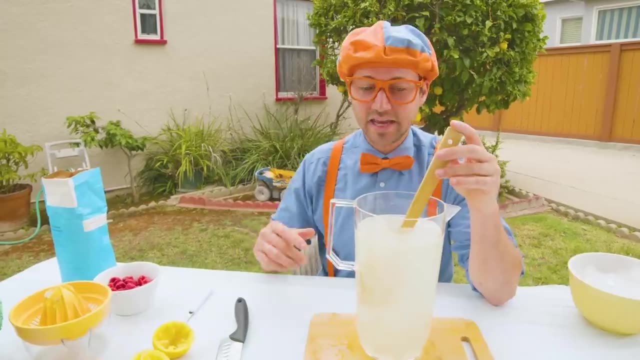 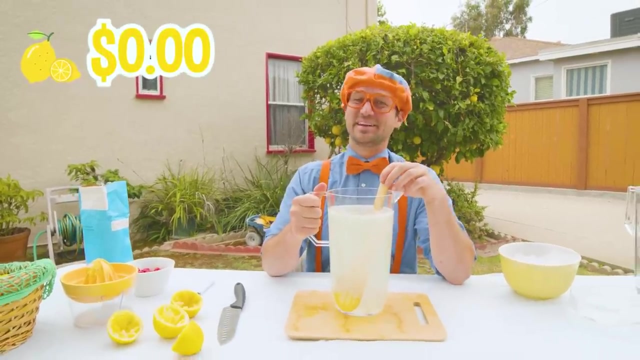 But we have that extra ingredient from earlier. remember Raspberries? Yeah, we're going to make raspberry lemonade, But before we add those, let's calculate how much this lemonade has cost us thus far. Well, the lemons were free because we have a great friend. 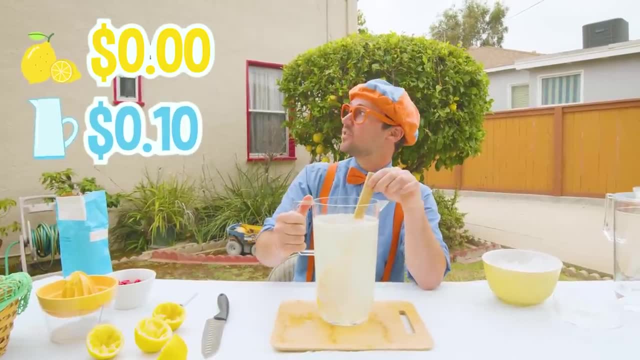 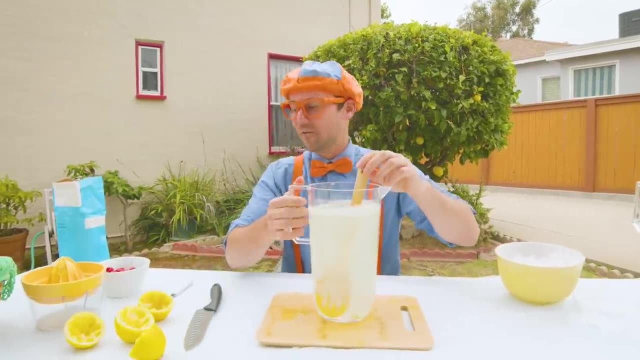 The water was 10 cents And then the sugar was 40 cents, So right now we're at 50 cents for this whole pitcher Whoa. All right, Now we can add our raspberries. Woo, Oh. 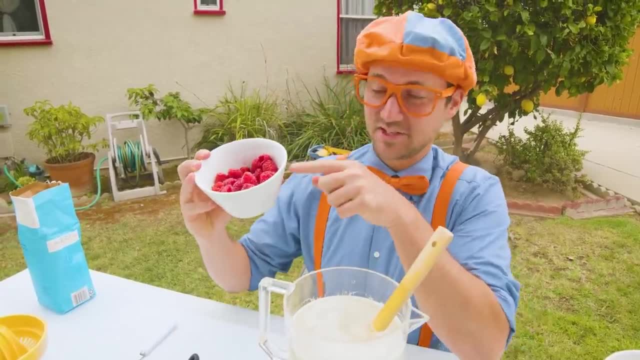 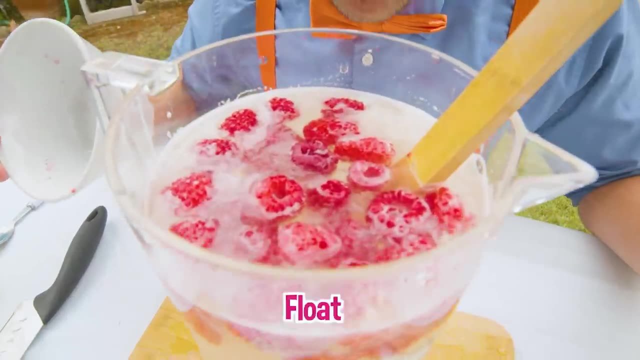 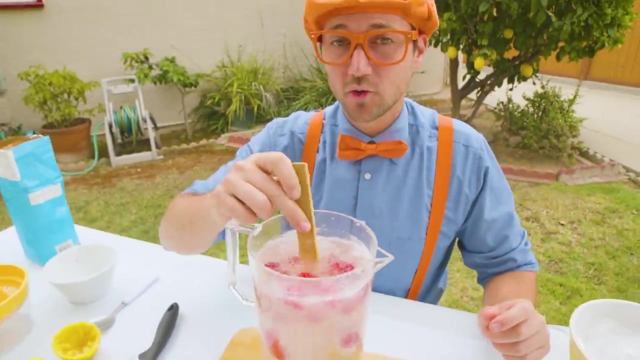 That silly one fell out. I'm not going to touch it, I'm going to just use these. Ready, Here we go. Whoa, Looks like they float Whoa Raspberry lemonade. Okay, So now our total cost. let's calculate. 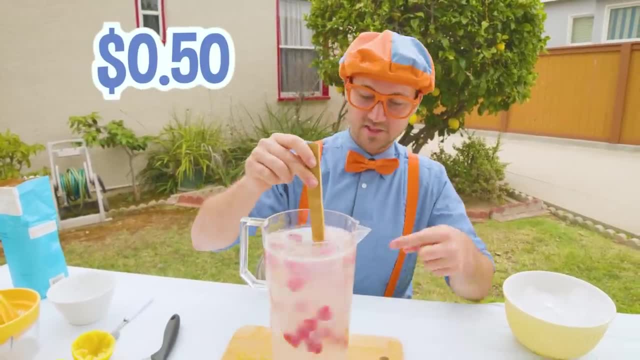 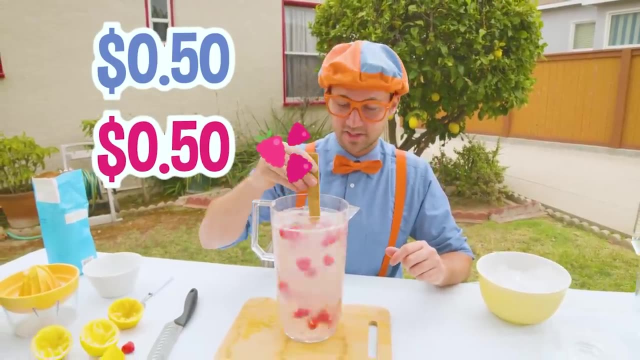 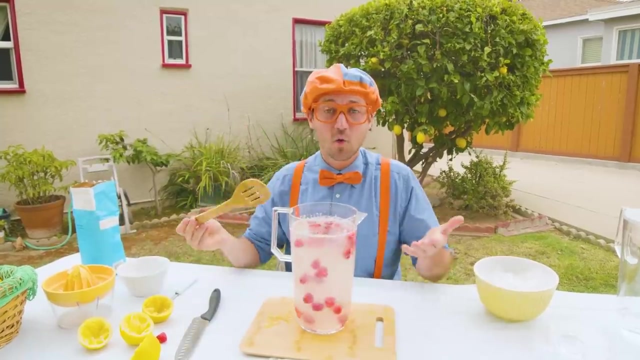 So earlier it was 50 cents And Raspberries cost me 50 cents from the grocery store. So 50 cents plus 50 cents is $1.. Wow, This whole pitcher cost us $1.. All right, 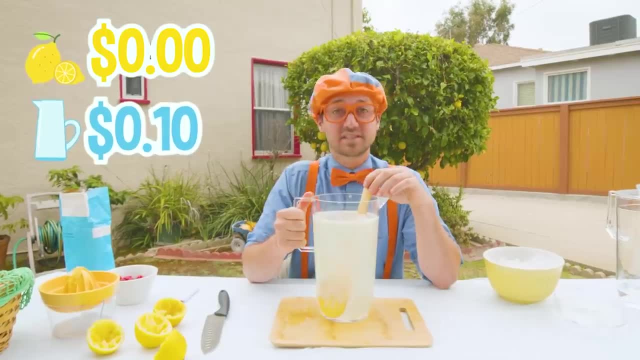 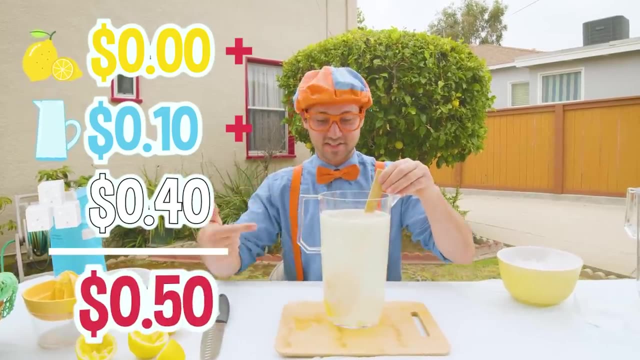 because we have a great friend. The water was 10 cents and then the sugar was 40 cents. Right now we're at 50 cents for this whole pitcher Whoa. All right Now we can add our raspberries. 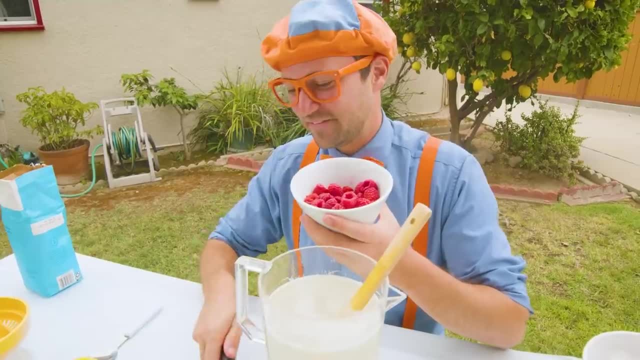 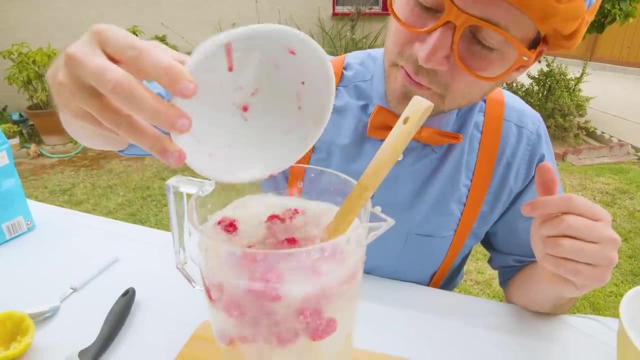 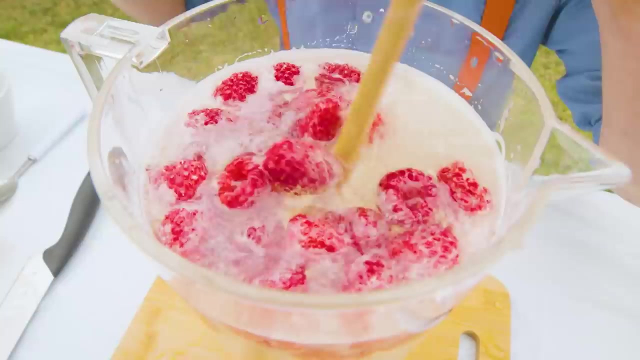 Whoo, Oh, That silly one fell out. I'm not going to touch it, I'm going to just use these. Ready, Here we go. Whoa, Looks like they float Whoa Raspberry lemonade. Okay, So now our total cost. let's calculate. 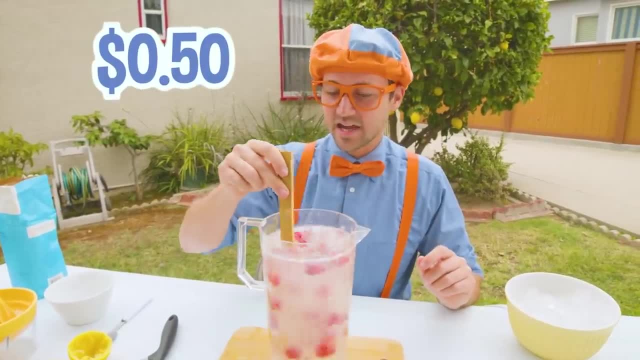 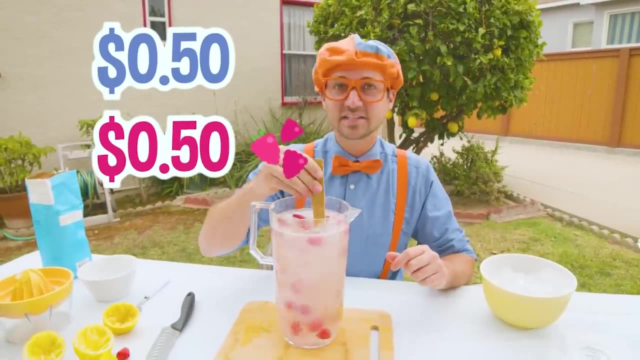 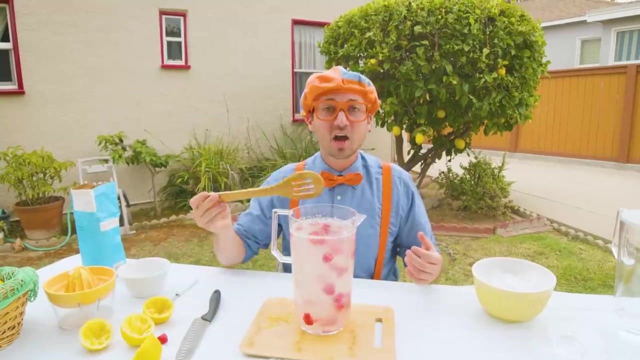 So earlier it was 50 cents And these raspberries cost me 50 cents from the grocery store. So 50 cents plus 50 cents is $1.. Wow, This whole pitcher cost us $1.. All right, Let's put in some ice. 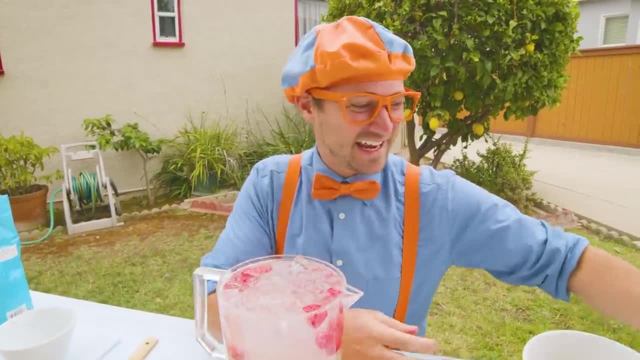 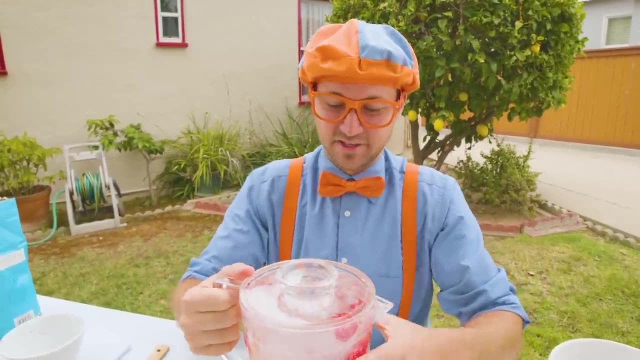 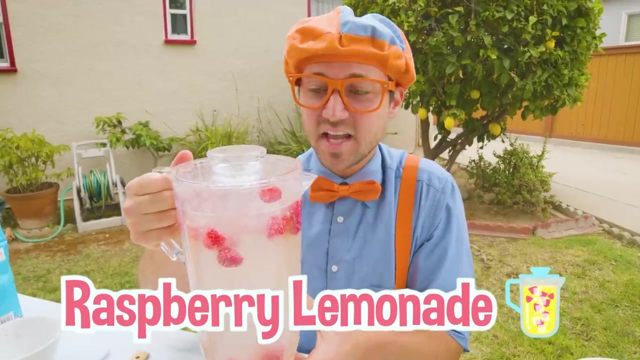 Whoa To chill it down, So then we can go and sell it. The ice was free because our friend also has a freezer full of ice. So now that we have nice cold lemonade- raspberry lemonade- we can go and sell it. 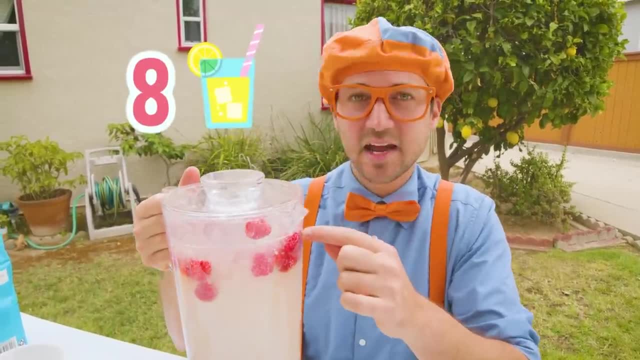 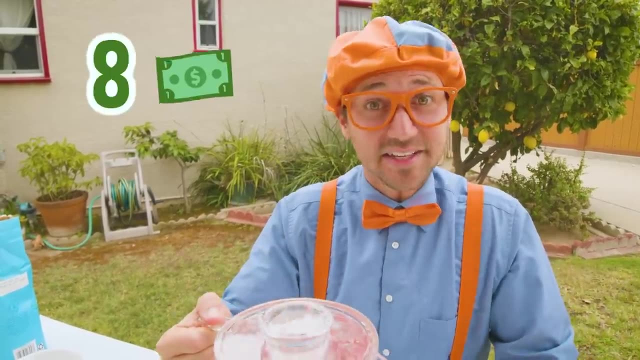 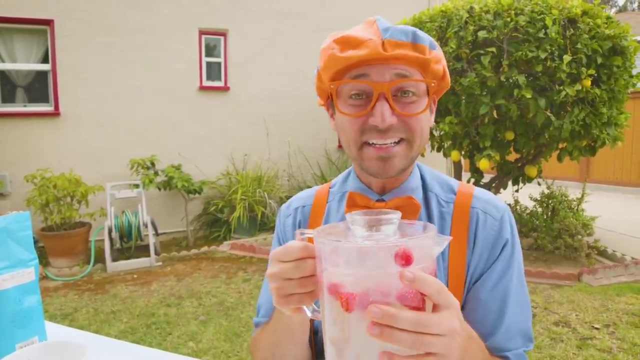 I think there's about eight cups in here And our cost is $1.. So eight cups, if we sell them for $1, would be $8. And if we minus $1, that's $7.. Whoa, We're going to make $7.. 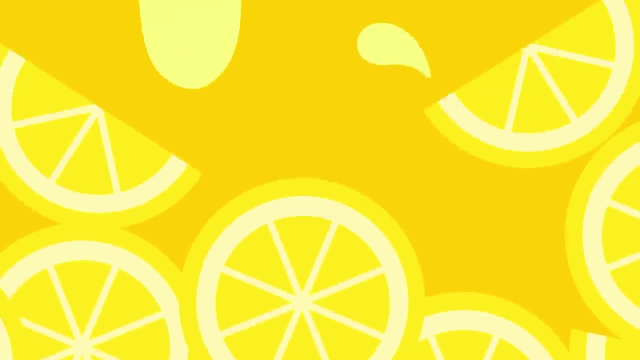 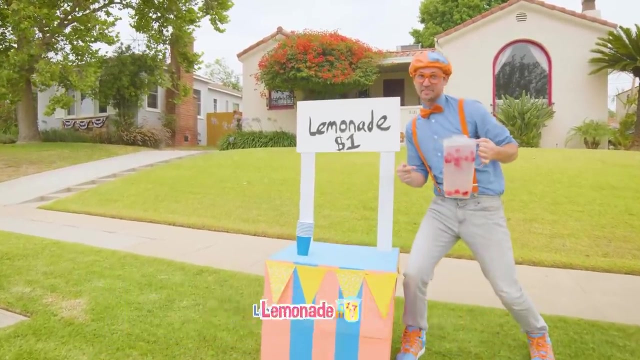 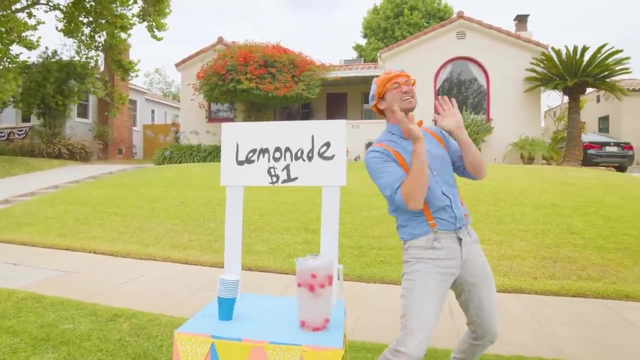 Let's go. Whoa, We did it. We built this amazing lemonade stand. We made some tasty lemonade. Yeah, Now it's time to sell some lemonade. Here we go: Lemonade, Lemonade. Who wants some lemonade? 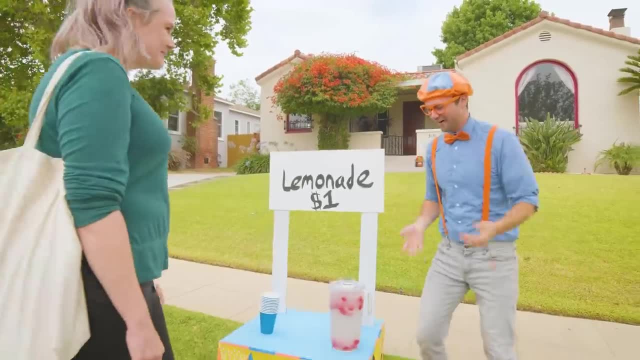 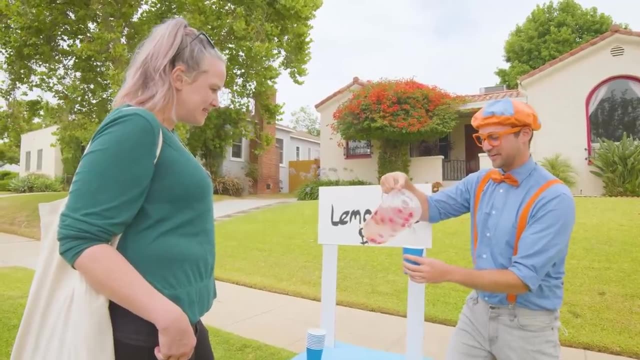 I'd love some lemonade. Oh, okay, How are you doing today? Good, I'm a little thirsty. Ooh, really. Well, it looks like I might have something just for me. Oh, fantastic, How much is it? 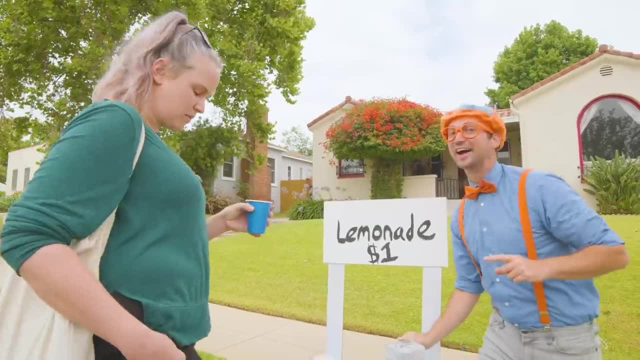 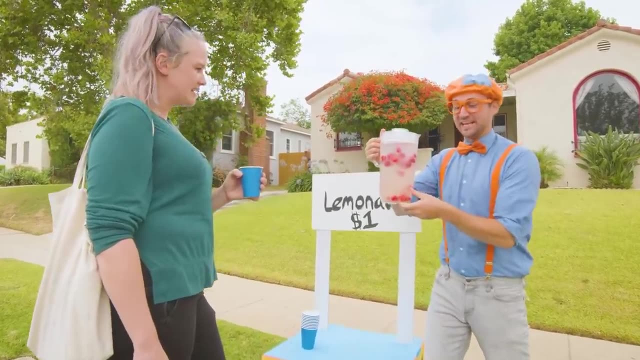 It is $1.. $1? I got that right here. Amazing, Thank you. What kind is this? This is not normal lemonade. It is raspberry lemonade, My favorite. I can't wait to try. Thank you, All right. 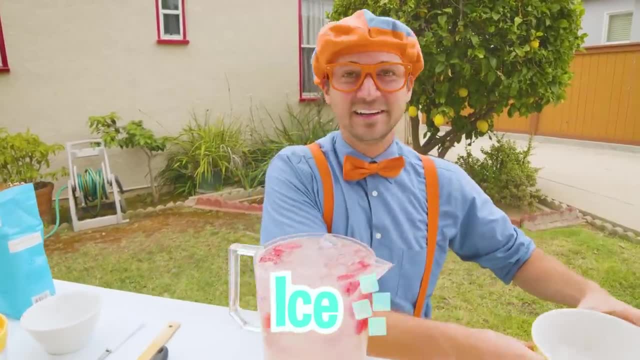 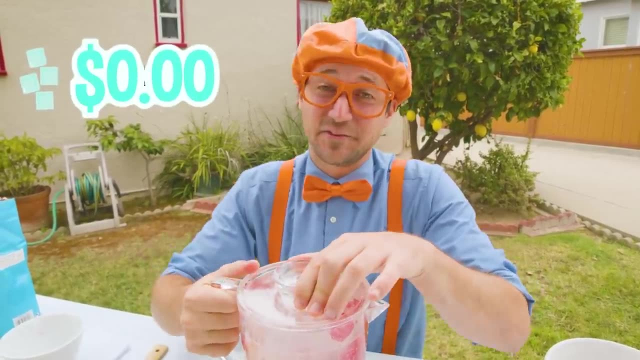 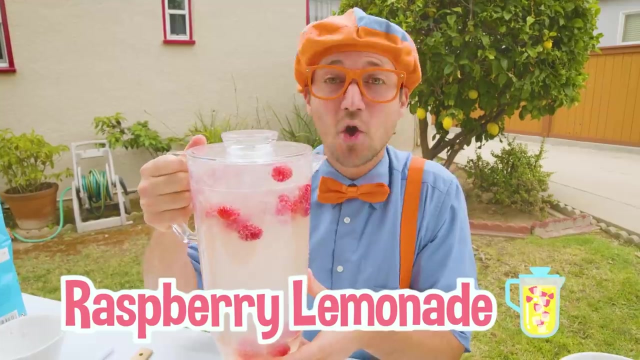 Let's put in some ice Whoa Whoa To chill it down, So then we can go and sell it. The ice was free because our friend also has a freezer full of ice. So Now that we have nice cold lemonade- raspberry lemonade. 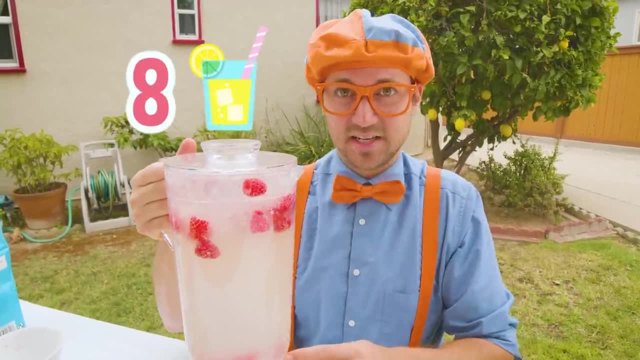 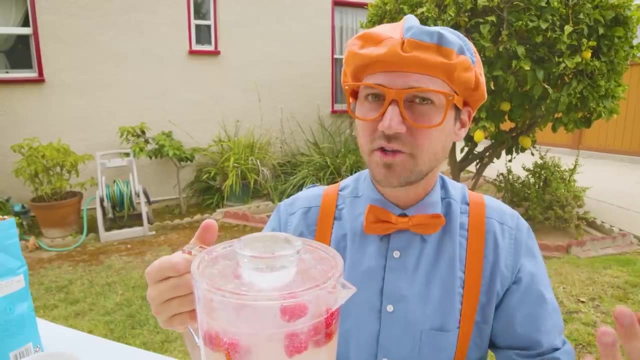 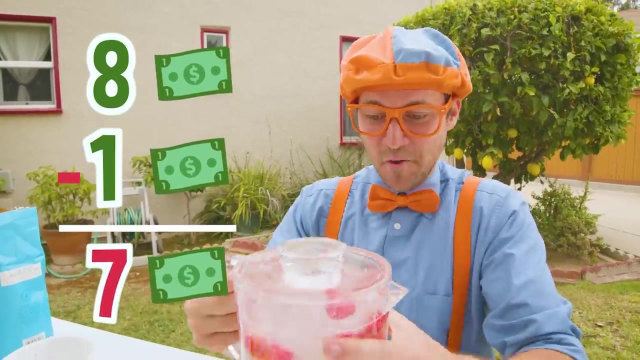 we can go and sell it. I think there's about eight cups in here And our cost is $1.. So eight cups, if we sell them for $1, would be $8. And if we minus $1, that's $7.. 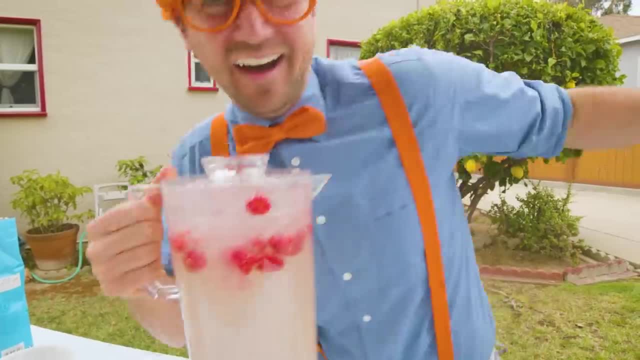 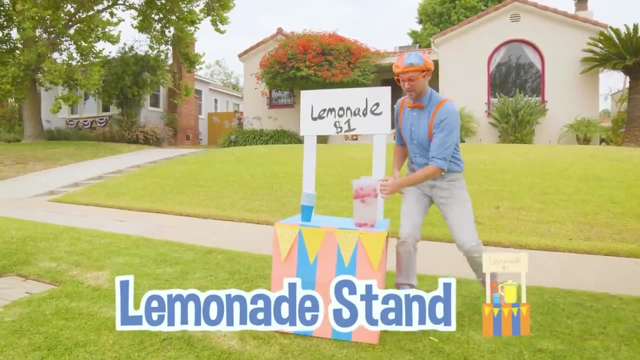 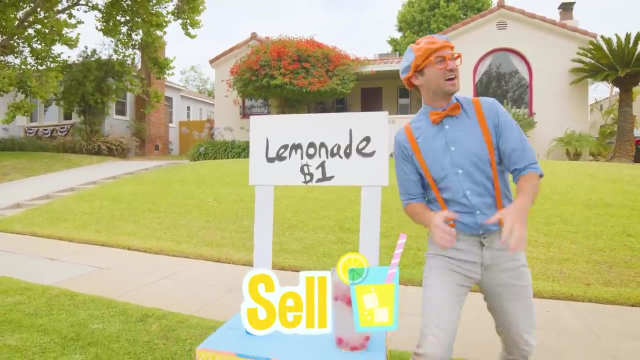 Whoa, We're going to make $7.. Let's go. Whoa, We did it. We built this amazing lemonade stand. We made some tasty lemonade. Yeah, Now it's time to sell some lemonade. Here we go. 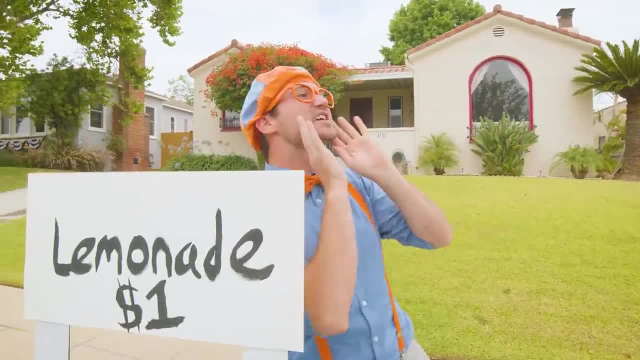 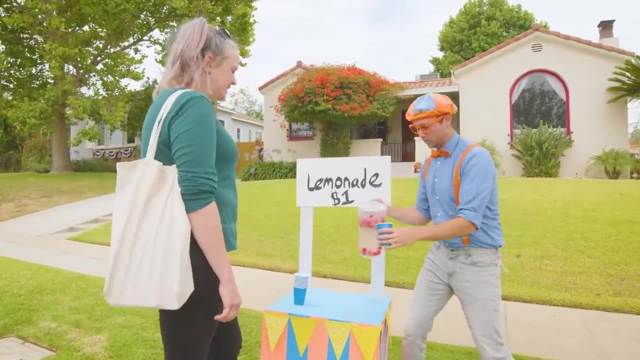 Lemonade, Lemonade. Who wants some lemonade? I'd love some lemonade. Oh okay, How are you doing today? Good, I'm a little thirsty, Oh, really. Well, it looks like I might have something just for you. 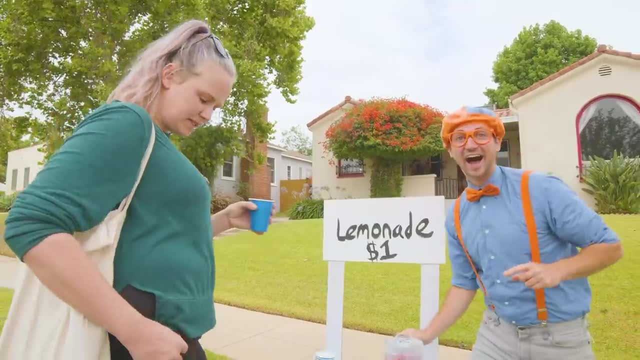 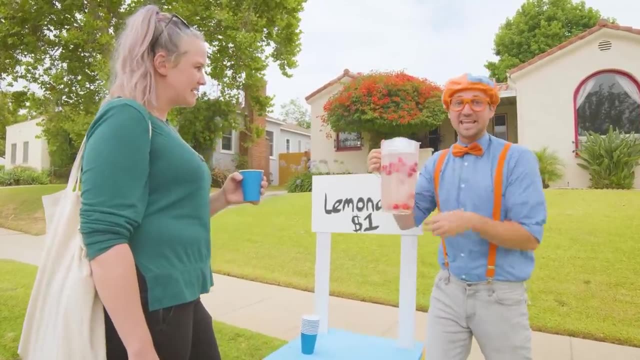 Oh fantastic. How much is it? It is $1.. $1?. I got that right here. Oh amazing, Thank you. What kind is this? This is not normal lemonade. It is raspberry lemonade, My favorite. 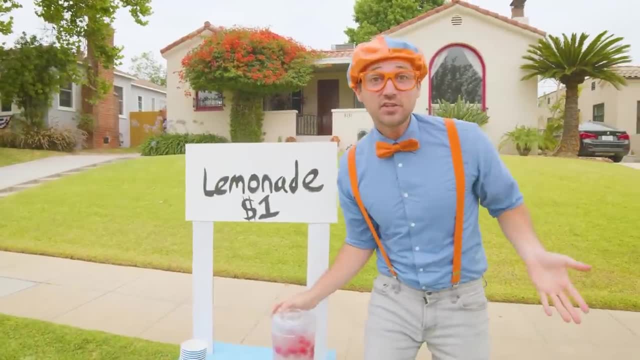 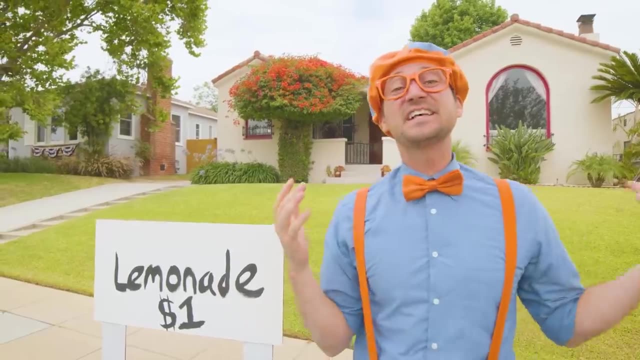 I can't wait to try. Thank you All right, See you later. Bye, Did you see that You and I just made our very first lemonade sale? Good job, Well, this has been so much fun learning about business. 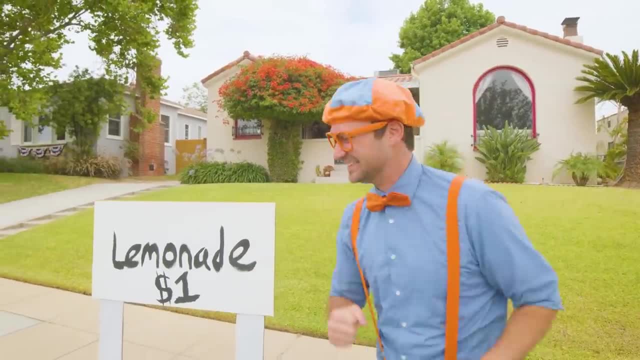 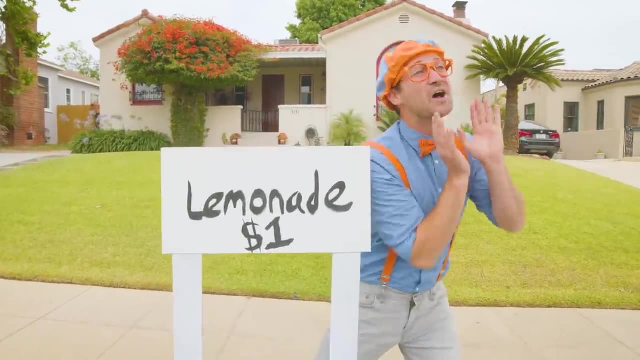 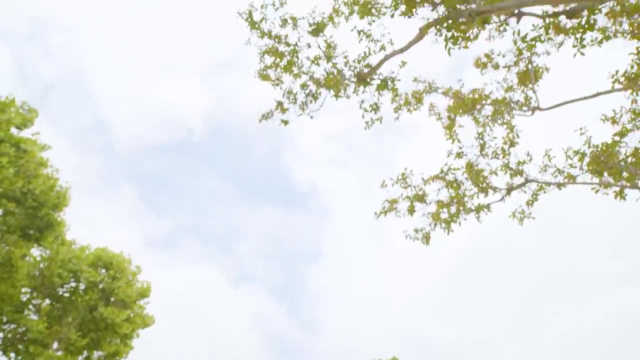 how to make lemonade with you and having fun along the way. Well, time to sell some more lemonade, Lemonade, Lemonade. Who wants some lemonade? Woohoo, Yeah, Blippi. So much to learn about. 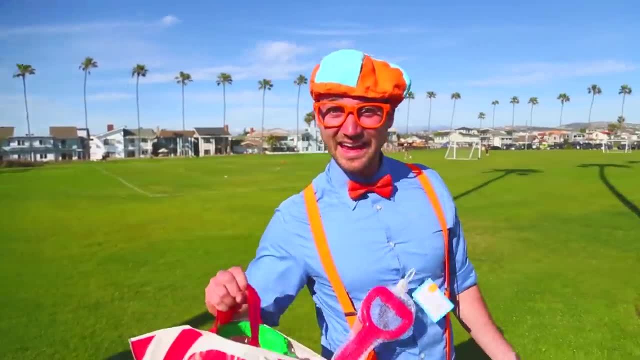 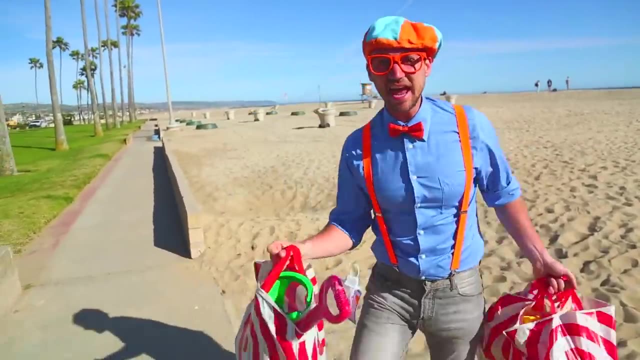 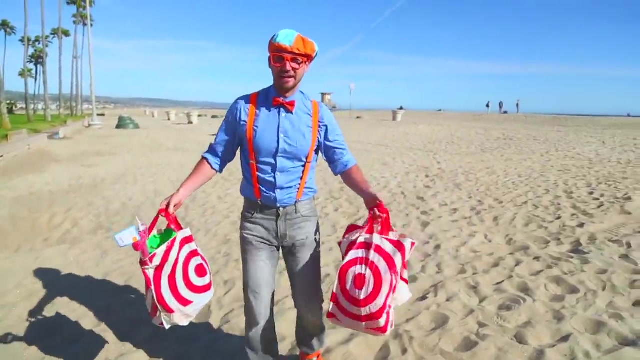 It'll make you want to shout Blippi. Hey, look at what I have. Ooh, I have some bags of sand toys And today we are going to play in the sand. Whoa, Whoa. Okay, first things first. 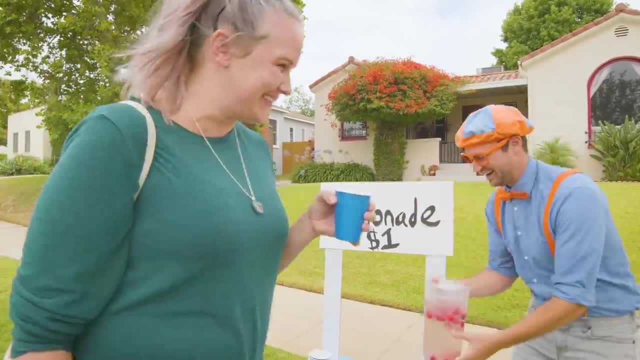 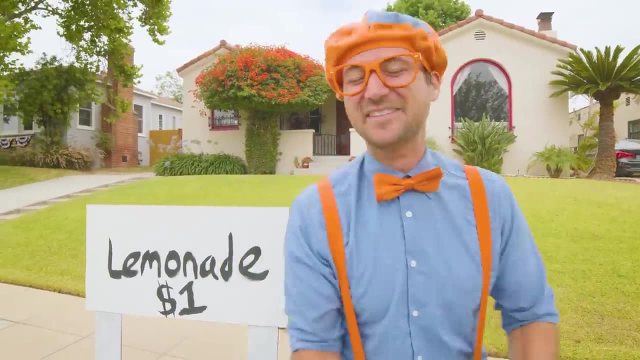 See you later. Bye, Did you see that You and I just made our very first lemonade sale? Good job. Well, this has been so much fun learning about business, how to make lemonade and how to make lemonade. 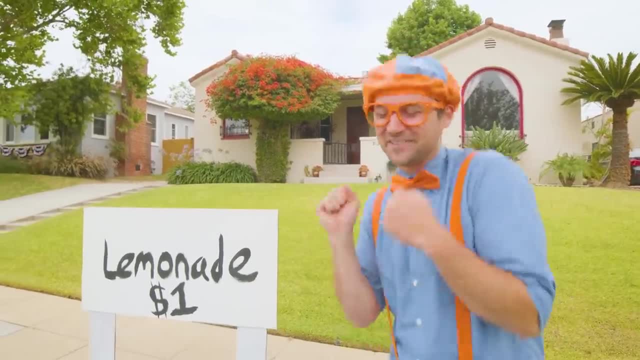 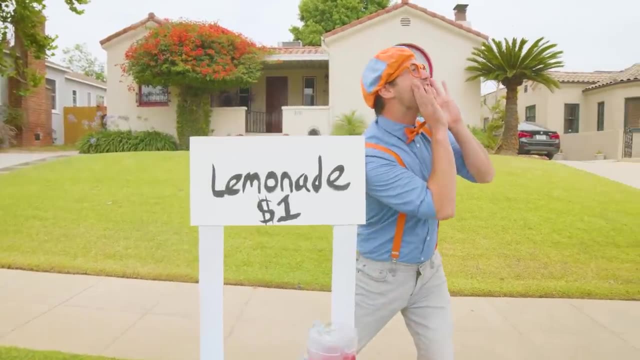 And having fun along the way. Well, time to sell some more lemonade, Lemonade, Lemonade. Who wants some lemonade? Yeah, So much to learn about. It'll make you want to shout Blippi. Hey, Look at what I have. 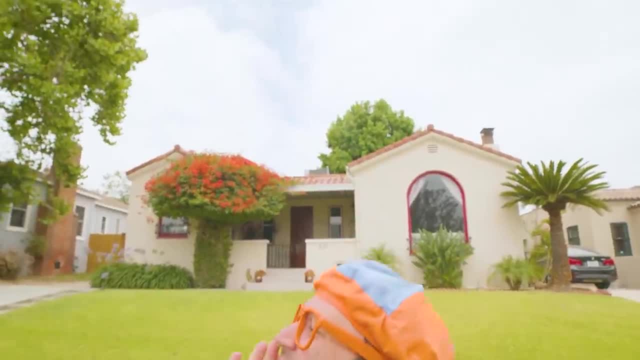 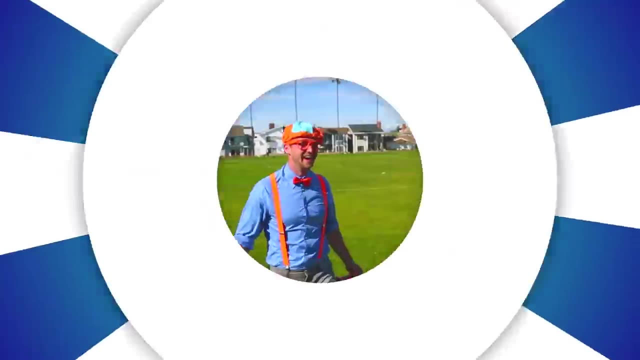 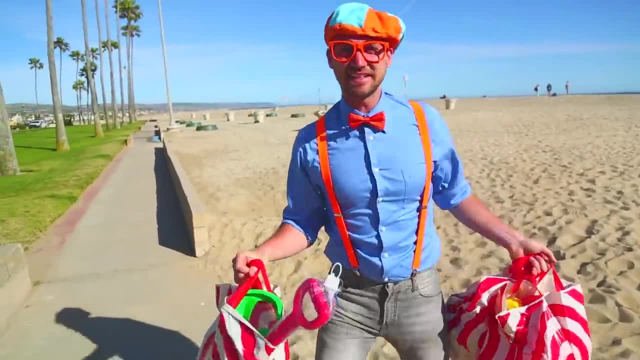 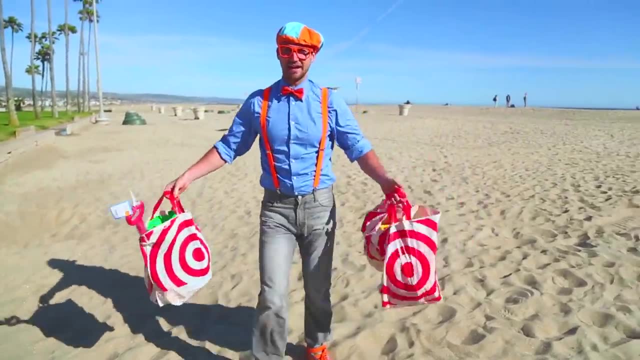 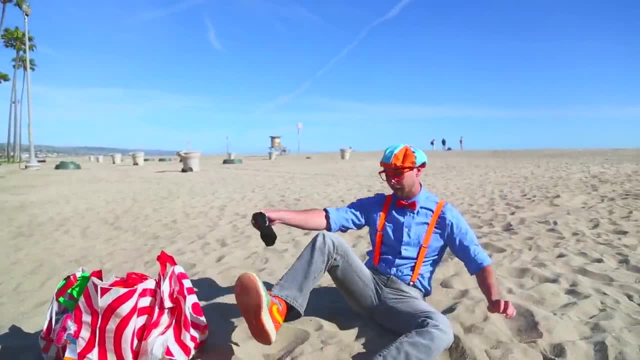 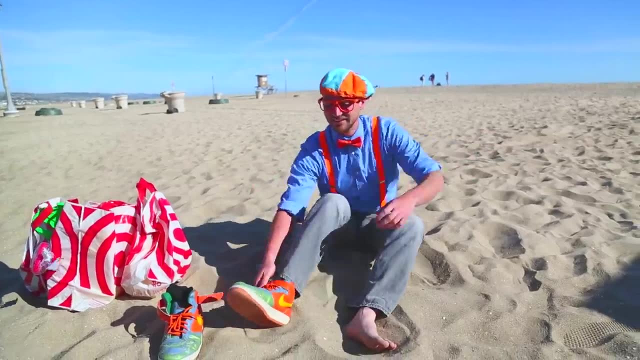 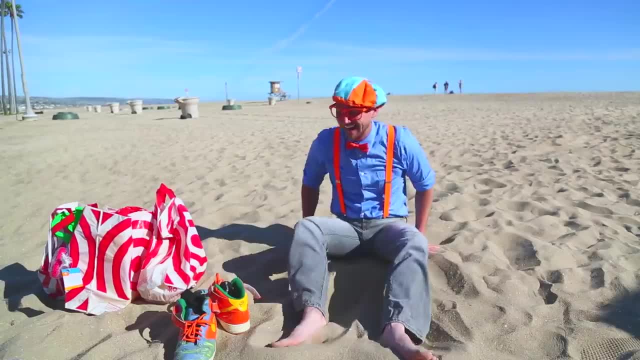 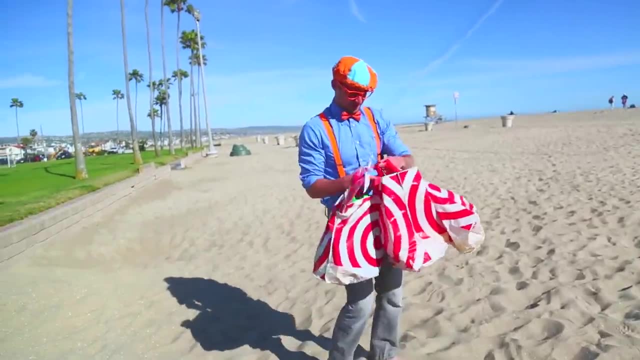 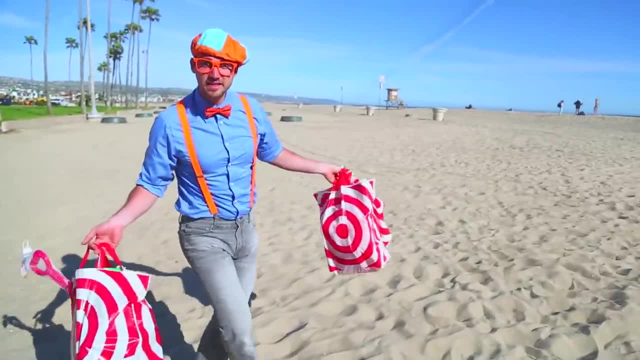 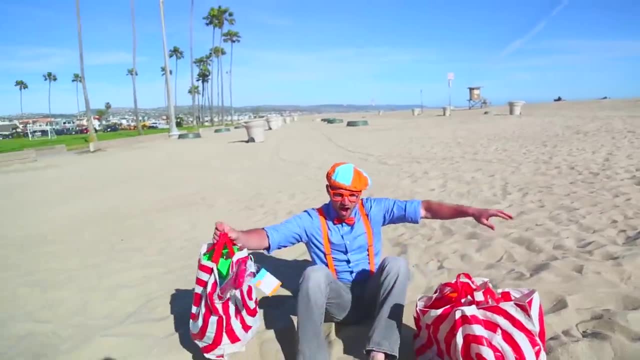 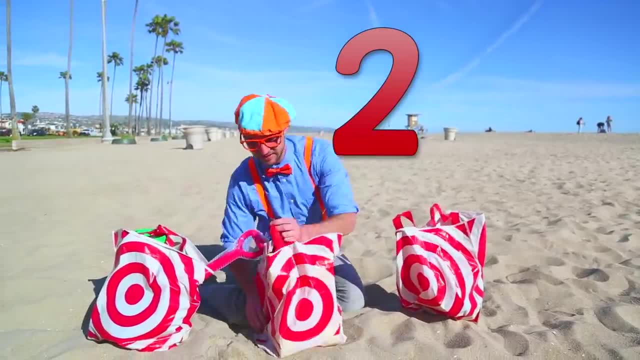 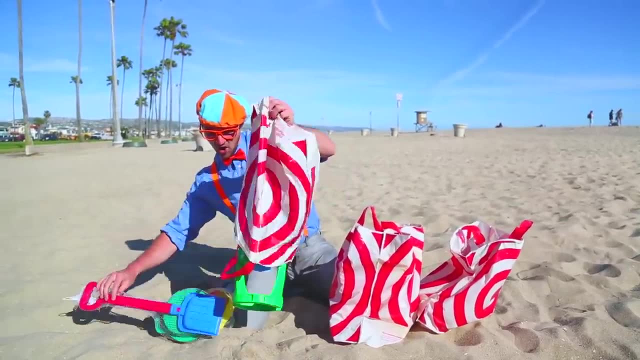 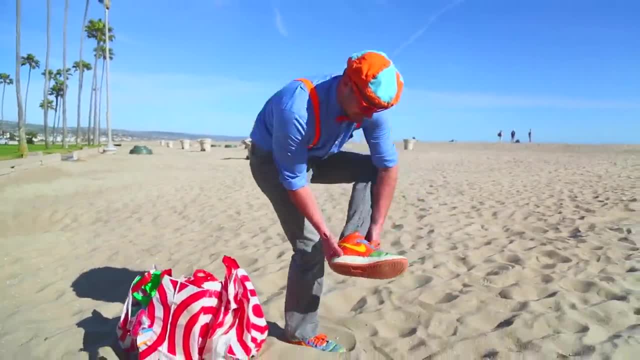 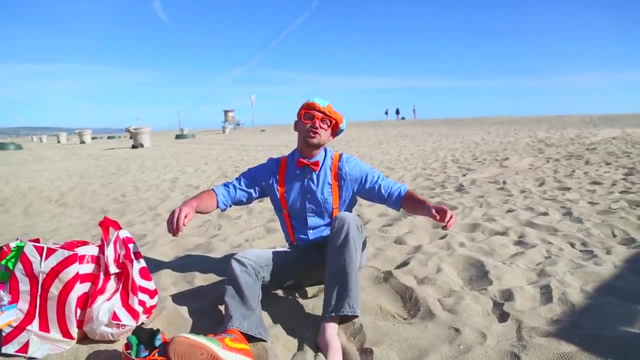 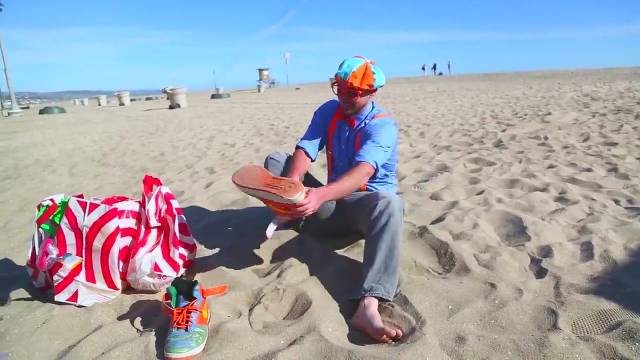 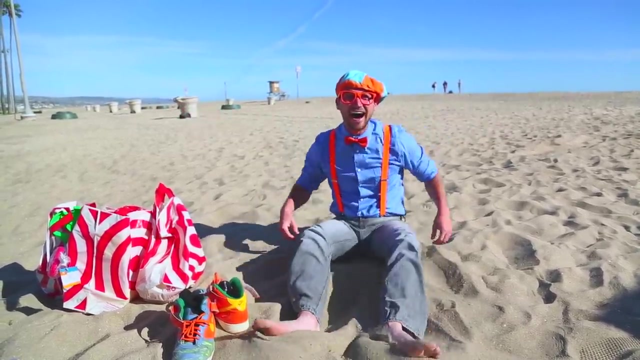 Let's take off our shoes. The reason why I'm taking off my shoes, Whoa, is because Sam feels so good on my feet, Whoa, Okay, now my other shoe. Ah, yes, Ah, Whee, Whee. 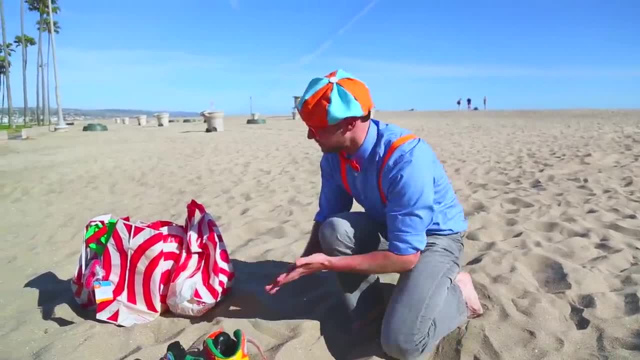 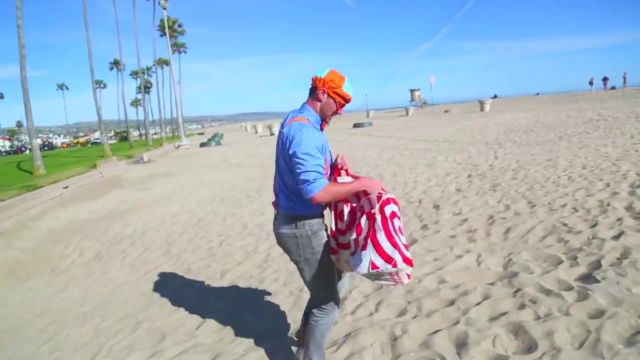 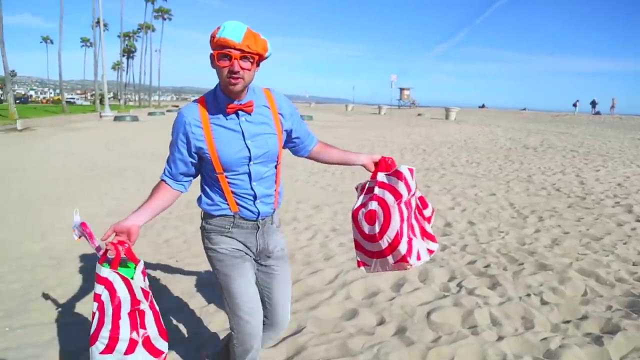 Ha ha ha. Okay, I'll leave my shoes right here And let me grab the bags and let's go out in the sand. I am so excited to show you all the sand toys that I have. Does this look like a good spot? 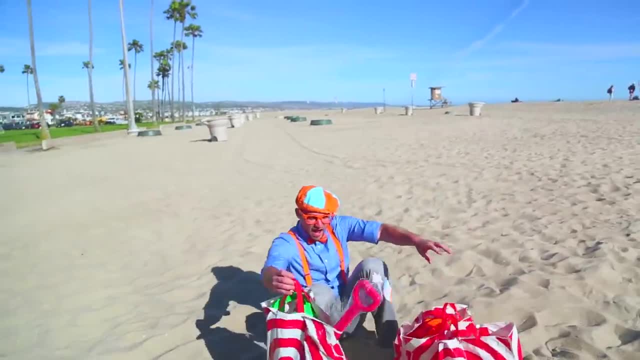 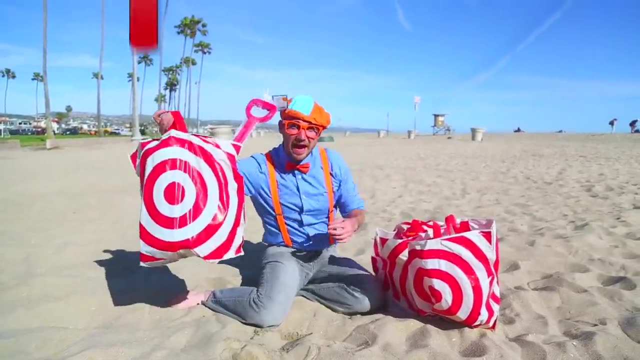 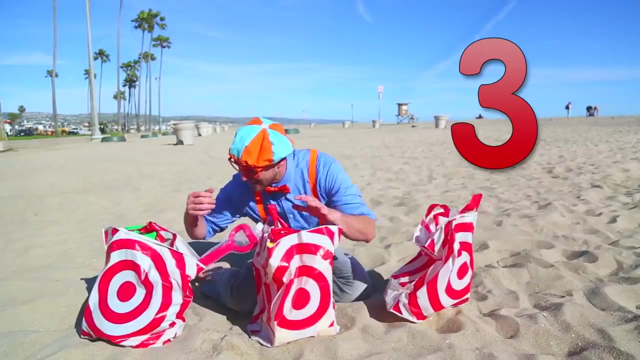 I think so. Okay, look Like I said, I feel so good on my feet. Okay, I have one bag, I have two bags, Two bags And three bags. Okay, let's see what we have in here. Oh, ho, ho ho. 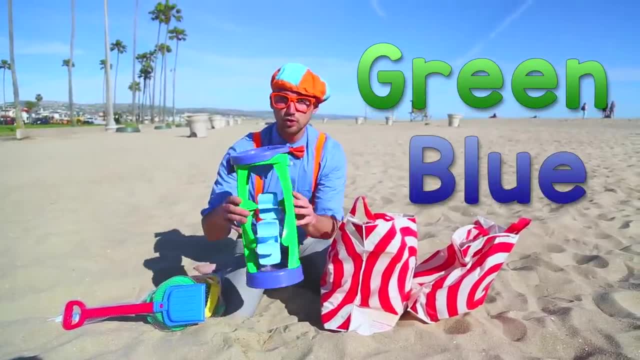 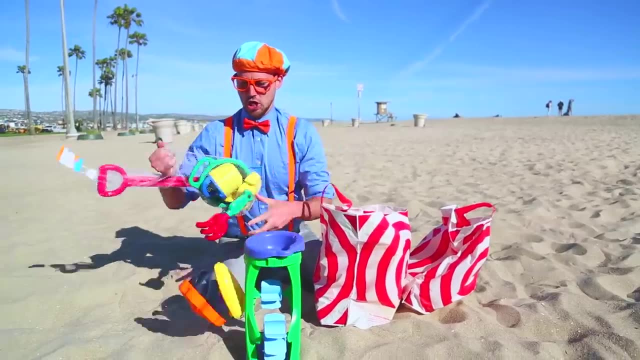 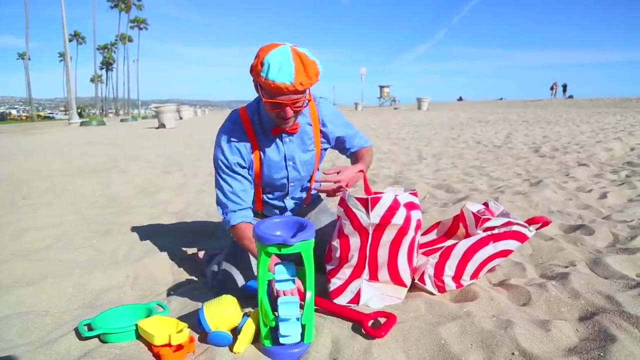 Okay, the first bag has a green and blue toy. We'll play with that in just a little bit. And then Whoa, Oh, ho, ho, ho. This has so many other toys in it, Like the shovel, And 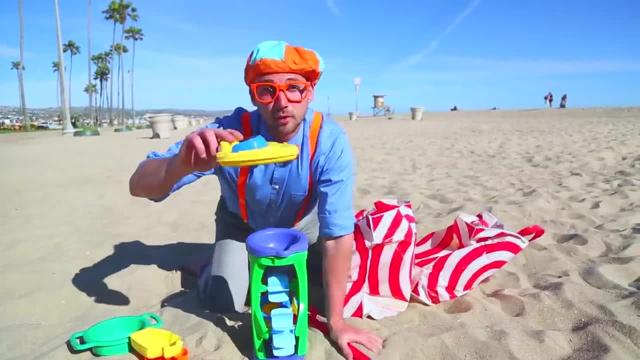 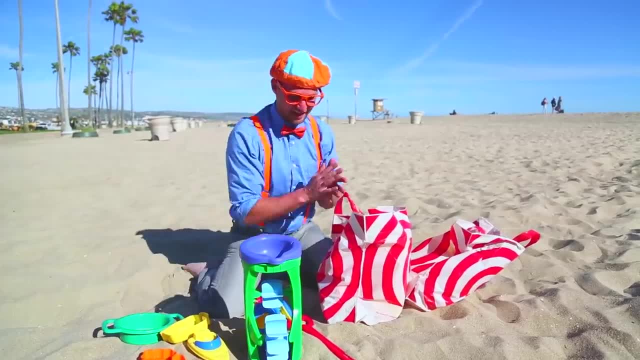 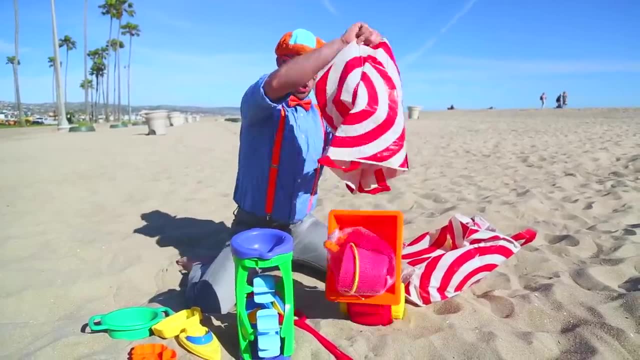 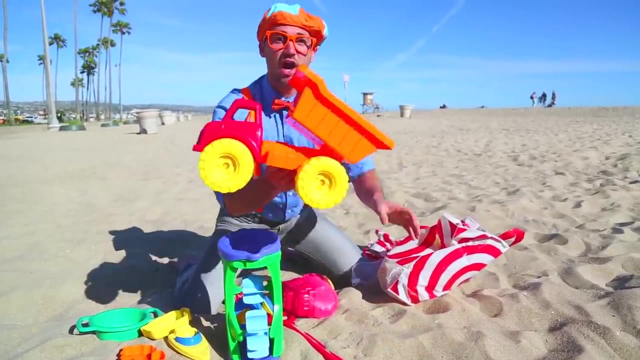 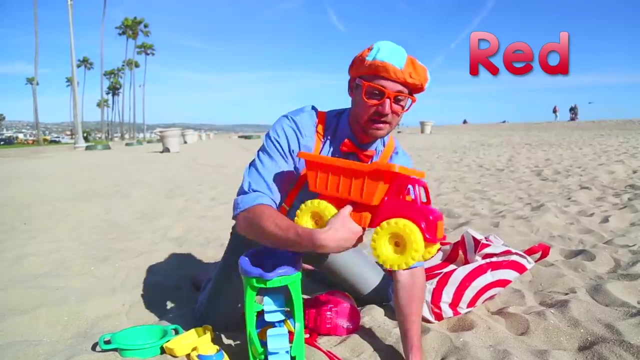 And some other cool looking toys. Okay, All right, Let's see what bag number two has, Whoa. Bag number two has A giant dump truck, Whoa. This dump truck is the color red, yellow and orange. Okay, 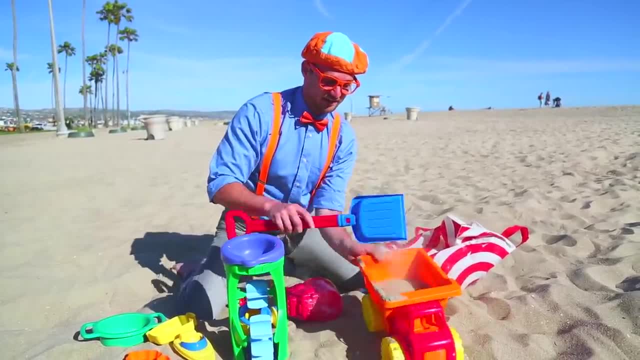 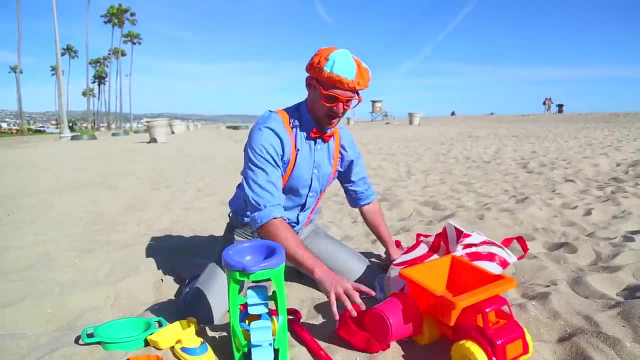 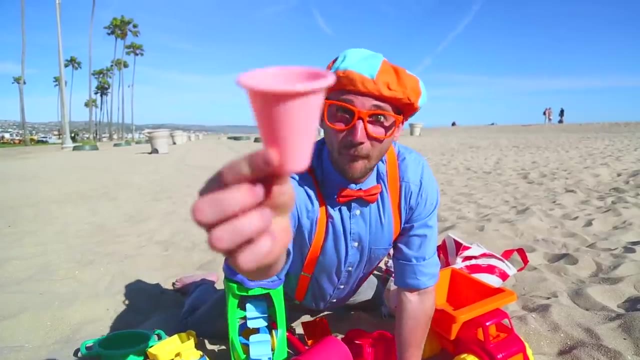 We're gonna put a bunch of sand in this later, Just like that, But a lot more of it. Okay, And a lot of other toys: A red one and a pink one And a big one. Look, Whoo, That's funny. 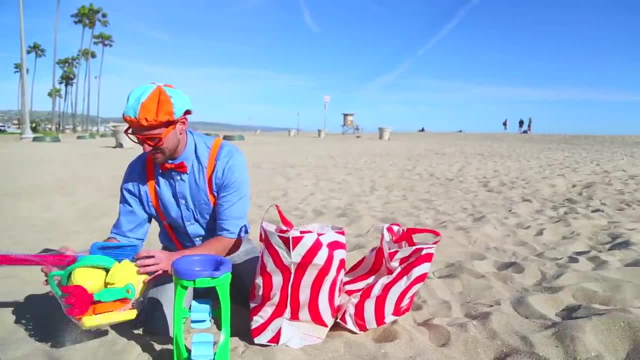 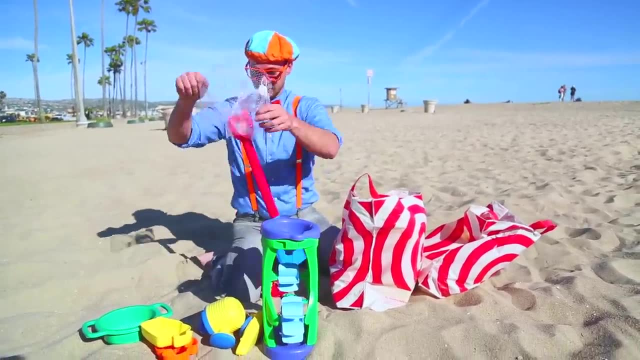 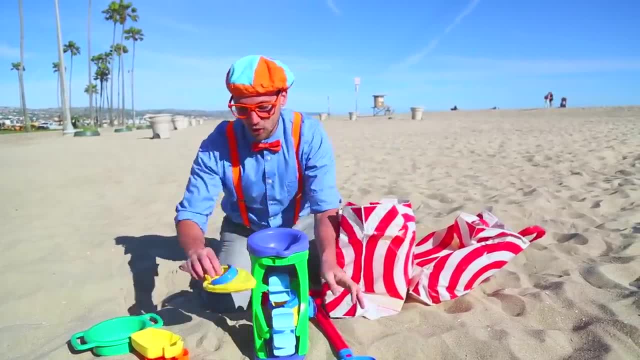 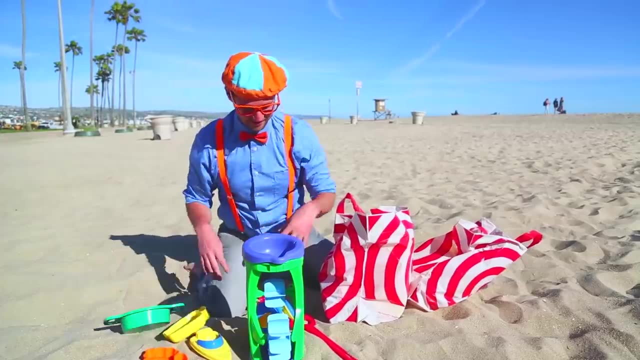 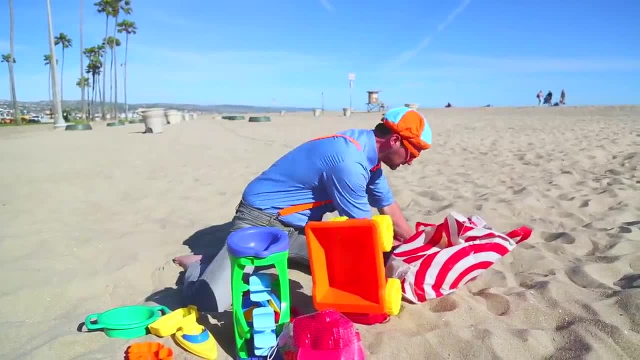 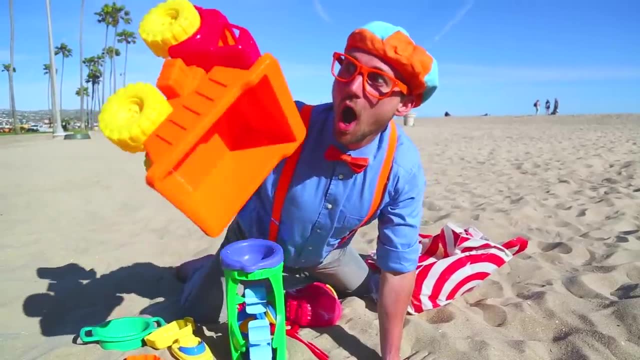 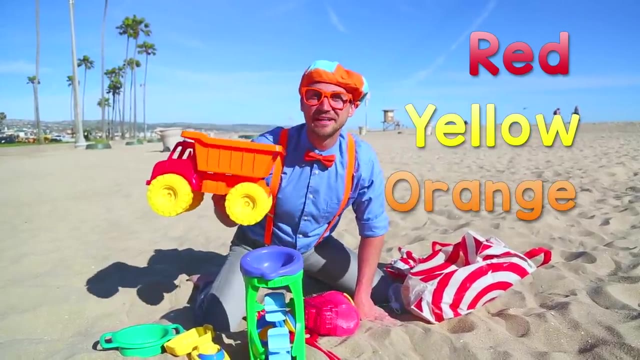 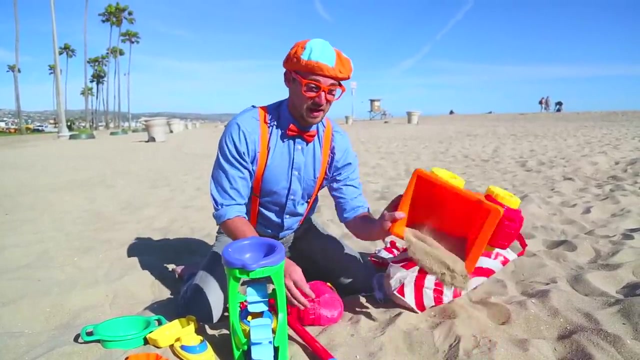 Blippi, Blippi, Whoa. bag number two has a giant dump truck, Whoa. this dump truck is the color red, yellow and orange. Okay, we're gonna put a bunch of sand in this later, just like that, but a lot. 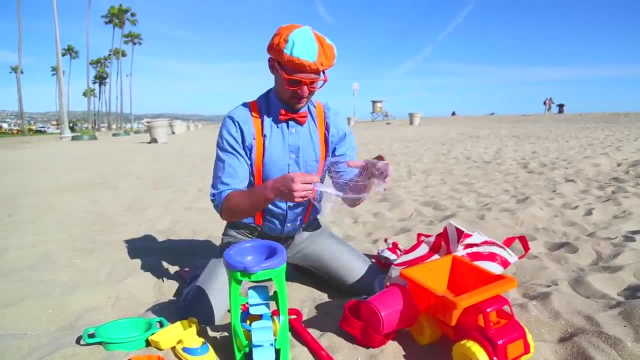 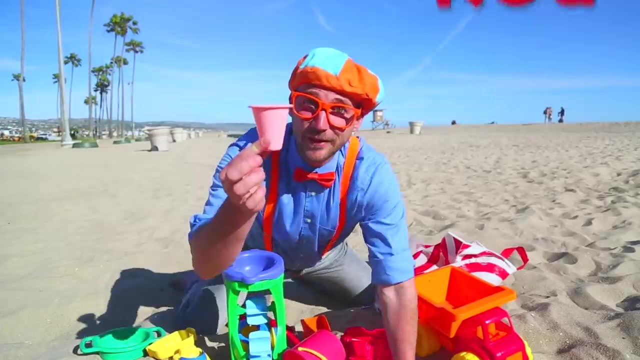 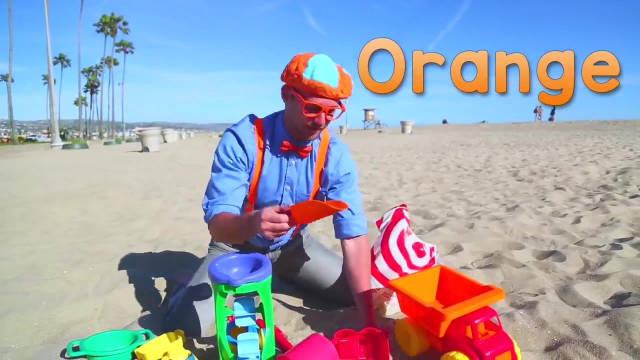 more of it. Okay, and a lot of other toys: A red one and a pink one, Itty bitty one- look That's funny. And a scooper. Look at this orange scooper. Okay, and the last bag has. 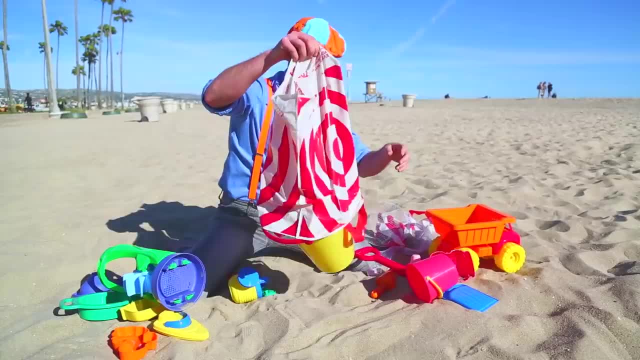 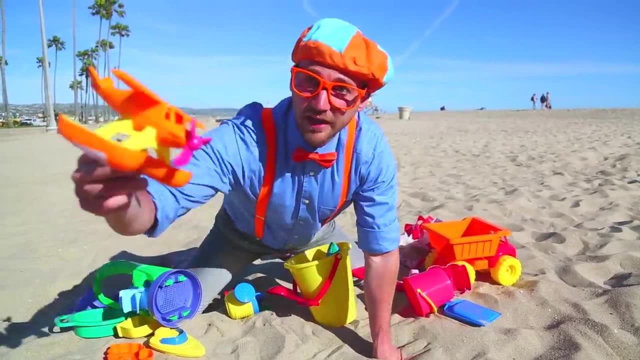 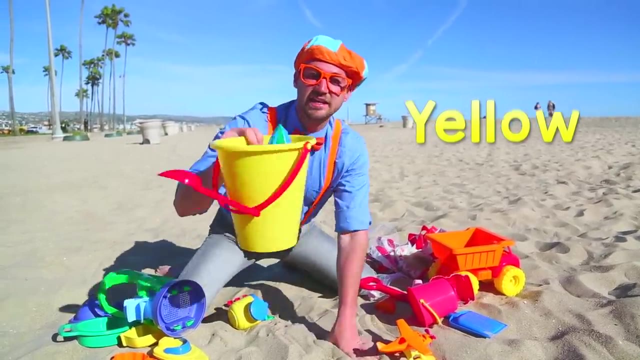 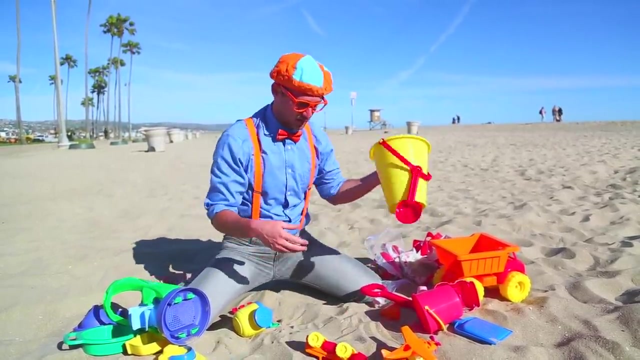 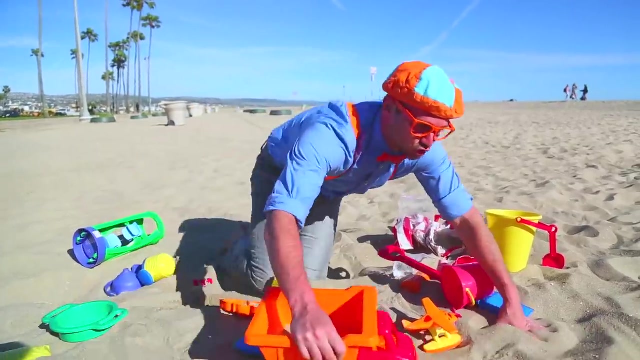 I'm so excited to see what's in this bag. This bag has whoa, an airplane And a yellow bucket with a red scooper and some other toys. Okay, okay, I think we should take the dump truck. Come over here. 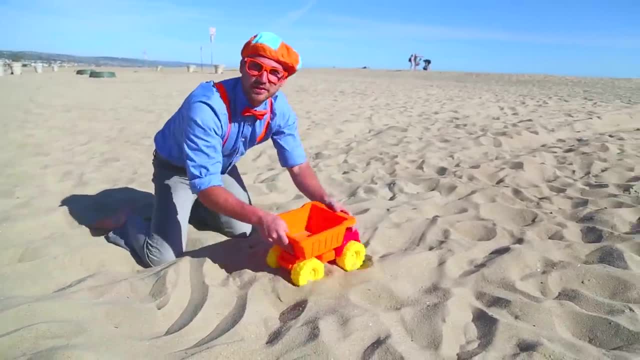 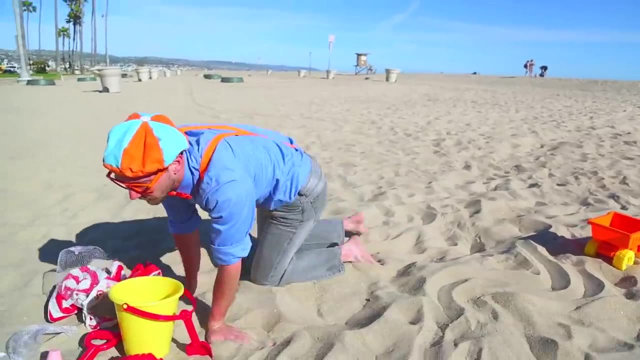 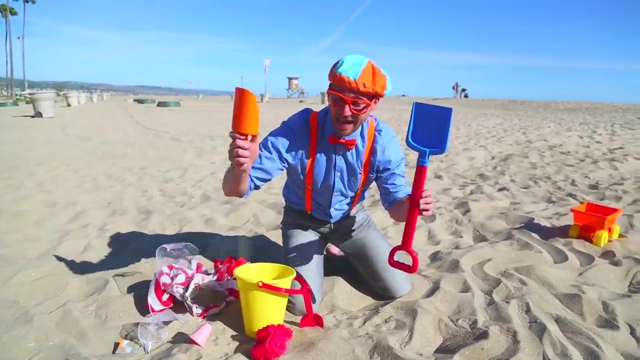 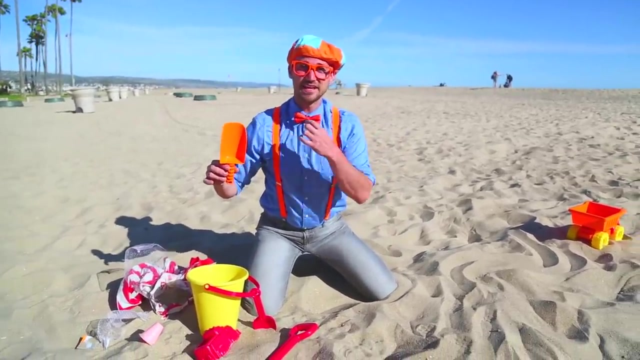 Okay, let's put the dump truck right here. Okay, and I need a scooper, Come on. Okay, should we use this big shovel or this orange hand shovel? Um, let's use this orange one, because it's the color of my suspenders. 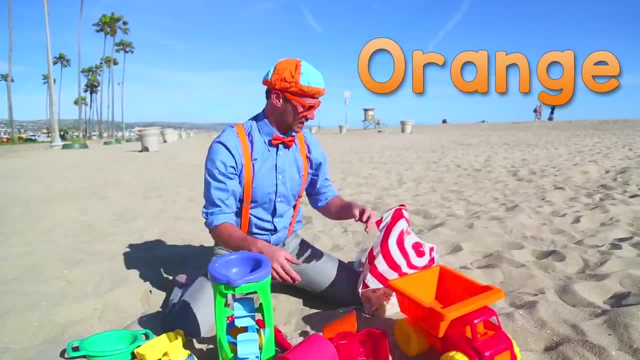 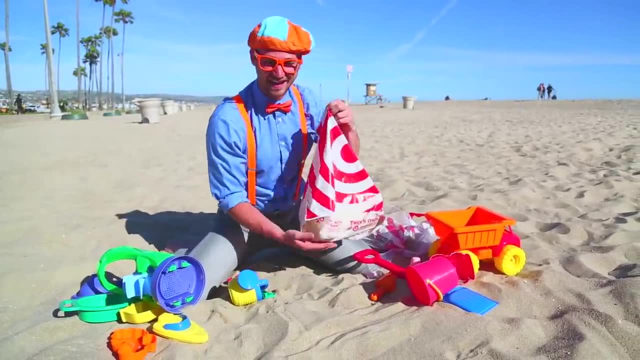 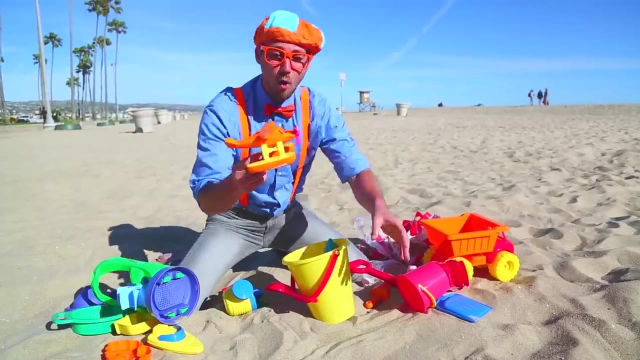 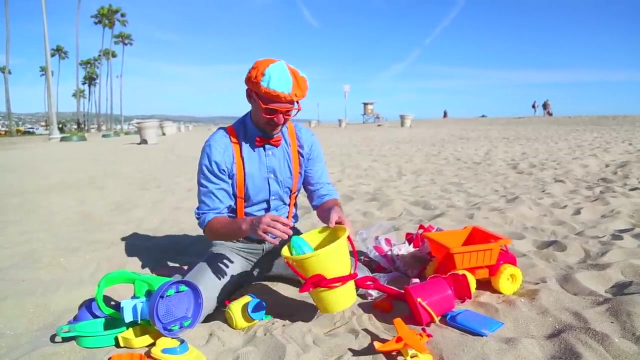 And a scooper. Look at this orange scooper. Okay, And the last bag has. I'm so excited to see what's in this bag. This bag has Whoa, An airplane Whoa And A yellow bucket. 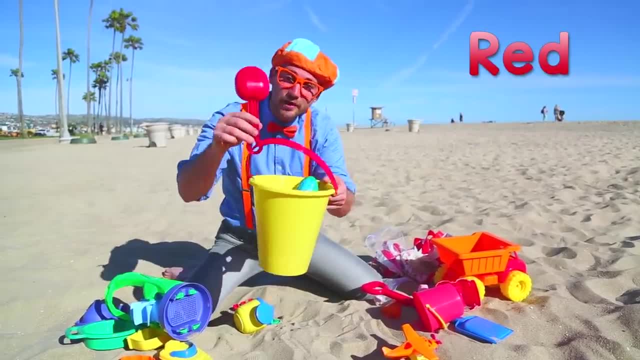 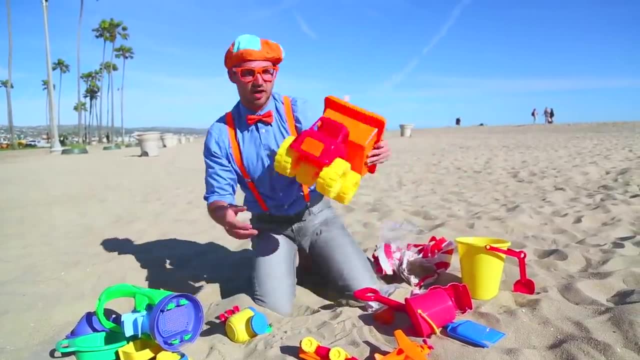 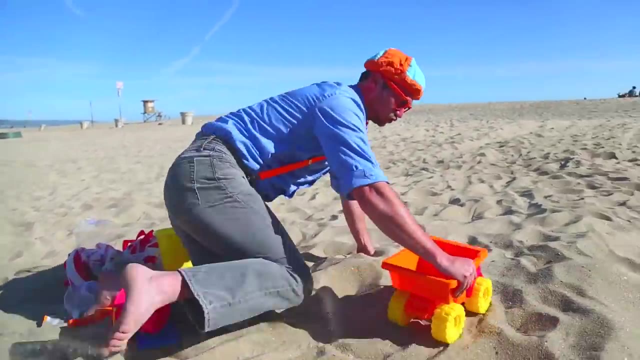 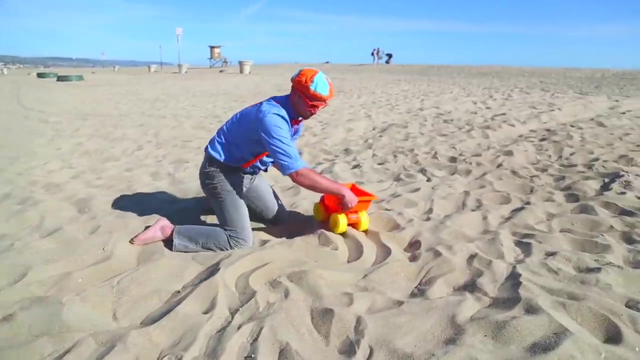 Whoa And a red scooper, Eek eek, eek, eek eek And some other toys. Okay. Okay, I think we should take the dump truck. Come over here, Come on. Okay, let's put the dump truck right here. 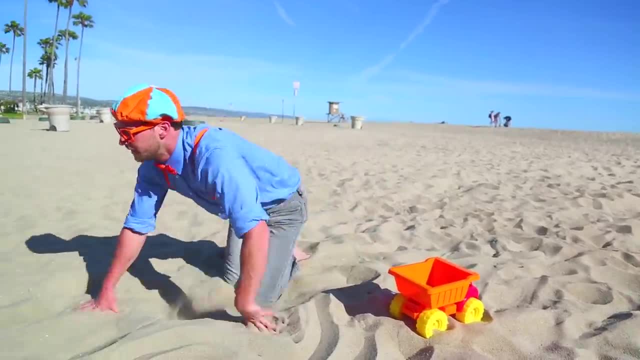 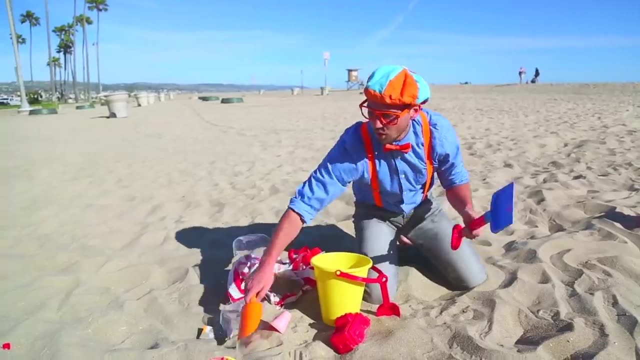 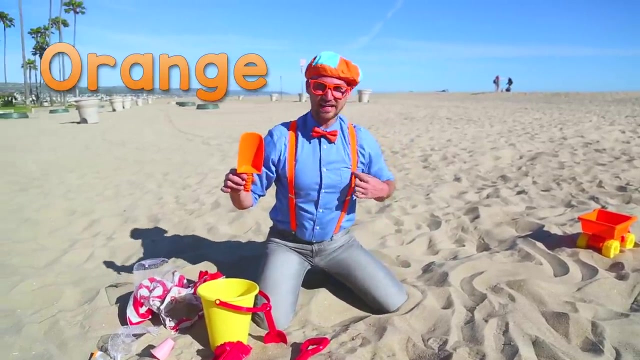 Okay, Okay, and I need a scooper, Come on, Okay, Should we use this big shovel Or this orange hand shovel? Um, let's use this orange one, Because it's the color of my suspenders and bow tie. 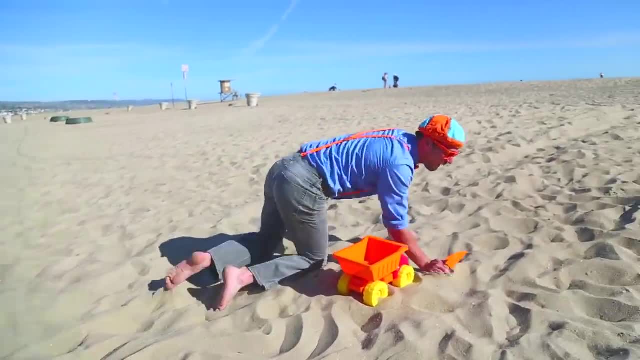 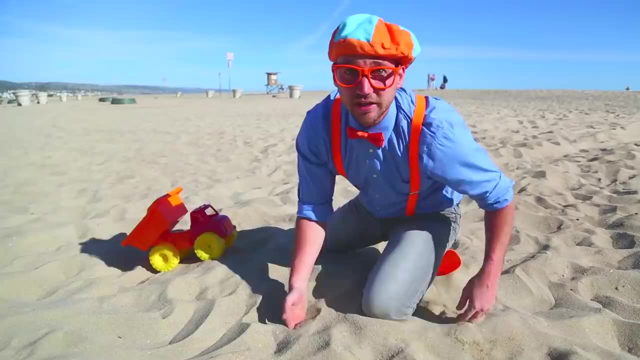 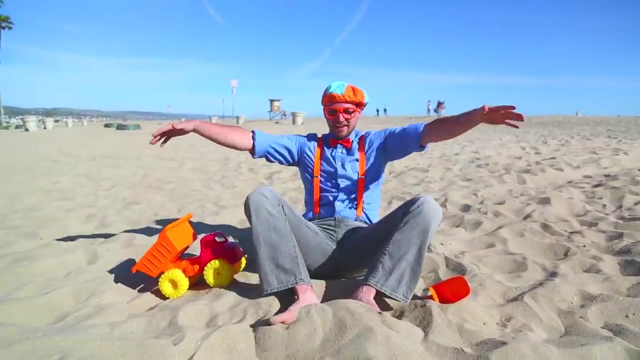 Come on. Oh, this sand feels so good in my hands, Get a close-up. Oh, this sand feels so good in my hands, Get a close-up, Get a close-up. Look at this. Whoa, Whoa, My hands and my feet. 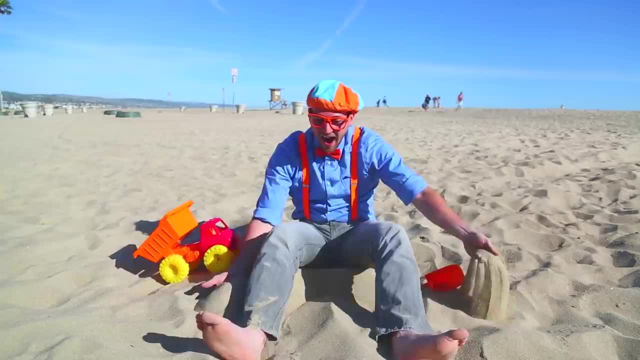 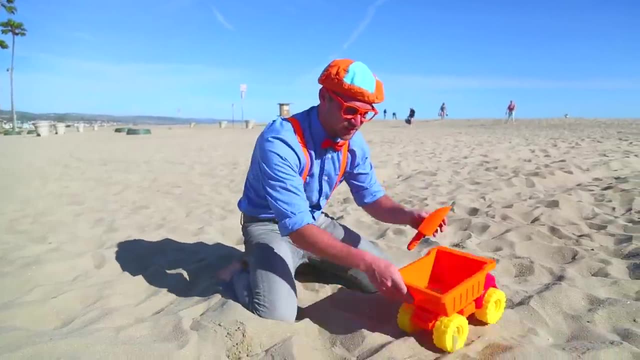 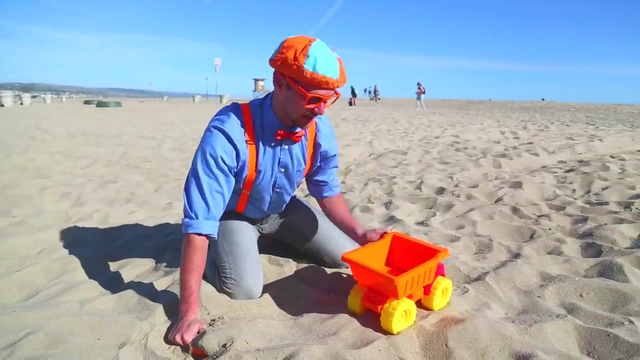 Oh, it feels so good, Wow, Okay, now let's get a big scoop in the back of the dump truck. See, Vroom, vroom, vroom, vroom, vroom. Okay, let's count them together. 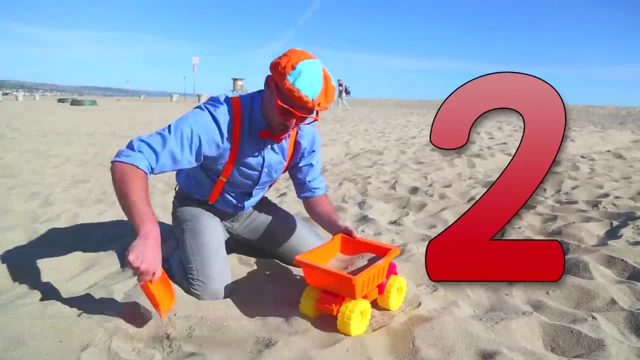 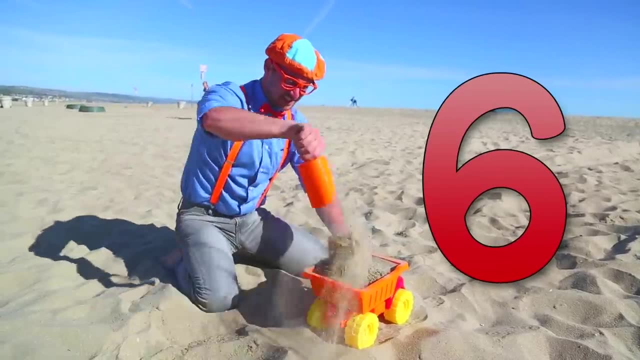 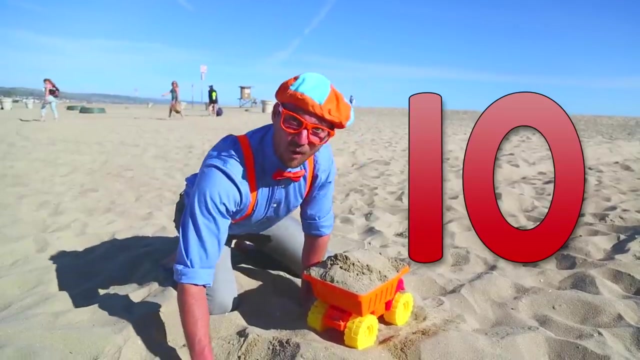 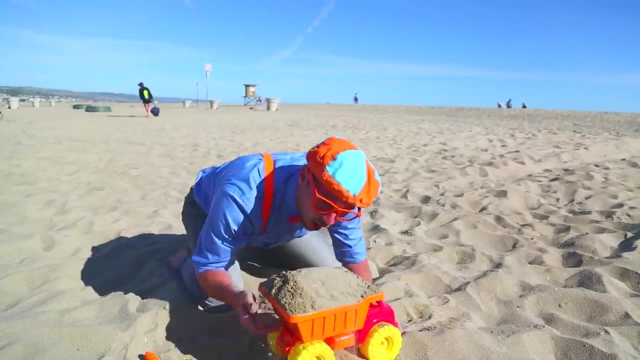 Get it all empty. One, Two, Three, Four, Five, Six, Seven, Eight, Nine, Ten, One more, Eleven, Oh yeah, Look at, oh, it's so heavy. Wow, look at this giant. oh, 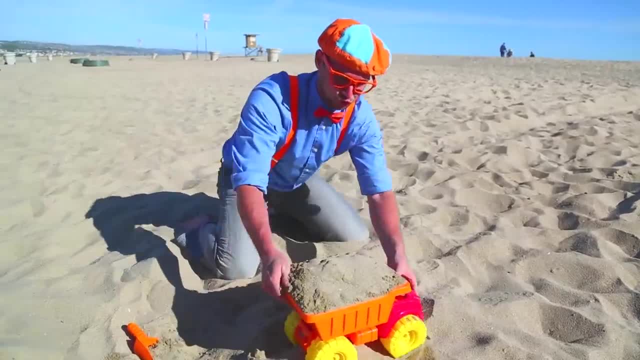 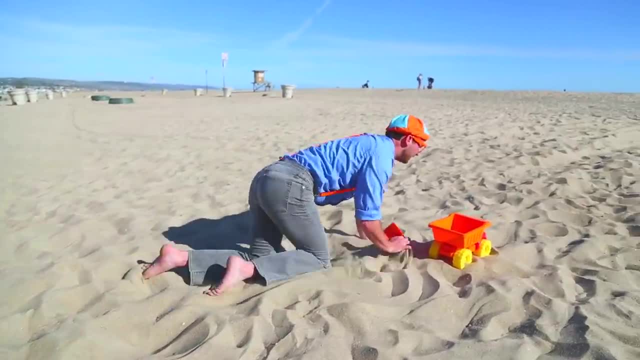 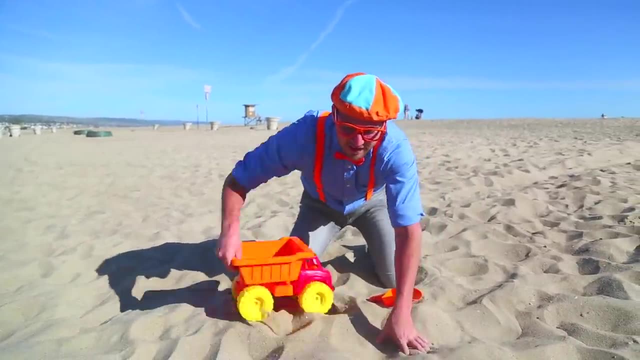 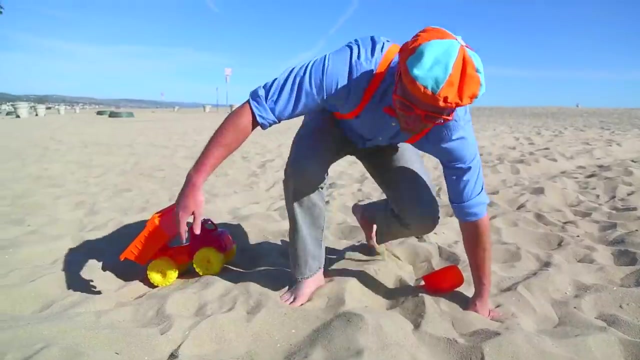 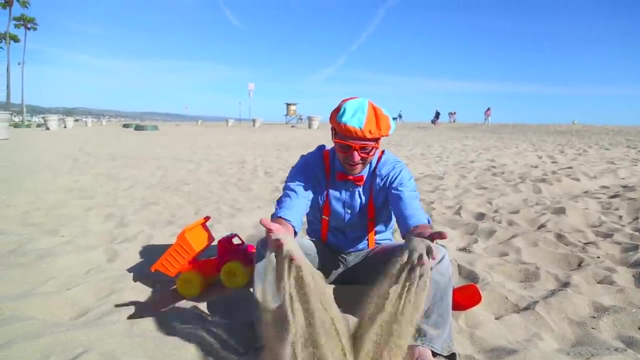 and bow tie. Come on, Oh, this sand feels so good in my hands. Get a close-up. look at this. Whoa, Whoa, My hands and my feet Feels so good, Wow, Okay, now let's get a big scoop in the back of. 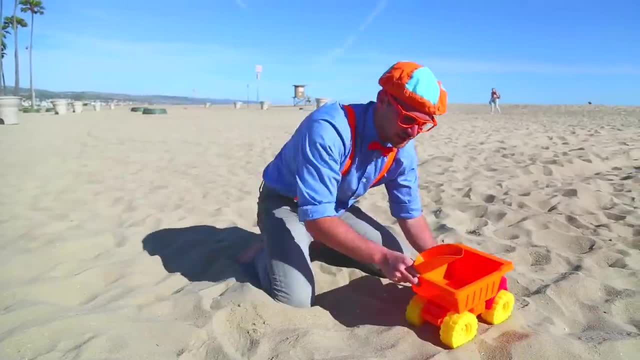 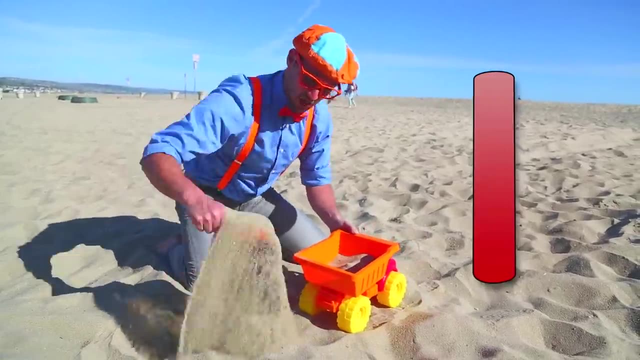 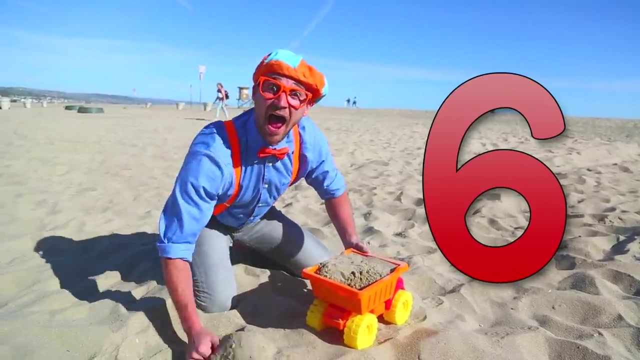 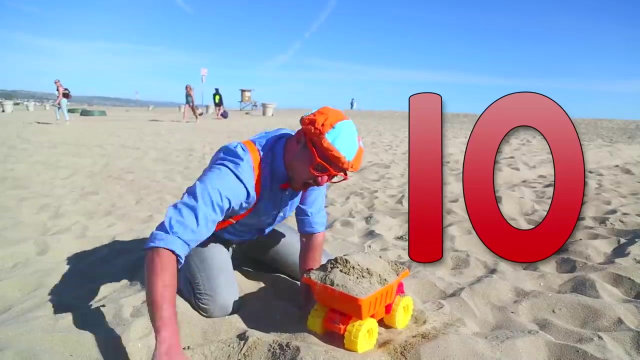 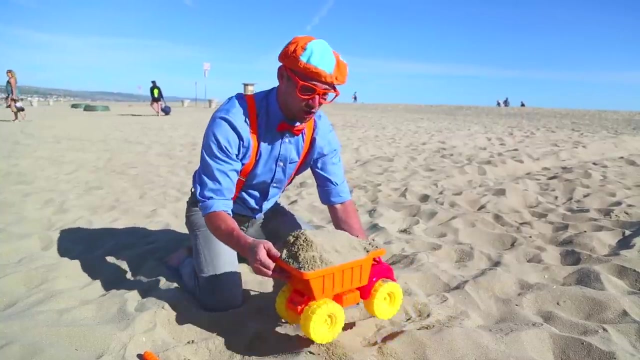 the dump truck. See, Let's count them together. Get it all empty: One, two, three, four, five, six, seven, eight, nine, ten, One more Eleven. Oh yeah, Look It's so heavy. 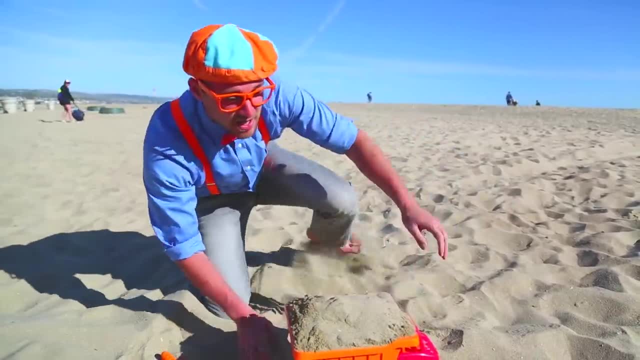 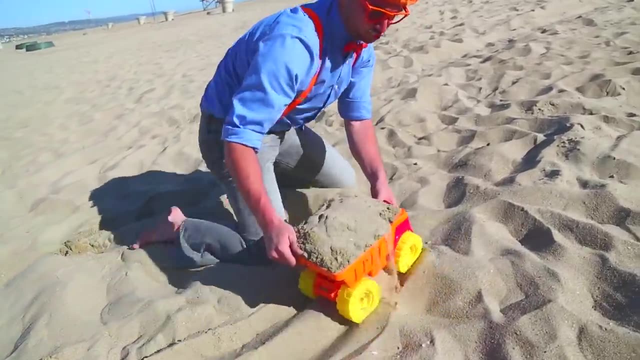 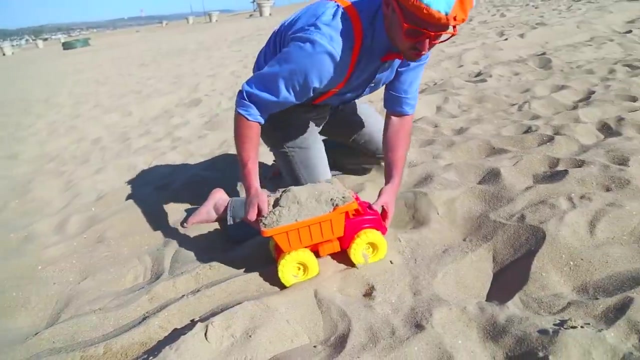 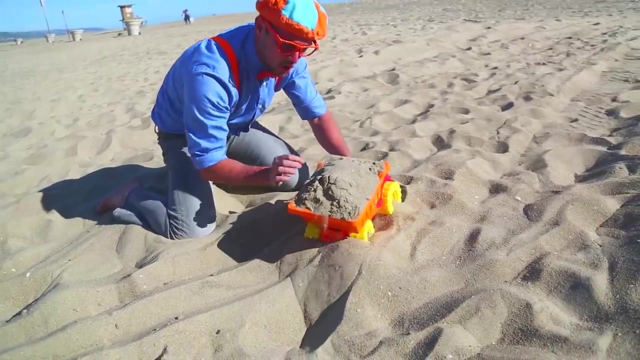 Wow, Look at this giant. Okay, let's dump it out together. Ready, Come this way. Oh, how about? right here? Okay, right here, Ready. Beep, beep, beep, beep, beep, beep, beep. 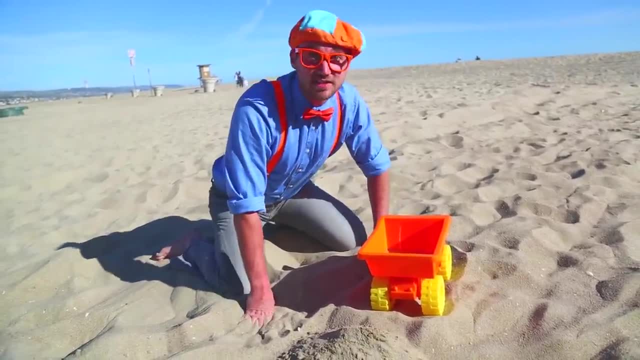 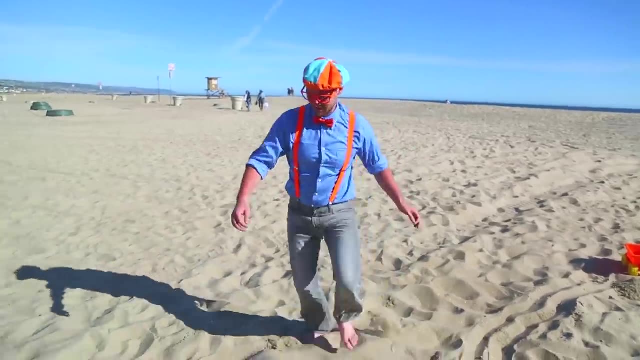 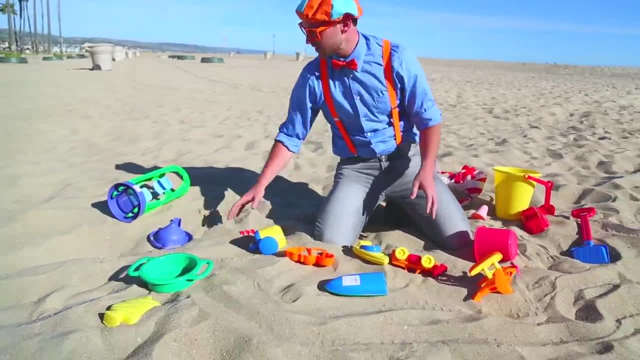 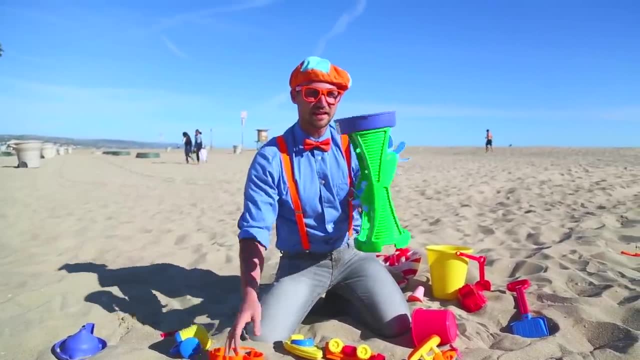 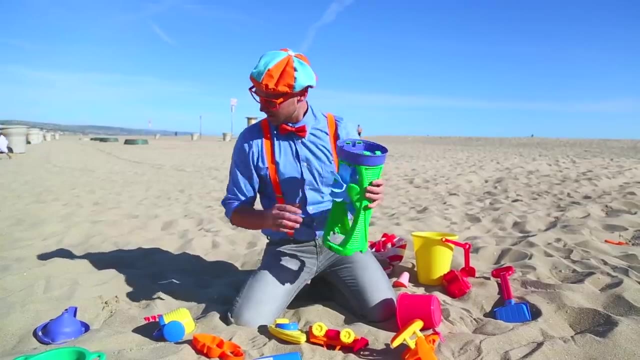 Okay, Look at all the toys. Let's see what other toys- Whoa, Look at this toy. Whoa, Like I said earlier, this toy is the color blue and green. Okay, Let's see. Oh look, I think this goes on top. 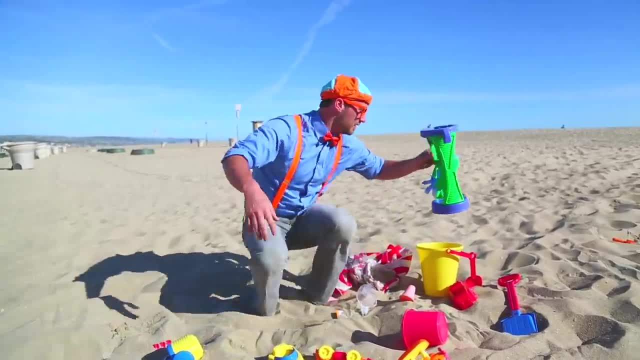 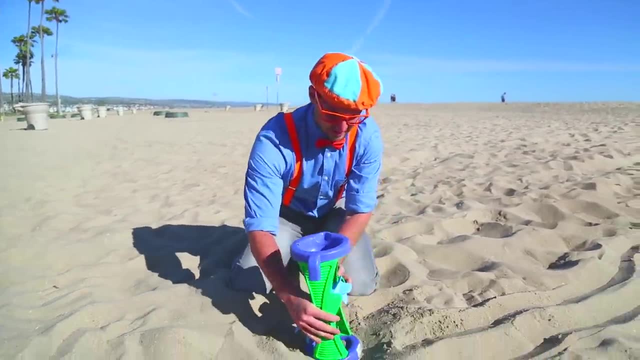 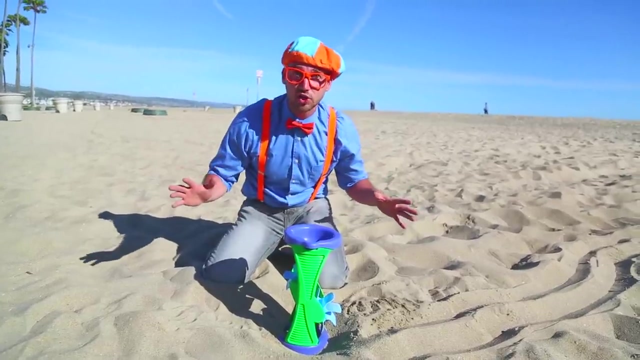 And then we put sand on top. Come on, Let's put it right, right where this scooper was. Okay, You might have to get a close-up shot of this later, but let me grab that really big shovel from earlier. right, The shovel. 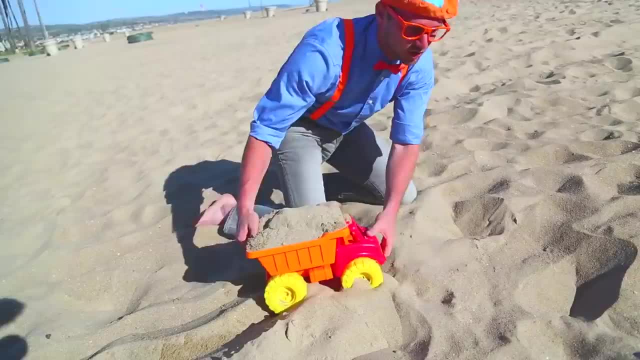 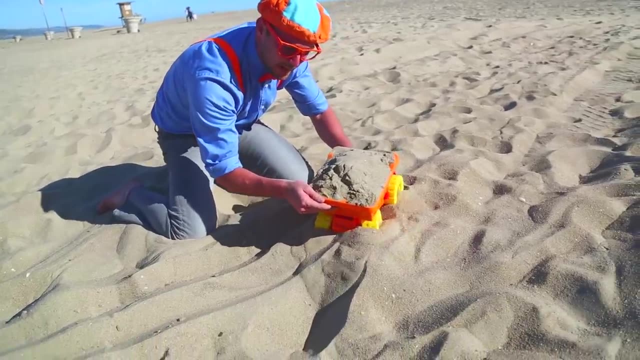 Vroom, vroom, vroom. Oh, how about right here Vroom, vroom, vroom, vroom. Okay, right here Ready Beep, beep, beep, beep, beep, beep, beep Poof. 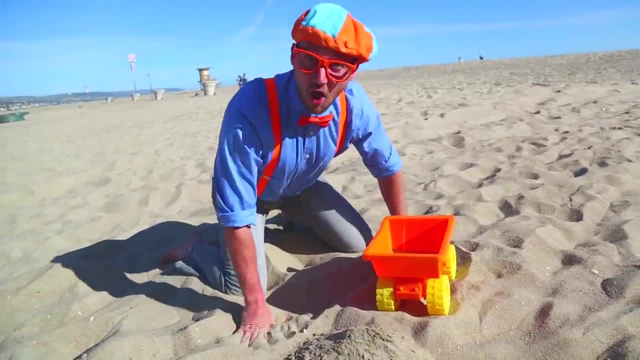 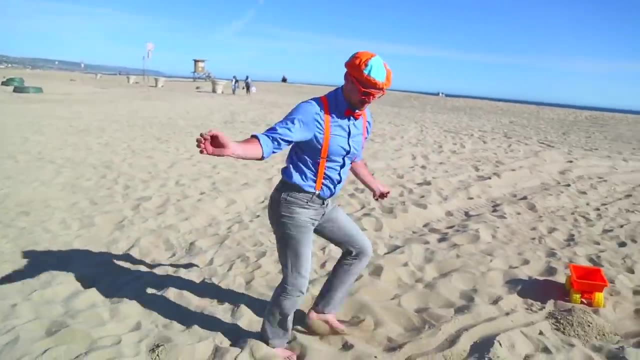 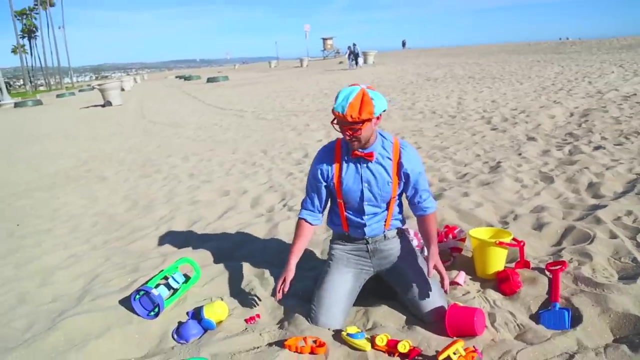 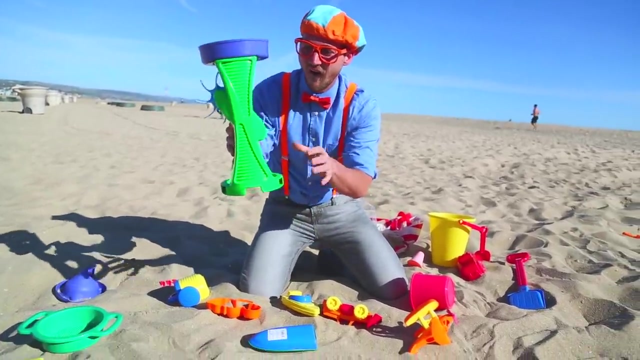 Poof. Yeah, that was awesome. Let's go get some more toys. Come this way: Beep, boop, boop. Okay, look at all the toys. Let's see what other toys Whoa, Look at this toy. 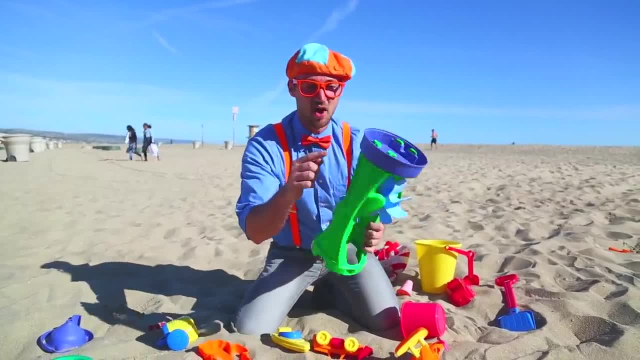 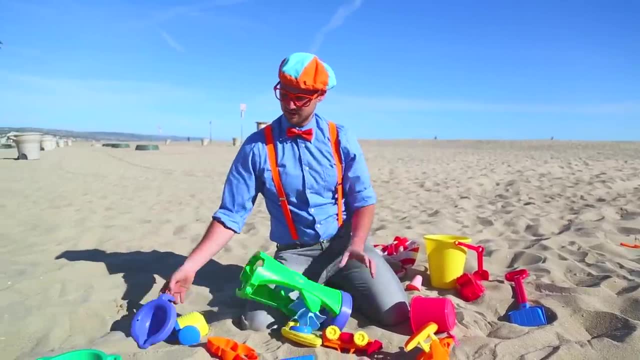 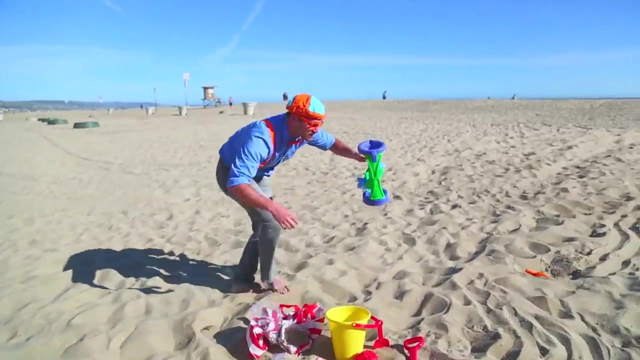 Whoa. Like I said earlier, this toy is the color blue and green. Okay, let's see. Oh look, I think this goes on top, And then we put sand on top. Come on, Let's put it right where this scooper was. 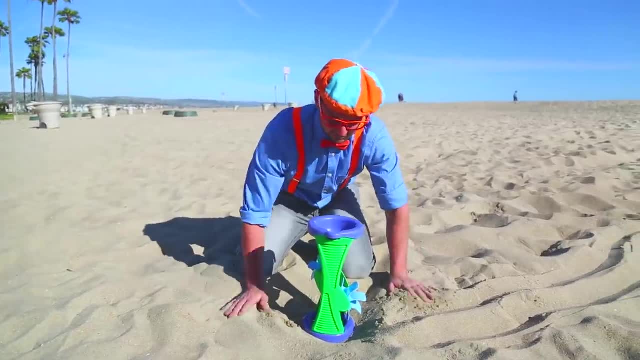 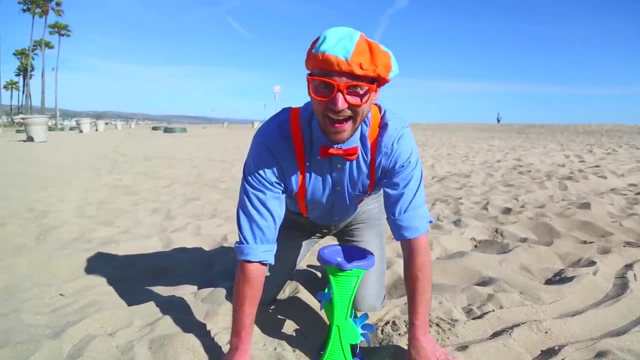 Okay, You might have to get a close-up shot of this later, but let me grab that really big shovel from earlier. right The shovel. Yeah, Okay, Come over here. Woo-hoo, Woo-hoo-hoo, Okay. 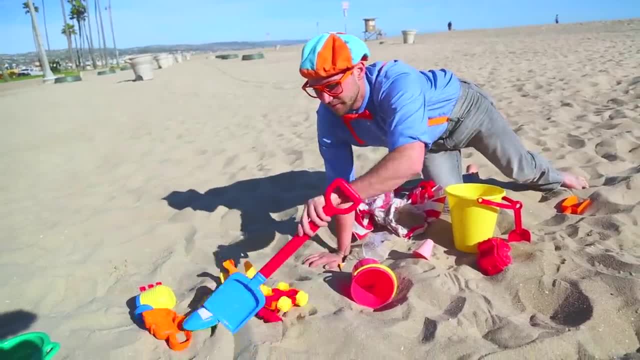 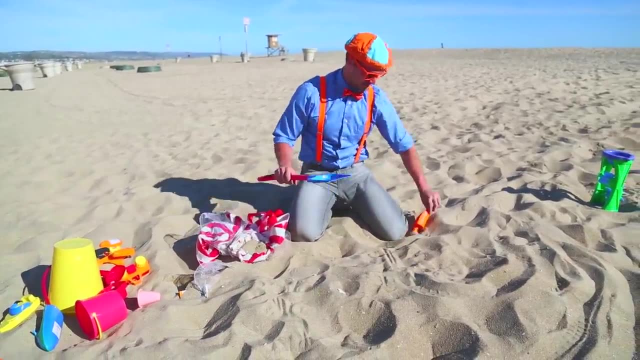 You go over here. Okay, Move around here. Move around here. toys, The shovel's making way. These are the bags from earlier. Okay, Consolidation. Okay, Great. Now I have the shovel. Okay, Let's shovel some sand. 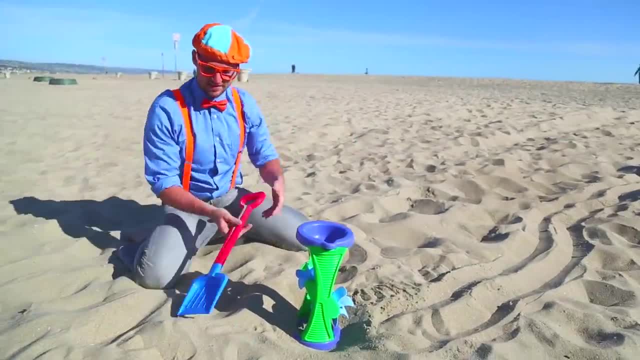 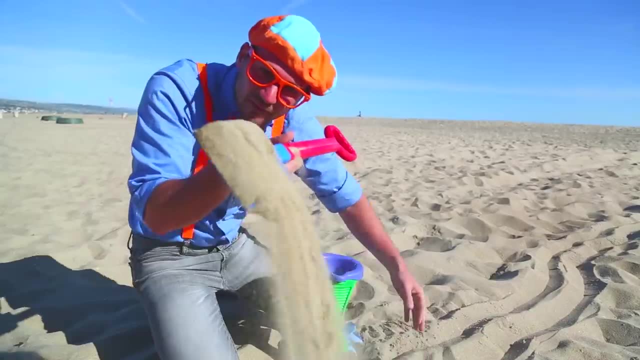 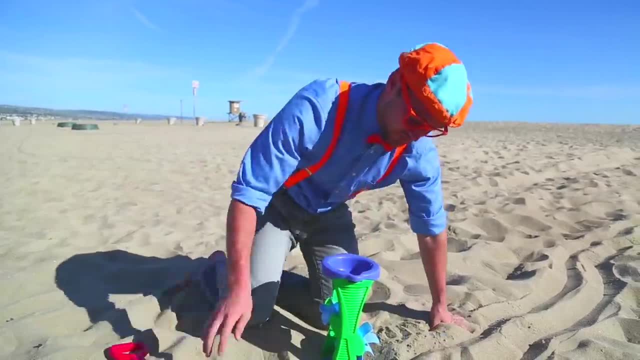 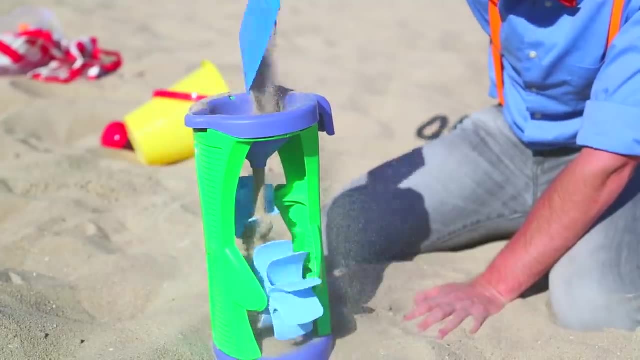 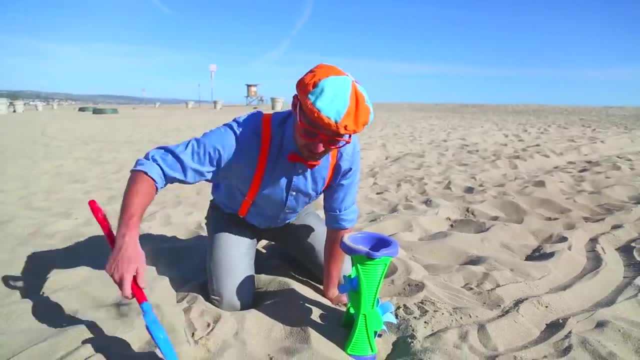 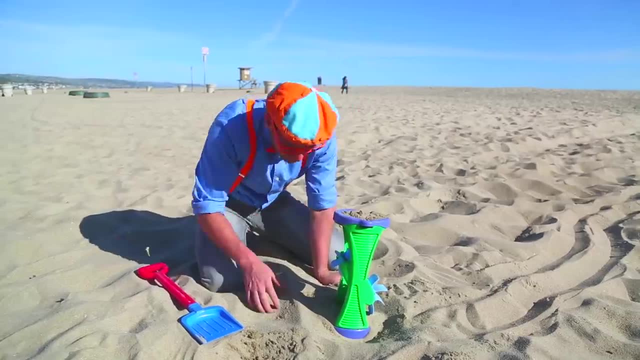 Look at this, Look at this. Now, this is a shovel- Whoa. Okay, Let's put some in here, And then you can get a closeup shot. Ready, Whoa, Wow, Did you see that One more time? 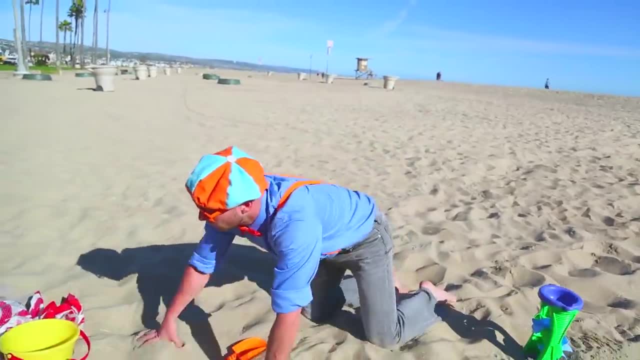 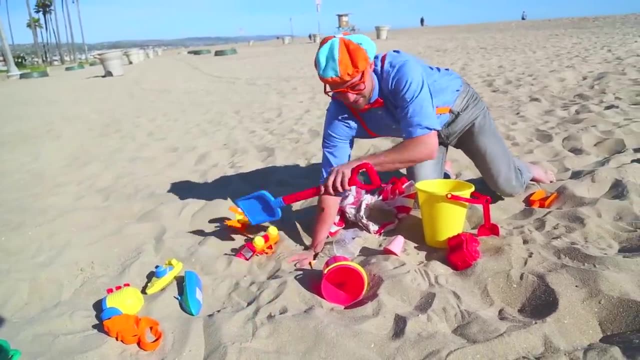 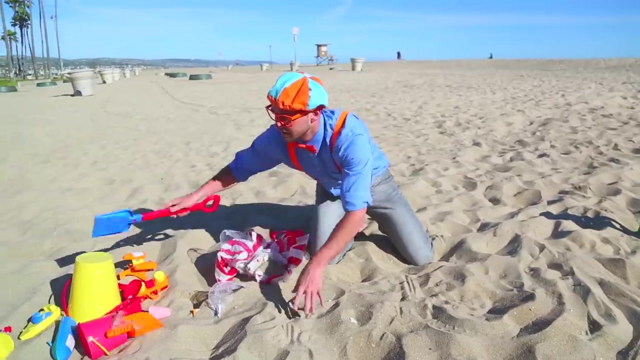 Yeah, Okay, Come over here. Woo-hoo, Woo-hoo-hoo, Okay, You go over here. Move around here. toys, The shovels make it way. These are the bags from earlier. Okay, Consolidation. 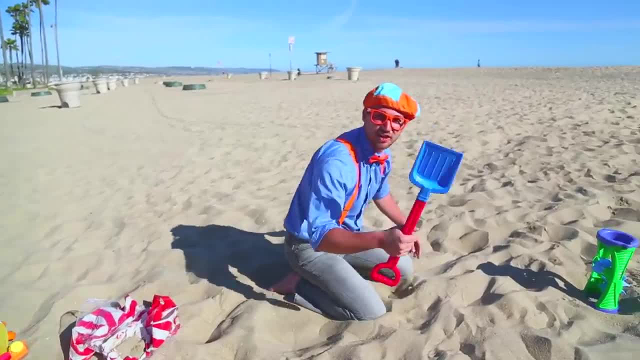 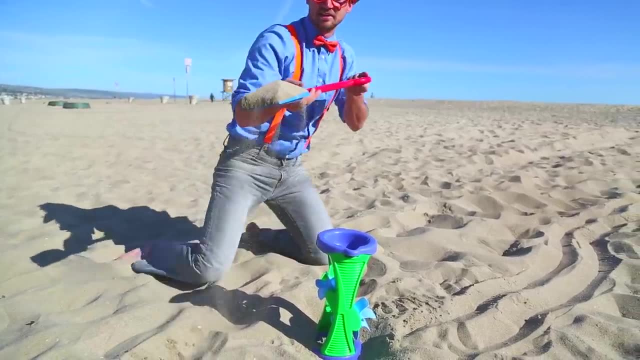 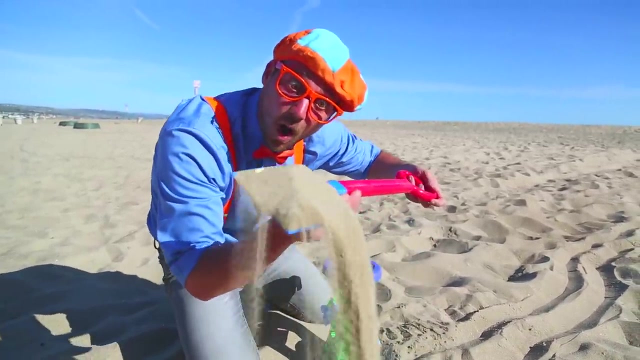 Okay, Great, Now I have the shovel. Okay, Let's shovel some sand. Look at this, Wow, Wow. You want to see that again, Whoa. Okay, Let's put some in here, And then you can get a close-up shot. 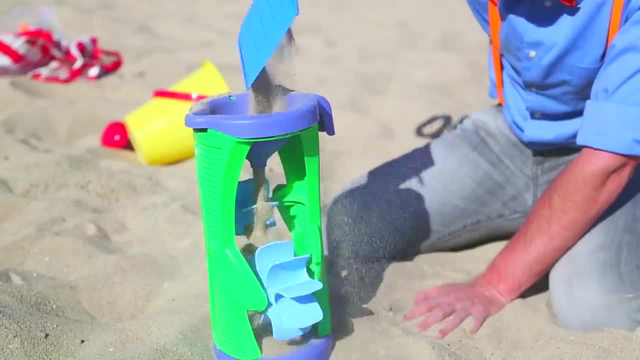 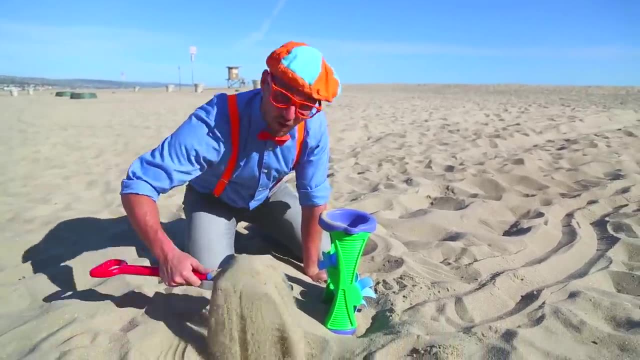 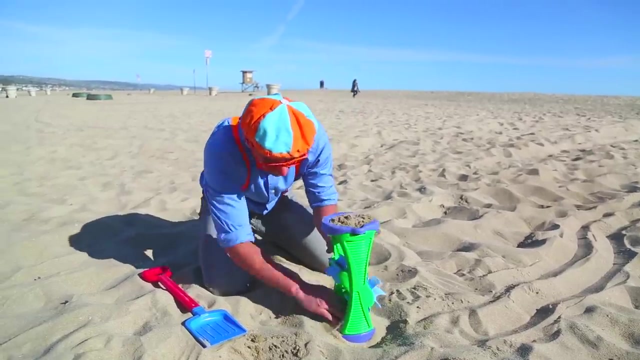 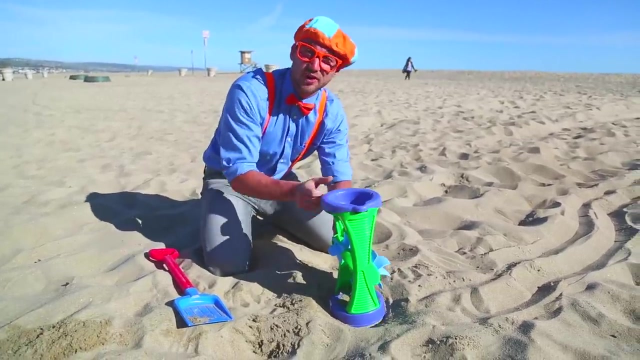 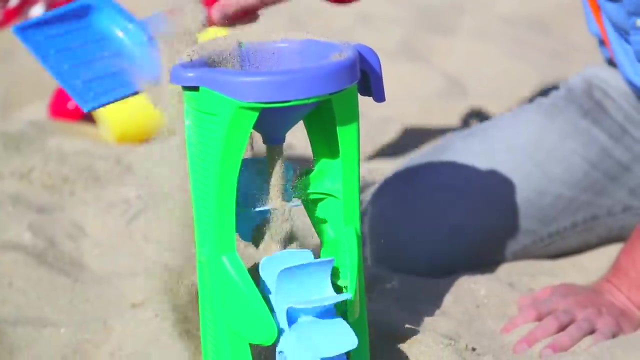 Ready? Whoa, Wow, Did you see that One more time? Shake, shake, shake. Come on, You can go. We might need drier sand. Okay, Here we go. Whoa, Did you see how fast that spun? 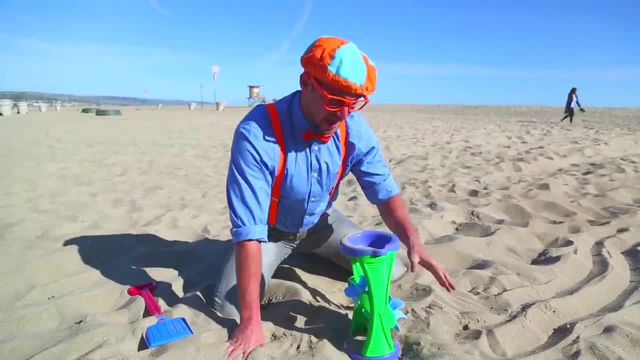 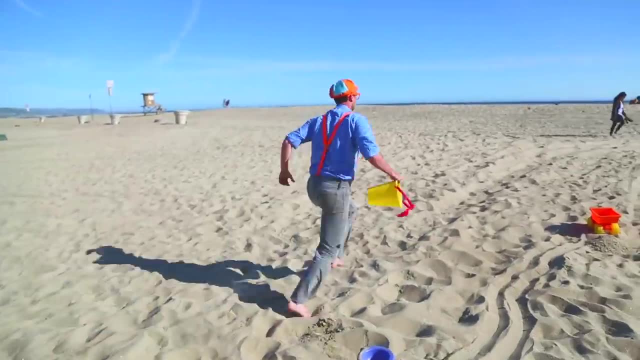 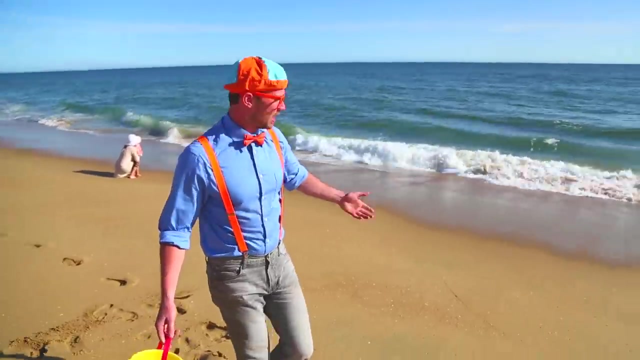 Now let me go grab a bucket and go fill it up with water, and we'll try this again with water Watch. Oh look, We made it to the water, But I don't have my bathing suit on, So I'm going to roll up my pants. 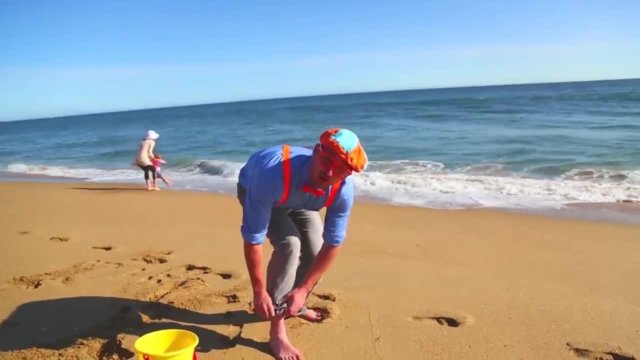 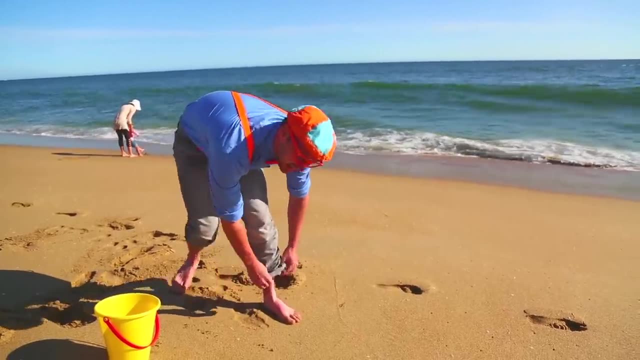 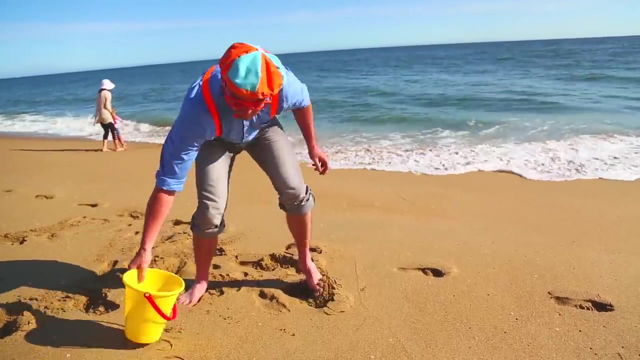 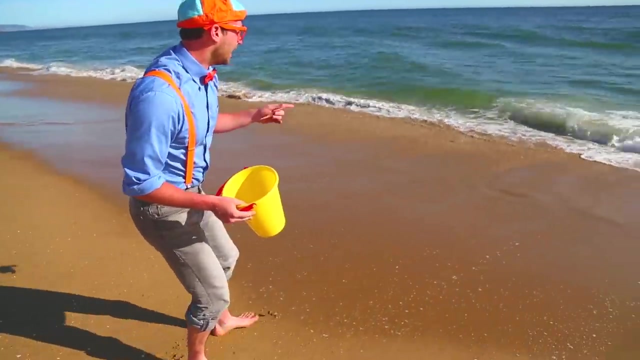 so they don't get wet. Just do a couple rolls up, just like this, Okay, And this one as well. Okay, I'm ready to get us some water. Come on, Whoa, Get ready for a wave and I'll scoop up some water. 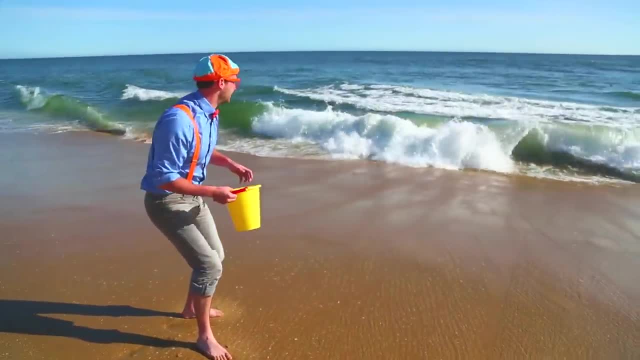 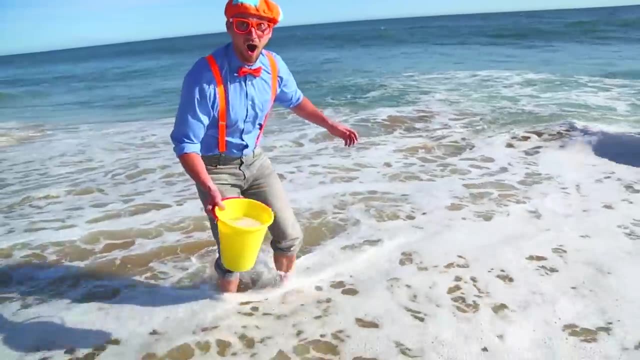 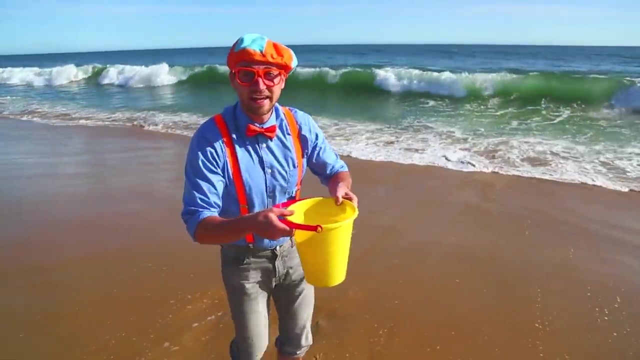 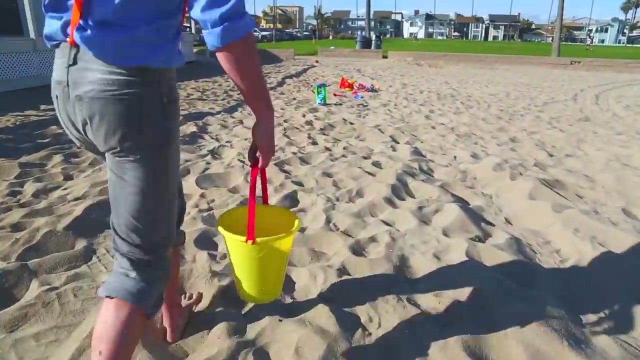 Whoa, Here comes a big one. I got some water. Look, Whoa See, I can't waste it. We got to go put it in the toy. Come on, Okay, Now that we have a full bucket of water. 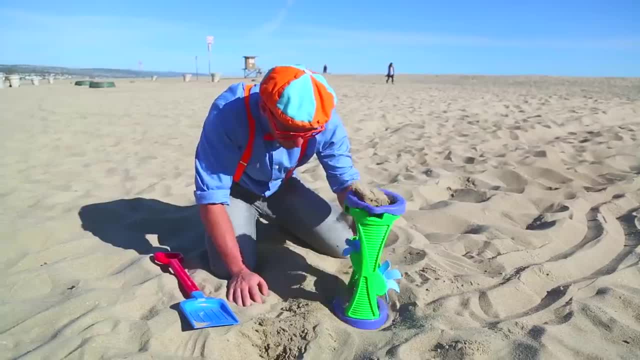 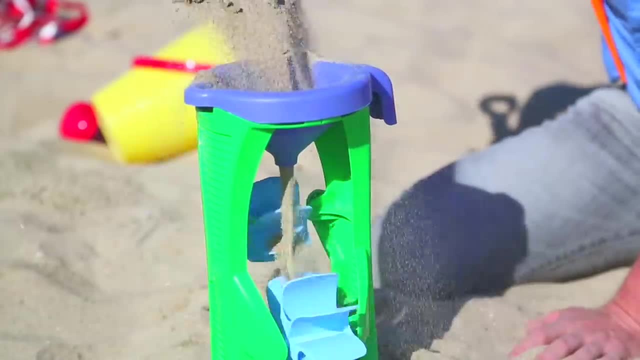 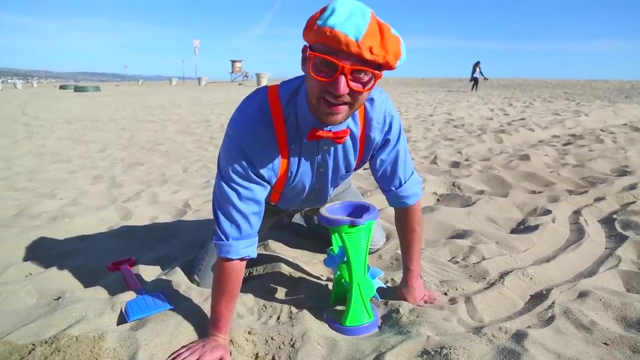 Oh, Shake, shake, shake. Come on, You can go. We made it to the top. Oh, we might need drier sand. Okay, here we go. Whoa, Did you see how fast that spun? Now, let me go grab a bucket and go fill it up with water. 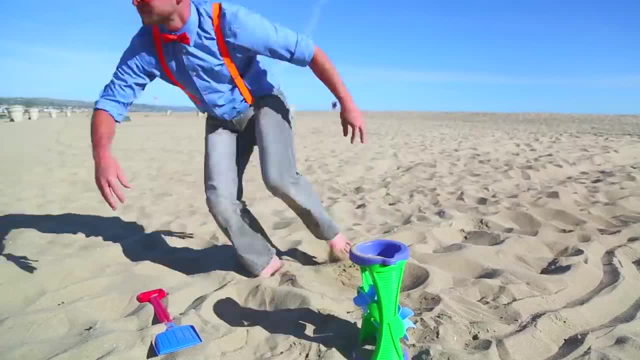 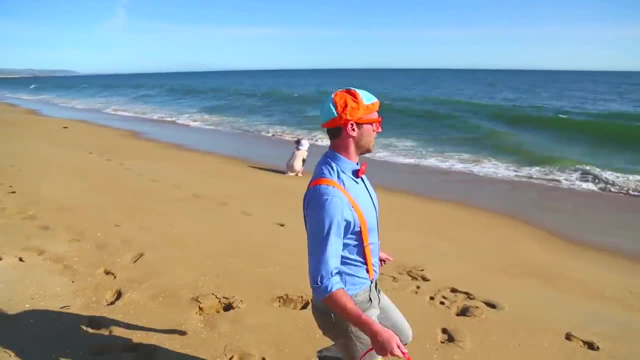 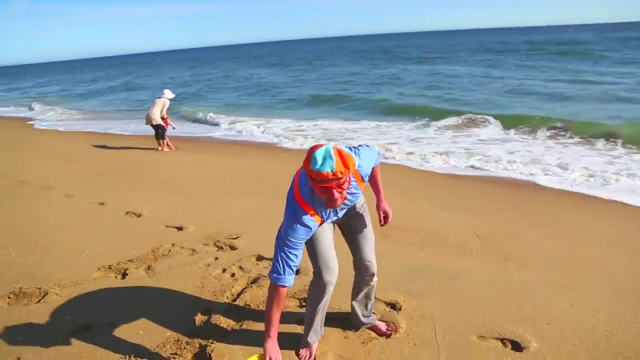 and we'll try this again with water Watch. Oh look, we made it to the water, but I don't have my bathing suit on, so I'm gonna roll up my pants so they don't get wet. Just do a couple rolls up, just like this, okay. 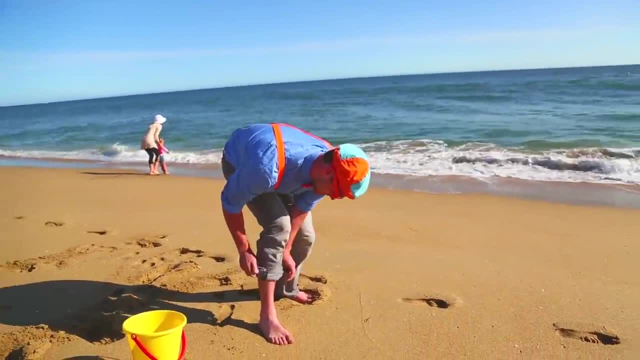 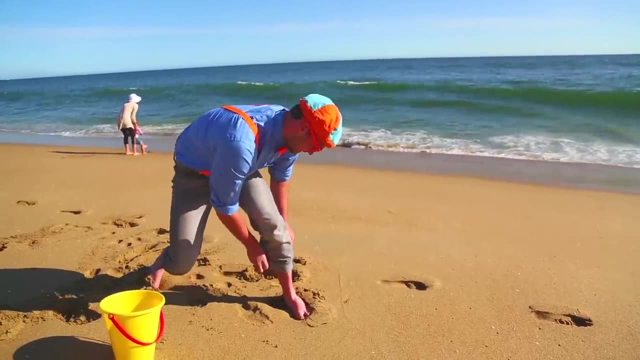 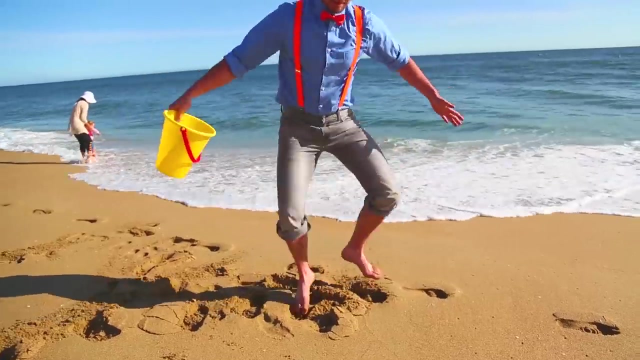 And this one as well. Oh look, we made it to the water. Oh, look, we made it to the water. Oh look, we made it to the water. Okay, I'm ready to get us some water, Come on. 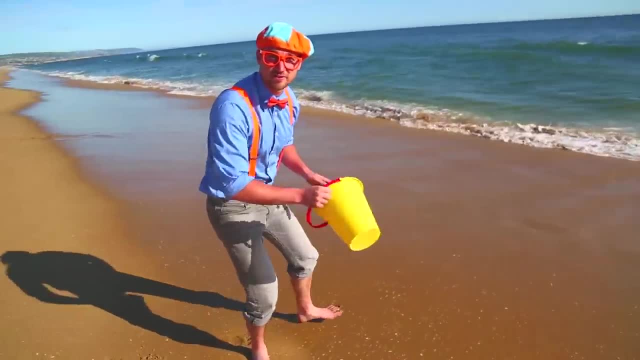 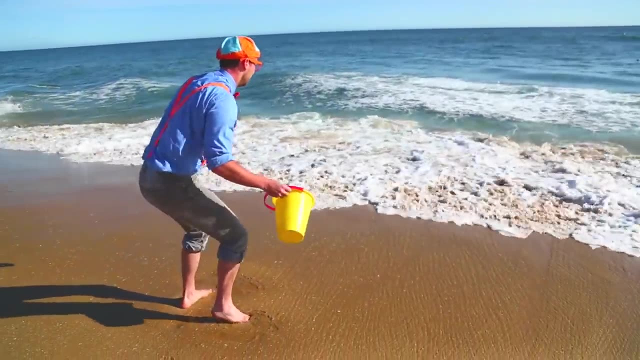 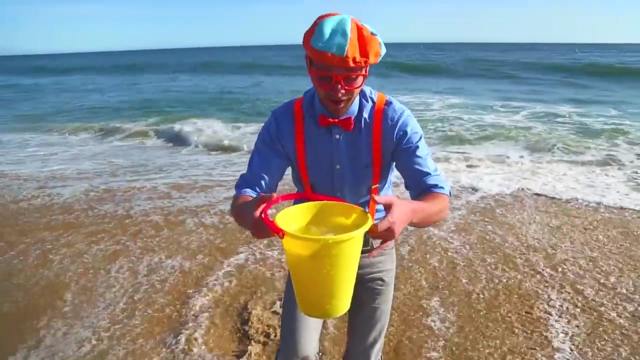 Whoa, Get ready for a wave and I'll scoop up some water. Whoa, here comes a big one. I got some water. look, Whoa See whee. Oh, I can't waste it. We gotta go quick. 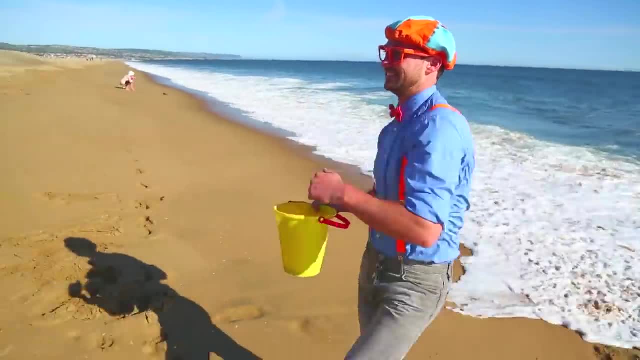 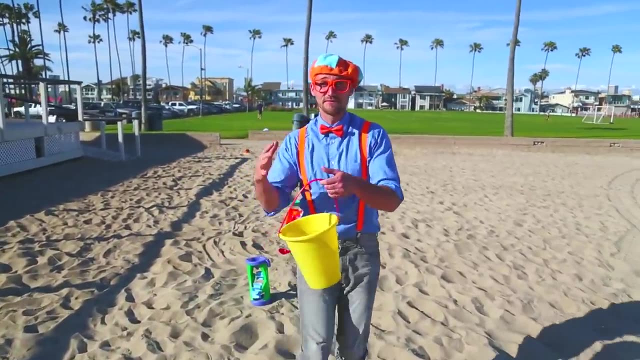 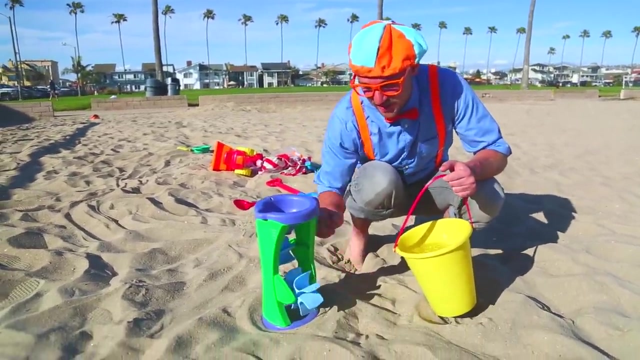 I'm gonna put it in the toilet, Come on. Okay, now that we have a full bucket of water, I kinda wanna see what it's like pouring water in here. okay, You know how these spin when we put sand in it. 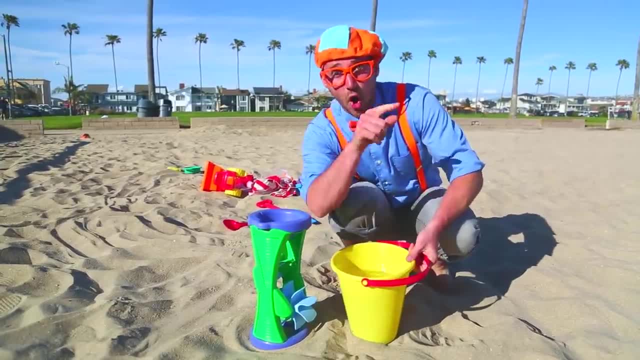 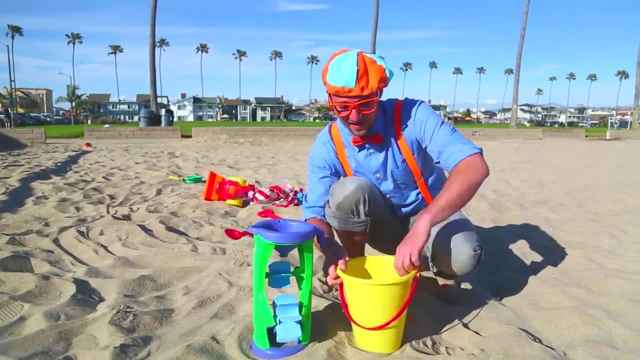 Yeah, Let's see if we pour water that we got from the ocean in here. if they spin, How does that look? Can you see them? Yeah, Okay, Here we go. Whoa, It's working. Oh, okay, Let's fix this one. 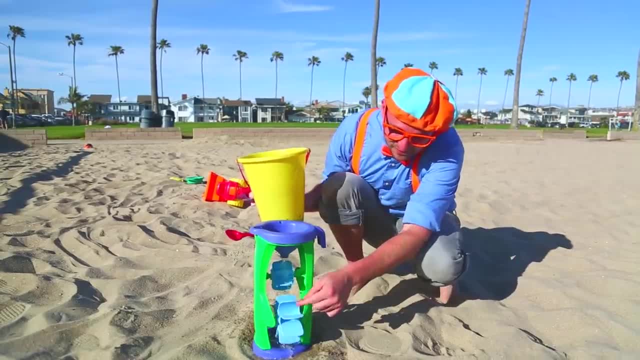 Okay, ready, Okay, here we go. Yeah, Oh yeah, It's working. Wow, That was so much fun playing with these sand toys with you. Well, I hope you enjoyed this video. I'll see you next time. 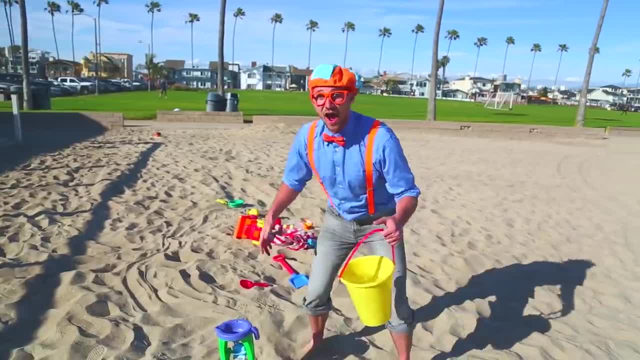 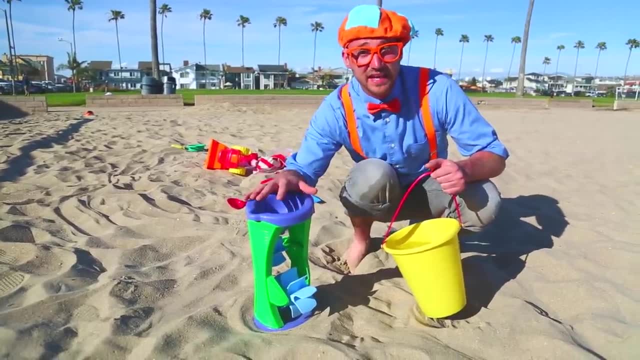 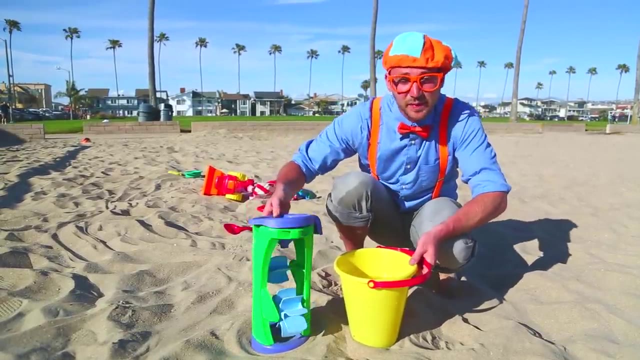 I kind of want to see what it's like pouring water in here. Okay, You know how these spin when we put sand in it. Yeah, Let's see if we pour water that we got from the ocean in here. if they spin, How does that look? 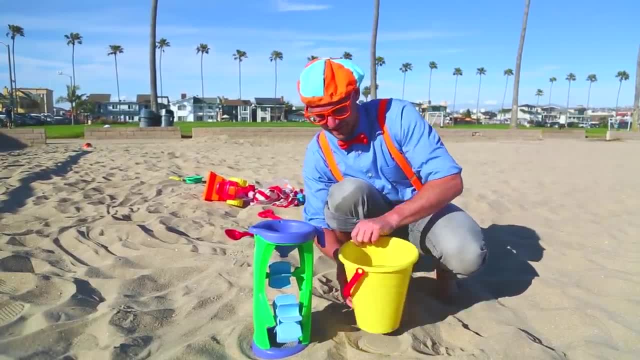 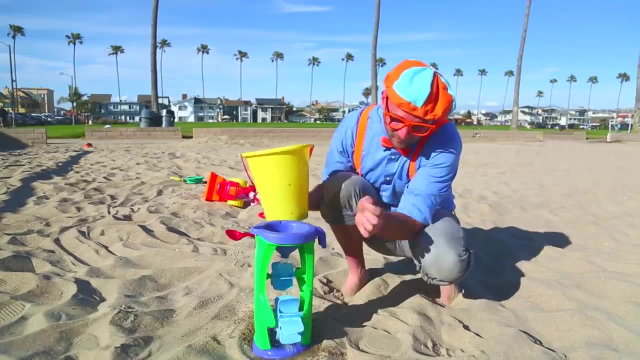 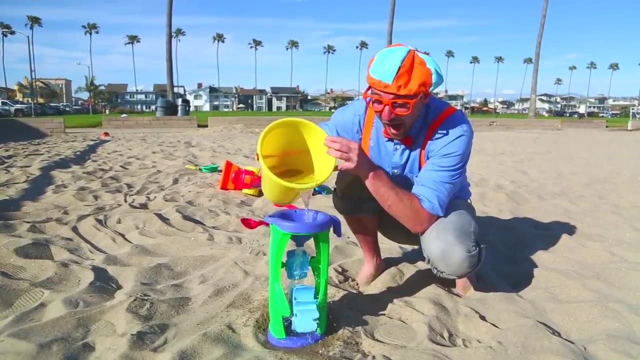 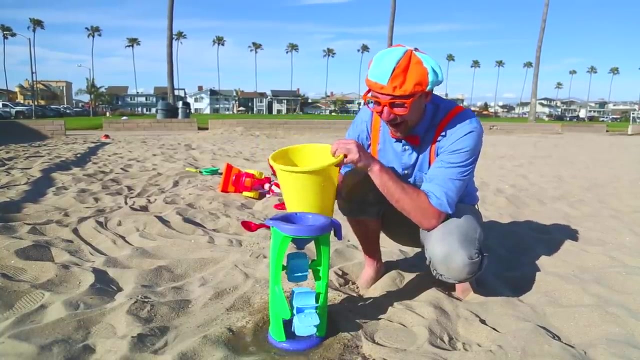 Can you see them? Yeah, Okay, Whoa, It's working. Okay, Let's fix this one. Okay, Ready, Okay, Here we go. Yeah, Oh, yeah, It's working. Wow, That was so much fun. 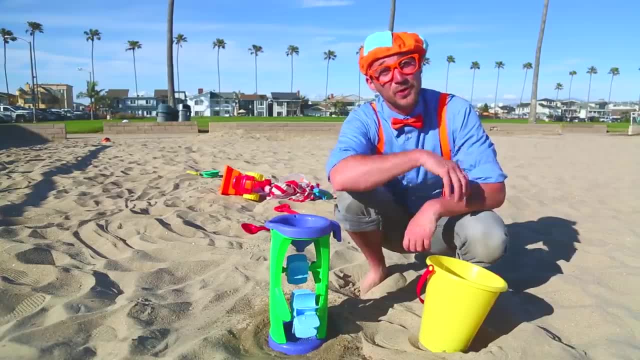 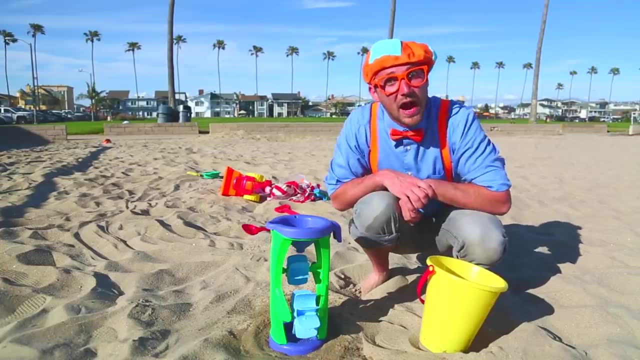 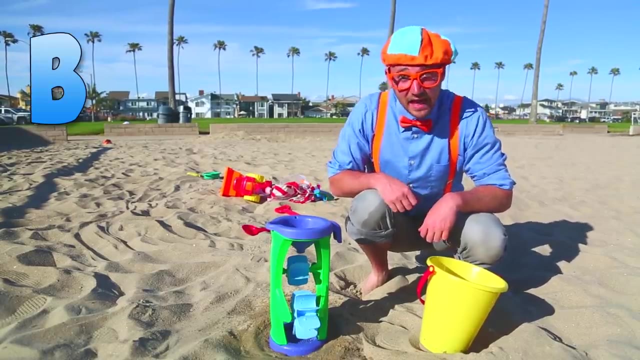 playing with these sand toys with you. Well, if you want to watch more of my videos, you know what to do. Search for my name. Do you know how to spell my name? Yeah, Let's spell it together: Ready B-L-I-P-P-I. 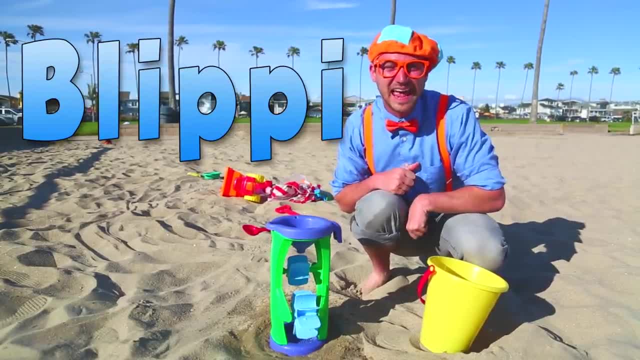 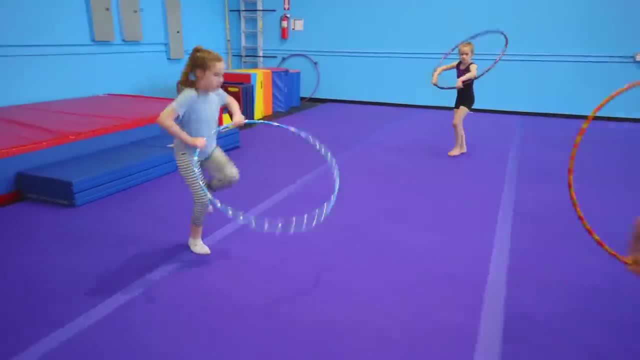 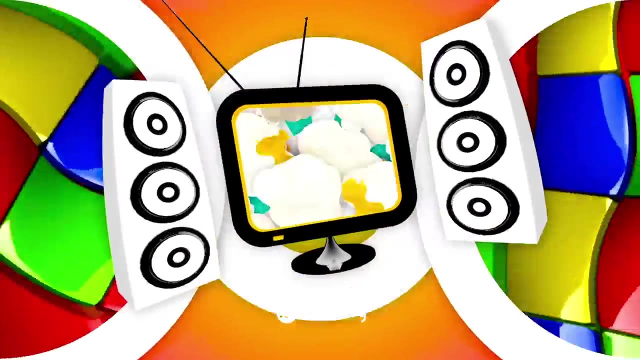 Blippi. Yeah, That's my name. Good job and see you again. Bye-bye, It's me Blippi, and this place is where kids can come learn some circus skills. Hey, it's me Blippi, and today I'm at. 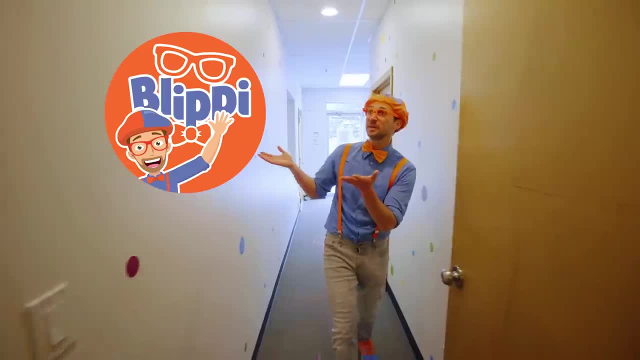 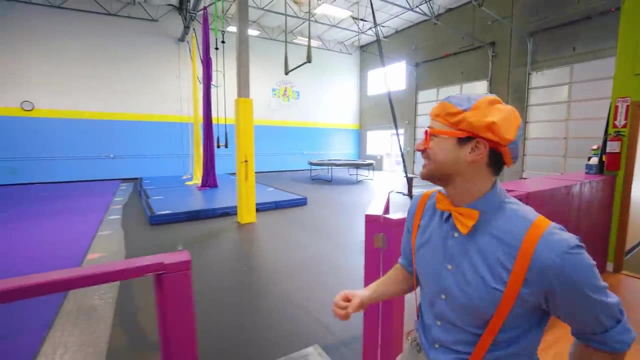 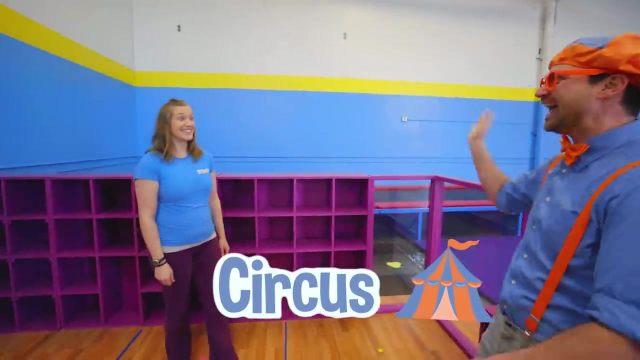 Synapt Circus Center in Auburn, Washington. Whoa, Look at this place. Whoa, It is so colorful And this place is where kids can come learn some circus skills. Oh hey, Who are you? I'm Coach Crystal and I'm going to teach you. 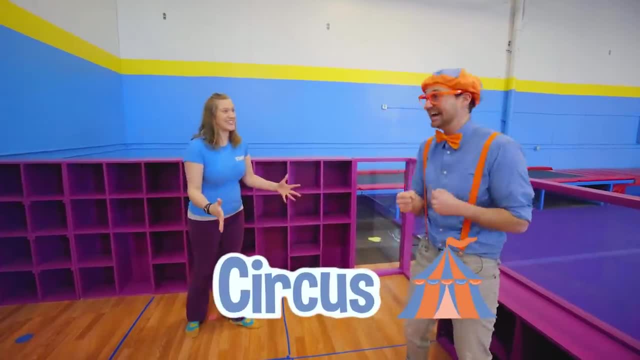 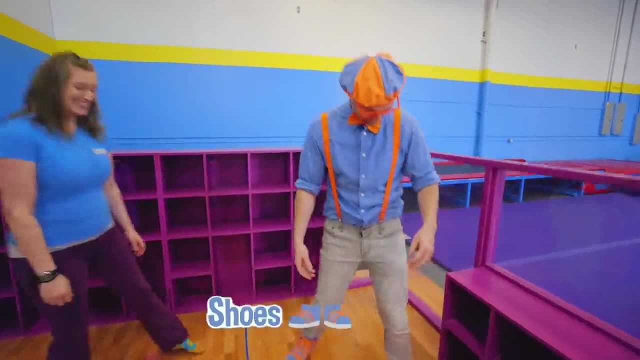 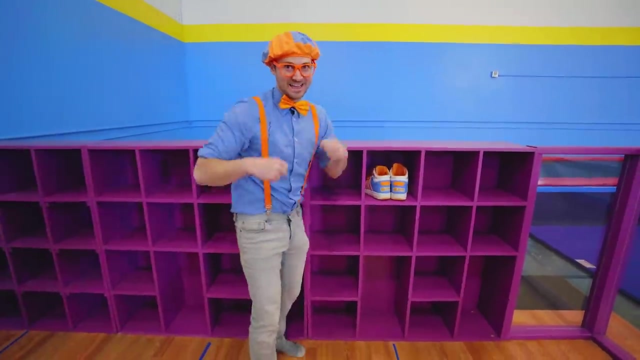 some circus skills today. Yeah, I'm so excited. The first thing you have to do is take off your shoes. Okay, Okay, I got to take off my shoes. Okay, Here we go. One shoe, Two shoe, All right, Now that my shoes are off. 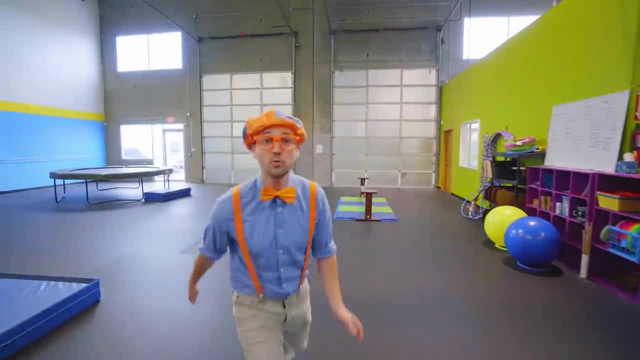 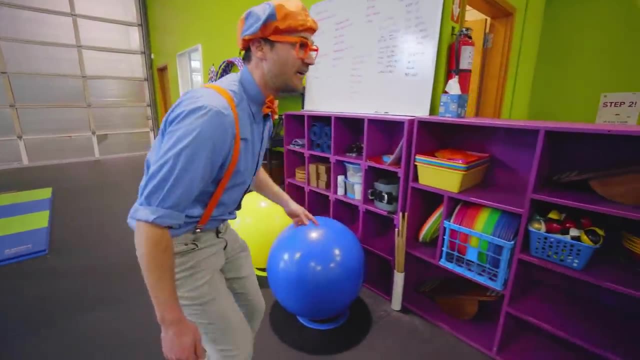 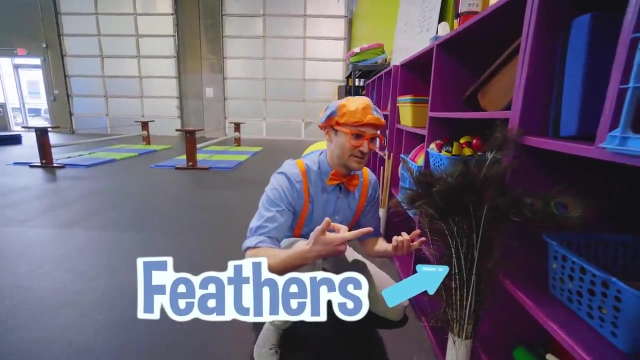 now we get to learn. Whoa, Check this place out. It's so cool. Looks like we have a lot of cool things over here. Whoa, Yeah, Looks like juggling balls. We'll get to those later. Feathers, What are these doing here? 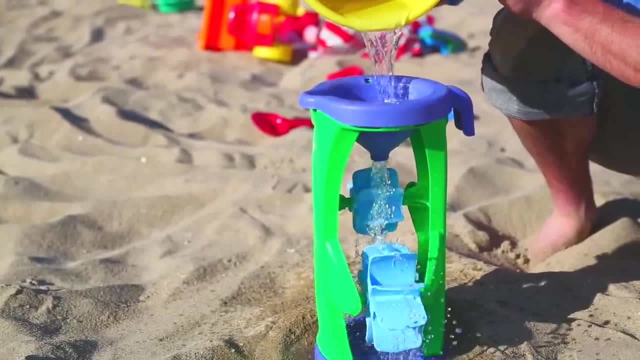 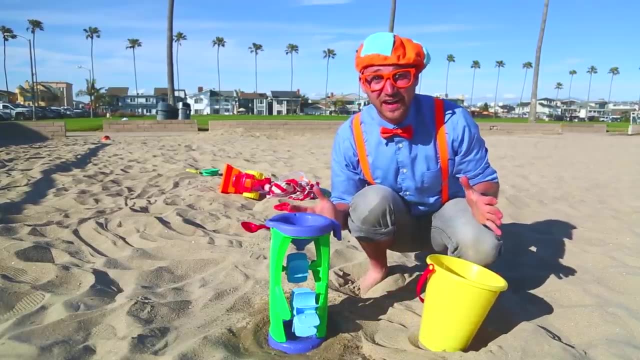 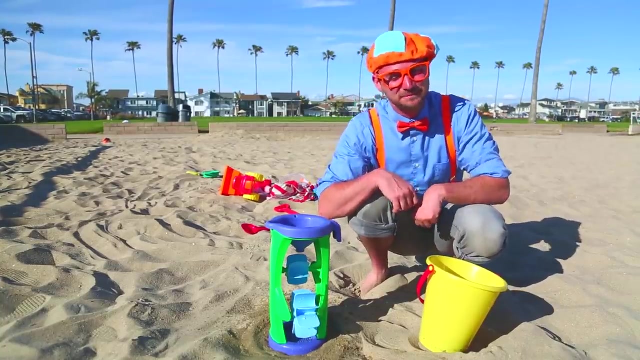 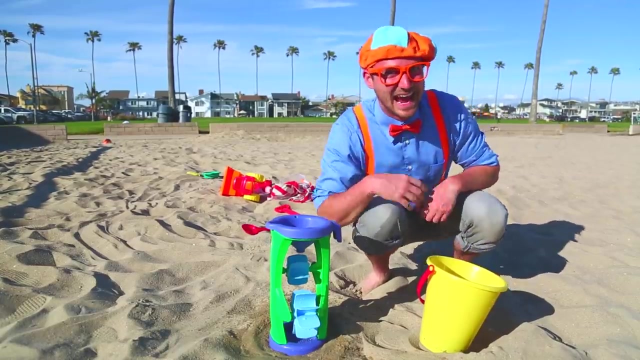 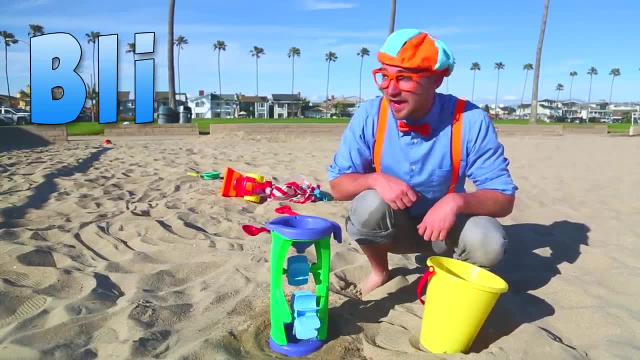 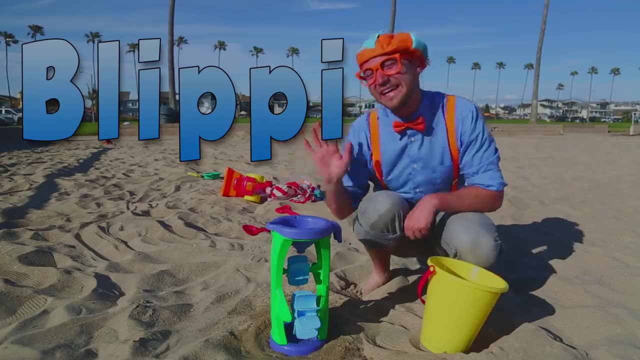 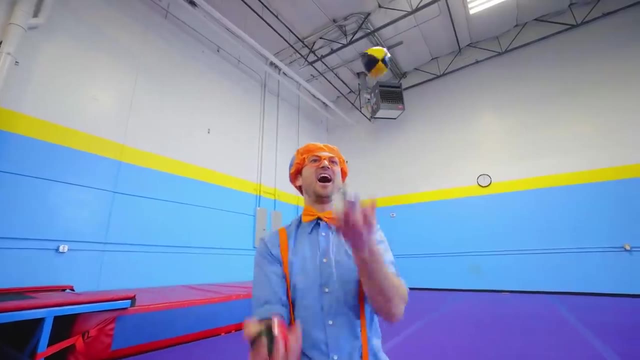 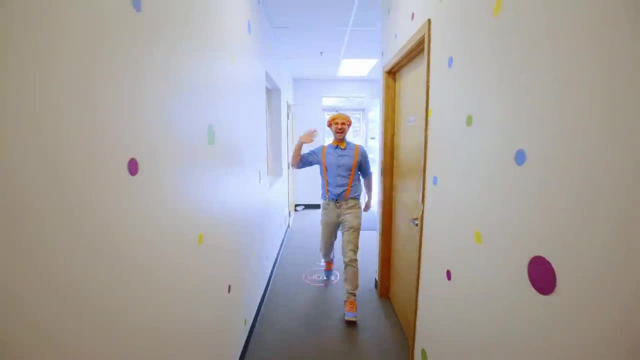 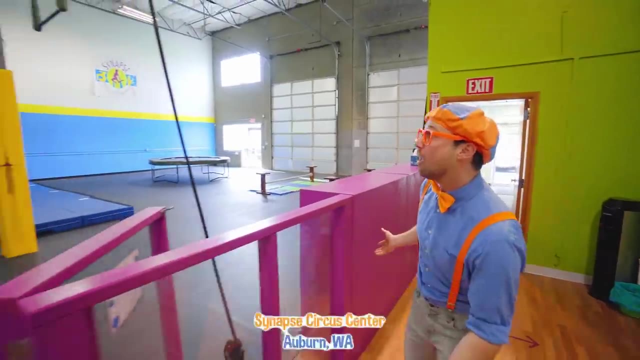 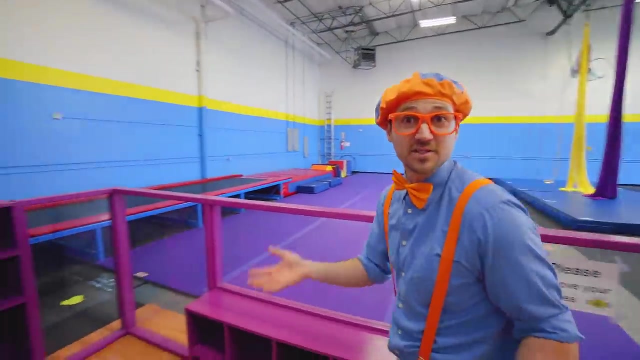 Blippi. Hey, it's me Blippi, and today I'm at Synapse Circus Center in Auburn, Washington. Whoa, look at this place. Whoa, it is so colorful. And this place is where kids can come learn some circus skills. 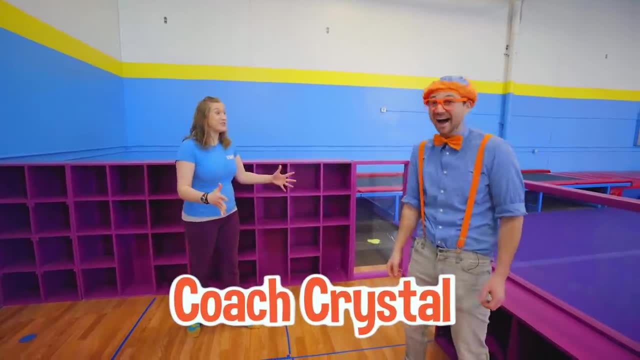 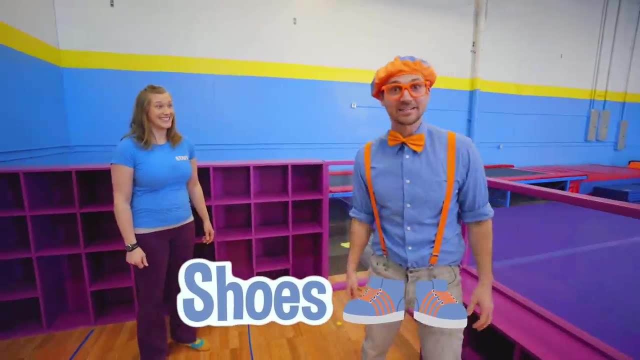 Oh hey, who are you? I'm Coach Crystal and I'm going to teach you some circus skills today. Yeah, I'm so excited. The first thing you have to do is take off your shoes. Okay, I gotta take off my shoes. 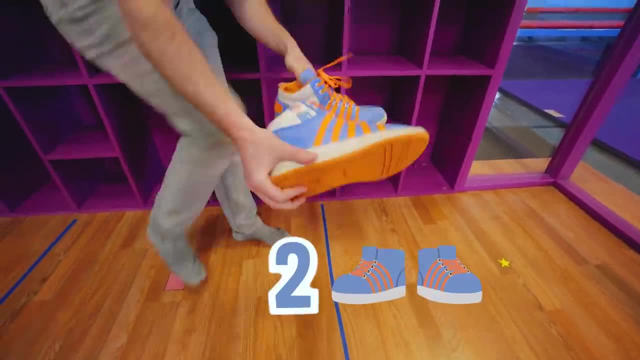 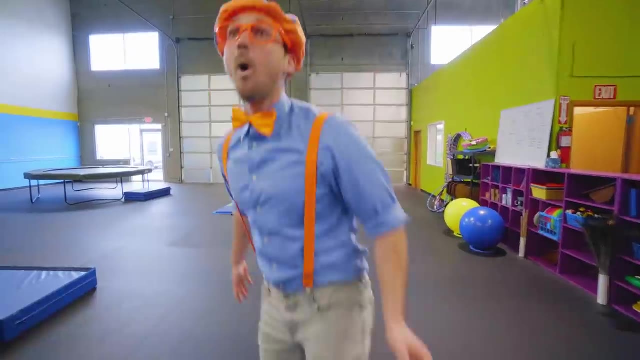 Okay, here we go. One shoe, two shoes. Alright, now that my shoes are off. now we get to learn. Whoa, check this place out. This is so cool. Looks like we have a lot of cool things over here. 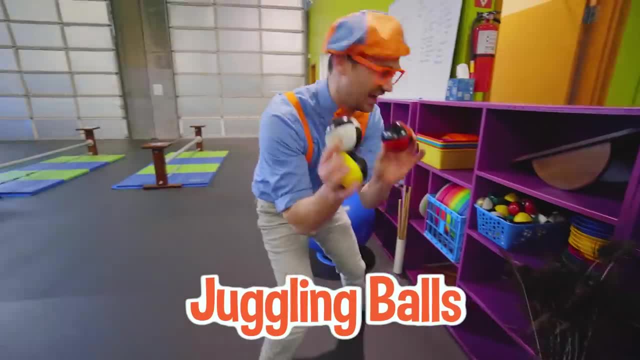 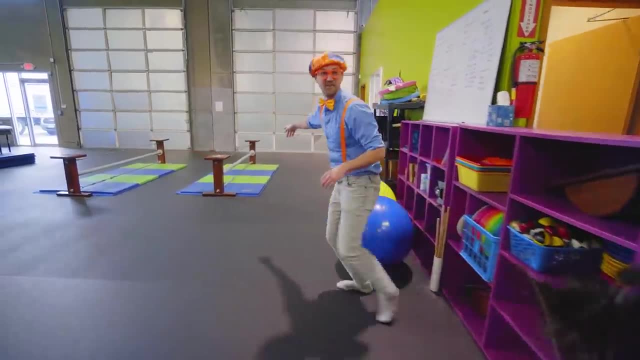 Whoa, yeah, looks like juggling balls. We'll get to those later. Feathers- What are these doing here? That's so silly. Whoa, look, Looks like tight wires. I am so excited to balance on these later. 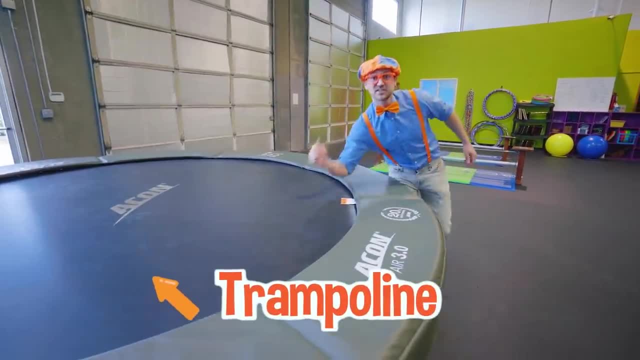 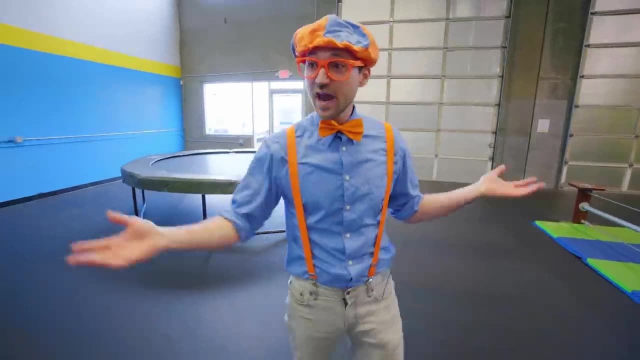 Wow, a trampoline. These are so bouncy. I really want to jump on this, but I probably shouldn't until I warm up and stretch. Yeah Whoa, look at this, Looks like a bar that you can hang on. 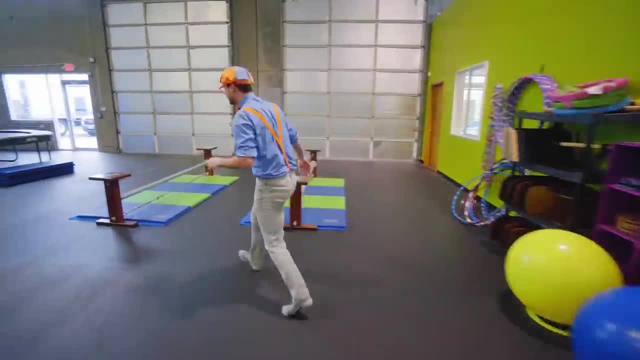 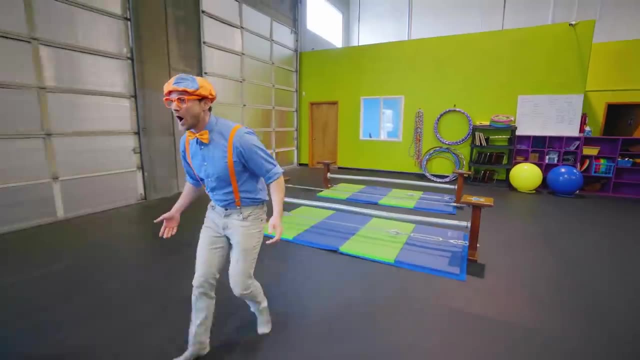 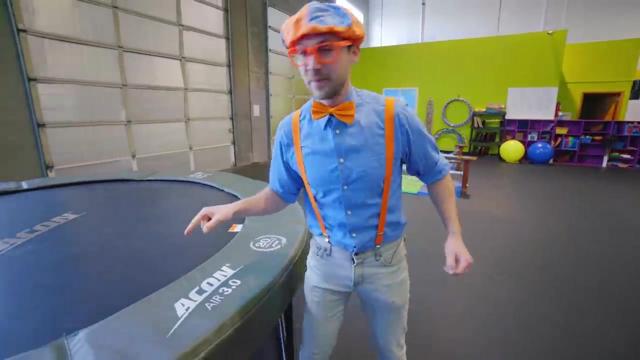 That's so silly. Whoa Looks like tight wires. I am so excited to balance on these later. Wow, A trampoline. These are so bouncy. I really want to jump on this, but I probably shouldn't until I warm up. 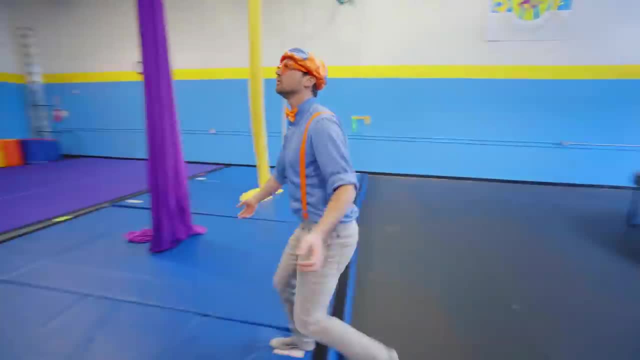 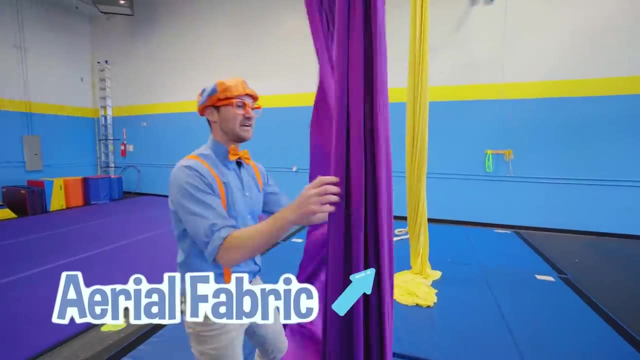 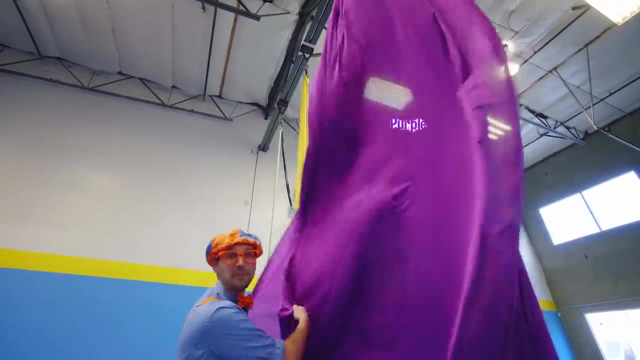 and stretch. Yeah, Whoa, Look at this. Looks like a bar that you can hang on. Whoa, Oh, An aerial fabric. Wow, What color is this? Yeah, This is the color purple. Oh, And over here, 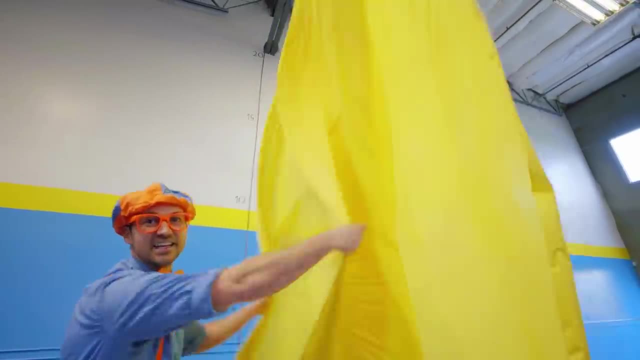 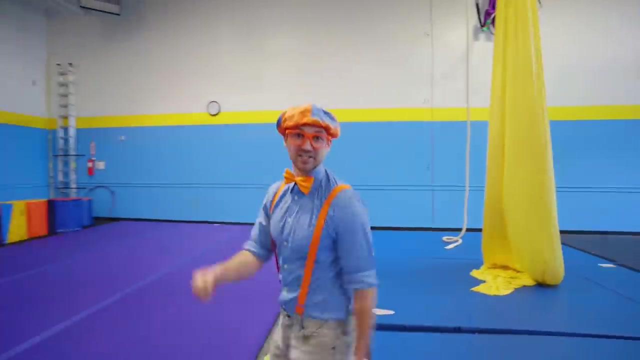 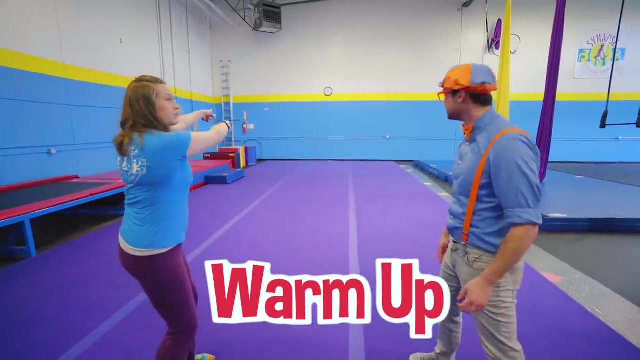 another one. This is the color yellow. Okay, Enough playing, Let's get warmed up, so then we can stretch and have some fun. Oh, Hey, Hi Brittany, You ready to warm up? Yeah, I'm ready. All right, We're going to run to the blue wall. 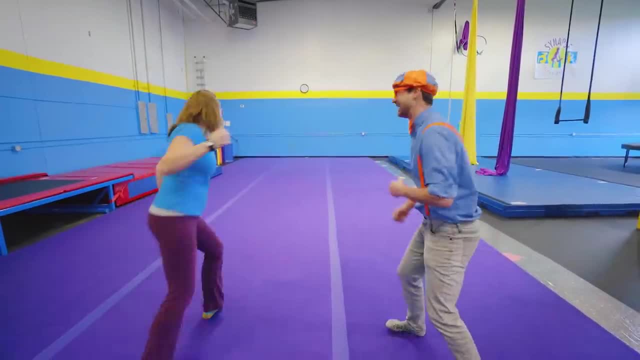 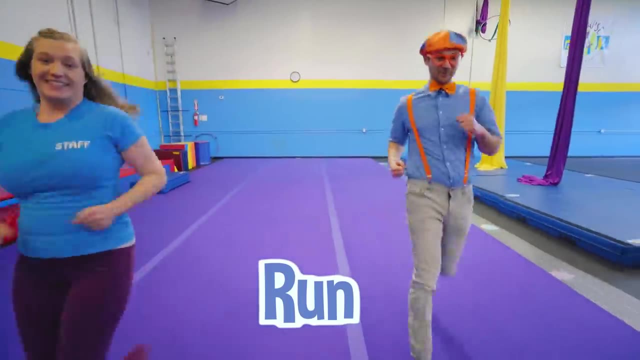 and then we're going to run back to get our bodies all ready to go. Okay, Let's go Check it out. I'm running, Whoa. All right, Let's make our circle in the middle of the park, Okay. 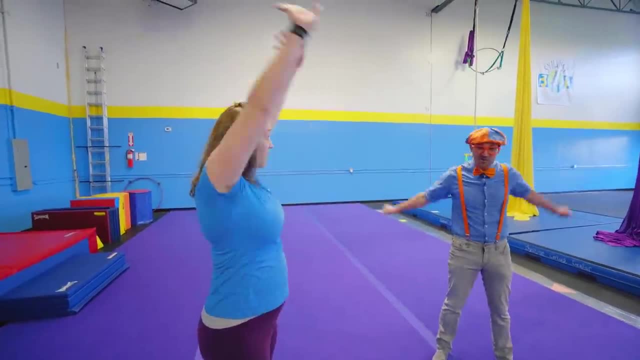 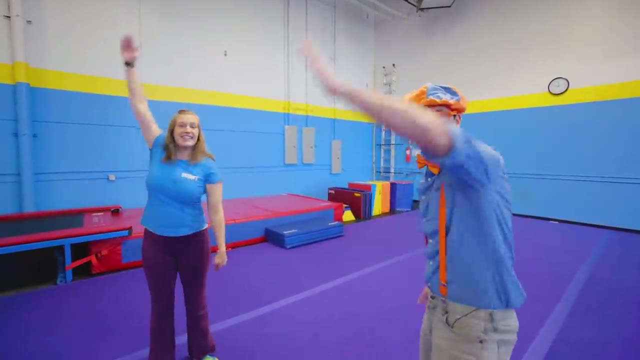 Arm circles backwards, Get our arms all ready to hang on the aerial fabric and the trapeze. Whoa, All right, Let's go forward now, like you're swimming. Okay, Check it out. I'm making big circles with my arm. 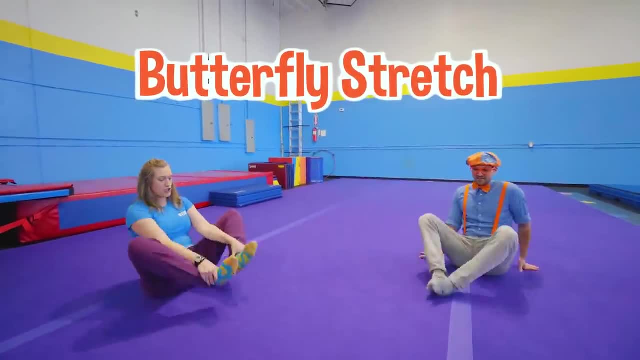 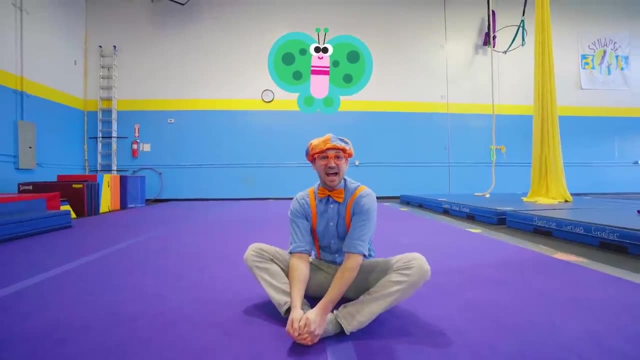 All right, Let's sit down in our butterfly, Put your toes together and make a butterfly. Whoa, Check it out, I'm flopping like a butterfly. Yeah, Butterflies start as caterpillars, They go through metamorphosis and then 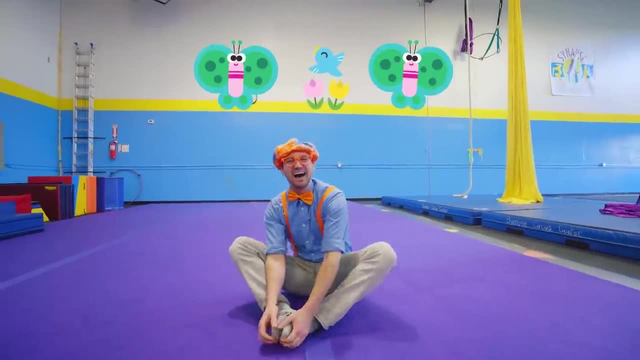 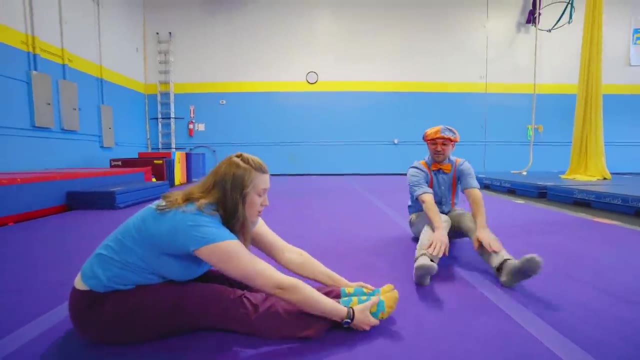 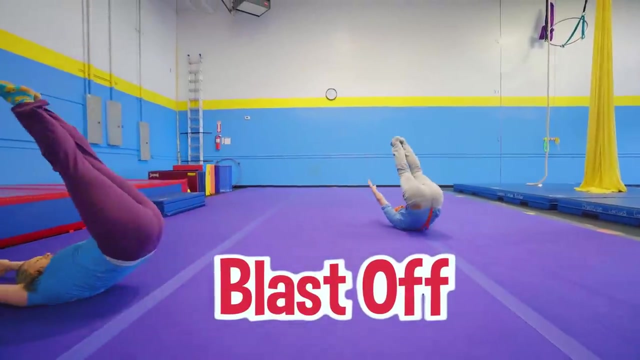 they become beautiful butterflies. Okay, Close your wings and squash them flat. We're going to blast off to the moon. Grab those toes Ready. Five, four, three, two, one. Blast off, Whoa. Try it one more time. 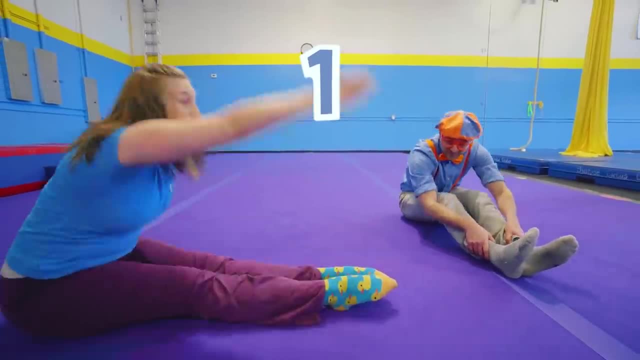 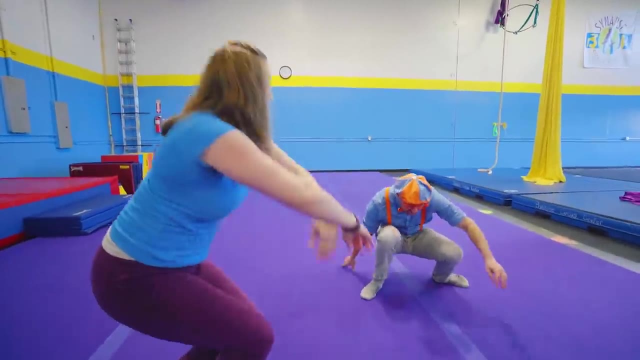 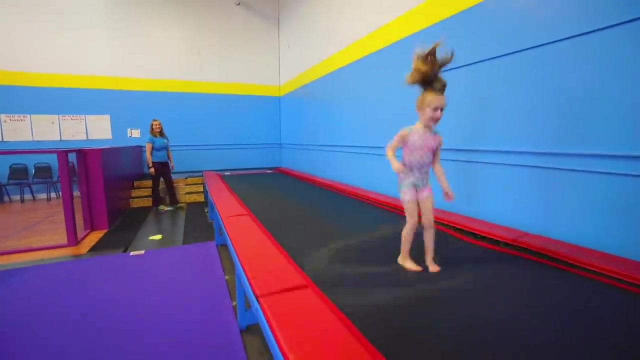 This time we're going to start at three, Three, two, one Blast off. Yeah, All right, Go ahead and stand back up. You feel warmed up? Yeah, All right, Let's go do some circuit stuff, Let's go. 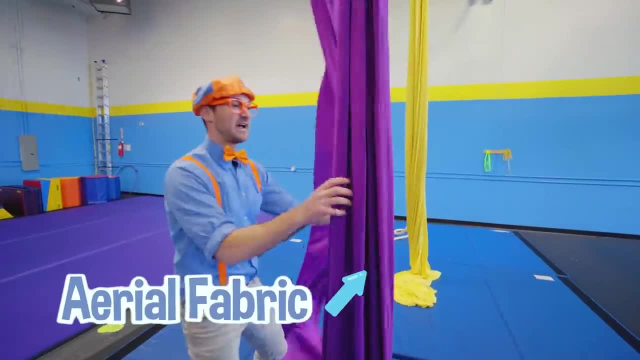 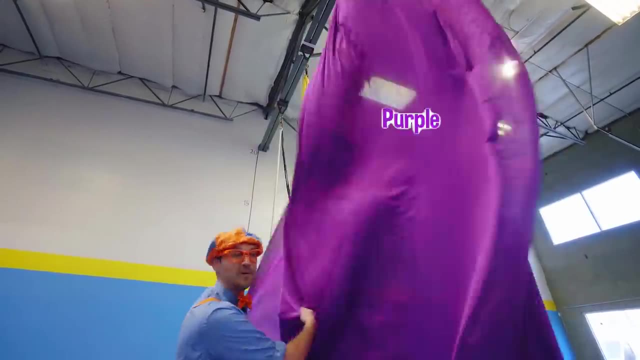 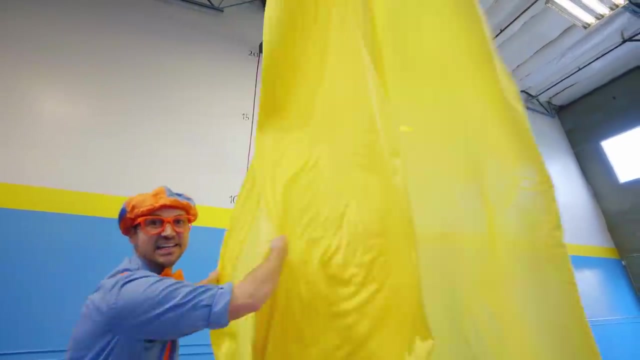 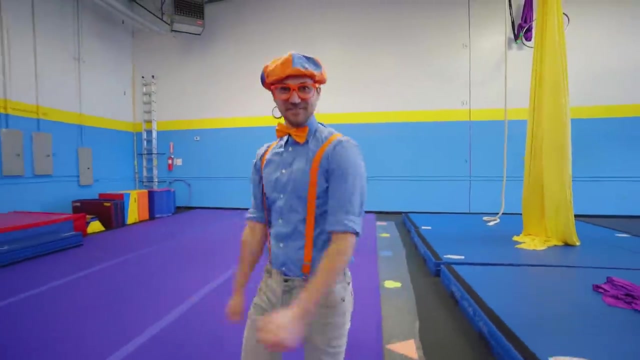 Whoa, oh, an aerial fabric. Wow, what color is this? Yeah, this is the color purple. Oh, and over here another one. This is the color yellow. Okay, enough playing, let's get warmed up, so then we can stretch and have some fun. 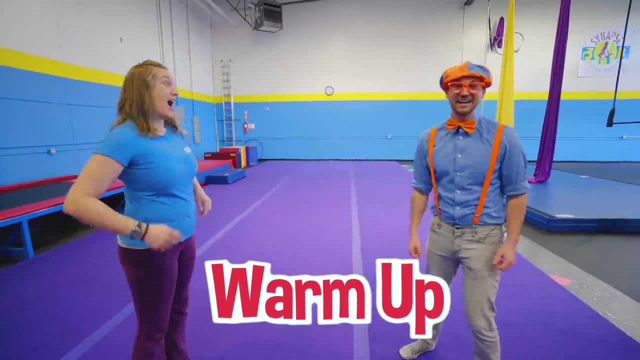 Oh hey, Hi Brittany, you ready to warm up? Yeah, I'm ready. Alright, We're going to run to the blue wall and then we're going to run back to get our bodies all ready to go. Okay. 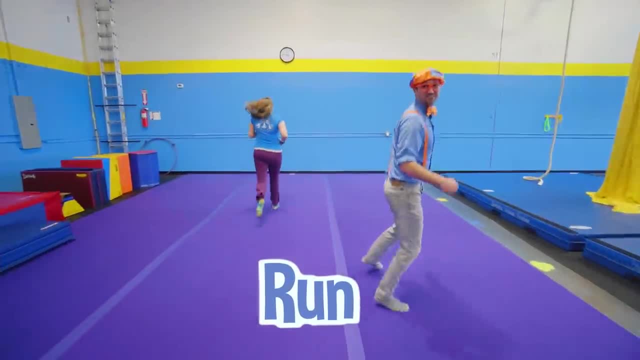 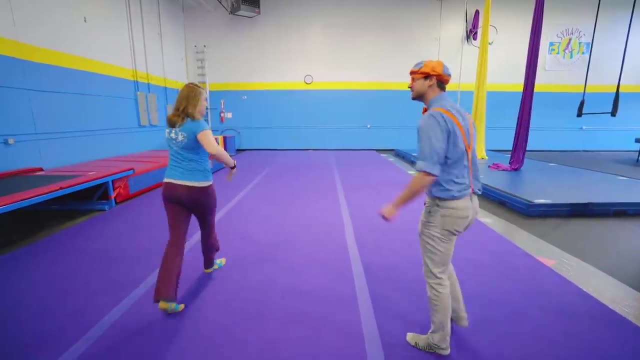 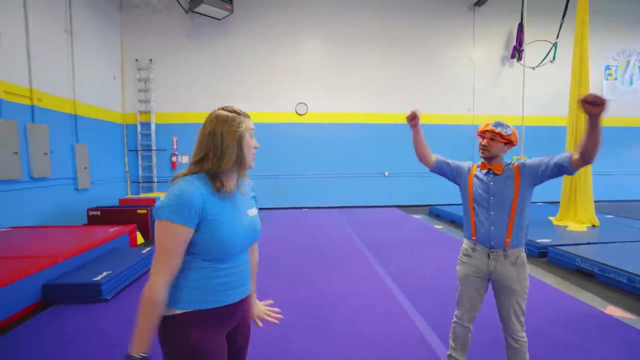 Ready? let's go Check it out. I'm running, Whoa. Alright, let's make our circle in the middle of the park. Okay, Arm circles backwards. We have to get our arms all ready to hang on the aerial fabric and the trapeze. 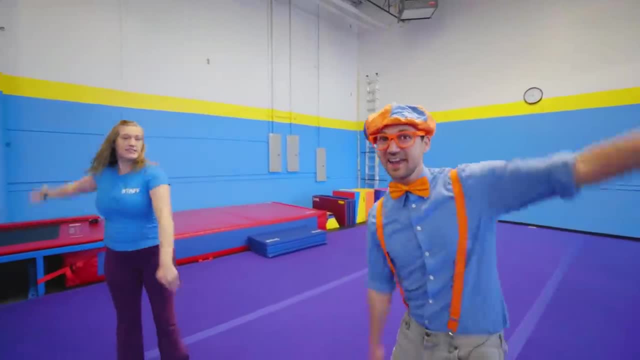 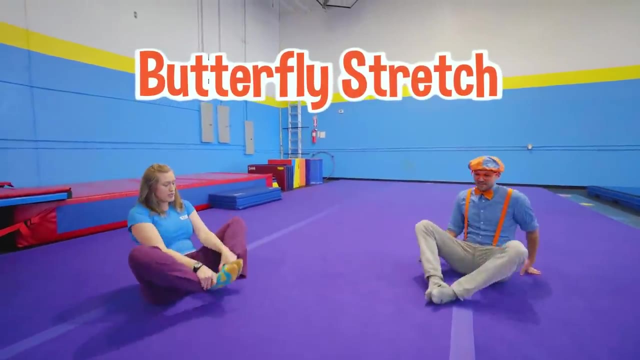 Whoa, Alright, let's go forward now, like you're swimming. Okay, check it out. I'm making big circles with my arms. Alright, let's sit down in our butterfly, Put your toes together and make a butterfly. Oh, check it out, I'm flapping like a butterfly. 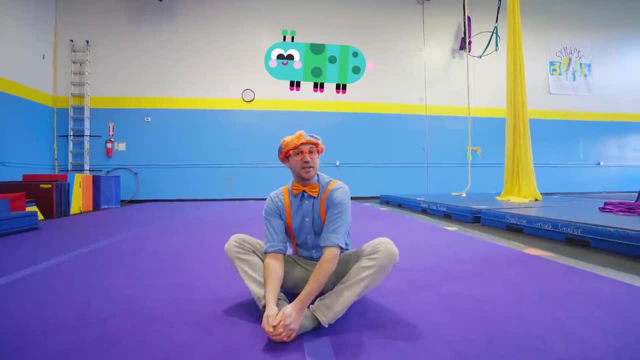 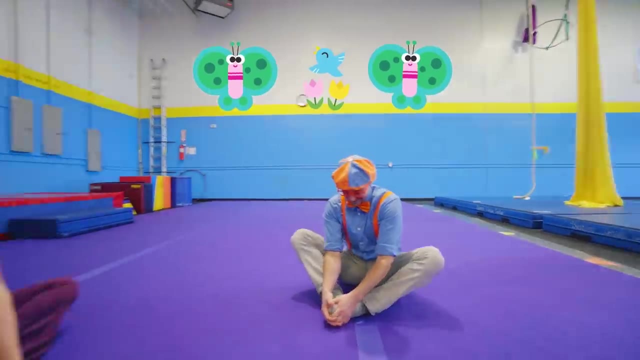 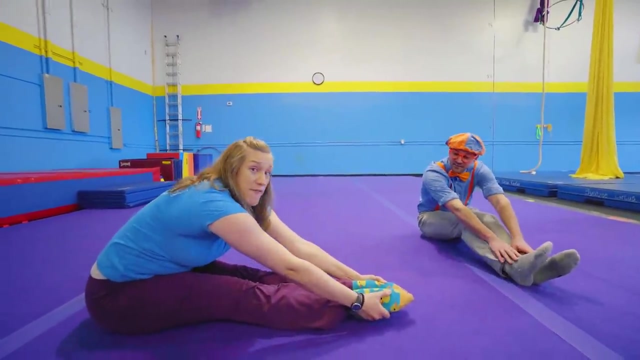 Yeah, butterflies start as caterpillars, they go through metamorphosis and then they become beautiful butterflies. Okay, close your wings and squash them flat. We're going to blast off to the moon. grab those toes, Ready Five. 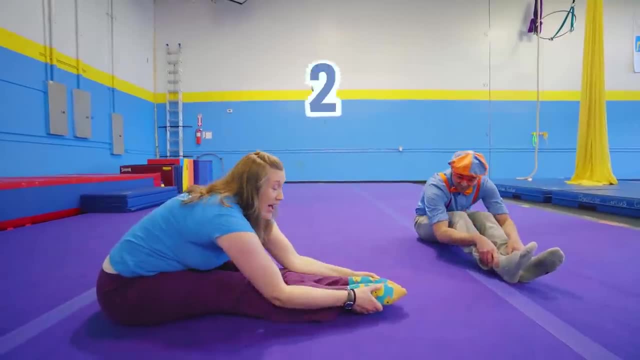 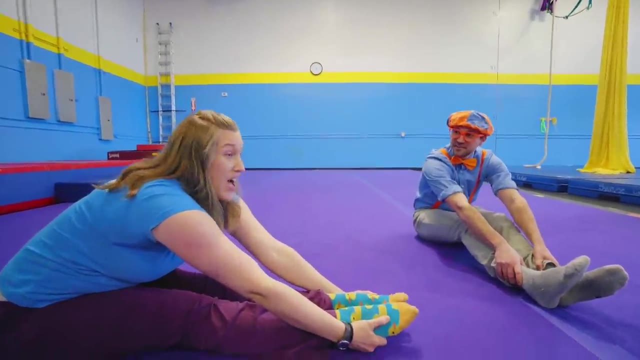 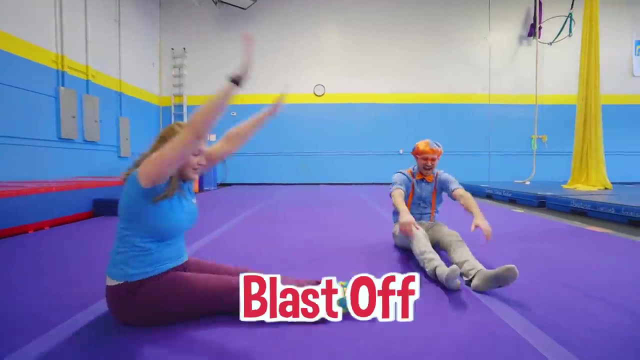 Four, Three, Two, One Blast off- Whoa, Alright, we're going to do it one more time. this time we're going to start at three, Three, Two, One Blast off. Whoa, Yeah, Alright, go ahead and stand back up. 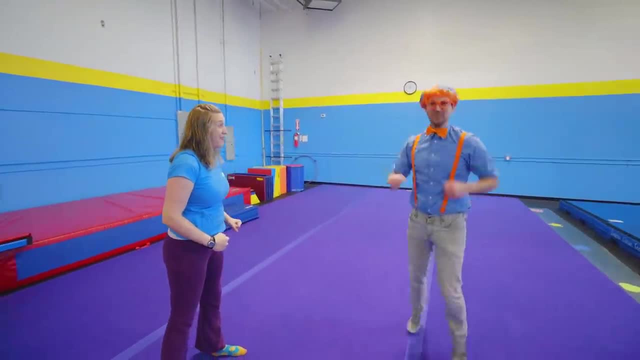 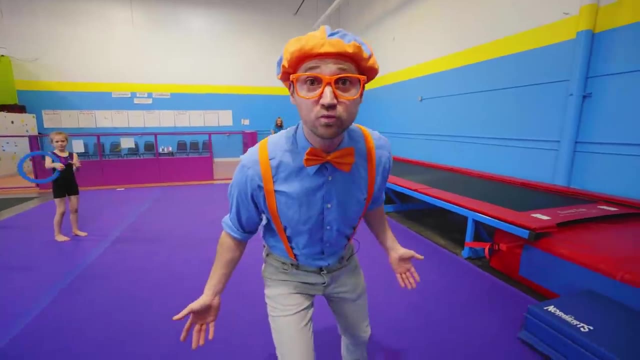 You feel warmed up? Yeah, Alright, let's go do some circuit stuff. Woohoo, let's go. Whoa, that was really good. Did you see how high she was jumping? Yeah, Whoa, And look at what she's doing. 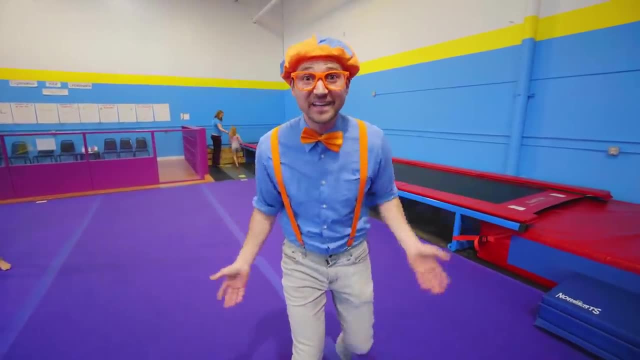 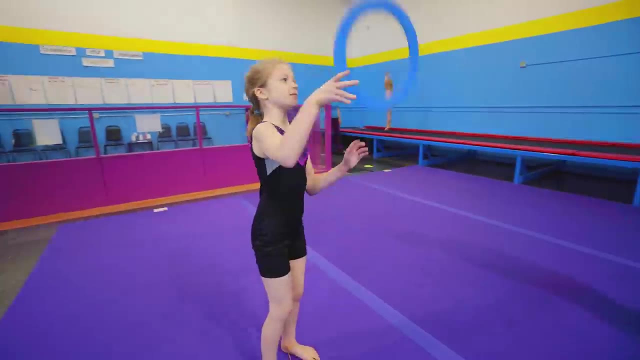 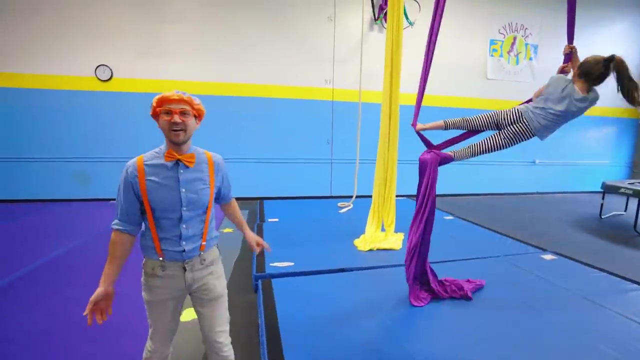 Whoa, That was really good. Did you see how high she was jumping? Yeah, Whoa, Look at what she's doing. Whoa, It is so cool how kids can come here and learn circus skills. Whoa, Look at her. 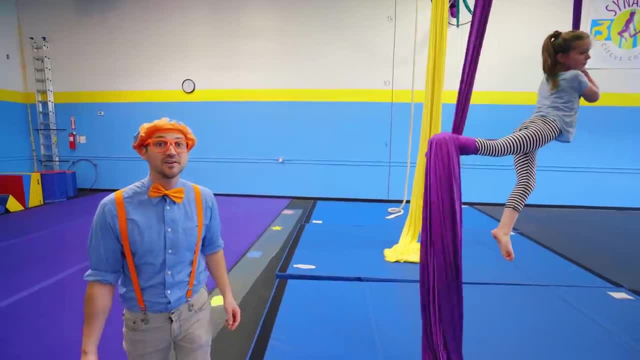 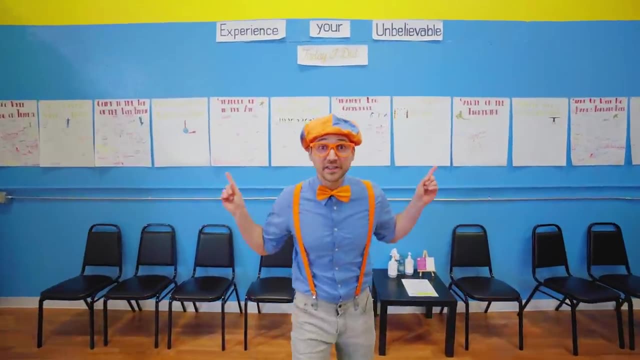 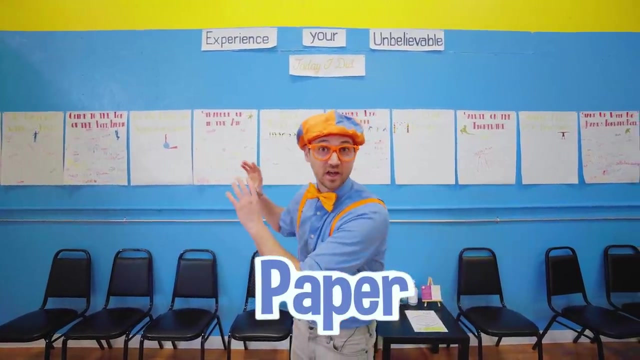 Whoa, She's using that aerial silk. so good, Check it out. Wow, Look at this area. This is so cool. Do you see these big pieces of paper behind me? Yeah, They have things written on them. Yeah, Like gold. 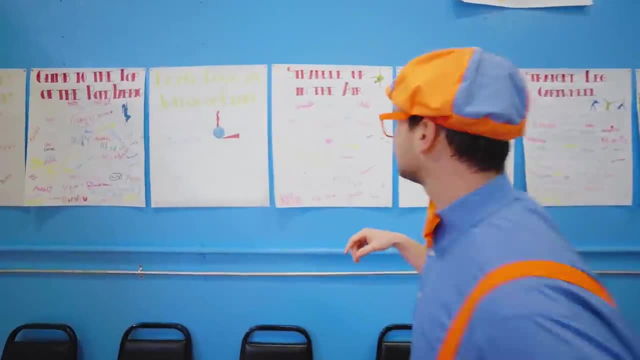 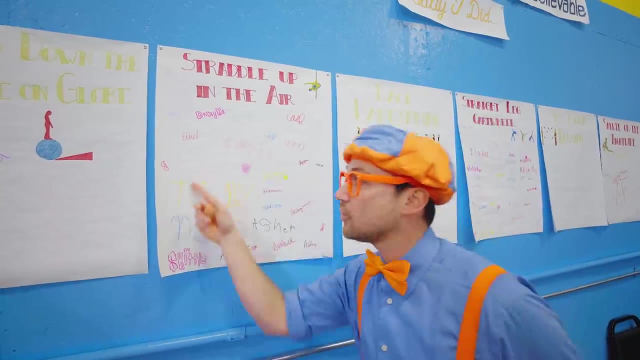 Once you accomplish that, you get to write your name on the board. Let's check it out. Straddle up in the air: Whoa, That means all these people that wrote their names on here. yeah, they accomplished that, Like Neil Alyssa. 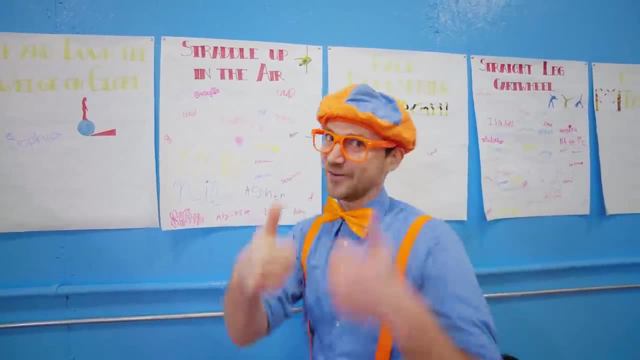 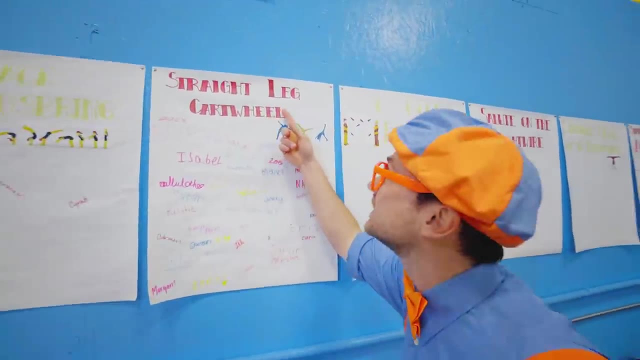 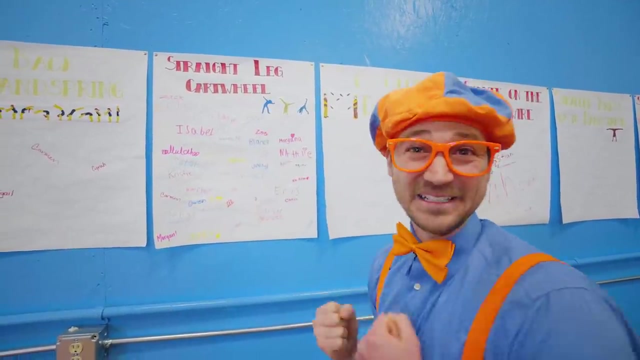 Jonah Zoey: Wow, Good job. Whoa, Let's see what else. Wow, Straight leg cartwheel- Whoa, That's hard. But look at all the people that did it. Whoa, That is so cool, Ooh. 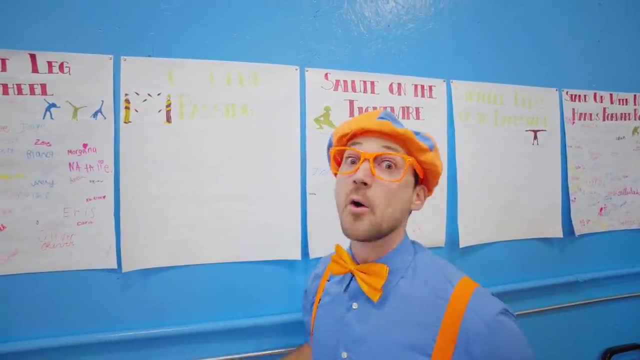 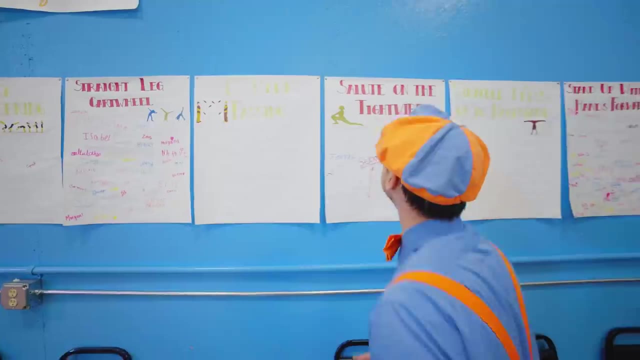 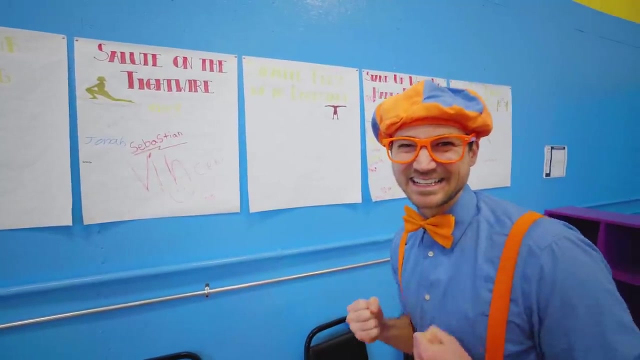 Six club passing. Wow, Now that is hard. Yeah, Not one single person accomplished it. Whoa, That's crazy. Hmm, I have an idea. What if I pick one of these and try and accomplish it today? That sounds like so much. 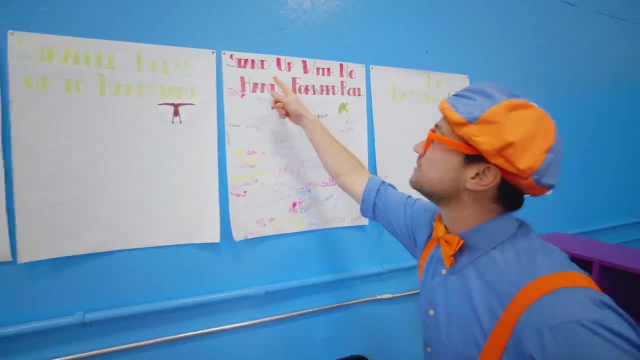 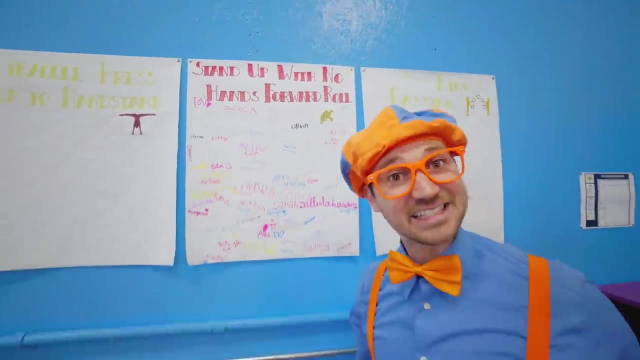 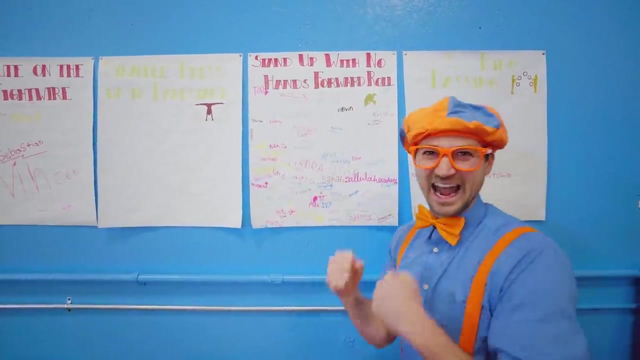 fun. Um, Oh, Here we go. Stand up with no hands, Forward roll. Oh, That seems fun. It's like a somersault, but then at the end, when you stand up, you can't use your hands. Yeah, I think. 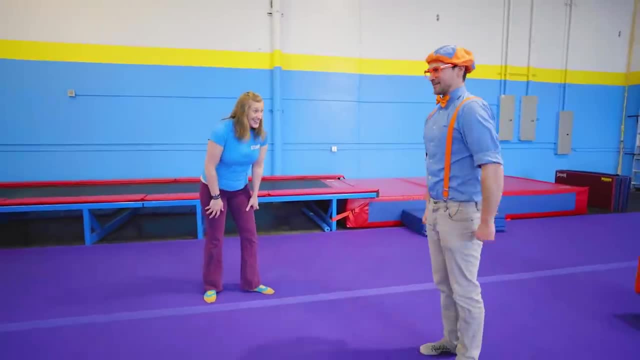 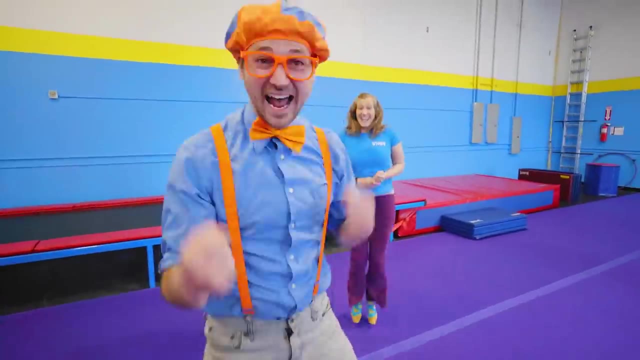 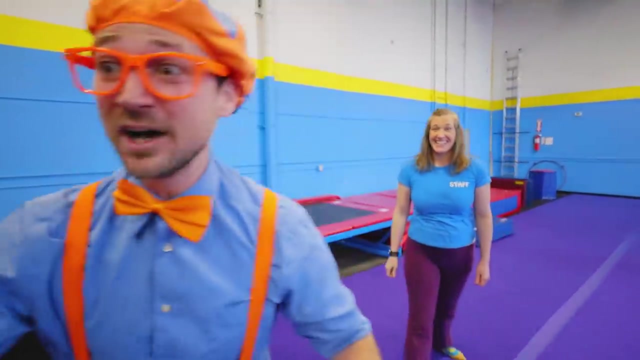 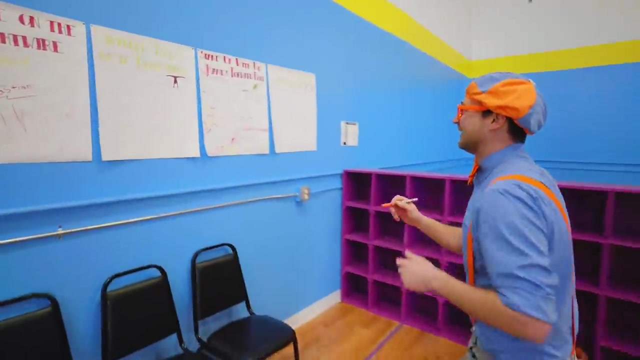 I should try that. This is gonna be fun. Yeah, I did it. Here's the pen. You can go write your name on the board now. Really, This is awesome. Oh, Yeah, Whoa, Yeah. Okay, Here we. 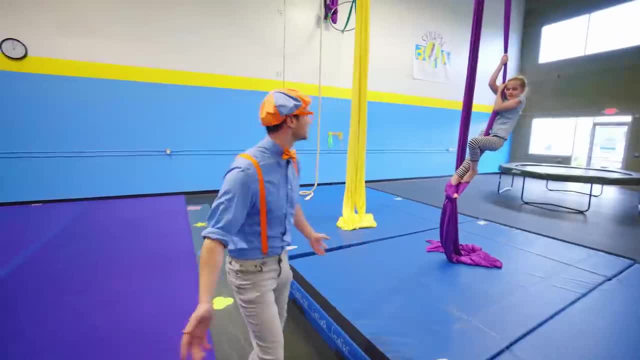 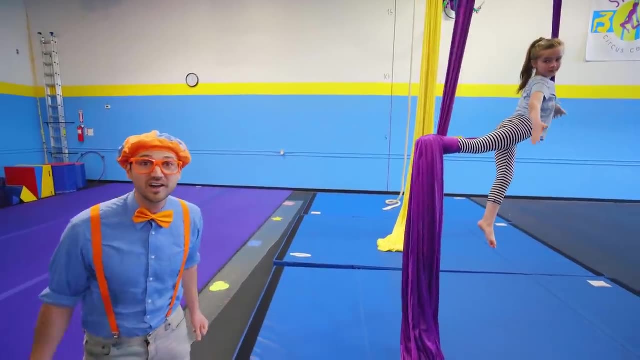 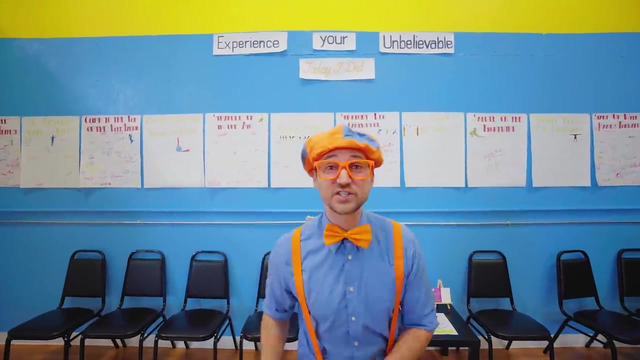 It is so cool how kids can come here and learn circus skills. Whoa, Look at her. Whoa, She's using that aerial silk. so good, Check it out. Wow, Look at this area. This is so cool. Do you see these big pieces of paper behind me? 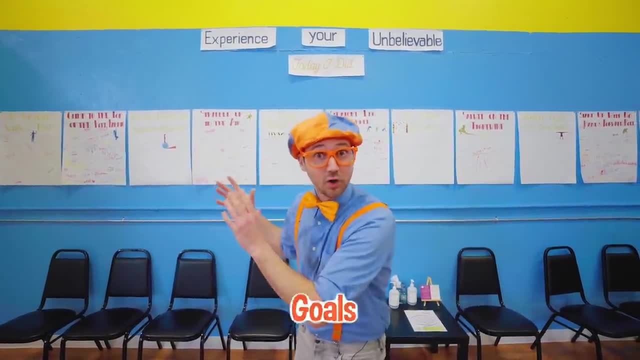 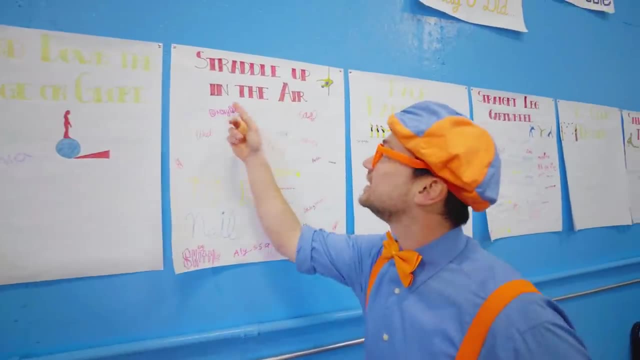 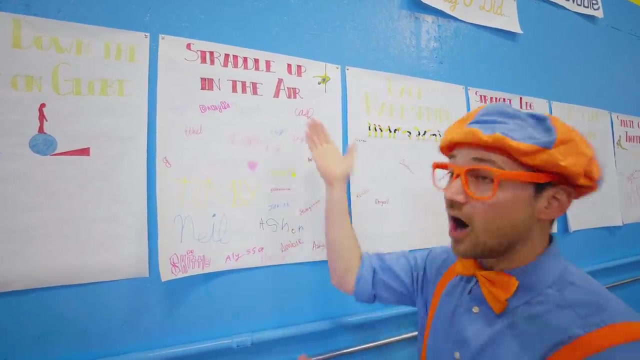 Yeah, They have things written on them. Yeah, Like gold, And once you accomplish that, you get to write your name on the board. Let's check it out. Straddle up in the air- Whoa, That means all these people that wrote their names on here. yeah, they accomplished that. 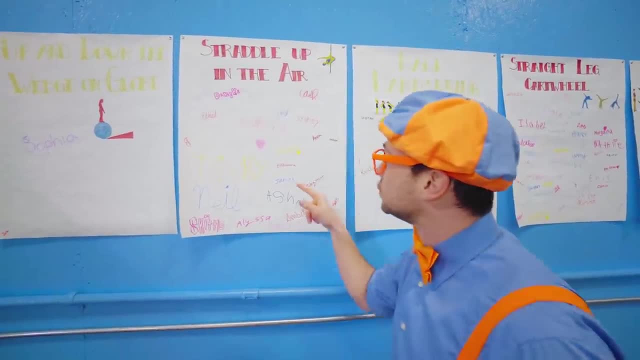 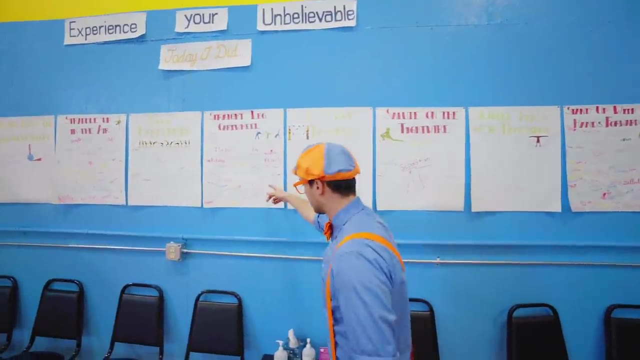 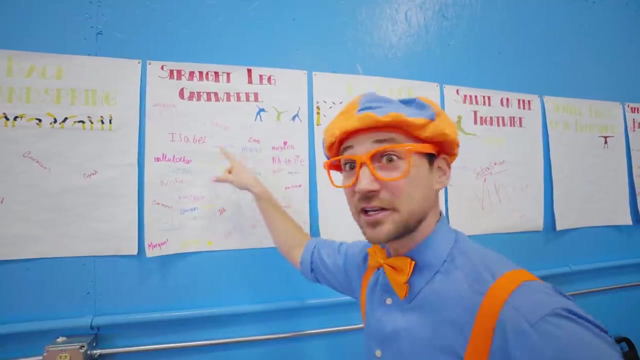 Like Neil Alyssa, Jonah Zoe- Wow, Good job. Whoa, Let's see what else. Um, wow, Straight leg cartwheel- Whoa, That's hard, But look at all the people that did it, Whoa. 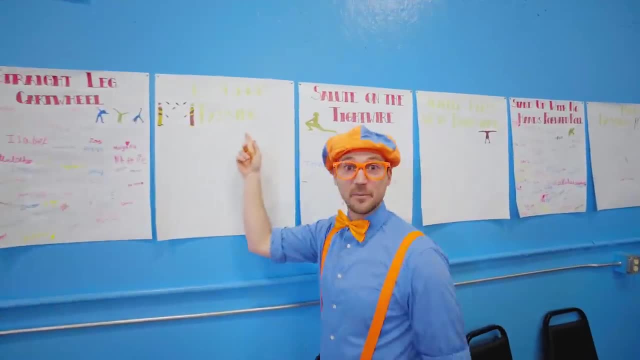 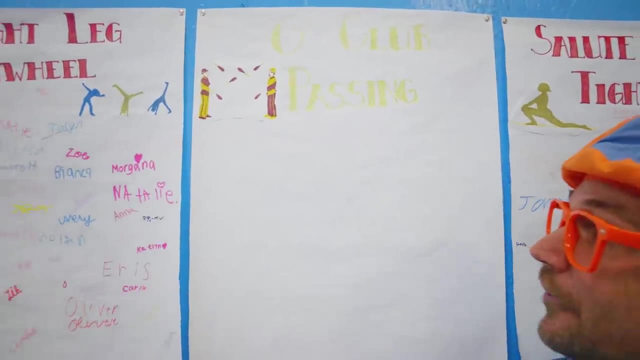 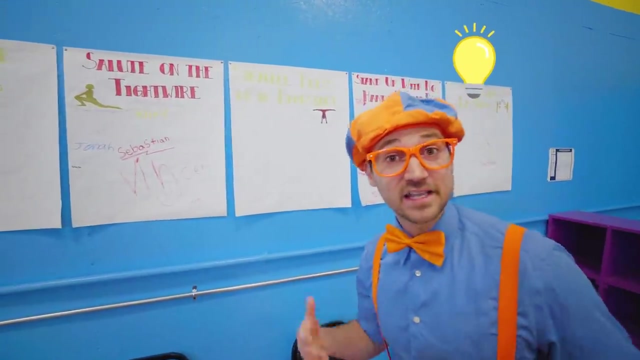 That is so cool. Ooh, Six club passing. Wow, Now that is hard. Yeah, Not one single person accomplished it. Whoa, That's crazy. Hmm, I have an idea: What if I pick one of these and try and accomplish it today? 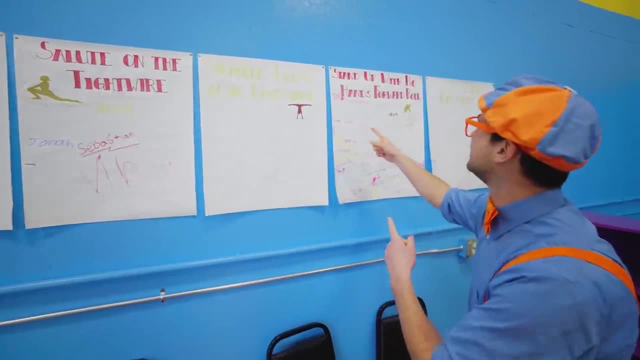 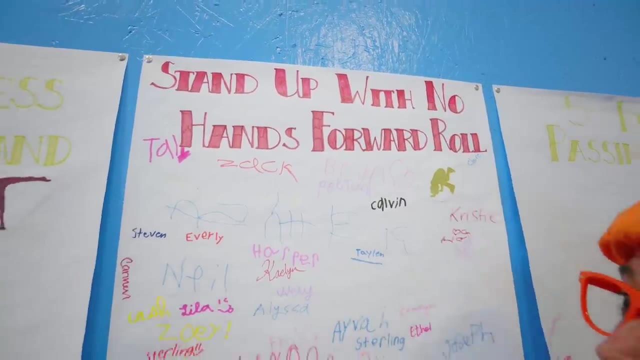 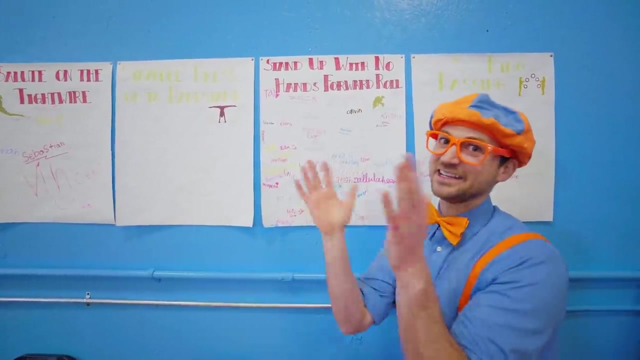 That sounds like so much fun. Um, oh, here we go, Stand up with no hands, forward roll. Oh, That seems fun, It's like a somersault. but then at the end, when you stand up, you can't use your hands. 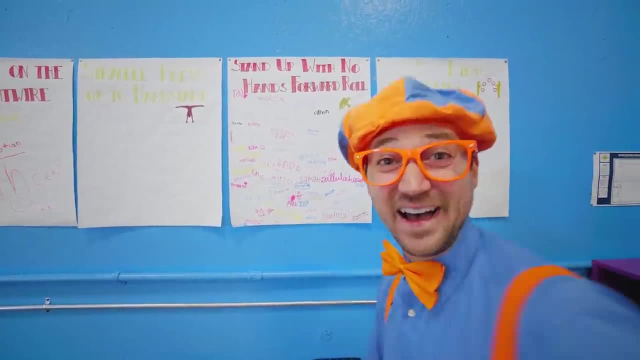 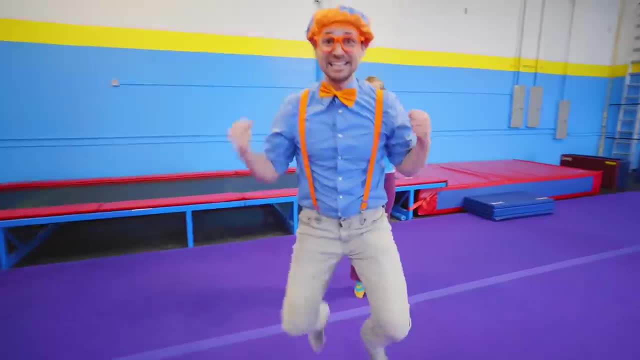 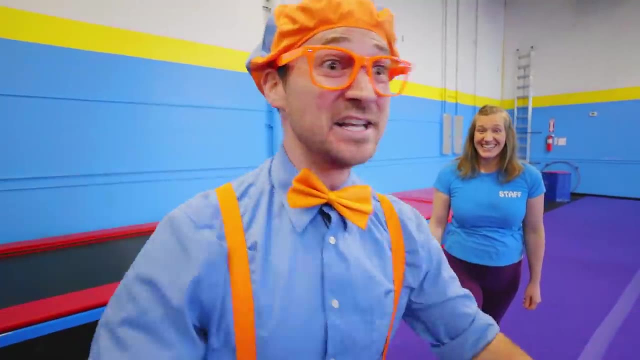 I'm going to try it. Yeah, I did it. This is a pen. You can go write your name on the board now. Really, This is awesome. Oh, Yeah, Whoa, Yeah. Okay, here we go. Now it's time to write my name. 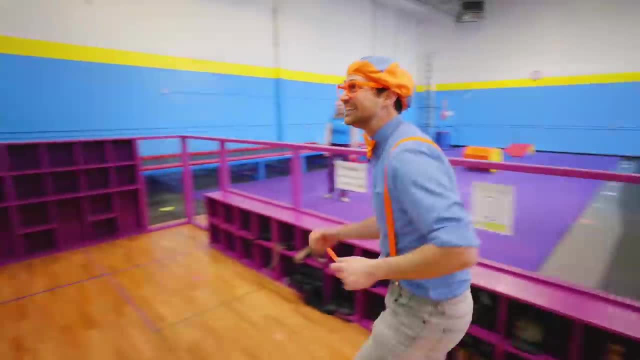 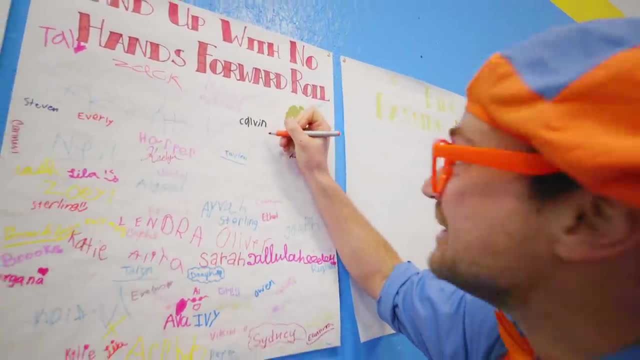 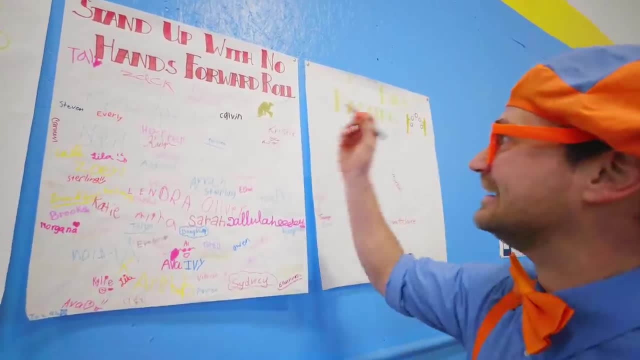 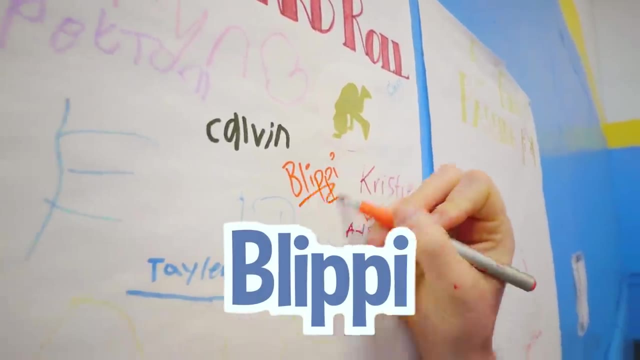 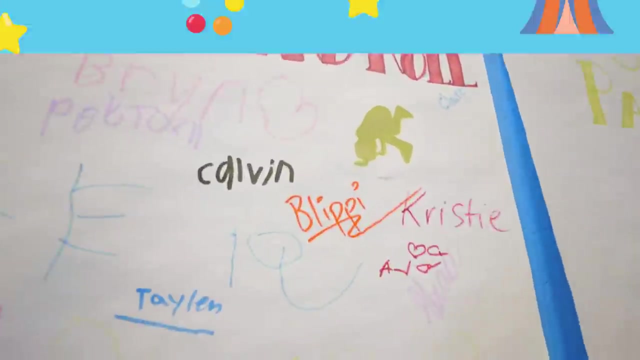 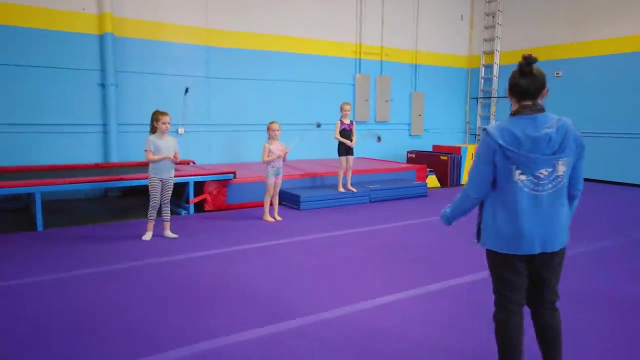 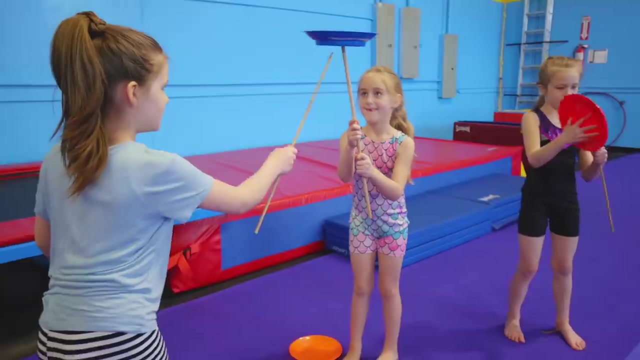 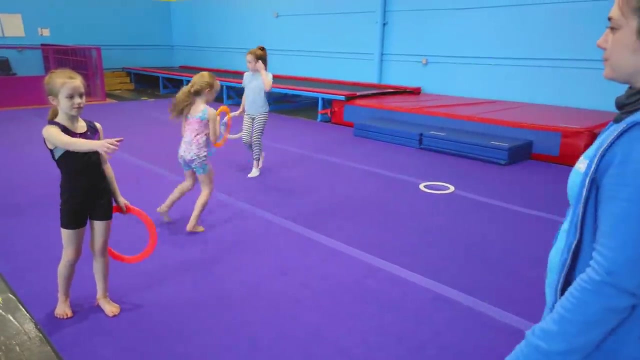 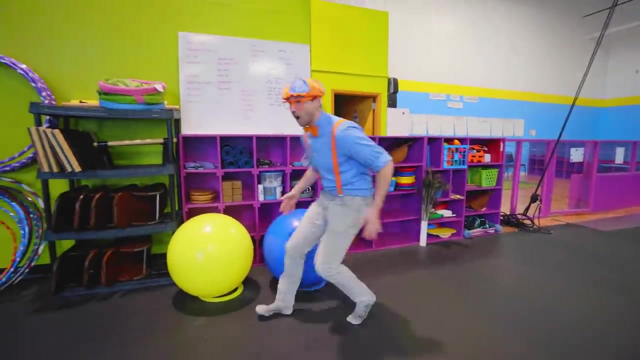 go. Now it's time to write my name: B- L-I- P-P-I Flippy. Wow, That was awesome. Yeah, Whoa, Check out this area. There are so many cool things. Whoa, What are these? 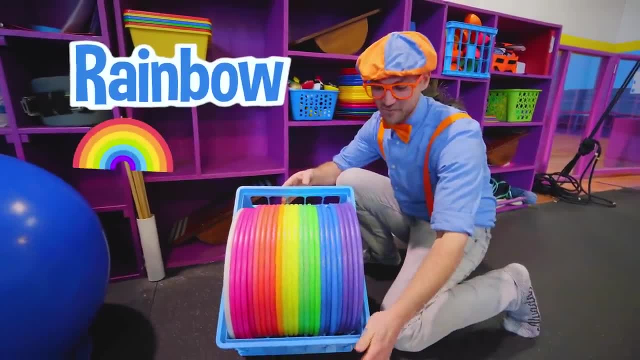 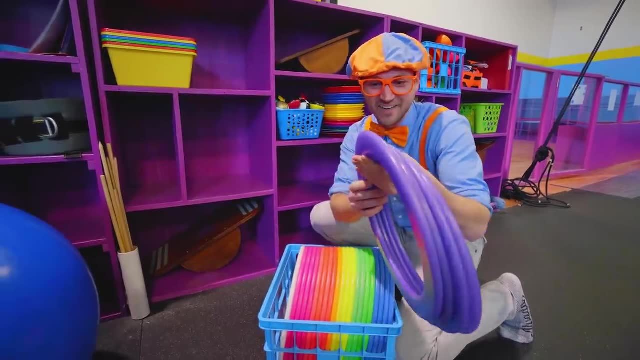 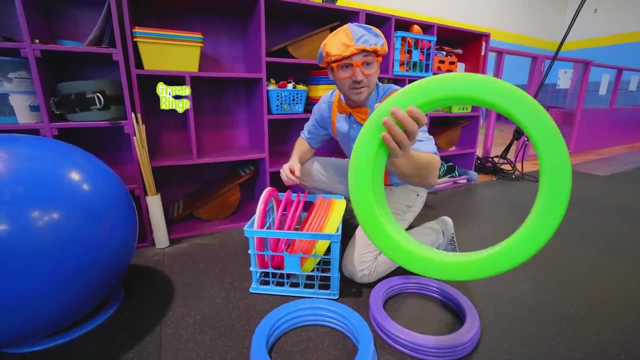 Wow, Kind of looks like a rainbow. Whoa, Yeah, We have some purple, Whoa, Purple rings. Whoa, Check it out. Then we have some blue rings, We have some green rings, We have yellow, We have some. 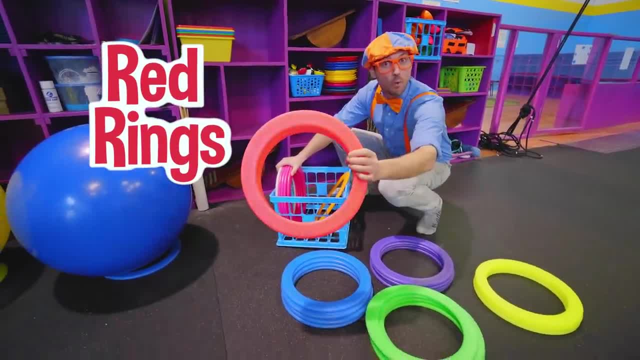 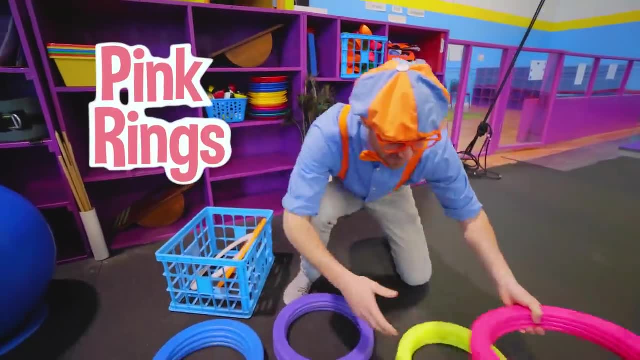 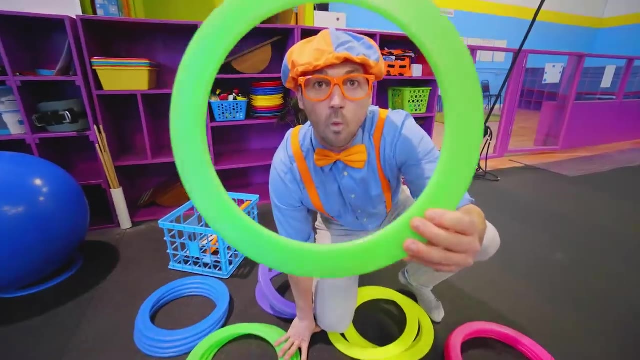 reddish rings. They kind of look orange. Let's just say they're red. And we have some pink rings. Whoa, That is so cool. They're so colorful. Hey, What shape is this? Yeah, A ring is a circle. 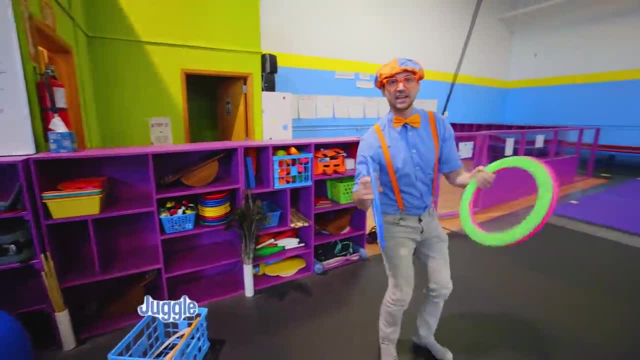 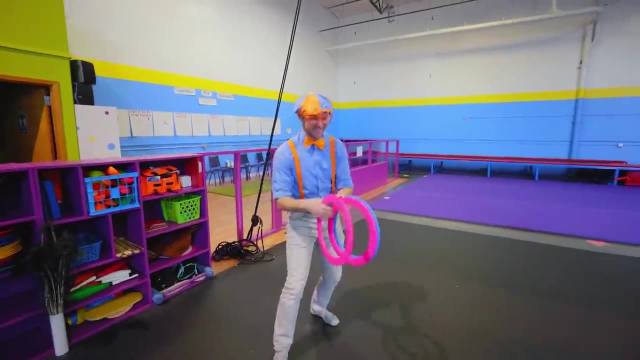 Check it out. Whoa, Maybe I can juggle with these. Here we go. Whoa, Whoa, I dropped one. That's funny. Check it out, You can even spin them on your arm. Whoa, What if I? 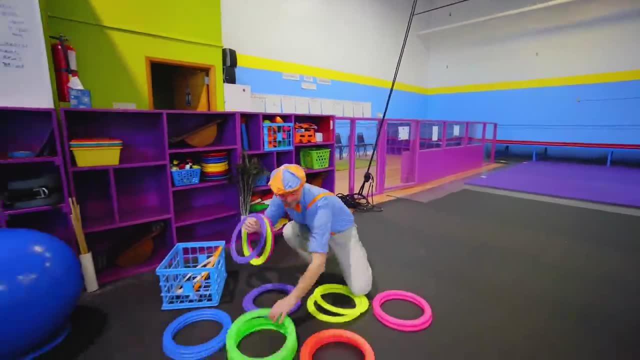 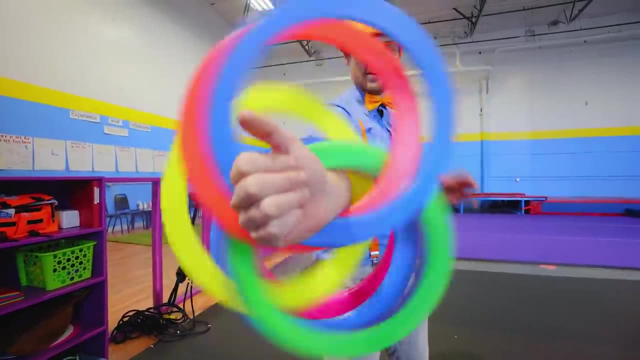 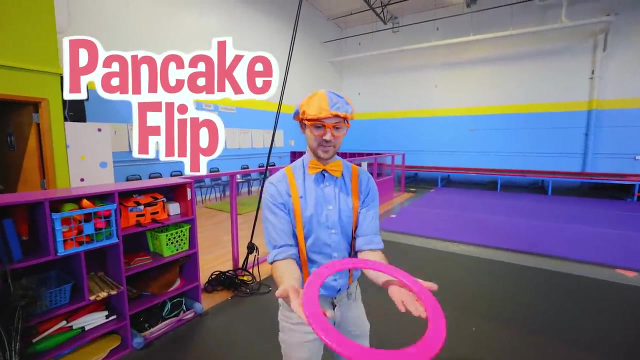 tried that with a lot of them. This is going to look so cool: Ready Whoa, Whoa, Whoa, Whoa. That's fun. Check this out. This is called a pancake flip. You can practice by going like this. 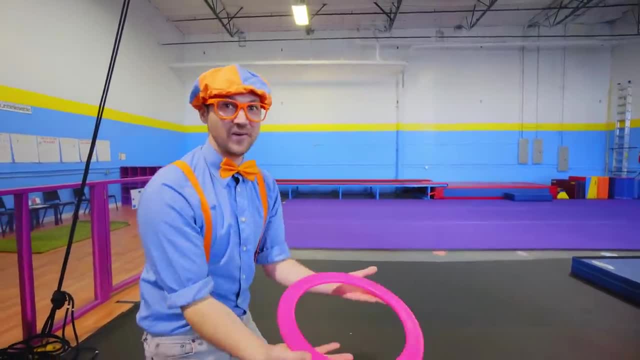 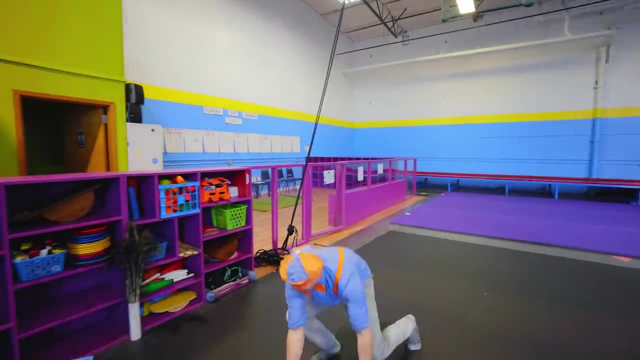 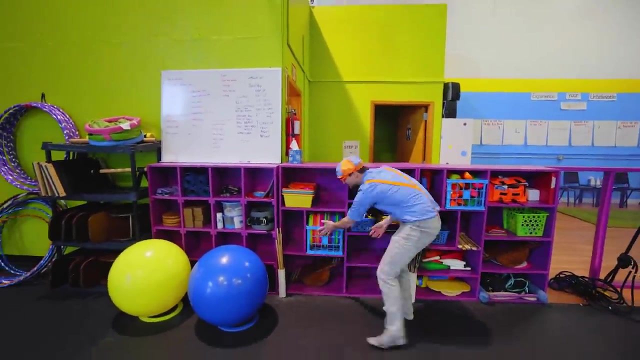 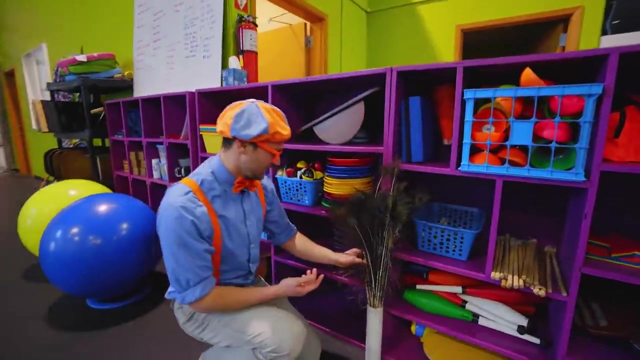 Yeah, Try and make it flip. Watch this, I did it. Okay, Let me put these back. Can't forget this one. Okay, Now that those are organized and put back in their place, maybe we can use other things. Whoa. 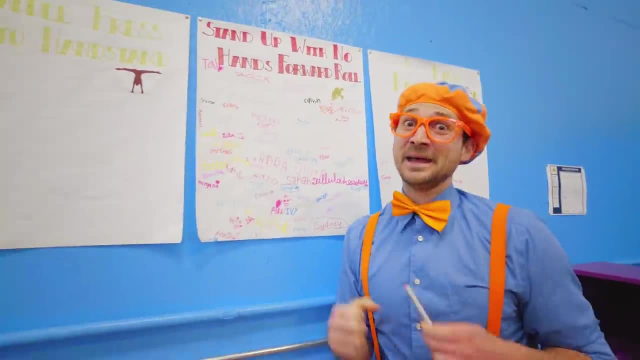 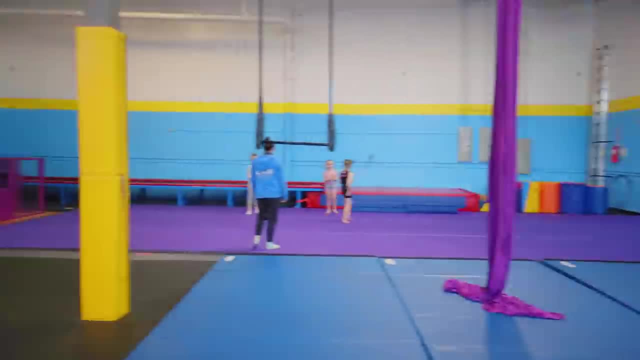 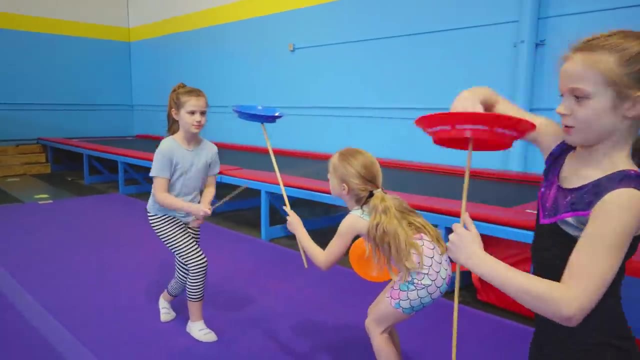 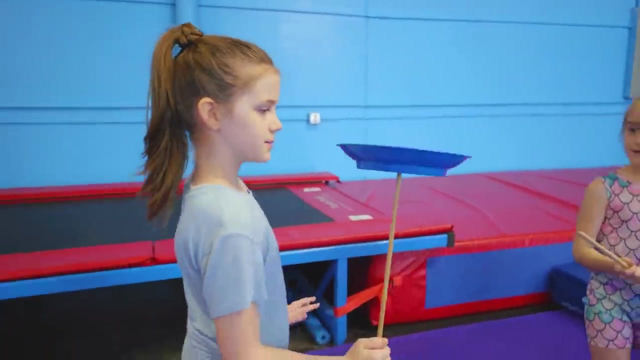 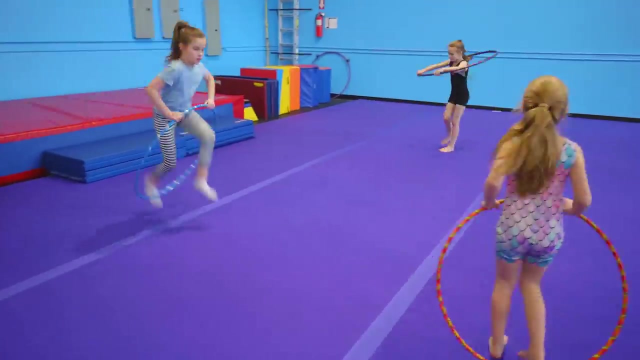 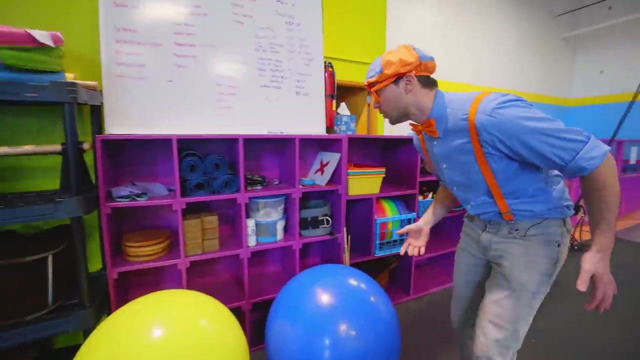 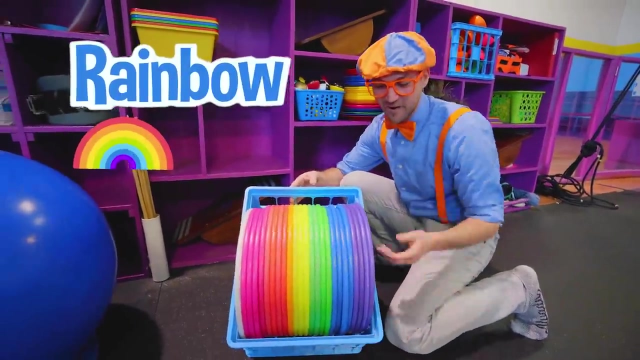 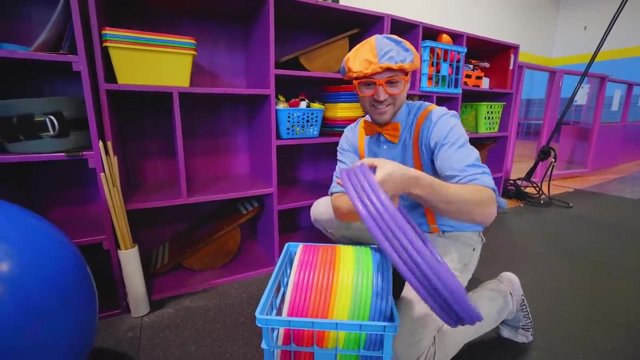 Whoa, check out this area. There are so many cool things. Whoa, what are these? Wow, kind of looks like a rainbow. Whoa, yeah, we have some purple Whoa, purple rings. Whoa, check it out. 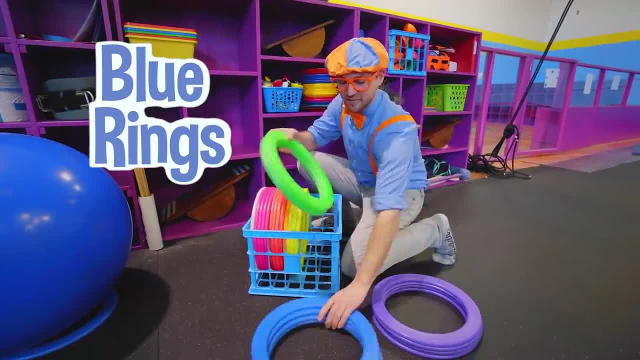 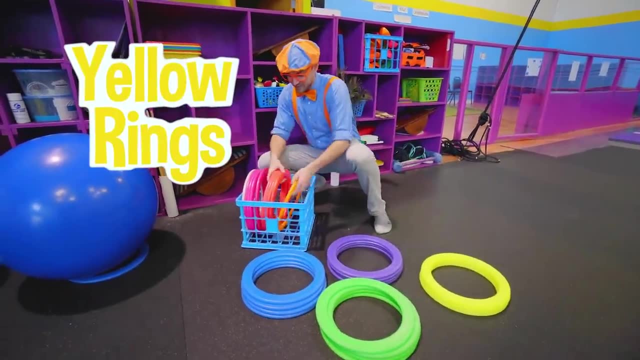 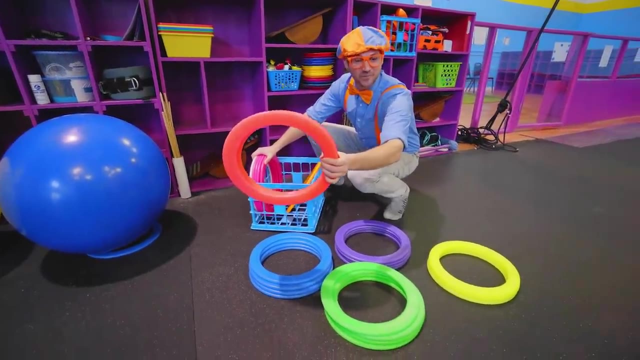 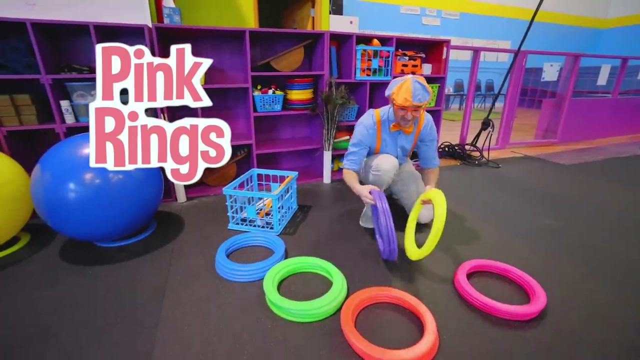 Then we have some blue rings, We have some green rings, We have yellow, We have some red Reddish rings- They kind of look orange, Let's just say they're red. And we have some pink rings. Whoa, that is so cool. 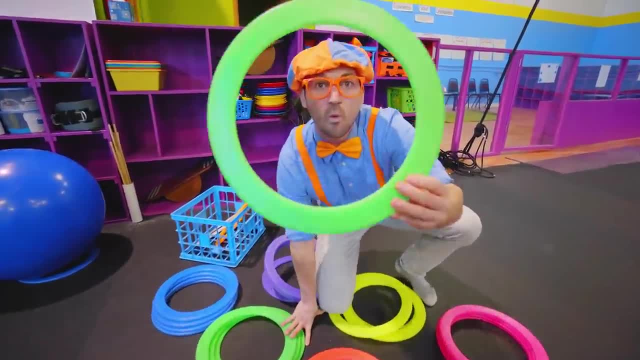 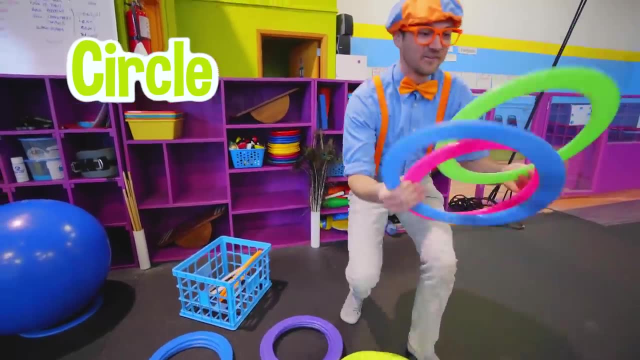 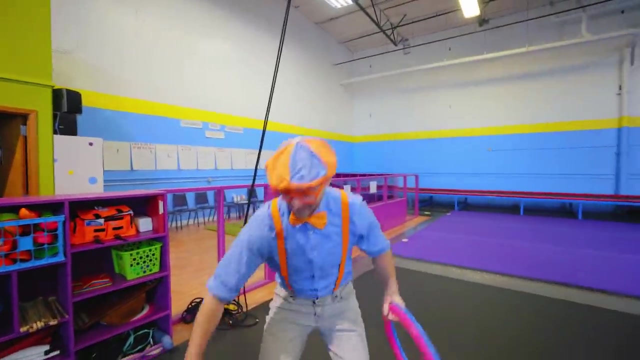 They're so colorful. Hey, what shape is this? Yeah, a ring is a circle. Check it out. Whoa, maybe I can juggle with these. Here we go, Whoa, whoa, I dropped one. That's funny. 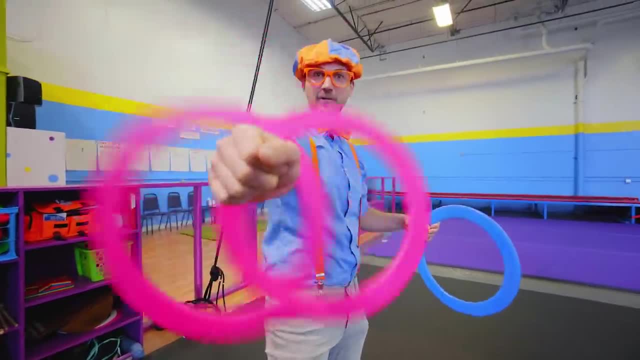 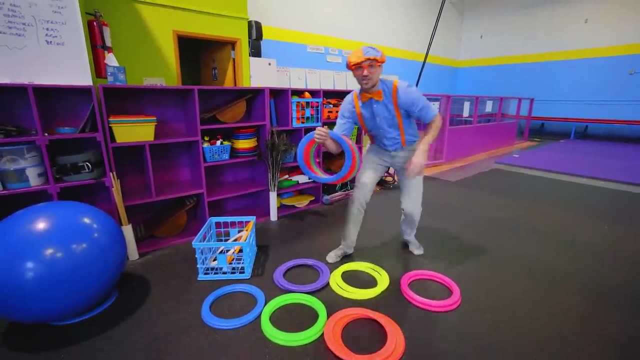 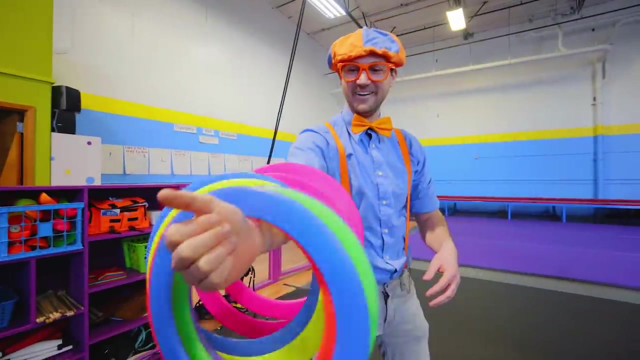 Check it out. You can even spin them on your arm. Whoa, What if I tried that with a lot of them? This is going to look so cool, Ready. Whoa, whoa, Whoa, Whoa, That's fun. 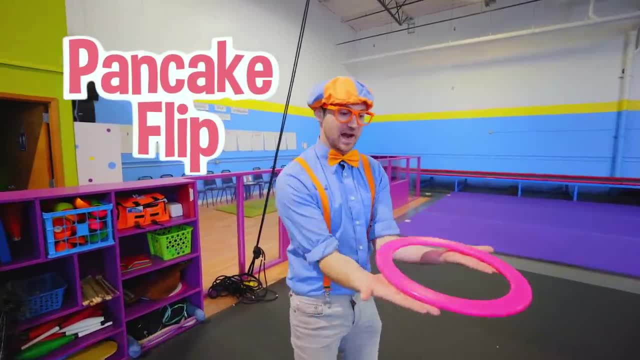 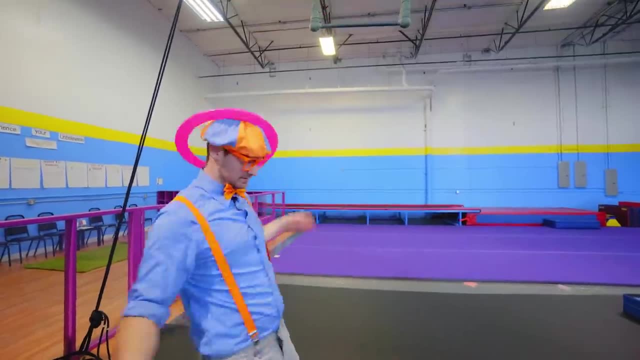 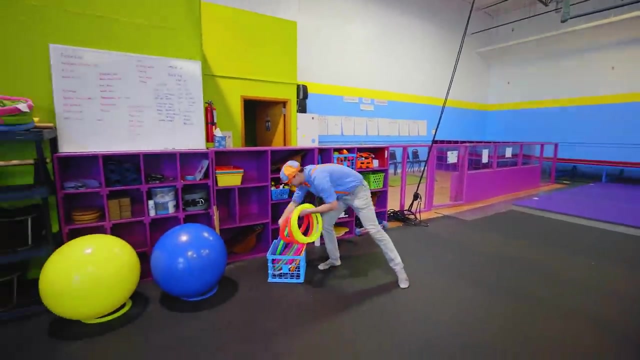 Check this out. This is called a pancake flip. You can practice by going like this: Yeah, Try and make it flip And watch this. Yeah, I did it. Okay, let me put these back. Can't forget this one. 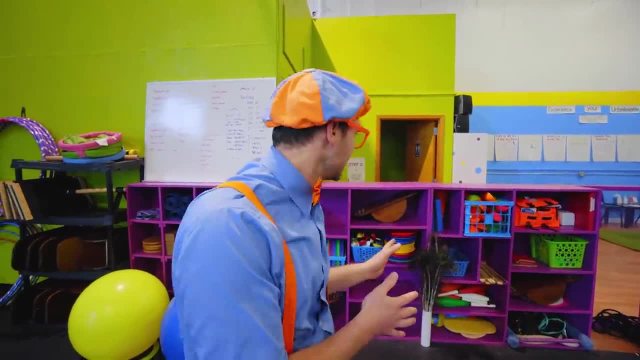 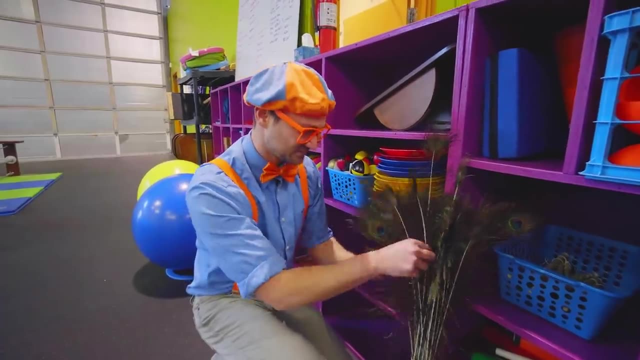 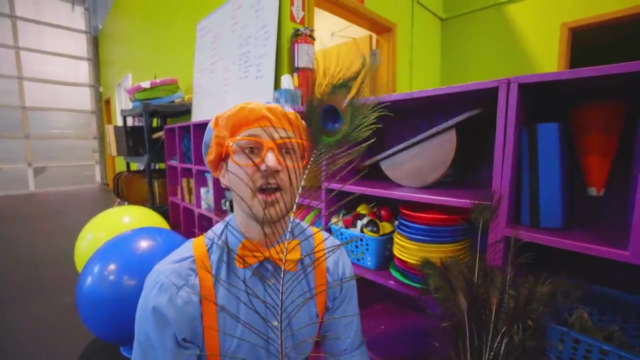 Okay, now that those are organized and put back in their place, maybe we can use other things. Whoa like this: This looks like a peacock feather. Whoa, Wow, Peacocks are so pretty. Have you ever seen a peacock before? 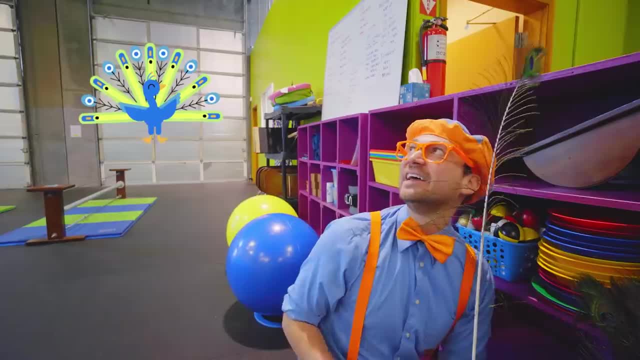 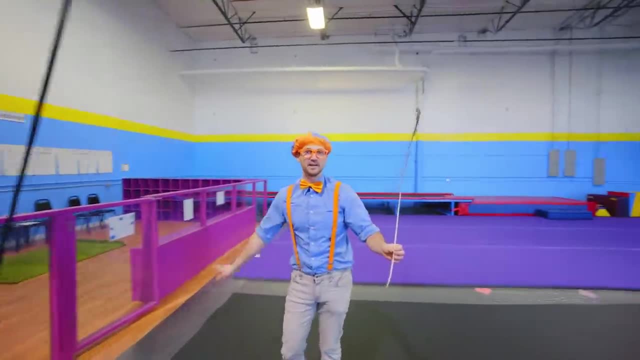 Wow, Yeah, They can spread their wings out and it looks so graceful. But today, what I'm going to do is I'm going to take this peacock feather and try and balance it. Okay, put it on my finger, Whoa. 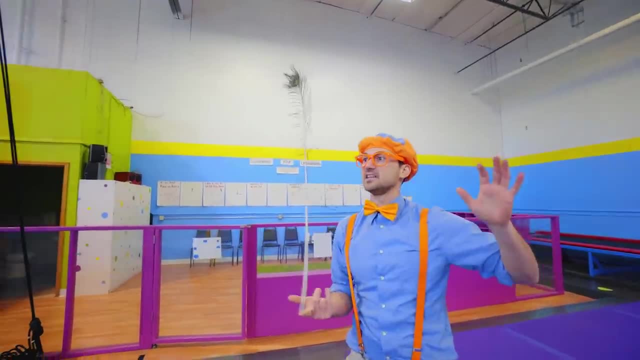 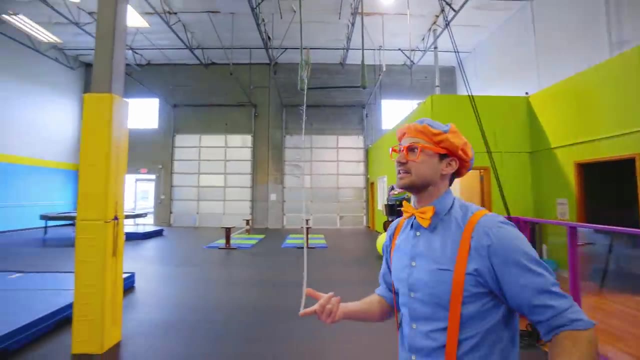 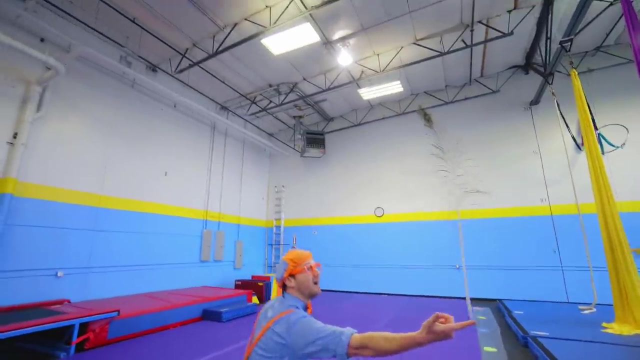 Check it out. Yeah, I'm balancing it. I'm trying not to drop it. I'm balancing it on the ground. Whoa, You can do it by standing in the same area, or maybe I can do it while moving. Whoa, whoa, this is hard. 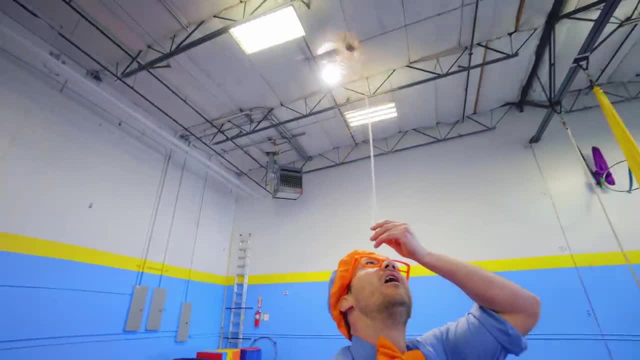 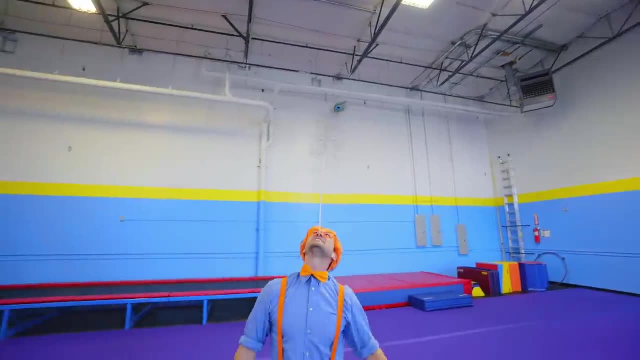 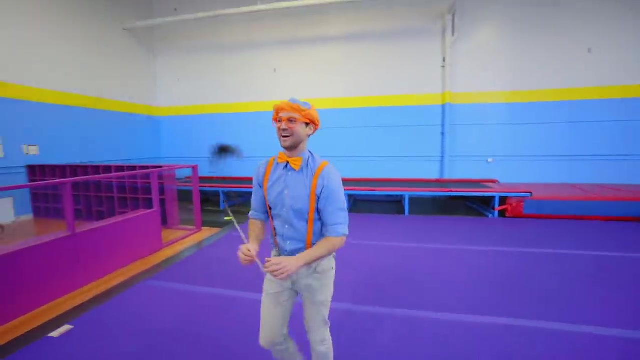 Whoa, Check this out Ready. Let's try and put it on my nose. Whoa, Whoa, I'm balancing it. Whoa, Whoa, Whoa, Whoa, Whoa, Whoa, That's so silly. 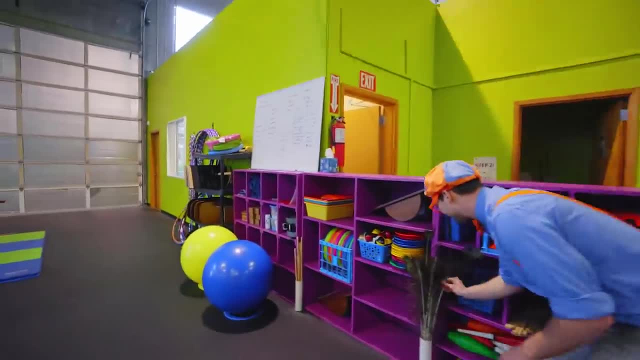 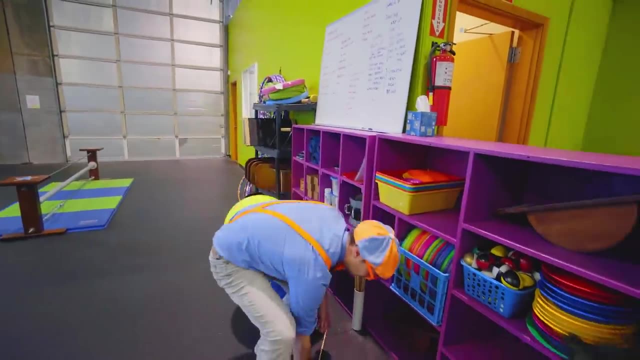 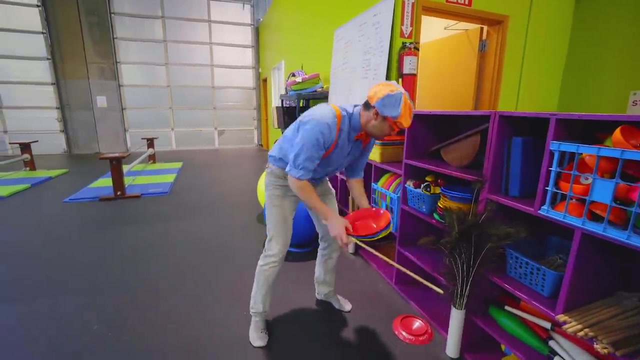 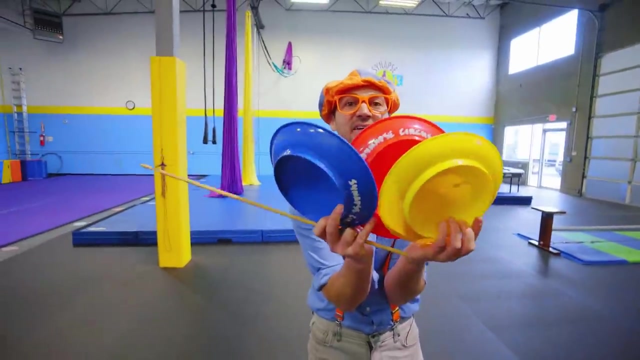 Wow, Balancing is so much fun. What else do we have here? Oh, it looks like we have some, oh, some rods and we have some plates. How many plates did I grab? Yeah, One, two, three. 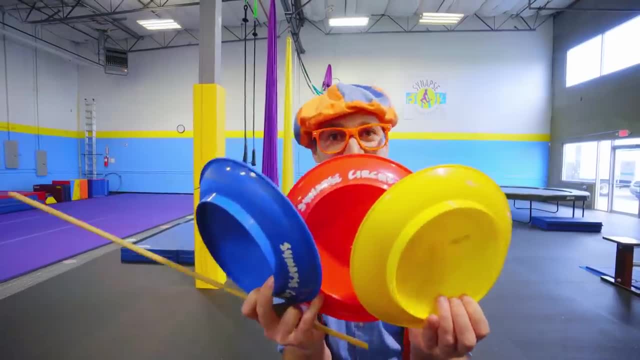 Oh, there's a lot: One, two, three plates. And what colors are these? Yeah, Blue, red, yeah, and yellow. Okay, let's take the blue one, which is one of my two favorite colors, and give it some. 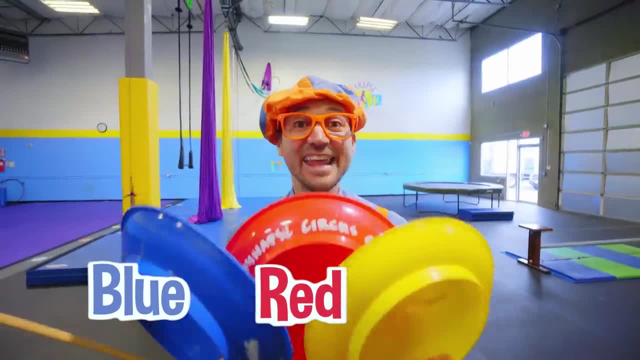 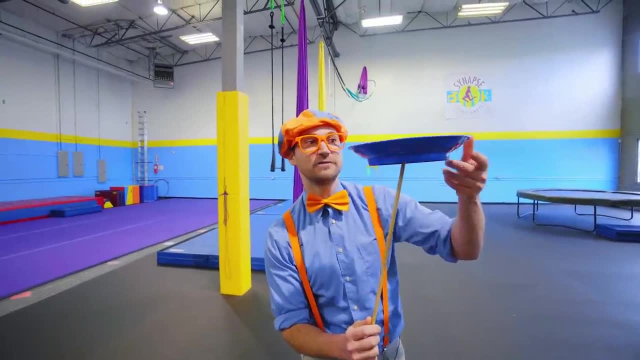 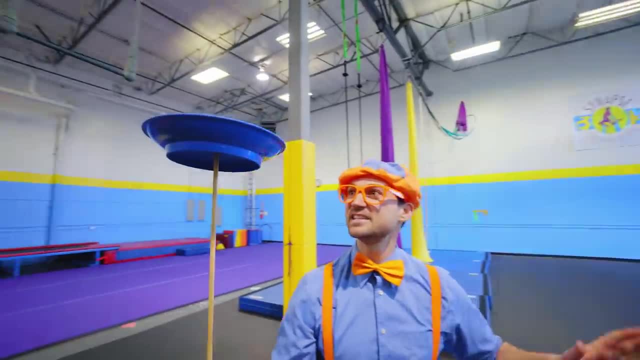 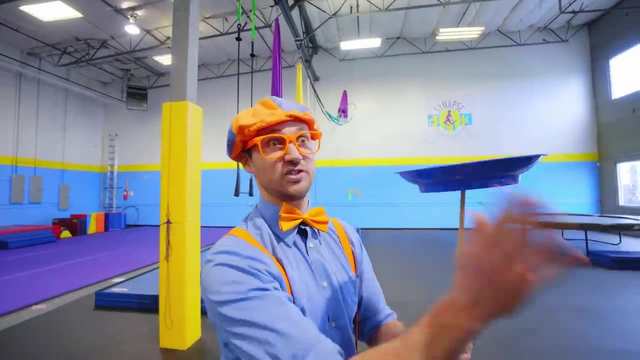 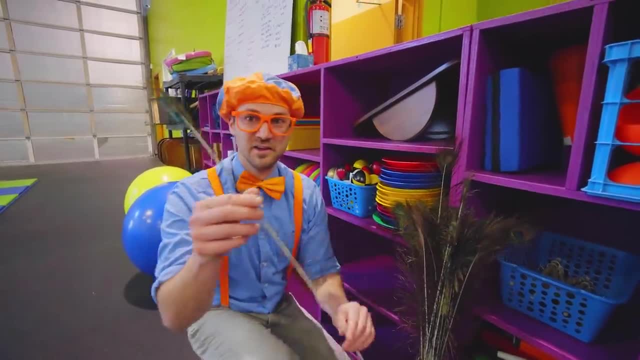 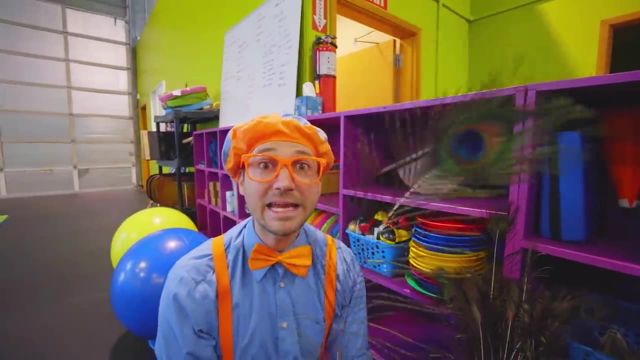 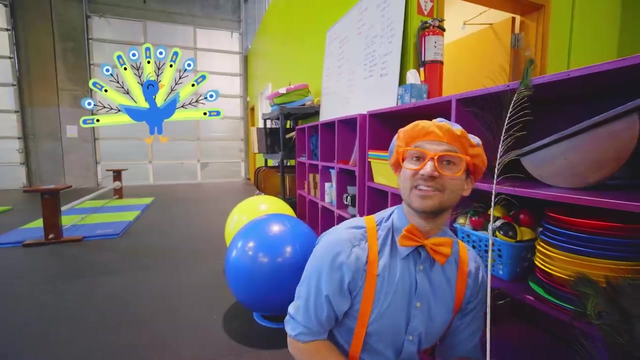 Like this. This looks like a peacock feather- Wow, Peacocks are so pretty. Have you ever seen a peacock before? Wow, Yeah, They can spread their wings out and it looks so graceful. But today, what I'm going to do is I'm going to 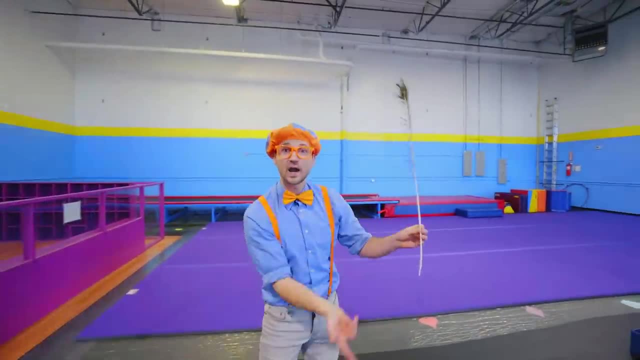 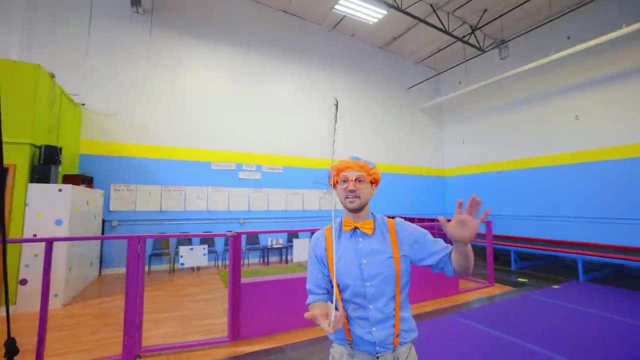 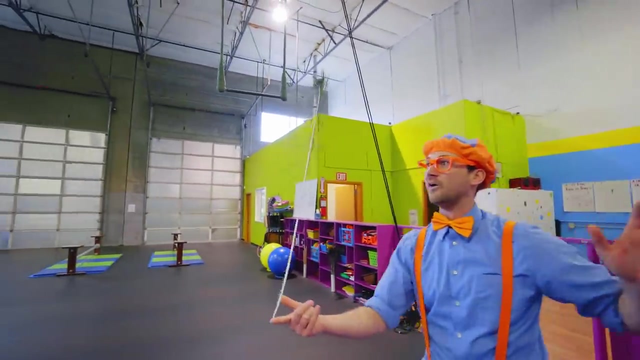 take this peacock feather and try and balance it. Okay, Put it on my finger, Whoa, Check it out. Yeah, I'm balancing it. I'm trying not to drop it on the ground, Whoa, And you can do it by standing in the same. 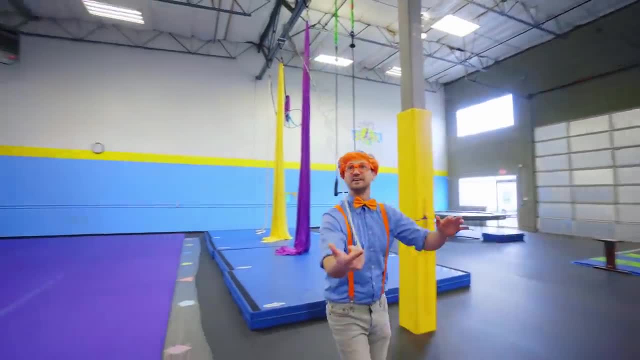 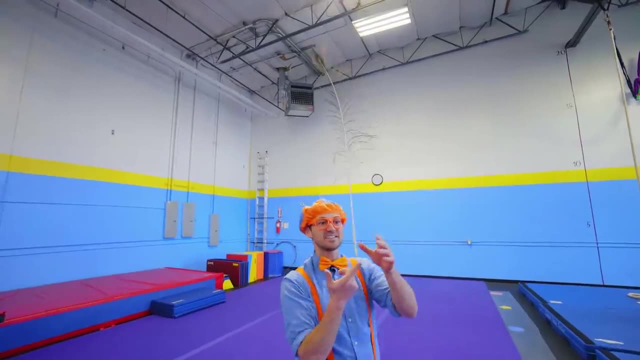 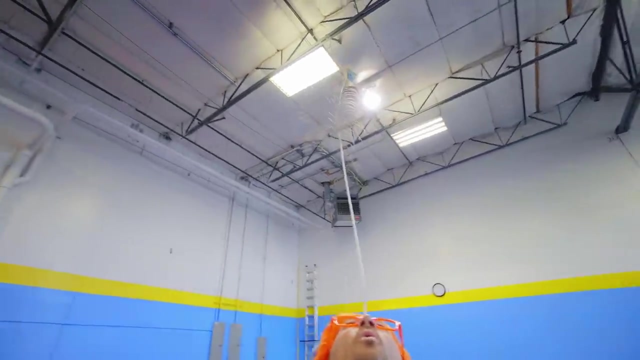 area, or maybe I can do it while moving. Whoa, Whoa, This is hard. Whoa, Check this out Ready, Try and put it on my nose. Whoa, Whoa, I'm balancing it, Whoa. 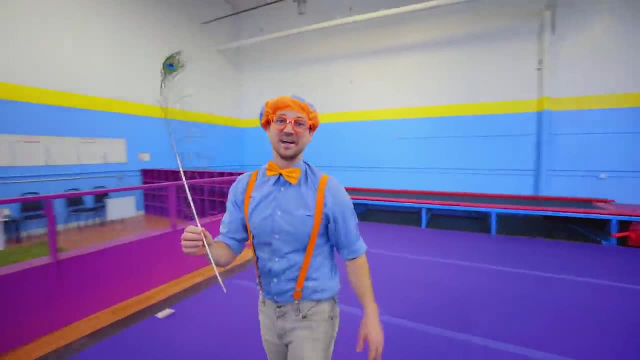 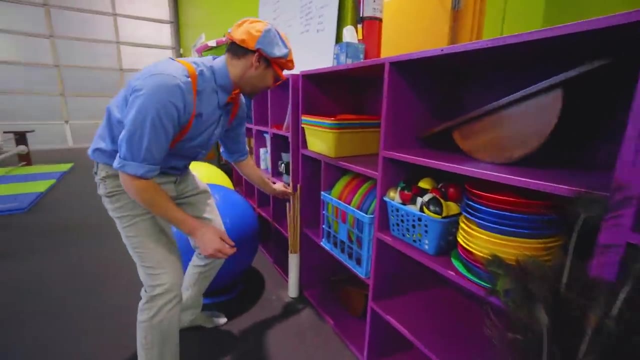 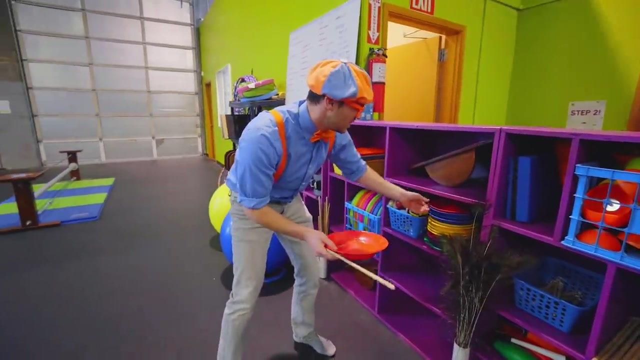 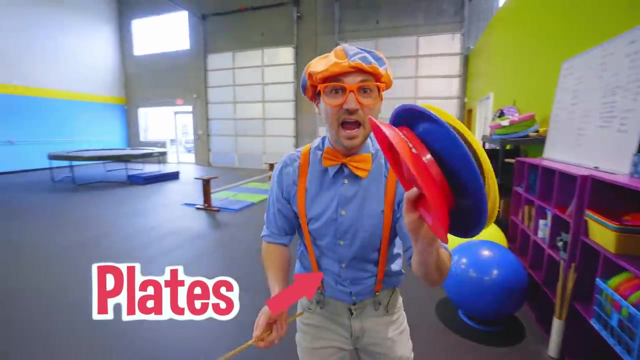 That's so silly, While balancing, it's so much fun. What else do we have here? Oh, it looks like we have some, oh, some rods and we have some plates. How many plates did I grab? Yeah, One, two. 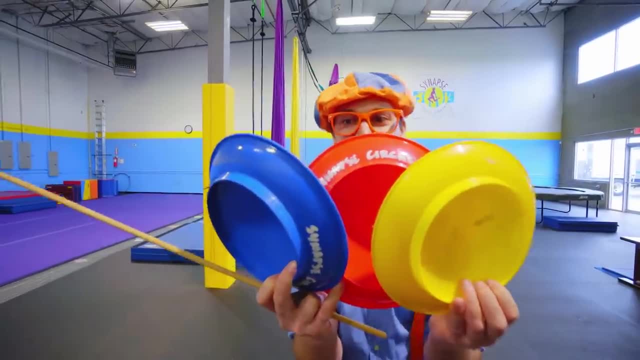 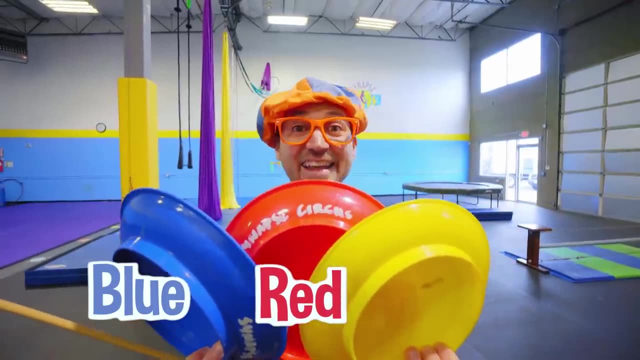 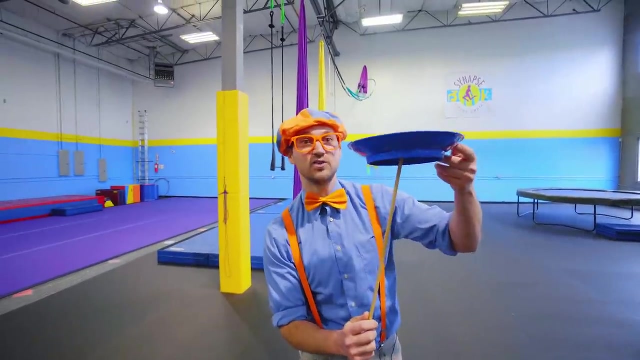 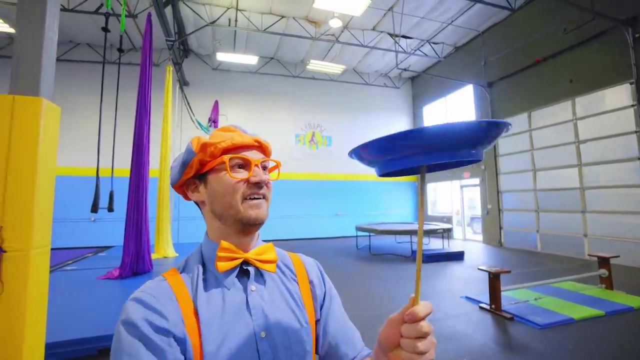 three plates. And what colors are these? Yeah, Blue, Red. Yeah, And yellow. Okay, Let's take the blue one, which is one of my two favorite colors, and give it some spin. Whoa, There we go, Yeah. 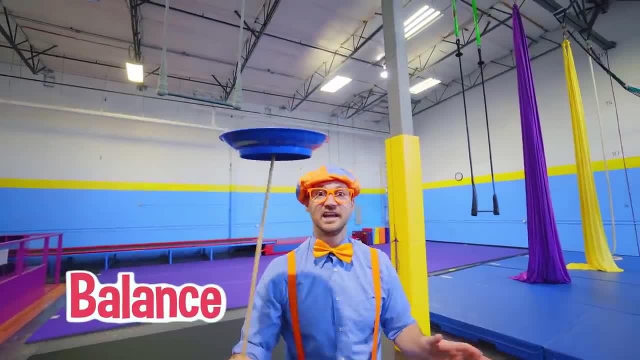 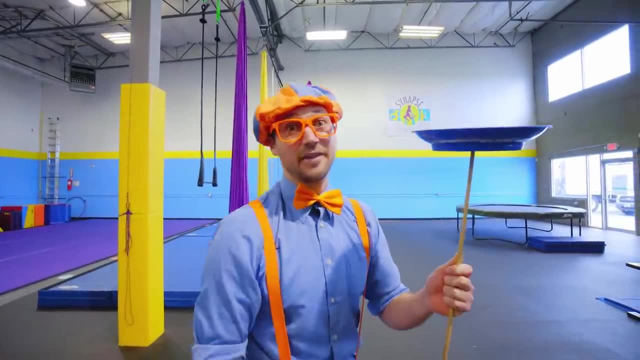 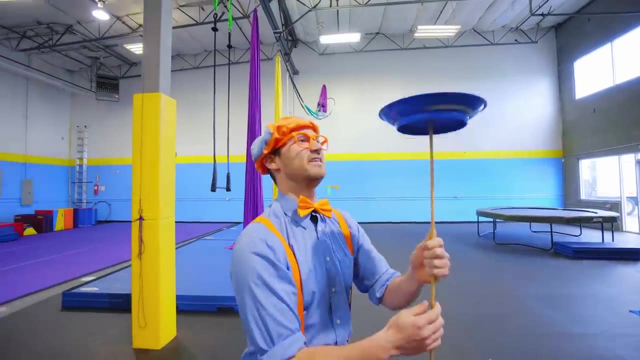 You see it spinning and balancing. Yeah Well, hey, These plates are plastic. You definitely shouldn't try this at home with your plates at home. If they fall, they'll break. Whoa, Yeah, These are circus plates. Spin, spin, spin Ready. 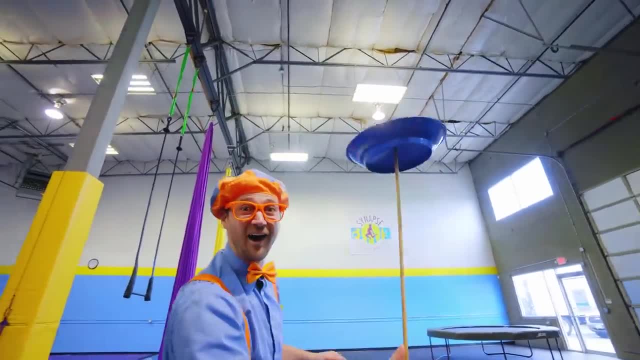 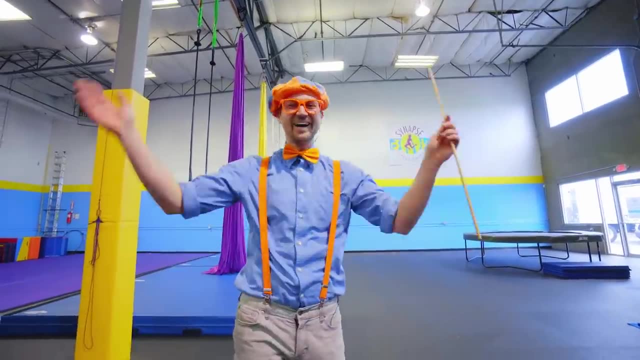 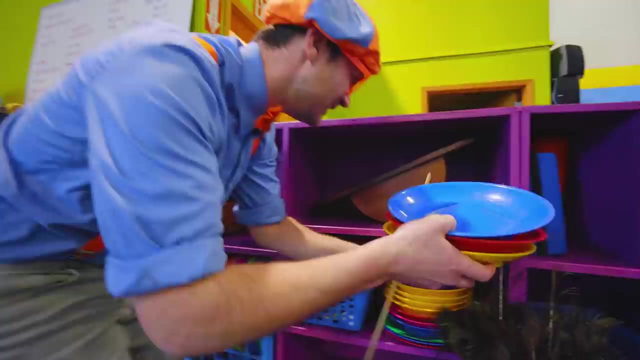 Whoa, I'll try that again. Whoa, Did you see that? Here we go. Oh, Whoa. Okay, I won't try it again. Okay, Let me put these back and see what else we have. Wow. 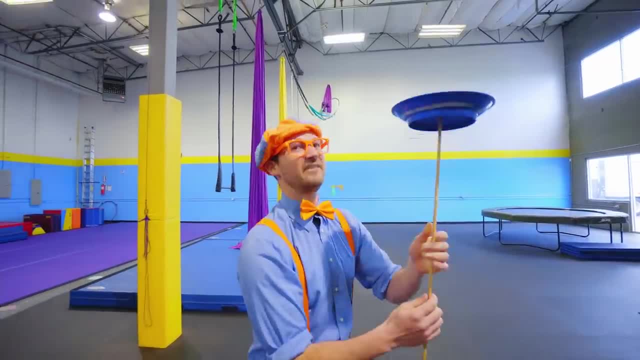 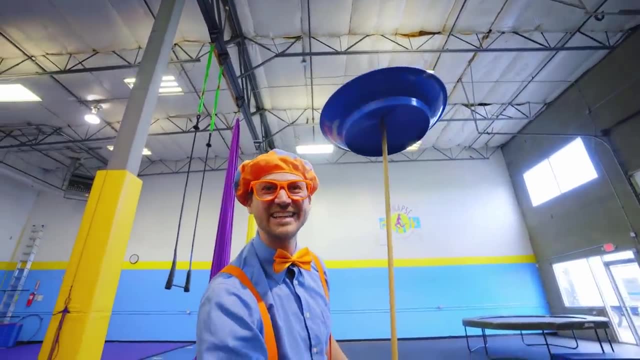 Good, good, good good. That's really cool. Oh, and they are giant. Wow, They're huge. Look at that. Whoa, Whoa. That's great. We can put them on this right here, Okay. 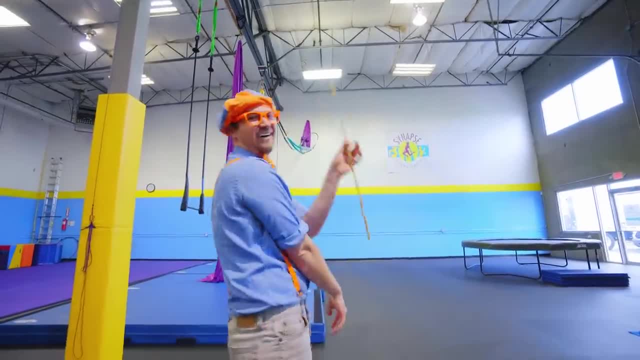 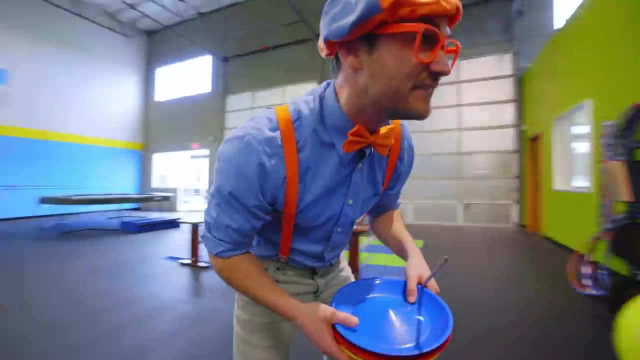 Hopefully this one will break if they fall. Yeah Well, hey, these plates are plastic. You definitely shouldn't try this at home with your plates at home. If they fall, they'll break. I won't try it again. Okay, let me put these back and see what else we have. 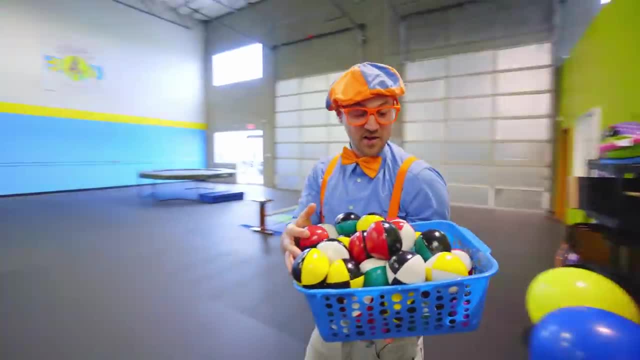 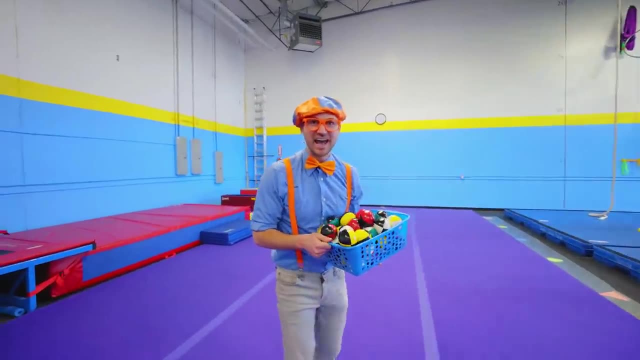 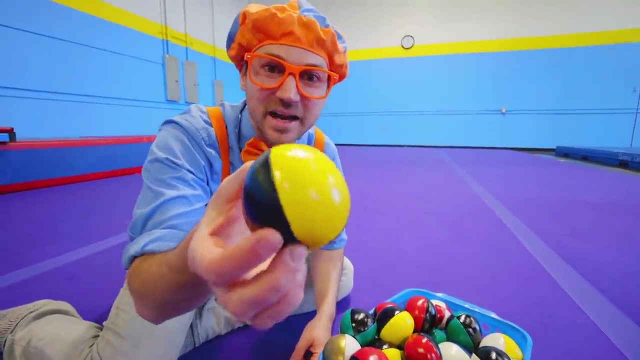 Wow, Check these out. So many juggling balls. Yeah, you know me. I sure do like juggling, don't I? Yeah, Okay, oh, they're so colorful. Check it out That one reminds me of a bee. 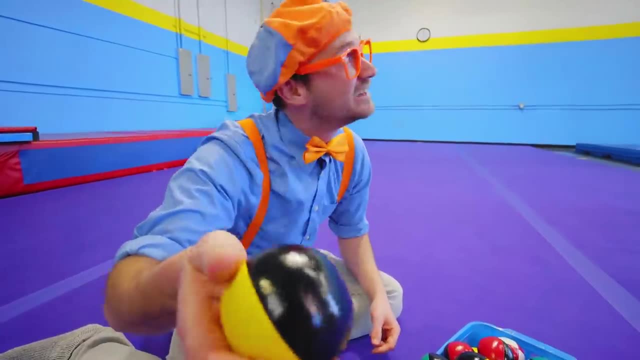 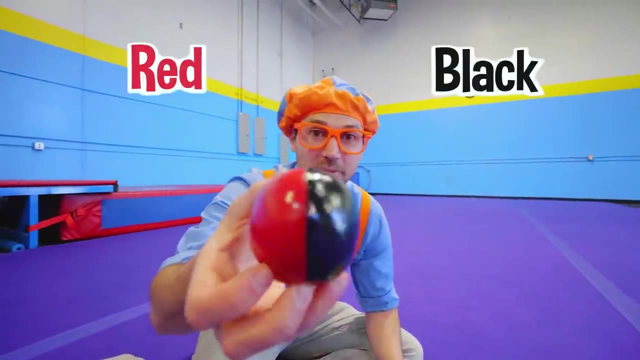 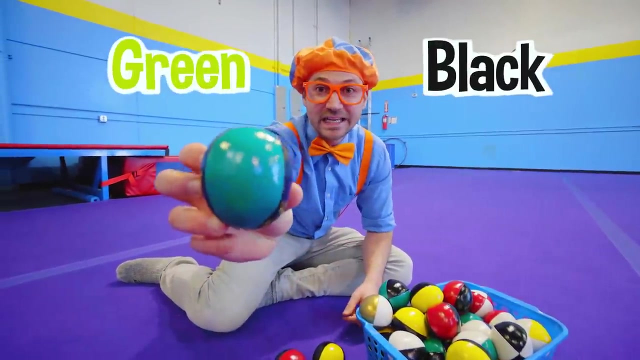 Yeah, bees are so great because they make honey. Yum, I love honey. Okay, looks like this is red and black and blue and white, green and black. Okay, I'm gonna pick three of these. How about these three? 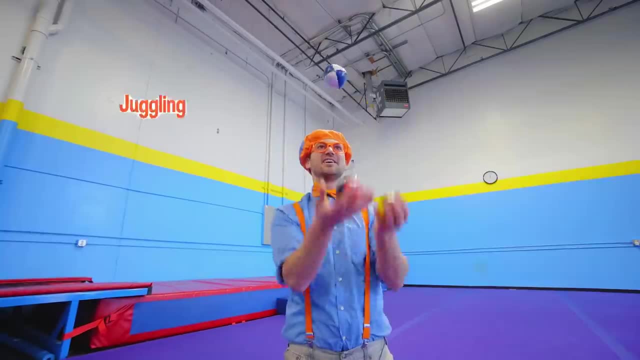 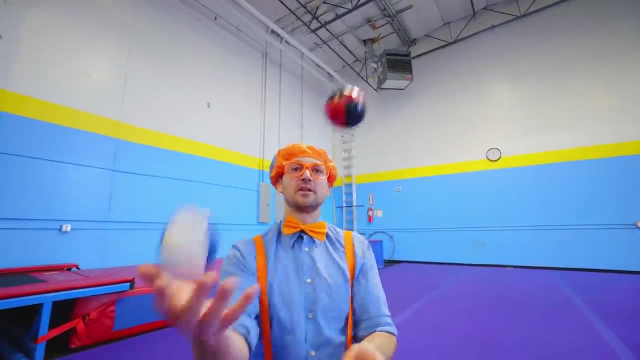 All right, ready, Start on my knees and start to juggle. Whoa. Oh, juggling is so much fun. It's pretty tricky though. Whoa, whoa, whoa, But with a lot of practice you can do a lot of cool things. 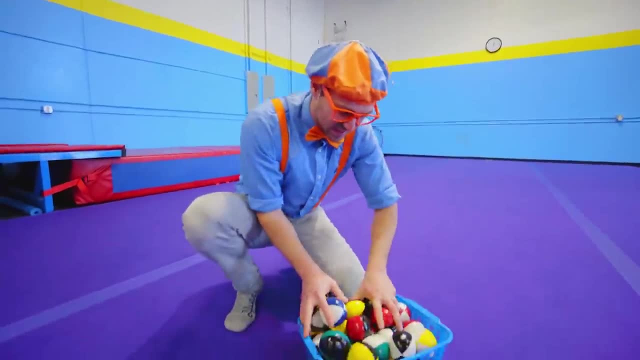 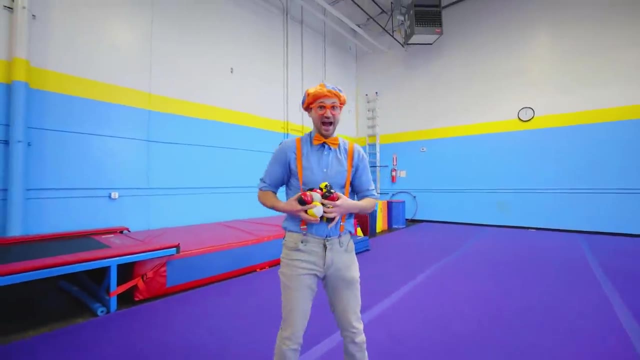 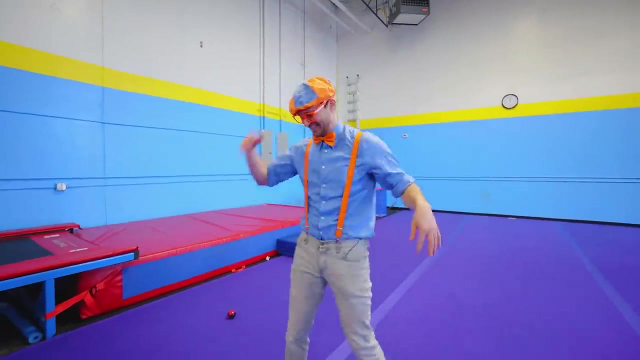 Ha ha, yeah, All right, now watch this. I'm gonna juggle this menu Ready. Okay, this is gonna be really tricky. Here we go. Oh, that was so silly. All right, I should probably pick these up. 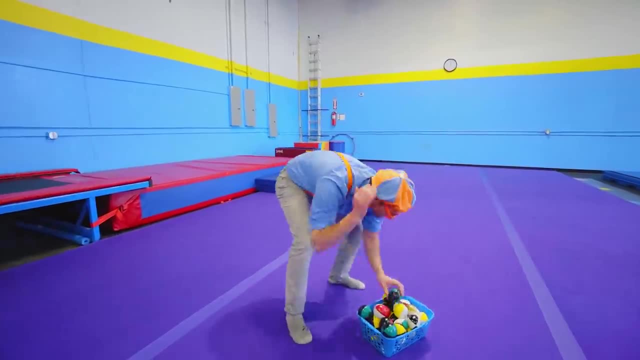 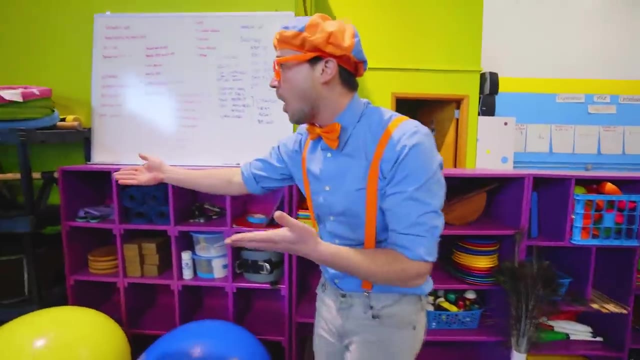 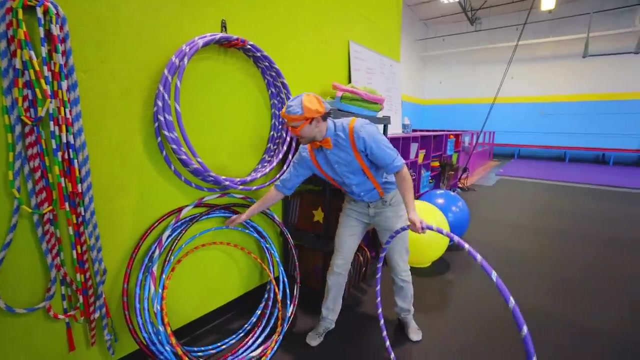 Here they are. I think I got some of these. Hmm, let's see. All right, let's see All right, let's see what else is over here. Whoa, check it out. Hula hoops- Yeah, I love hula hoops. 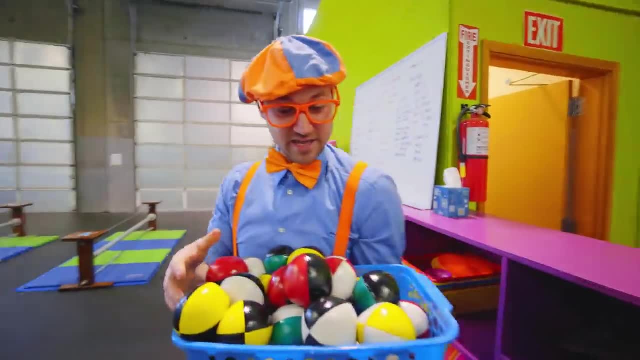 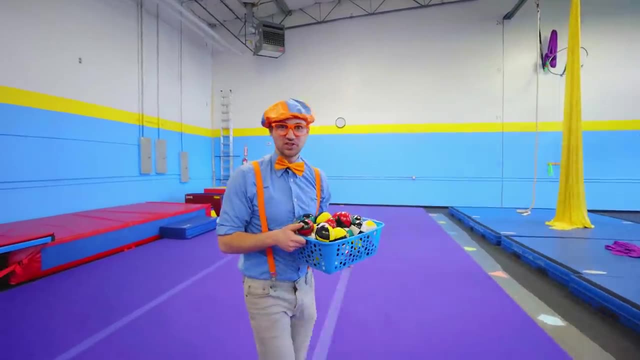 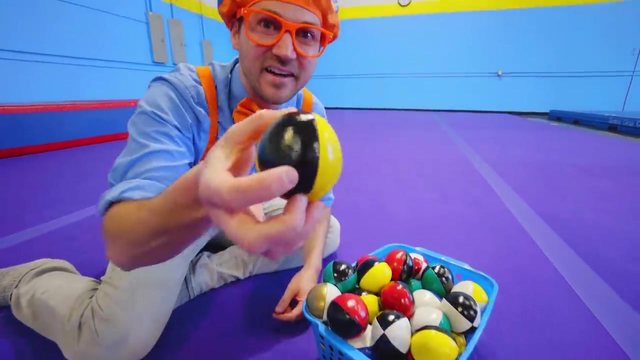 Wow, Check these out. So many juggling balls. Yeah, You know me. I sure do like juggling, don't I? Yeah, Okay, Oh, They're so colorful, Check it out That one reminds me of a bee. 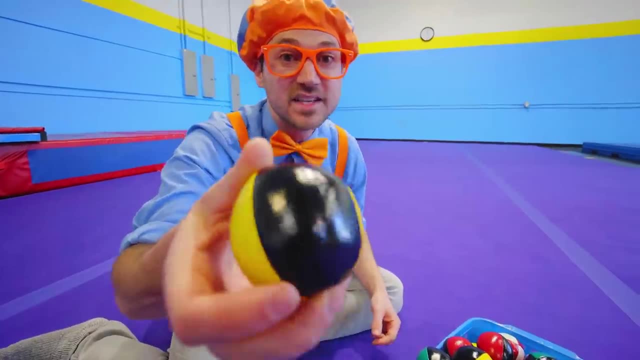 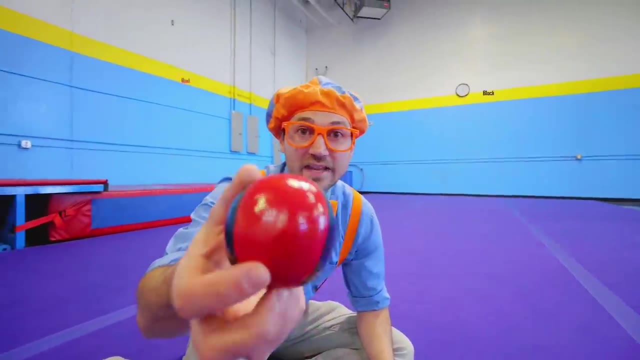 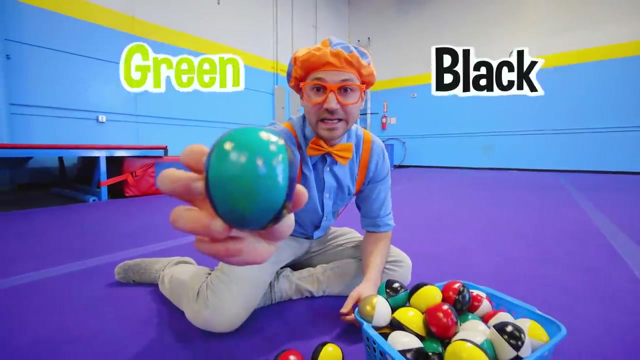 Yeah, Bees are so great because they make honey. Yum, I love honey. Okay, Looks like this is red and black and blue and white, green and black. Okay, I'm going to pick three of these. How about these? 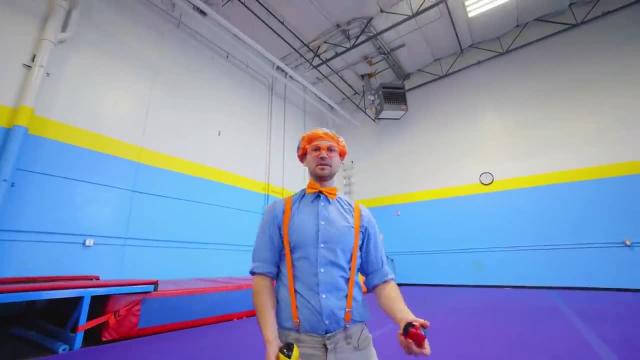 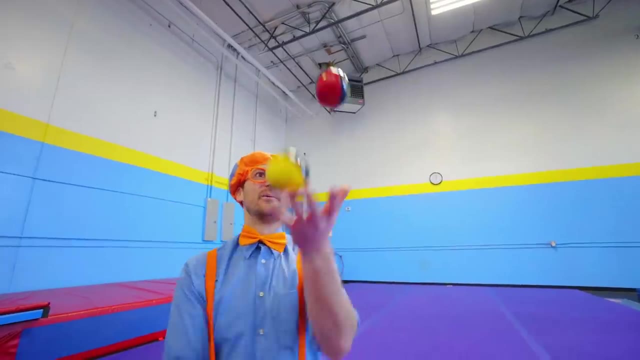 three. All right, Ready. I'm going to start on my knees and start to juggle. Whoa, Juggling is so much fun. It's pretty tricky though. Whoa, Whoa, Whoa, But with a lot of practice you can do. 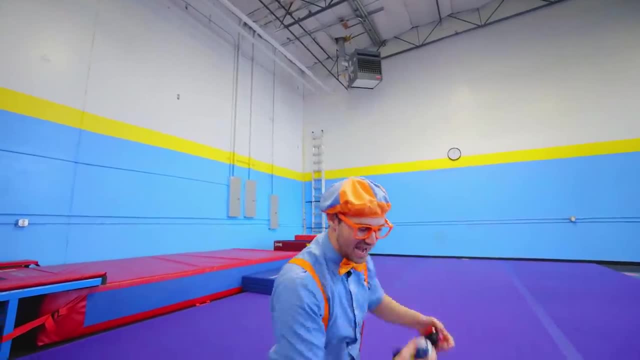 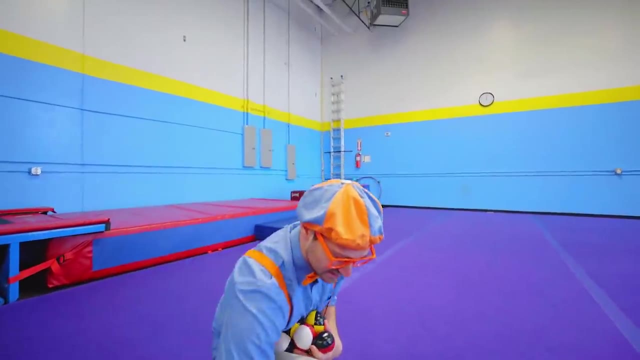 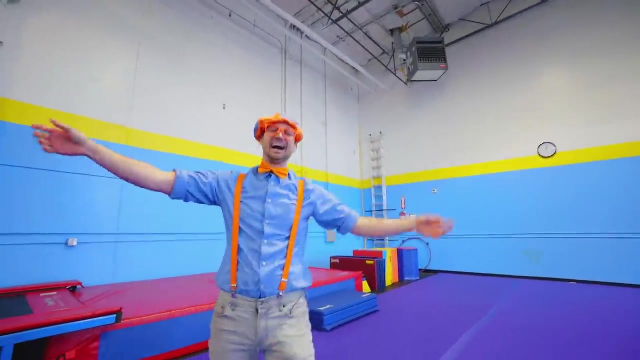 a lot of cool things. Yeah, All right, Now watch this. I'm going to juggle this menu Ready. Okay, This is going to be really tricky. Here we go. That was so silly. All right, I should probably pick these up. 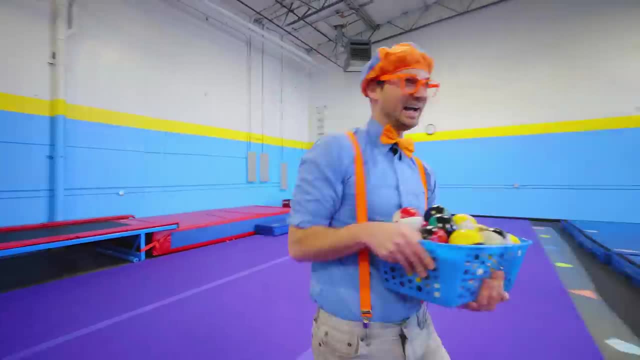 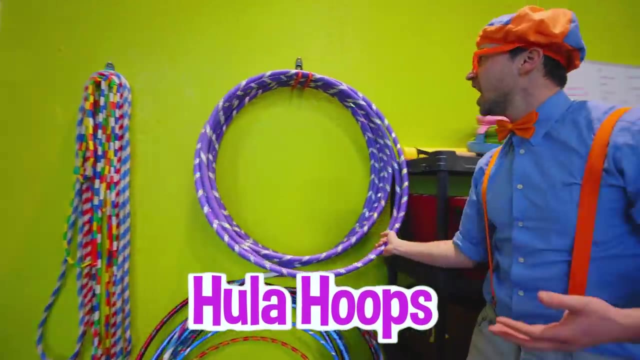 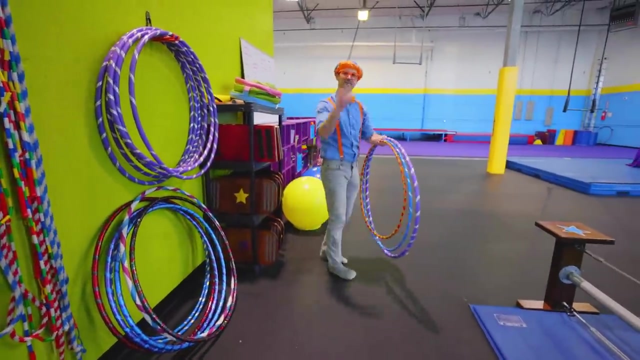 All right, Let's see what else is over here. Whoa, Whoa, Check it out. Hula hoops: Yeah, I love hula hoops. Yeah, Let's grab a few of these. All right, Come on over here. Wow. 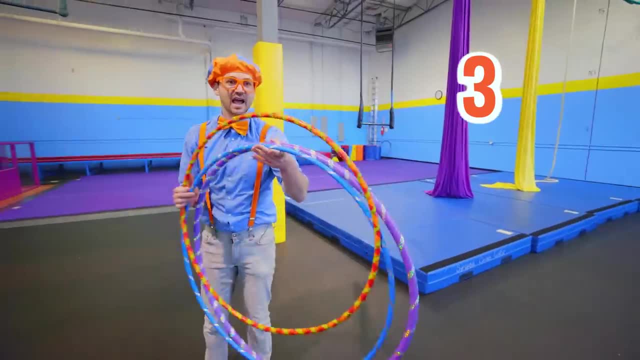 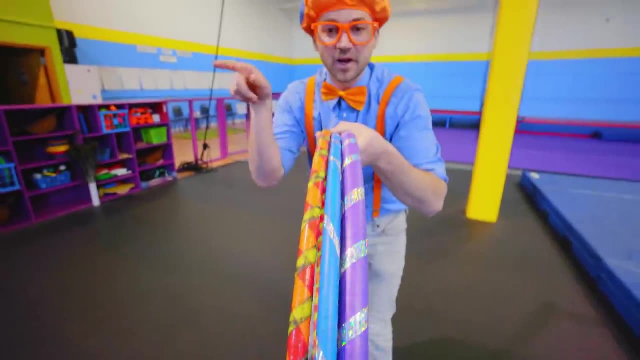 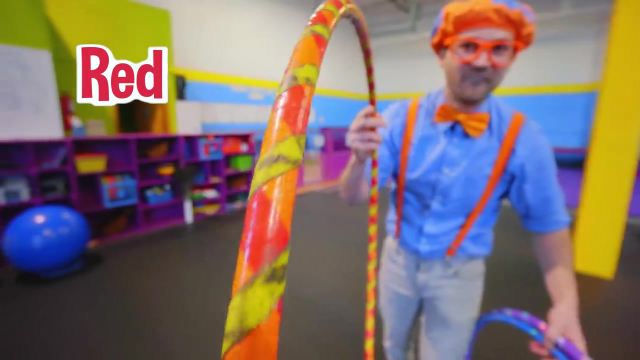 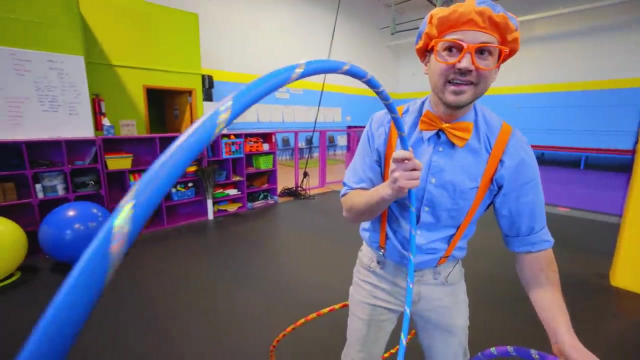 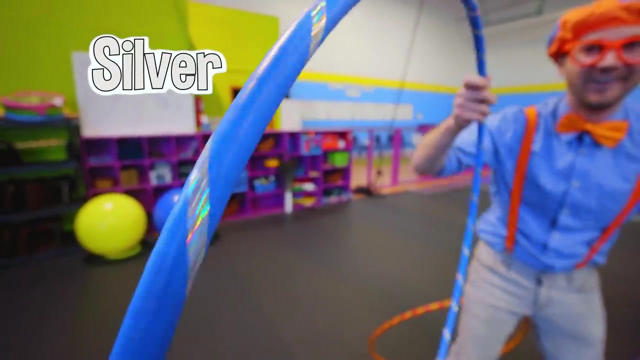 I grabbed three hula hoops. Yeah, What colors are these hula hoops? Yeah, This one is orange, Yellow, Red. Wow, What a cool hula hoop. And this one, yeah, is blue and shiny silver, Whoa. 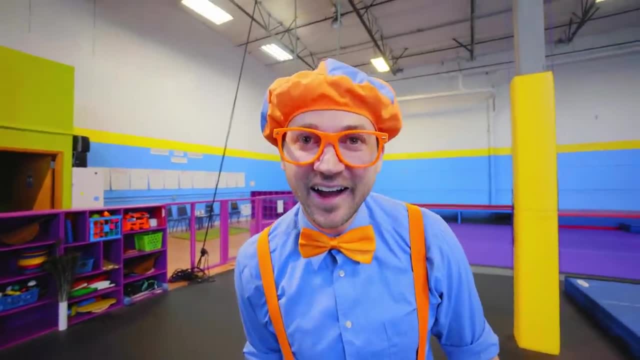 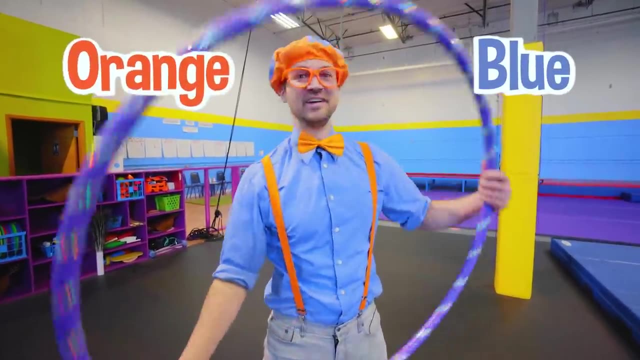 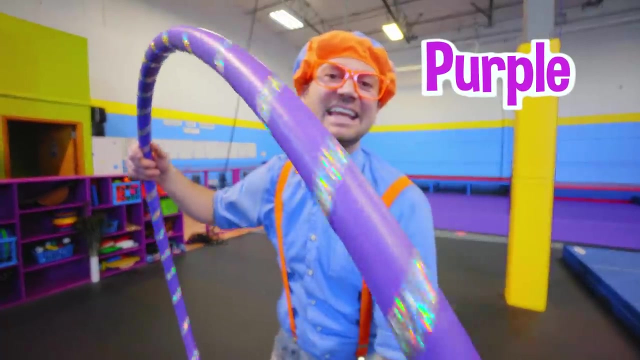 Hey, What's your favorite color? Wow, That's a great color. My two favorite colors are blue and orange, And this one, yeah, is the color purple And the shiny silver sparkle. Yeah, Let's use this one. All right, I'm going to first try and. 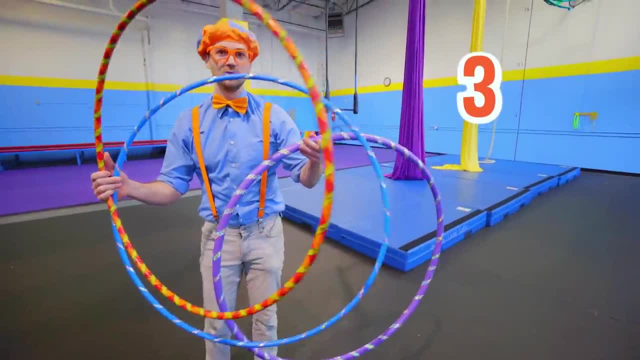 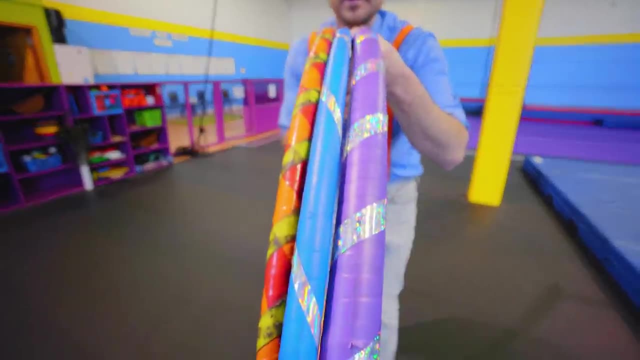 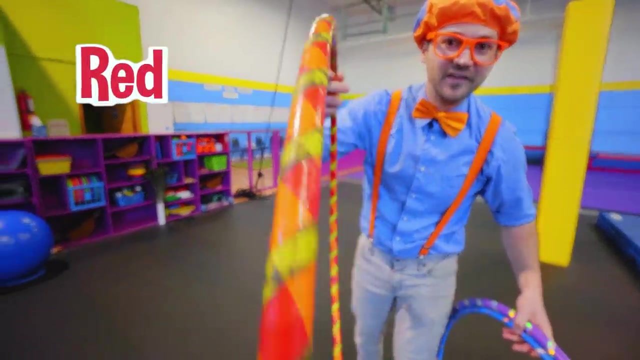 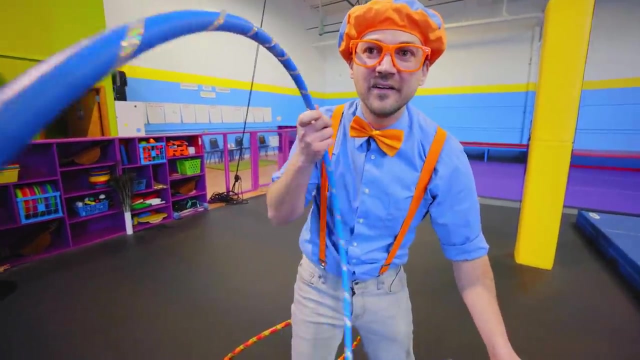 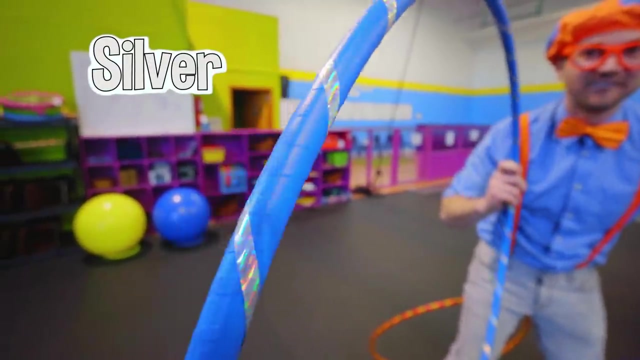 Yeah, Let's grab a few of these. All right, come on over here. Wow, are these hula hoops? Yeah, This one is orange, yellow and red. Wow, What a cool hula hoop. And this one, yeah, is blue and shiny silver, Whoa, Hey, what's your favorite color? 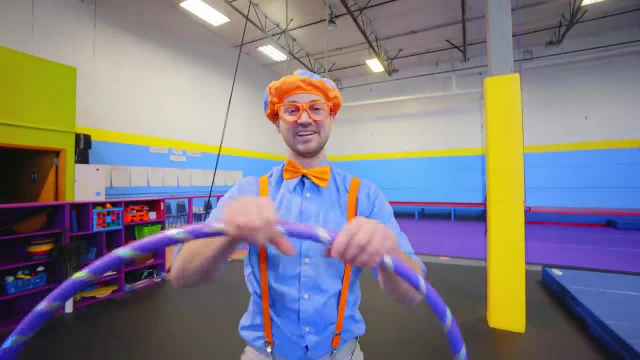 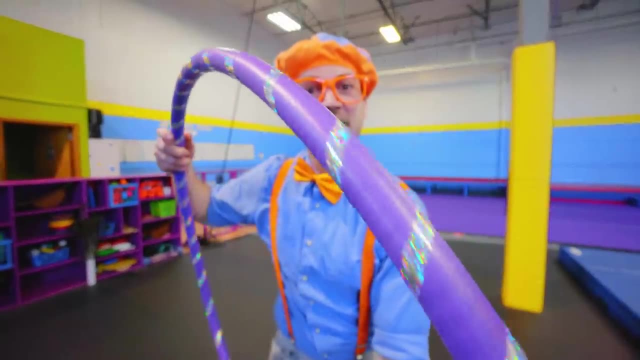 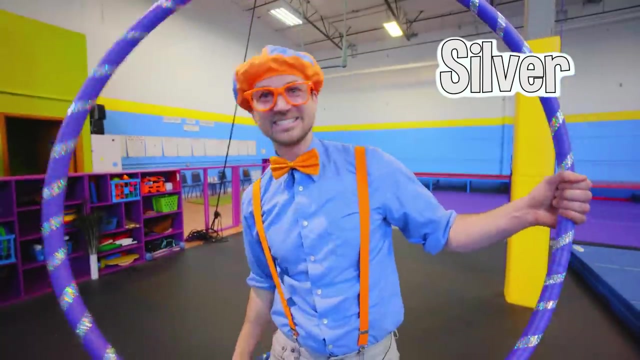 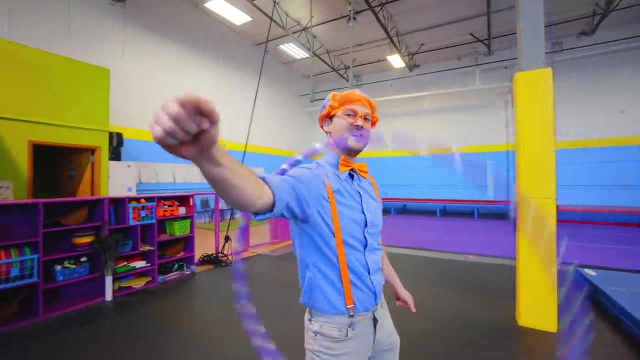 Blue. Wow, That's a great color. My two favorite colors are blue and orange, And this one, yeah, is the color purple and the shiny silver sparkle. Yeah, Let's use this one. All right, I'm going to first try and spin it on my arm. Whoa, Yeah. 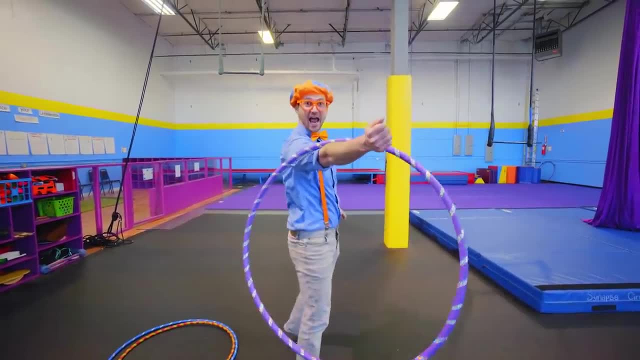 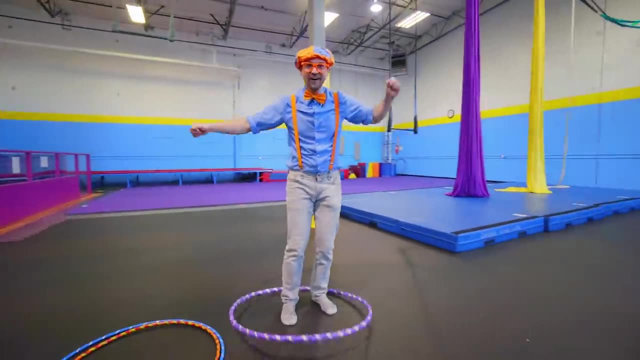 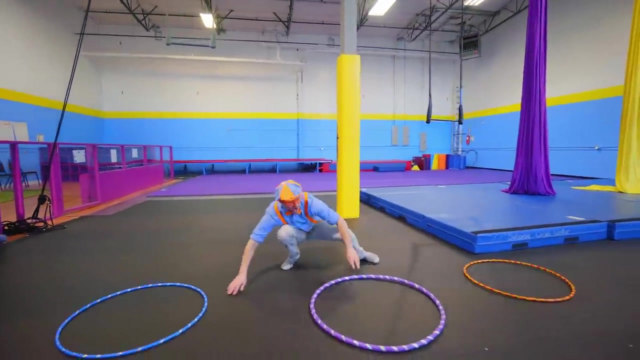 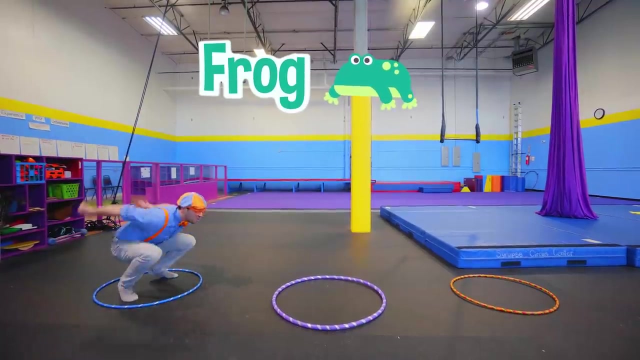 Check this out. Yeah, All right, Here we go. I have an idea. Now that they're on the ground, I think we should spread them out and try and hop through them. Yeah, All right, How about, like a frog, Ribbit, Ribbit, Ribbit, Ribbit. 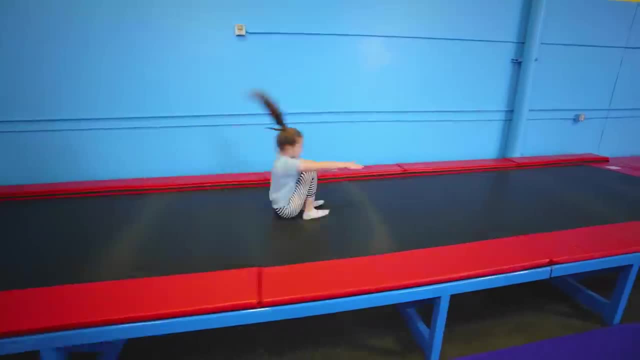 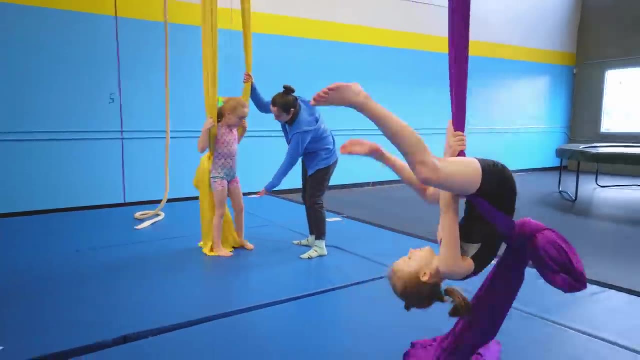 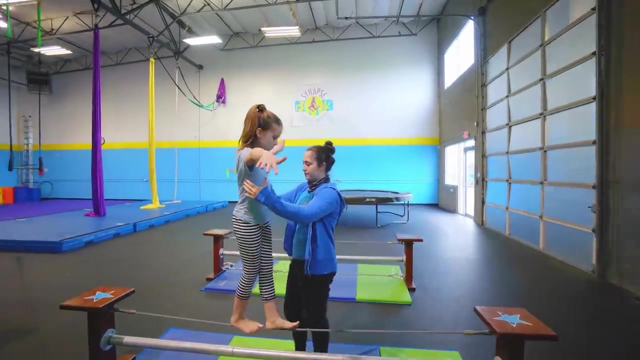 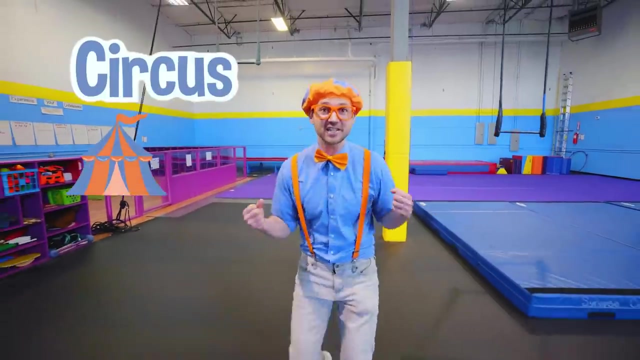 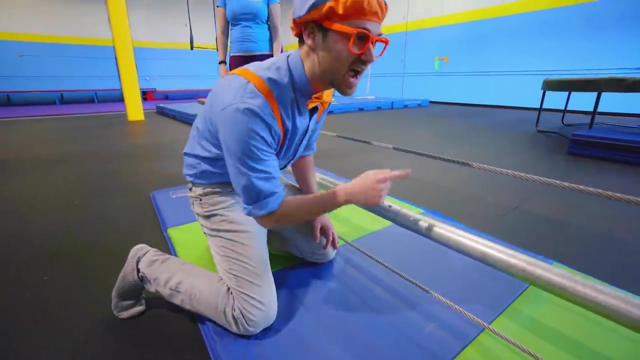 Yeah, Good job. Woo-hoo, This has been so much fun learning all these circus skills. Yeah, Whoa, Check it out. Yeah, Remember this. This is the tight wire. Whoa, Yeah, And you and I are going to try and balance. 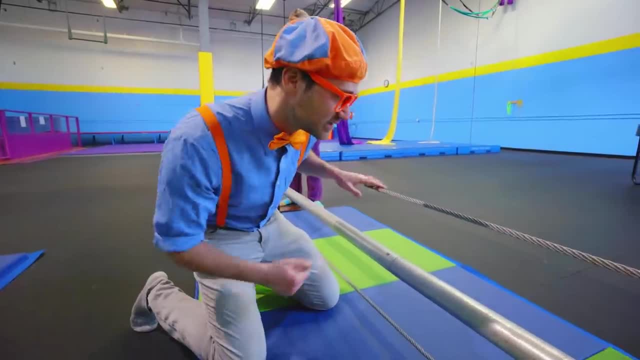 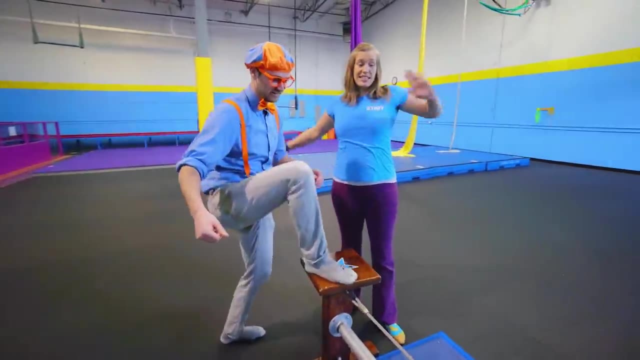 on this. It looks really hard, because how small it is. Whoa. All right, Let's try this. All right, Step right up here onto this platform and then you're going to stand up so tall and walk through the rest. All right, I'm in right here in case you fall. All right, Perfect, Here I go. 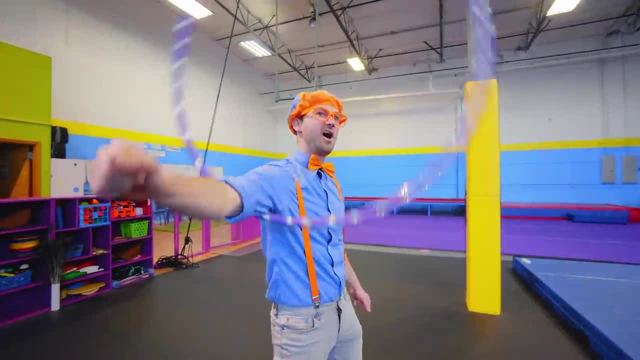 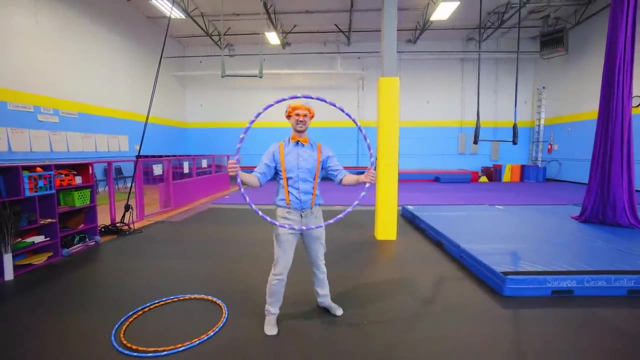 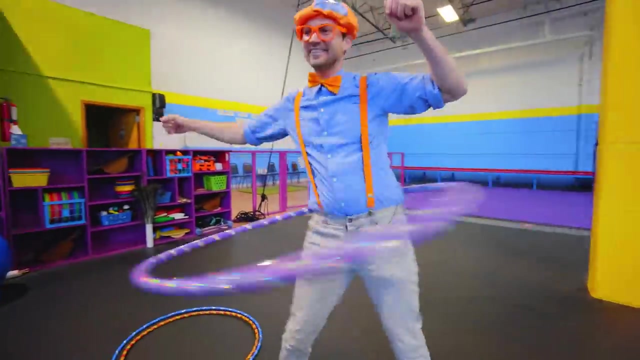 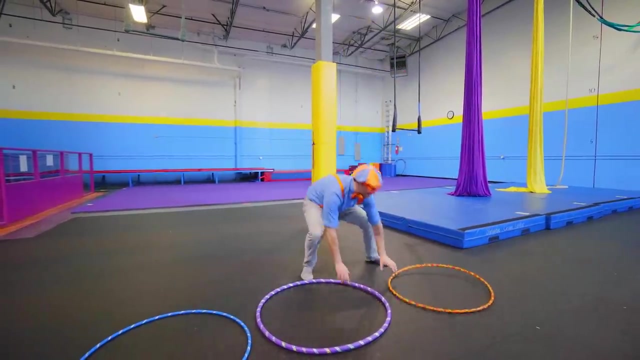 spin it on my arm. Whoa, Whoa, Yeah, Wee, Whoa, Check this out. Yeah, All right, Here we go. I have an idea: Now that they're on the ground, I think we should spread them out. 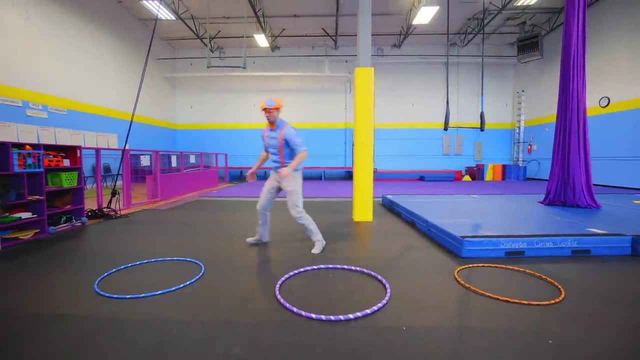 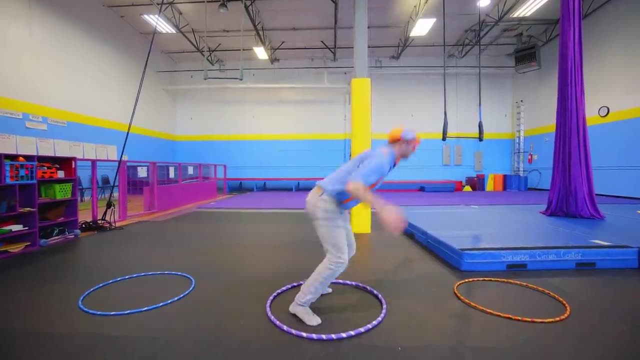 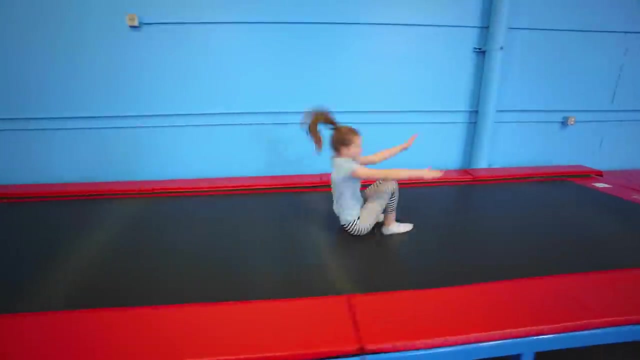 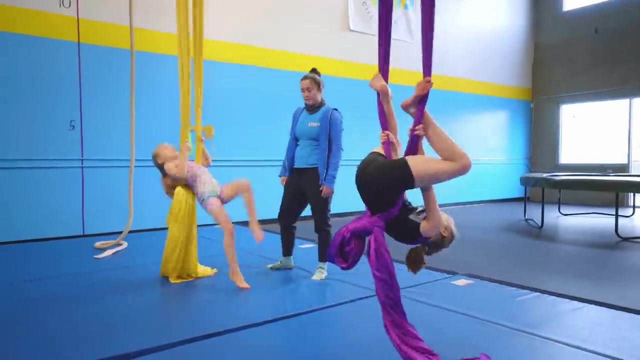 and try and hop through them. Yeah, All right. How about like a frog? Ribbit, Ribbit, Ribbit, Ribbit. Yeah, Good job. Woo hoo, hoo, hoo, hoo hoo. This has been so much fun learning all these. 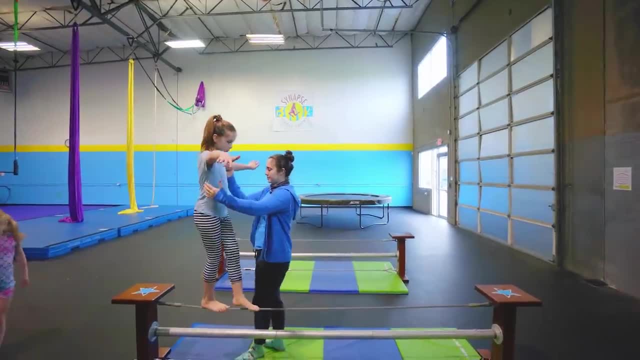 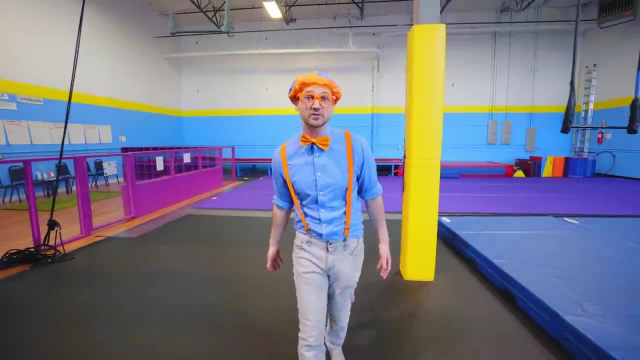 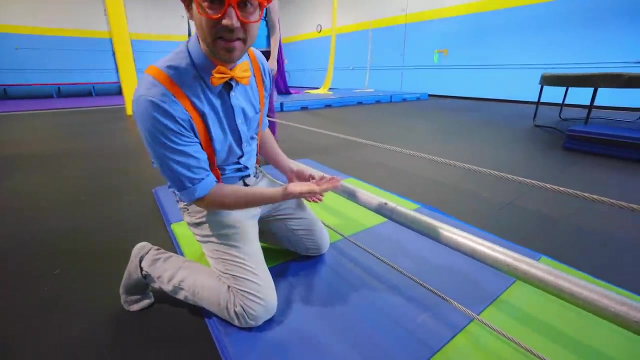 circus skills. Yeah, Whoa, Check it out. Yeah, Remember this. This is the tight wire, Whoa, Yeah, And you and I are going to try and balance on this. It looks really nice. Yeah, Yeah, Yeah. 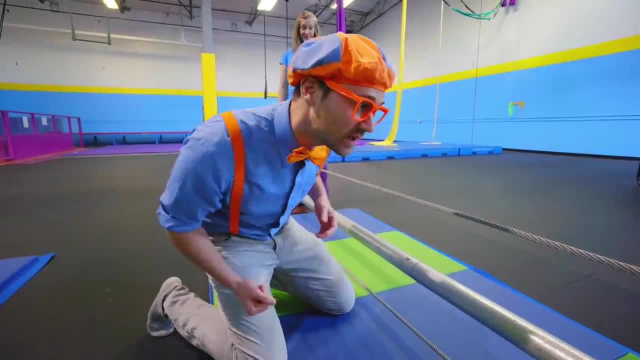 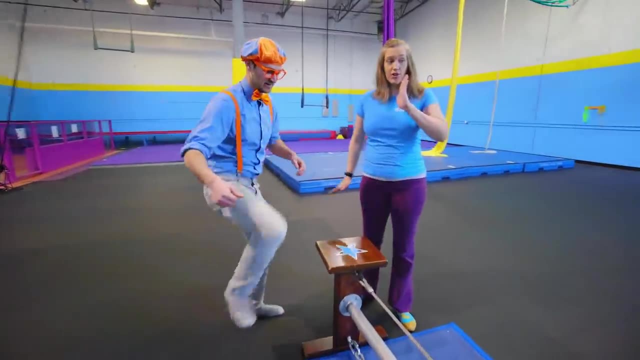 And you and I are going to try and balance on this. It looks really hard, because how small it is, Whoa. All right, Let's try this. All right, Step right up here onto this platform and then you're going to stand up so tall and walk through there. 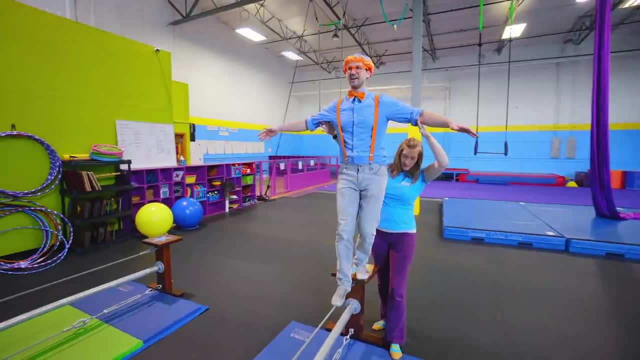 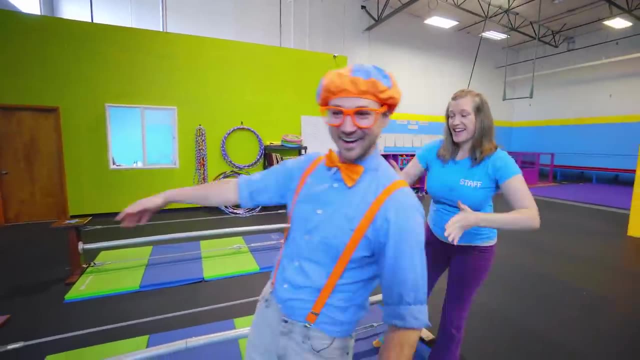 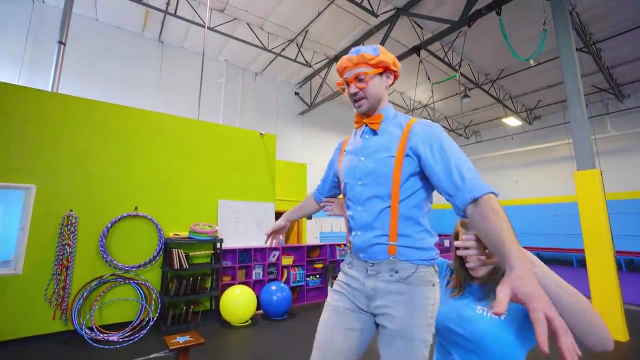 All right, I'm in right here in case you fall. All right, Perfect, Here I go. Whoa, Whoa, Whoa. I fell, That's okay, I'll try it again. Here we go, Whoa. 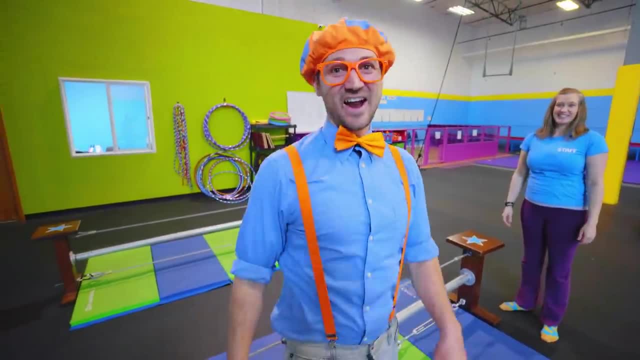 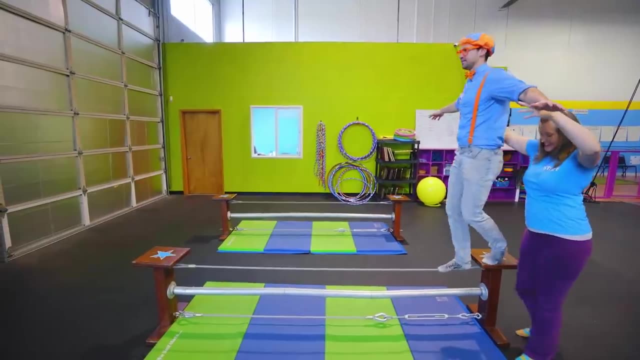 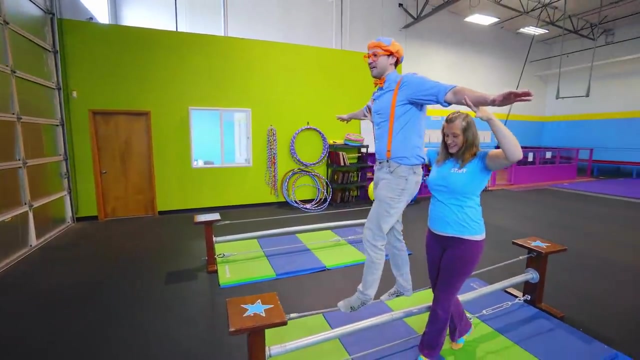 I fell again. That was so much fun though. All right, Let me try for a third time. Here we go. I got this Whoa, Check it out. I'm really doing it. Whoa, Whoa. Yeah, I did it. 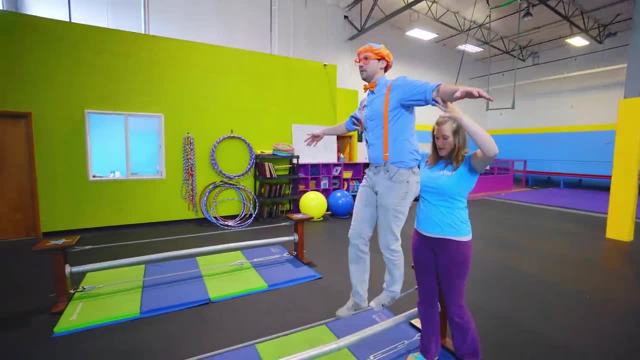 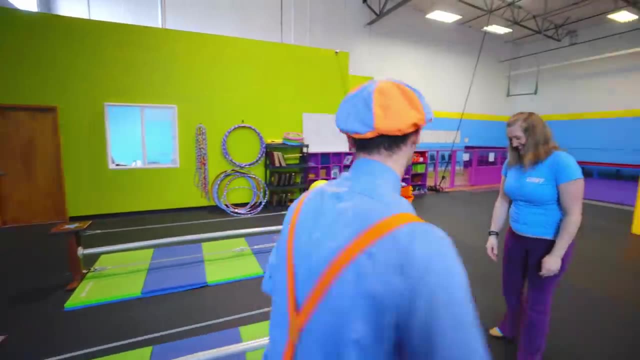 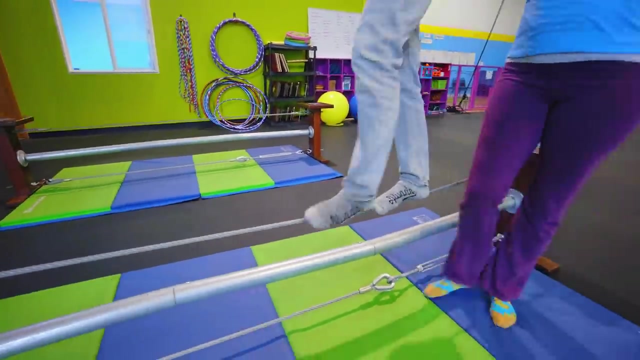 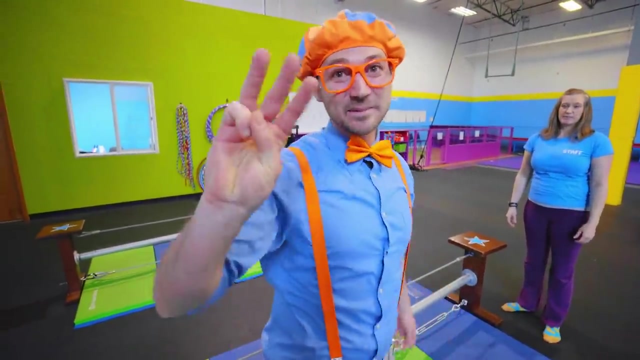 Whoa, Whoa, Whoa. Oh, I fell, That's okay, I'll try it again. Here we go. Whoa, I fell again. That was so much fun, though. All right, Let me try for a third time. 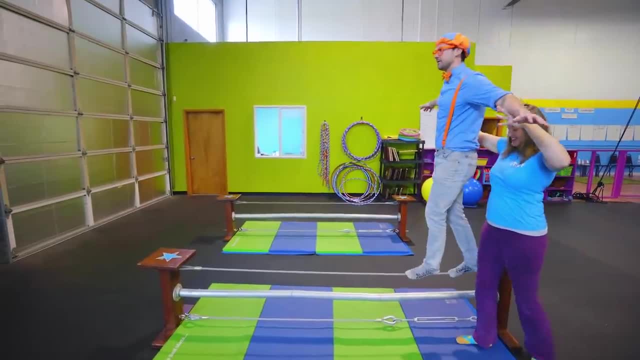 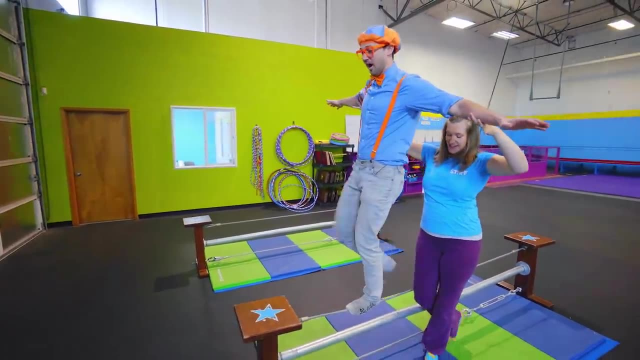 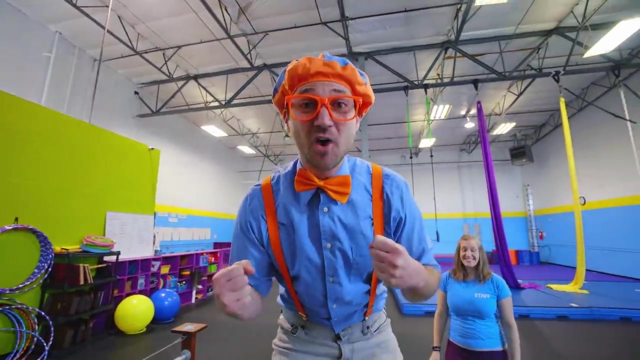 Here we go. I got this. Whoa, Check it out. I'm really doing it. Whoa, Whoa. Yeah, I did it. Did you see that? Yeah, that was really hard and it feels so good to accomplish something that was. 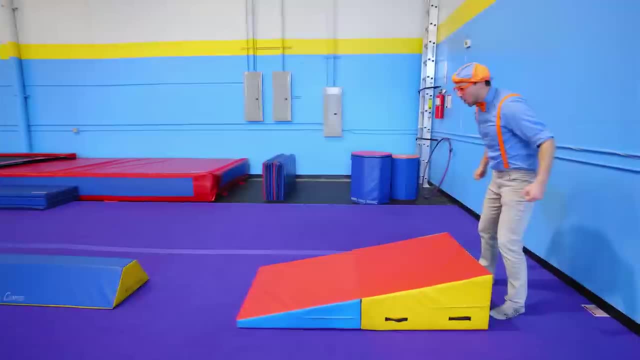 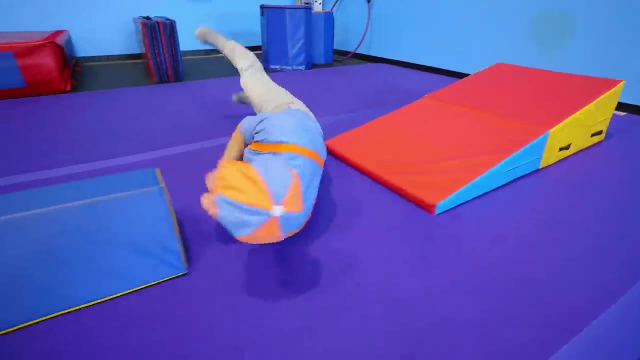 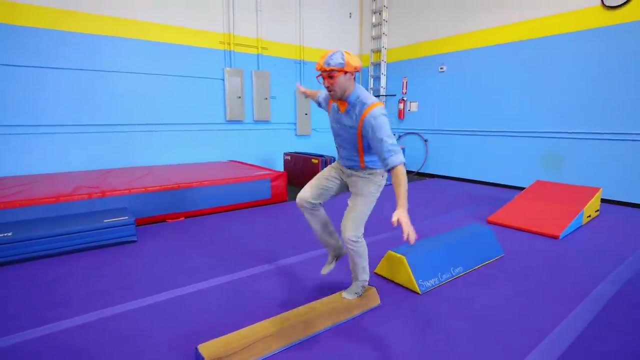 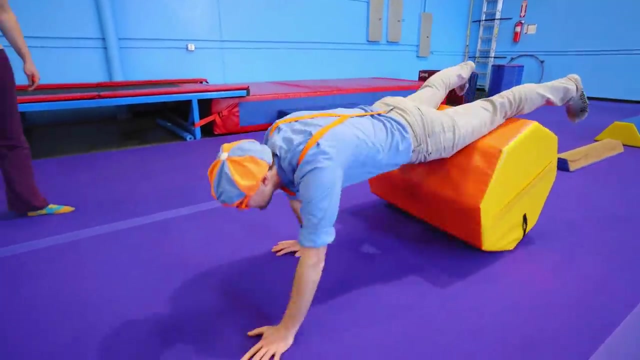 extra hard. Good job, Okay. first I'm gonna start with a roll. Here we go, Whoa. Alright, now for the balancing: Whoa, Whoa. Now for the arm walk: Here we go, Whoa, Whoa. 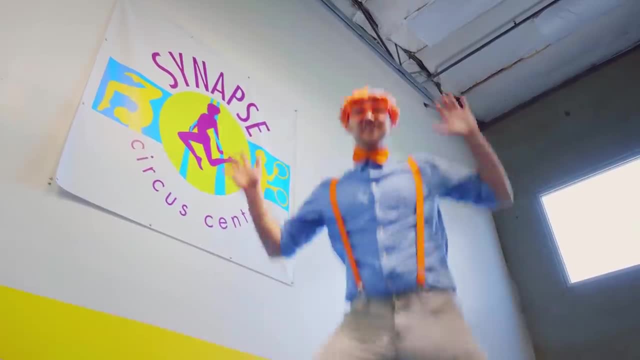 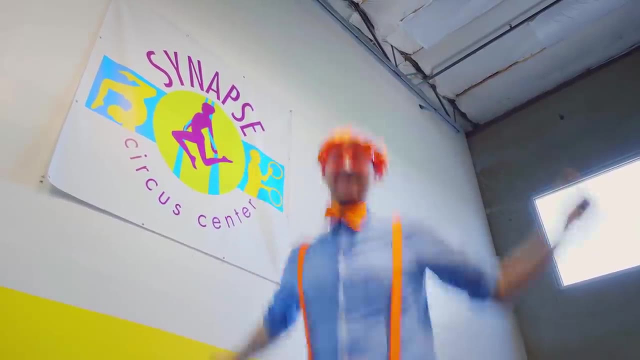 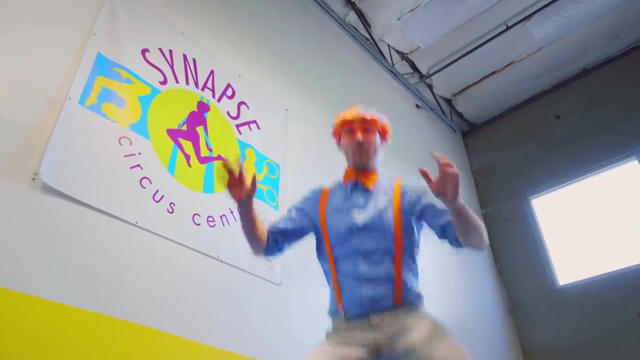 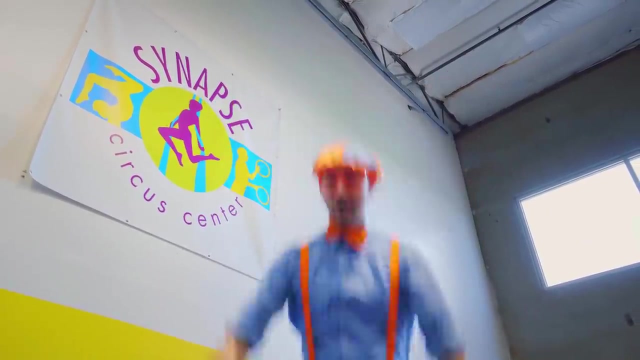 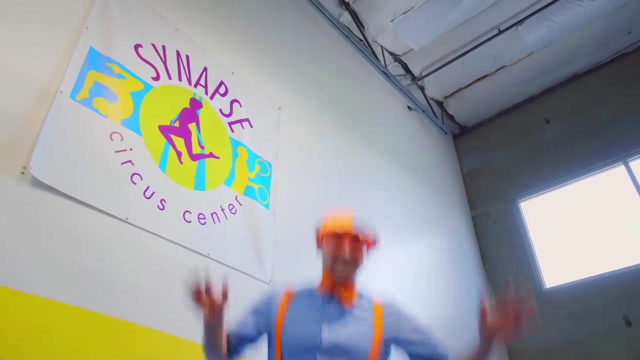 Yeah, Wow, This has been so much fun. Yeah, But this is the end of this video. If you want to watch more of my videos, all you have to do is search for my name. Will you spell my name with me? 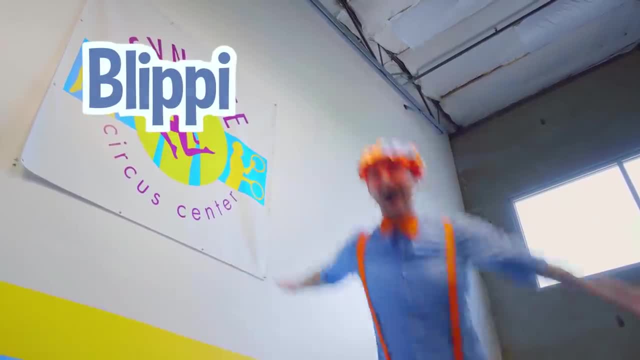 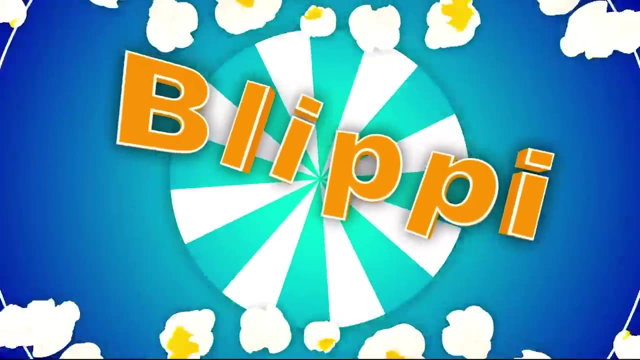 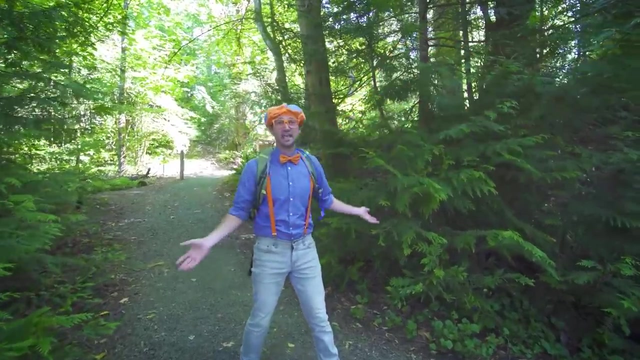 Ready, B-L-I, P-P-I. Woohoo, So much to learn about. It'll make you want to shout Blippi, Whoa. Hey, It's me Blippi, and today we're at Priest Point Park in Olympia, Washington. 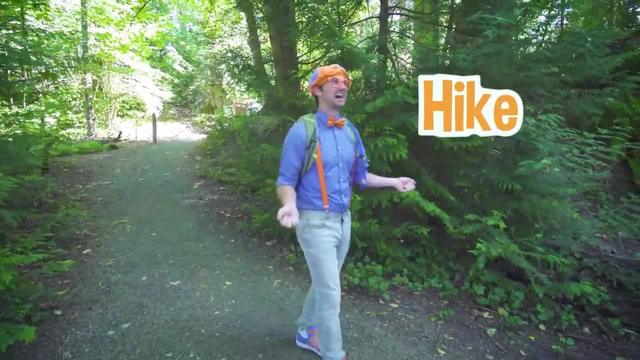 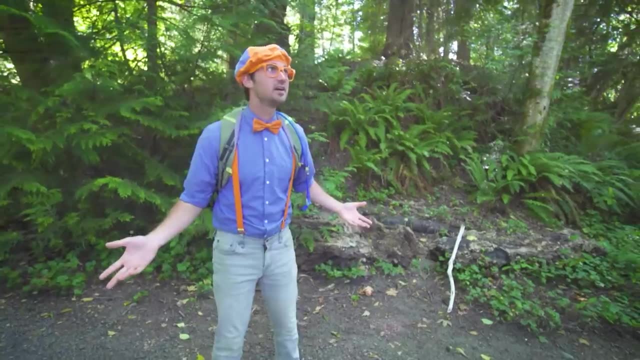 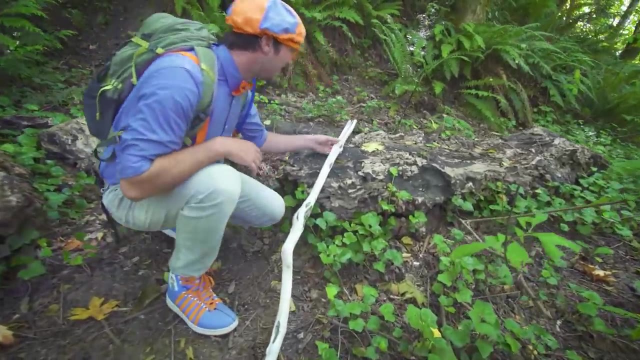 And I am going on a hike. I love hiking because you get to be out in the wilderness. Hey, speaking of hiking, I don't have a hiking stick. Maybe I could find one. Do you see one anywhere? Oh, Hey, Check it out. 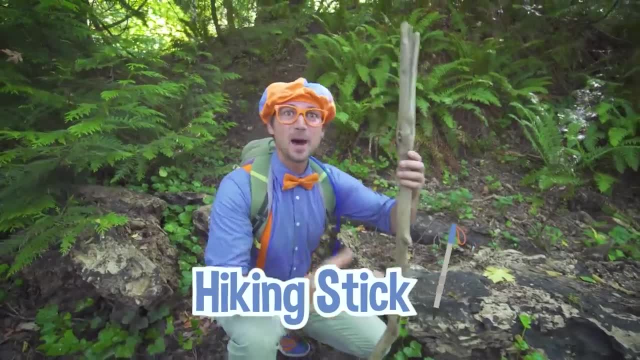 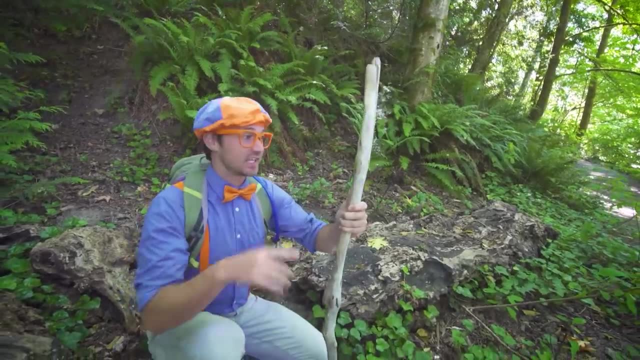 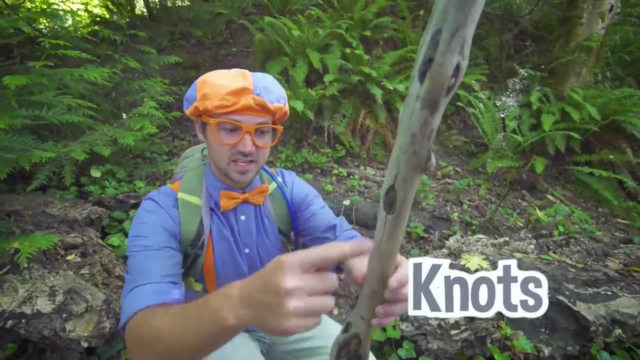 This is a perfect hiking stick. Amazing, It's so smooth. There's no bark on it. Yeah, I'm definitely not going to get any slivers with this stick. Wow, And look how unique this stick looks. There's a bunch of knots in it. 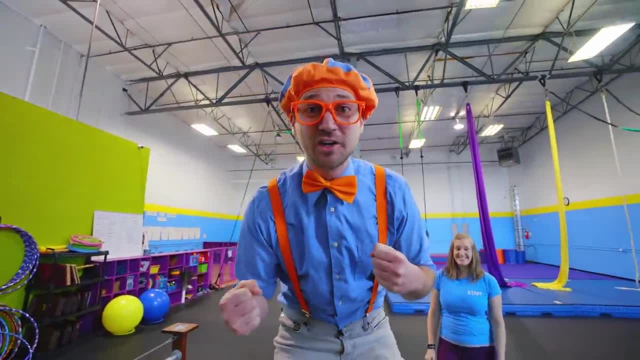 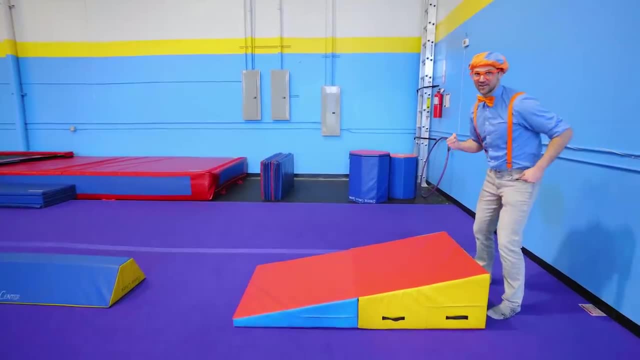 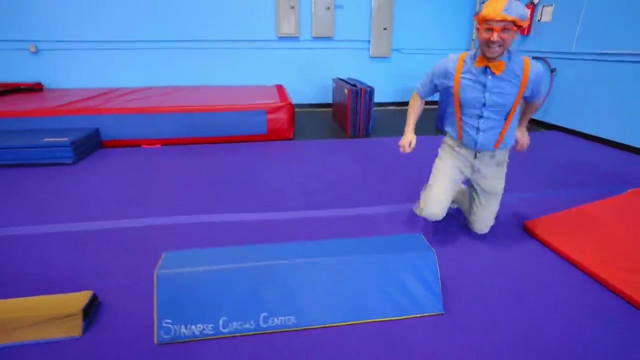 Yeah, That was really hard And it feels so good to accomplish something that was extra hard. Good job, Okay, First I'm going to start with a roll. Here we go. Whoa, All right, Now for the balancing. Whoa. 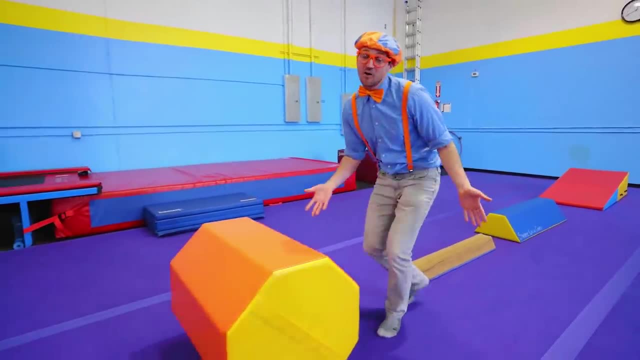 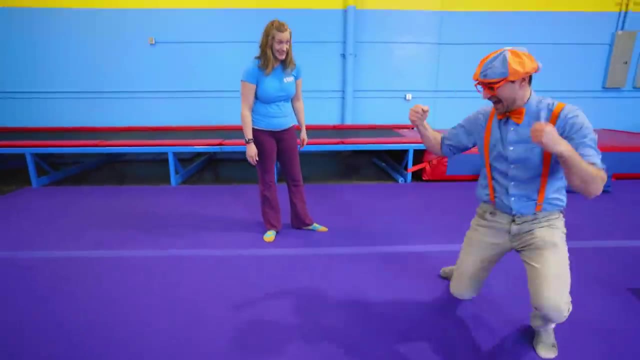 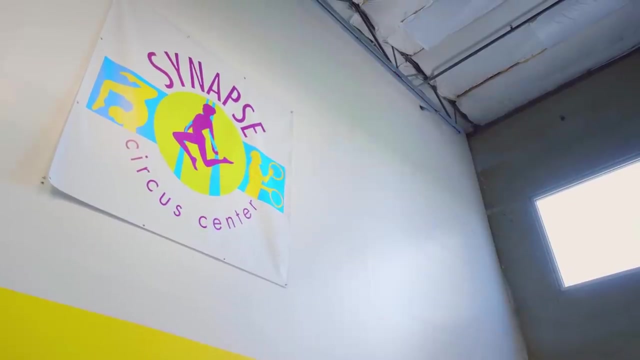 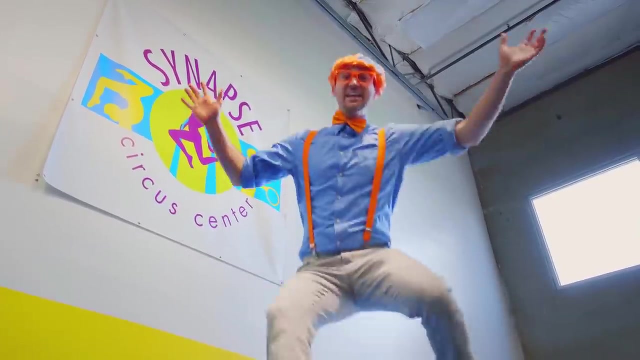 Whoa, Now for the arm walk. Here we go, Whoa, Whoa, Whoa, Yeah, Wow, This has been so much fun, Yeah, But this is the end of this video. If you want to watch more of my videos, 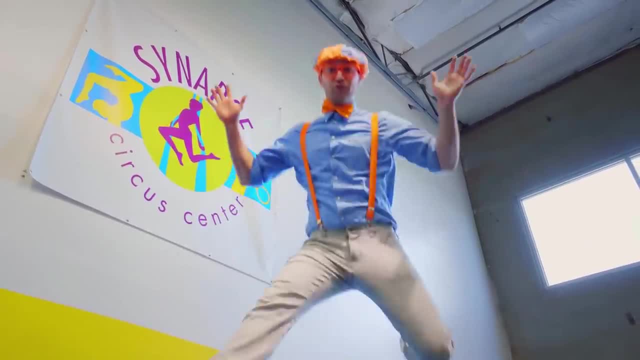 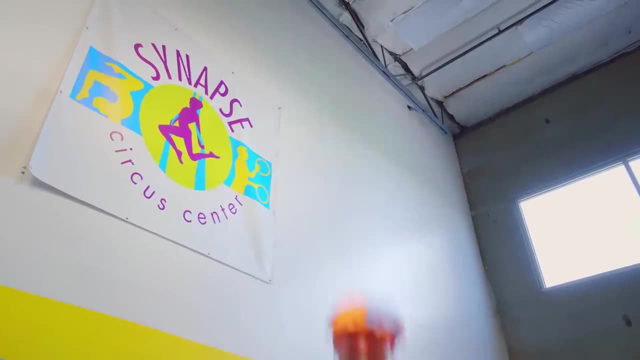 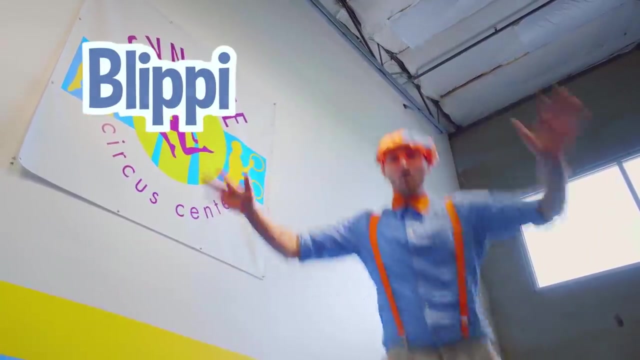 all you have to do is search for my name. Will you spell my name with me? Will you spell my name with me? Ready B-L-I-P-P-I, Ready B-L-I-P-P-I. Woohoo, So much to learn about. 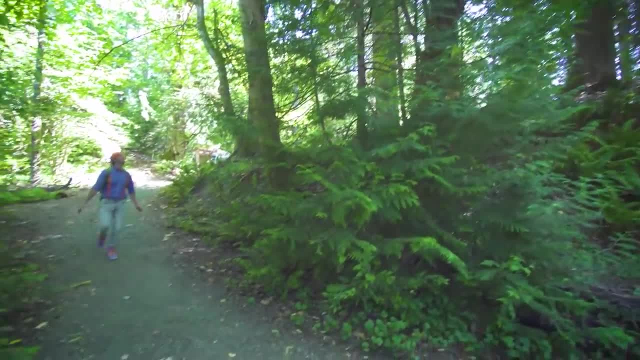 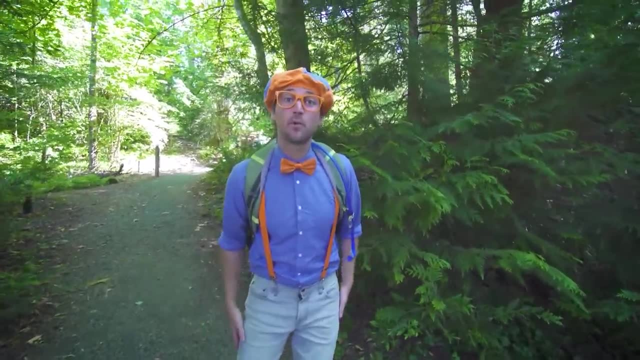 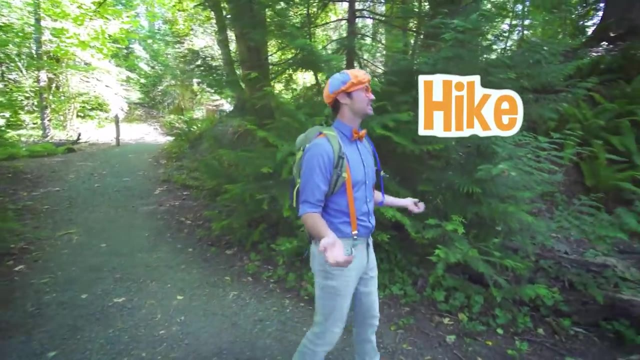 It'll make you want to shout: Blippi, Whoa. Hey, It's me Blippi. And today we're at Priest Point Park in Blippio, Washington And I am going on a hike. I love hiking because you get to be. 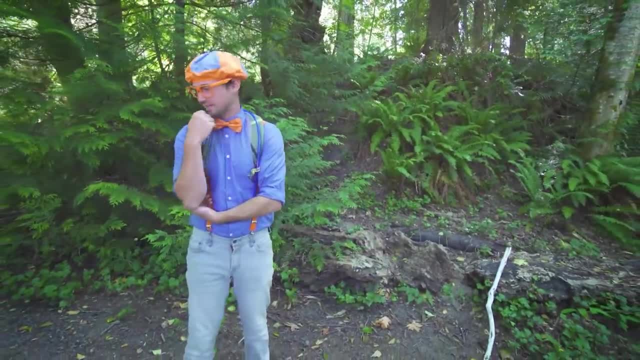 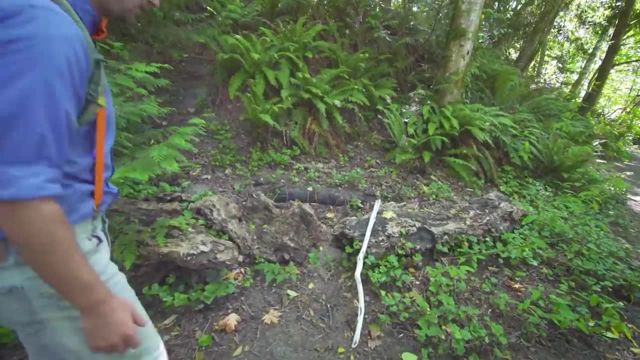 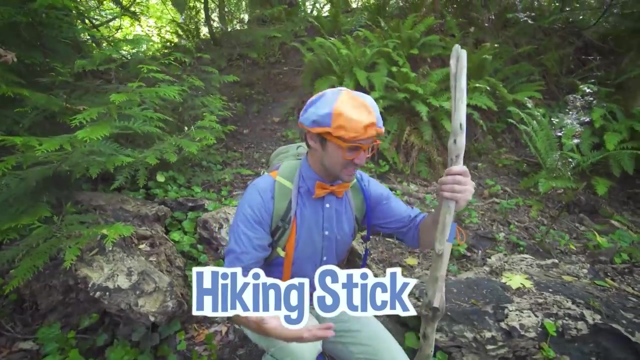 out in the wilderness. Hey, speaking of hiking, I don't have a hiking stick. Maybe I could find one. Do you see one anywhere? Oh, Hey, check it out. This is a perfect hiking stick. Amazing, It's so smooth. 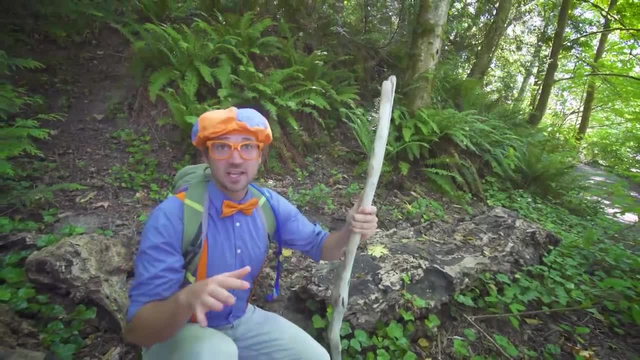 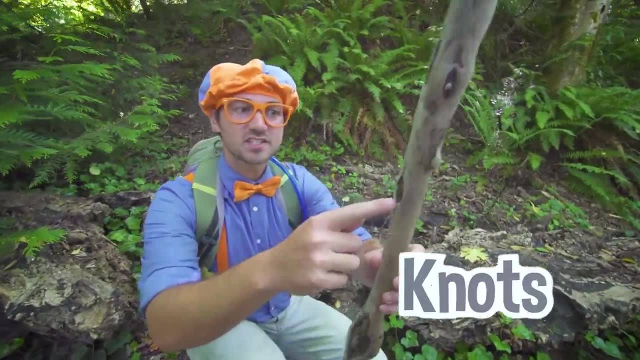 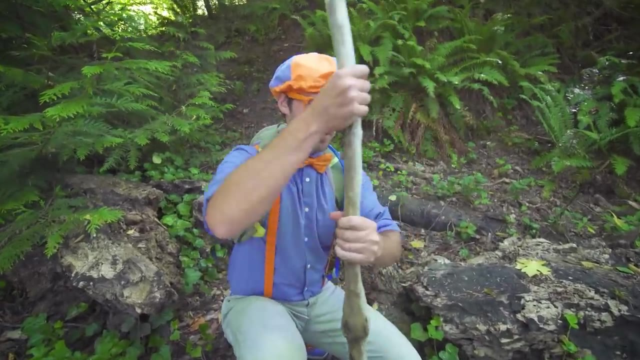 There's no bark on it. Yeah, You don't get any slivers with this stick, Wow, And look how unique this stick looks. There's a bunch of knots in it. Yeah, Whoa, That's a really cool stick. 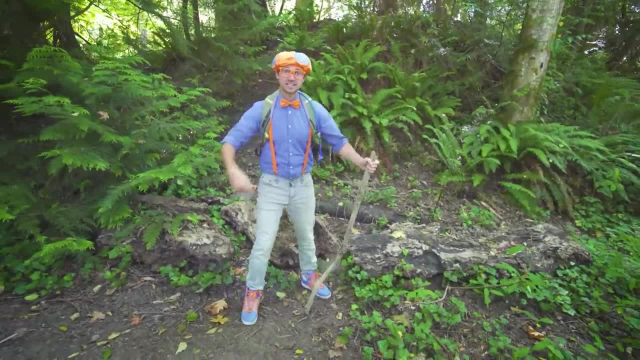 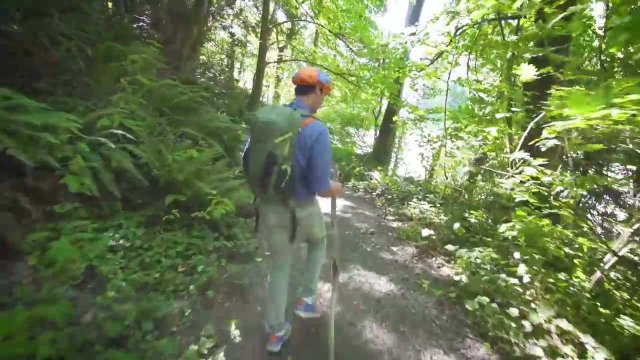 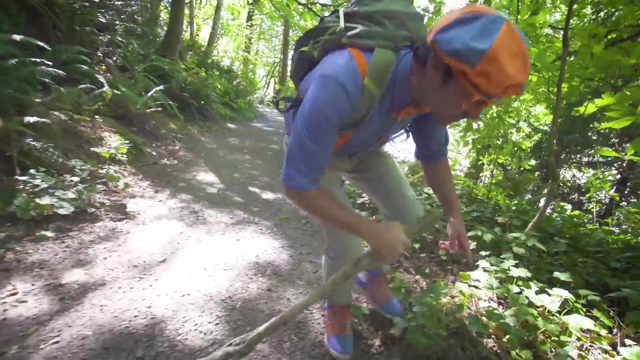 Alright, let's test it out. Awesome And it's really strong. Alright, let's continue hiking. Whoa, Whoa, Look down here. Look at what we found. Wow, do you see this? These are clam shells. 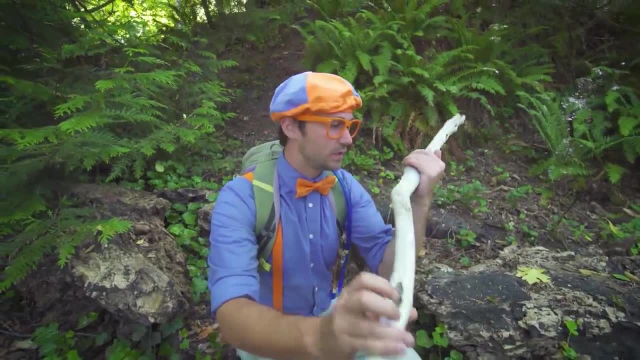 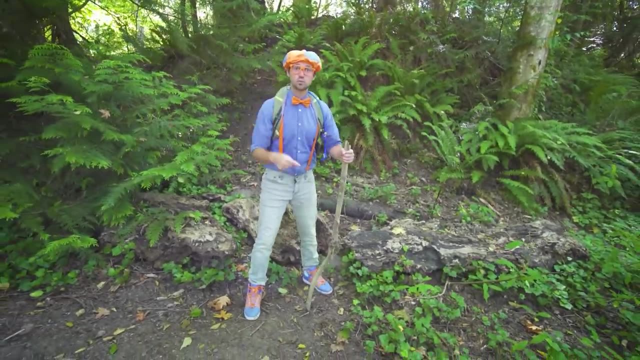 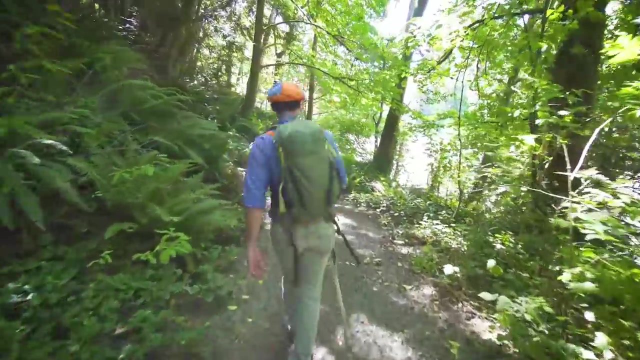 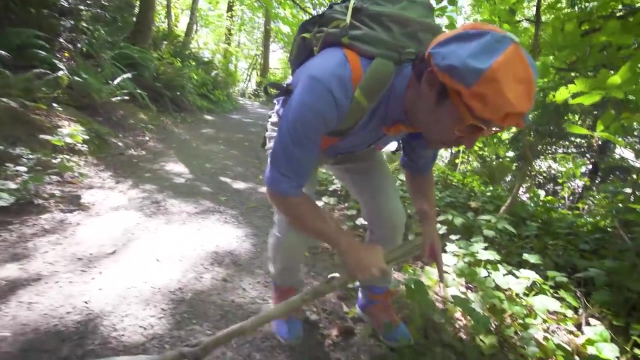 Yeah, Whoa, That's a really cool stick. Alright, let's test it out. Ugh, Awesome And it's really strong. Alright, let's continue hiking. Whoa, Whoa. Look down here. Look at what we found. 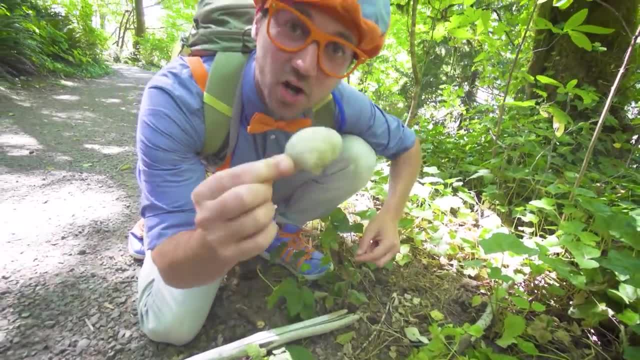 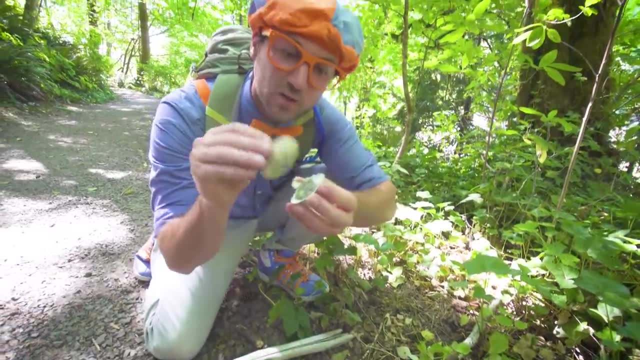 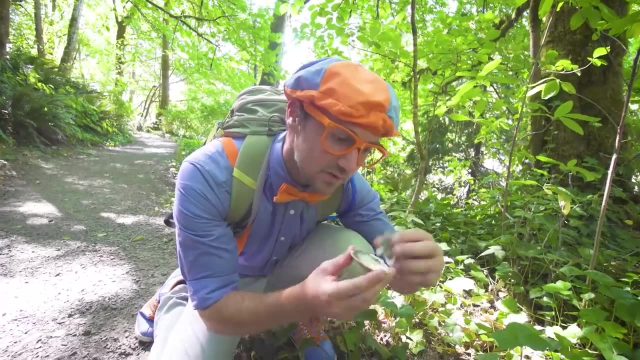 Wow, do you see this? These are clam shells. Yeah, do you see them? Whoa, These used to be fully closed, just like this, And there used to be a clam inside, But now there's no clam. Where'd the clam? 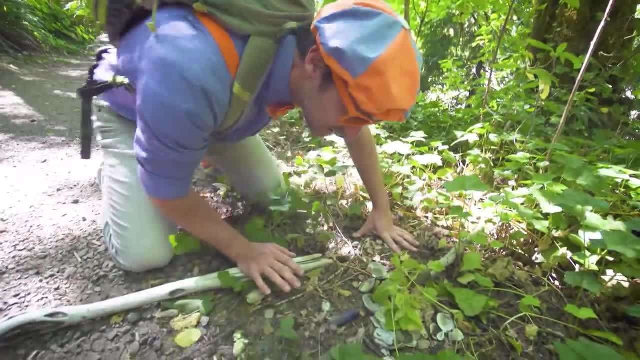 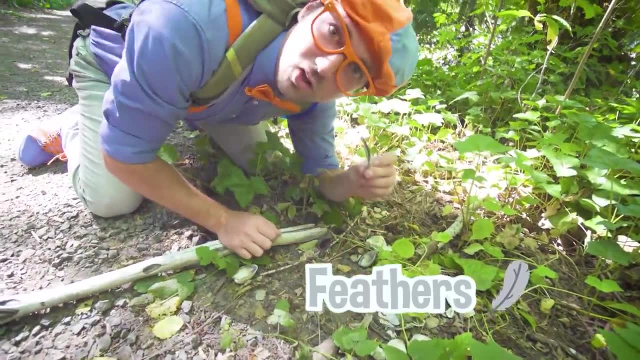 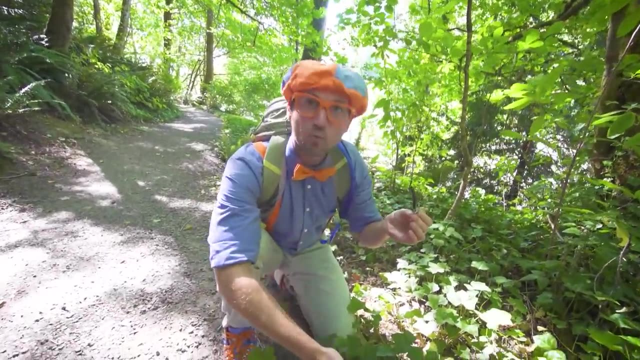 go. Wait a second, Do you see this? This is a clue. These are feathers. Yeah, Look, Bird feathers. Wait a second. I wonder if a bird was hanging out right here. Yeah, maybe it was having lunch. Okay, well, I'm going to take. 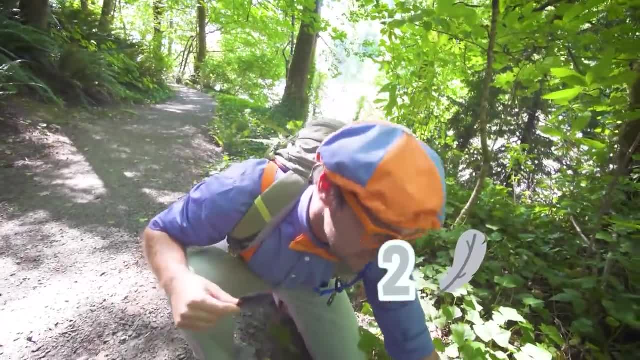 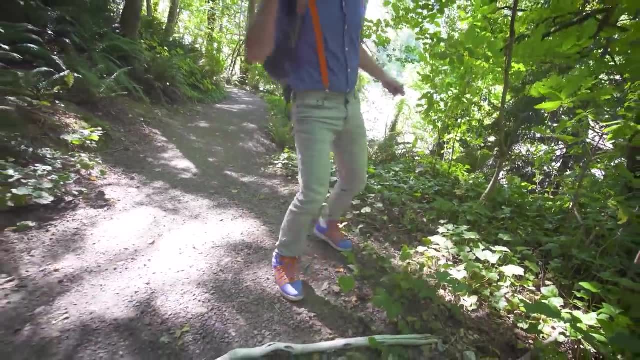 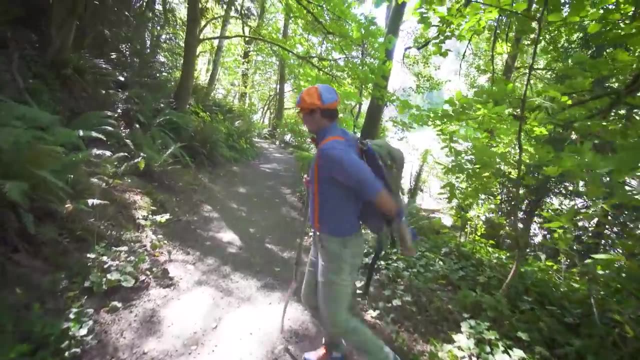 one of these two feathers and put it in my bag, and I'll show you something really cool later. And one clam shell. Alright, let me put it in my bag and then we'll continue on. Haha, Okay, let's go. Oh, gotta stay hydrated. 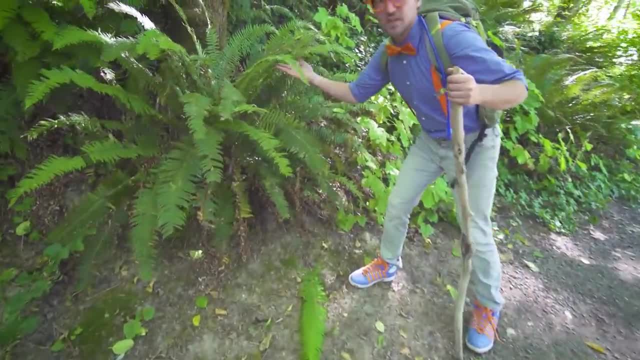 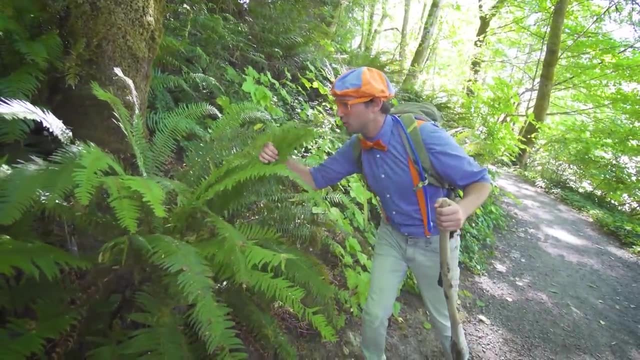 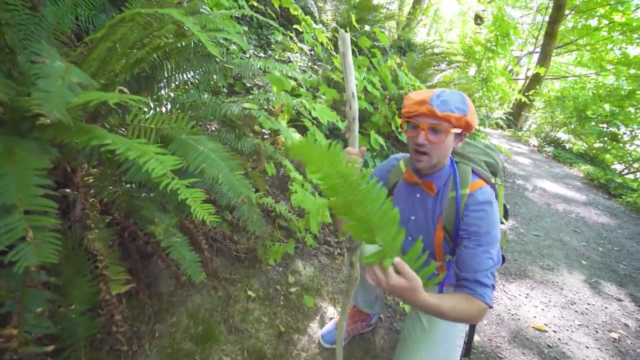 Whoa, Look at this plant. This plant is a fern. Wow, it's a beautiful plant. It's so cool looking. Oh, hey, It lost one of its limbs. Yeah, Yeah, a bunch of leaves are on this. 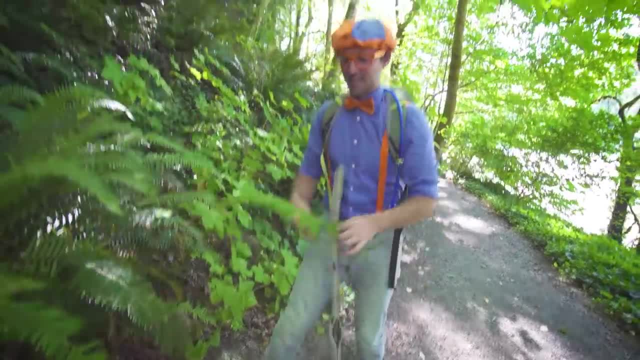 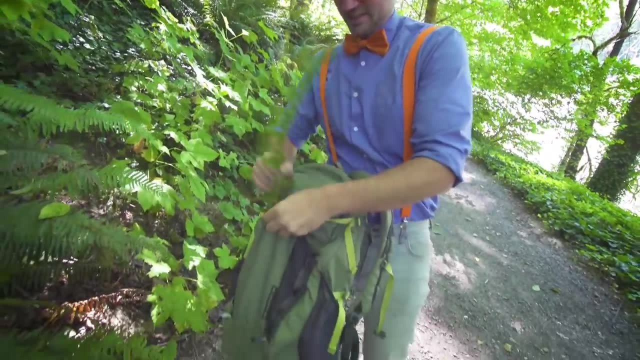 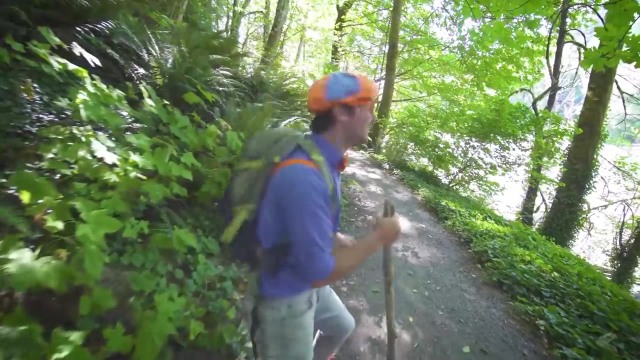 I have an idea What if we keep this and use it for something really cool later? Let me put it in my bag, just like this, and then I'll show you later. Haha, Alright, come on, let's go. Whoa. 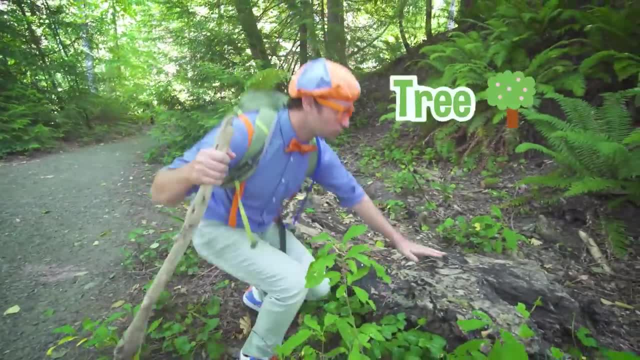 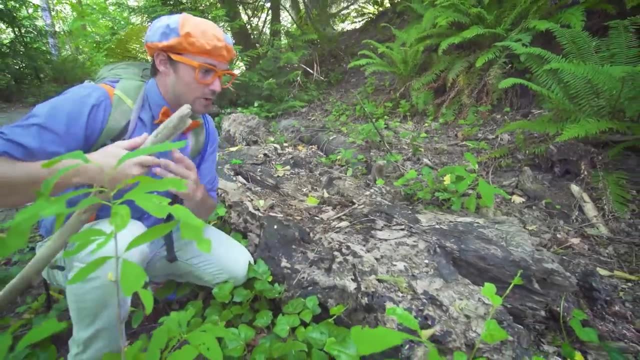 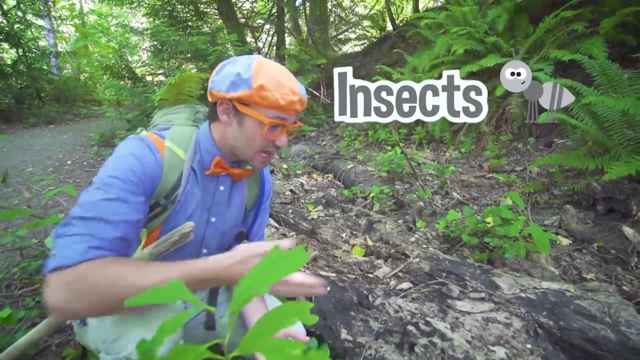 Check it out: Whoa, an old tree. Yeah, this tree used to be vertical and then it fell down, Whoa. and when trees fall down, they decompose and they allow for a great opportunity for insects- yeah- and animals to have a home. 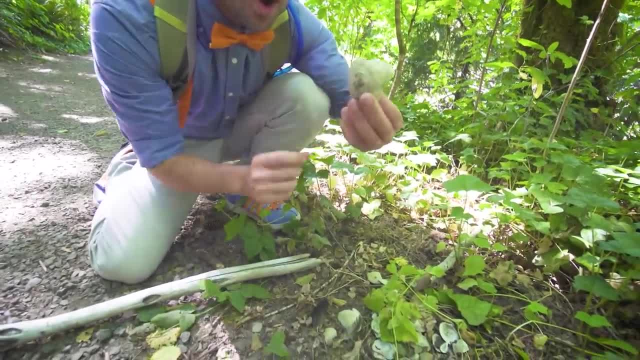 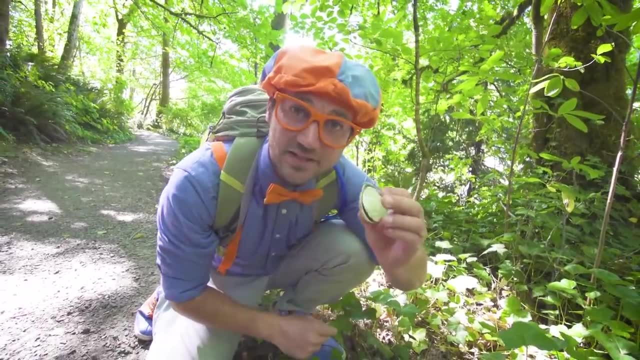 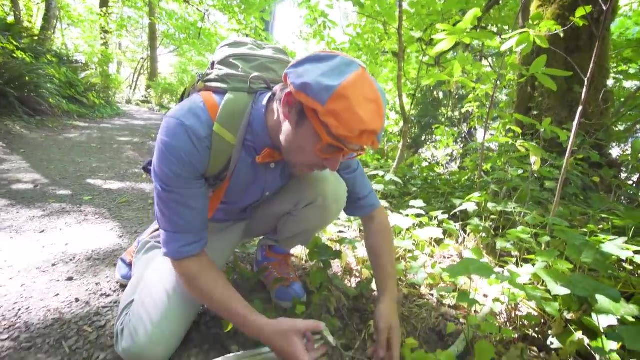 Yeah, do you see them? Whoa, These used to be fully closed, Just like this, And there used to be a clam inside, But now there's no clam. Where'd the clam go? Wait a second, Do you see this? This is a clue. 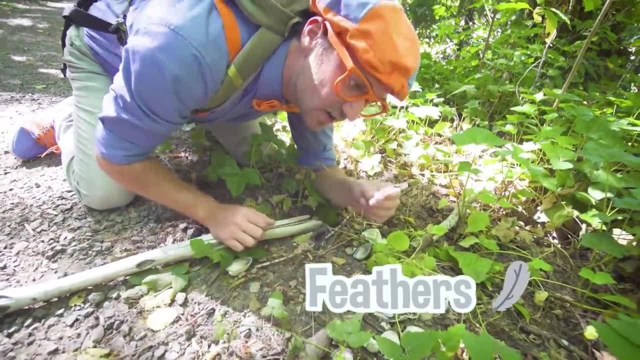 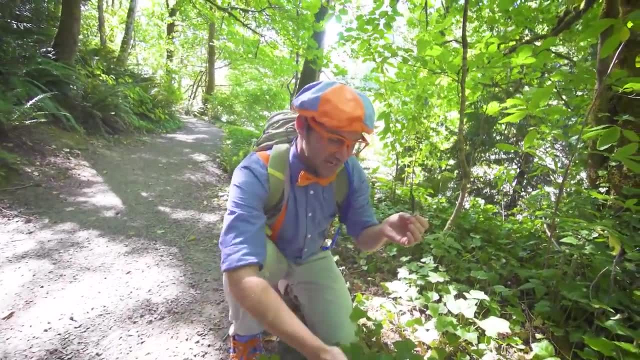 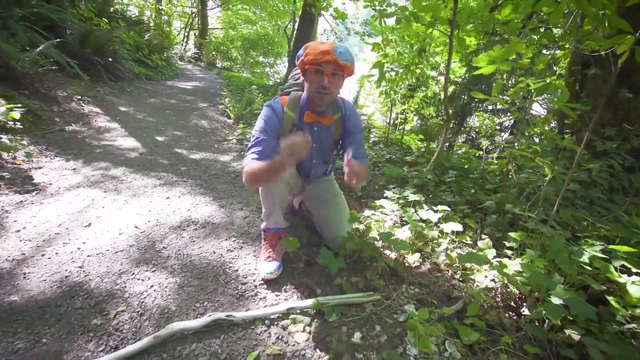 These are feathers. Yeah, Look, bird feathers. Wait a second. I wonder if a bird was hanging out right here. Yeah, maybe it was having lunch, Okay. Well, I'm going to take one of these two feathers and put it in my bag and I'll show you. 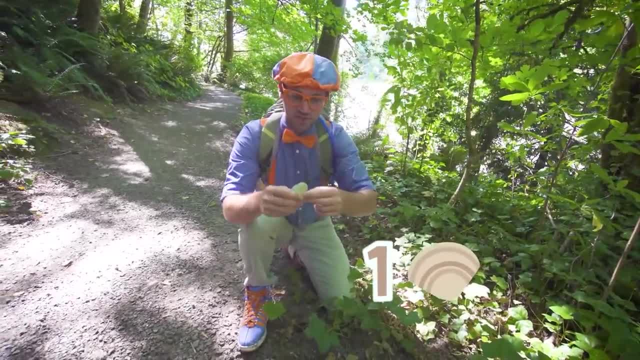 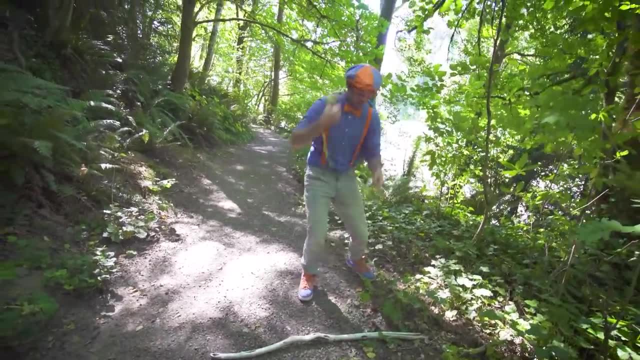 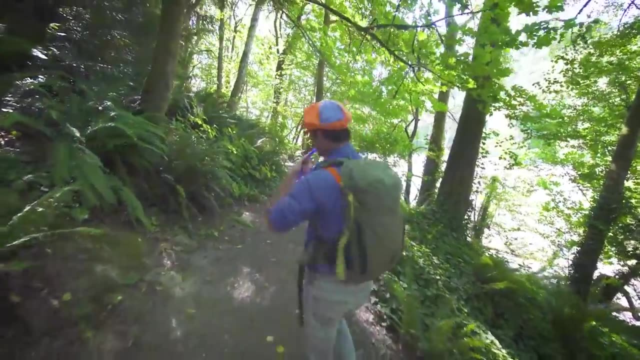 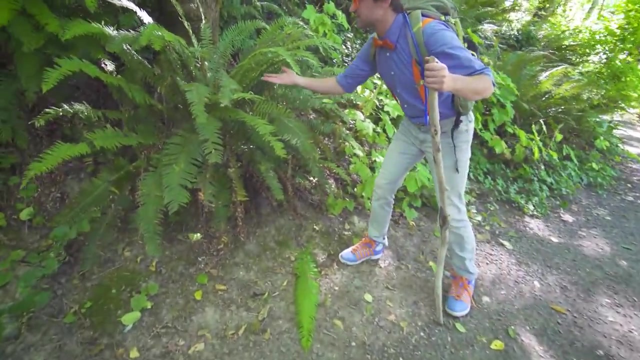 something really cool later And one clam shell. Alright, Let me put it in my bag And then we'll continue on. Okay, let's go. Gotta stay hydrated. Whoa, Look at this plant. This plant is a fern. 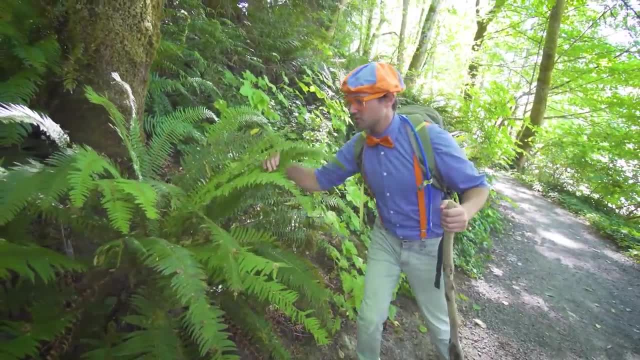 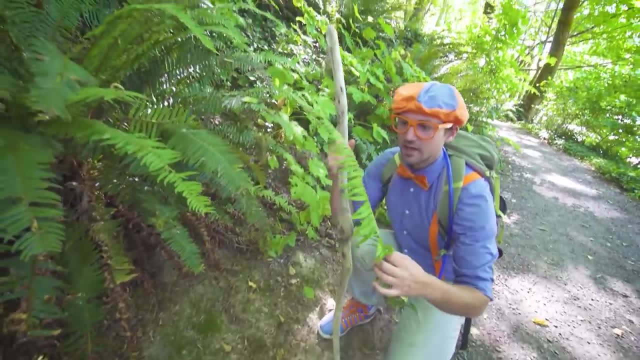 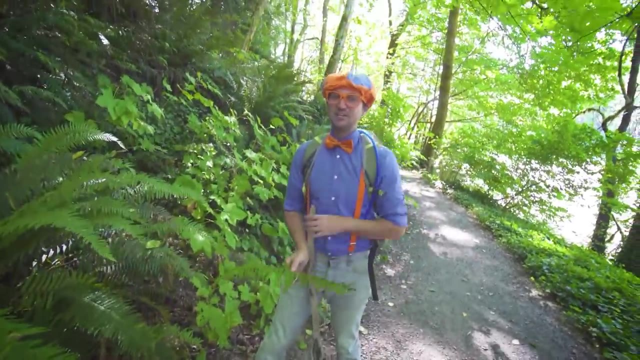 It's a beautiful plant. It's so cool looking. Oh, hey, it lost one of its limbs. Yeah, A bunch of leaves are on this. I have an idea What if we keep this and use it for something really cool later? 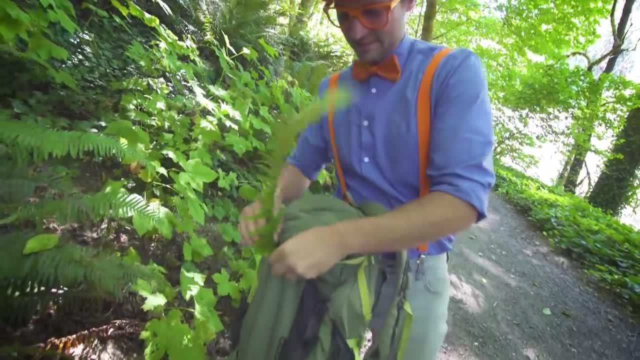 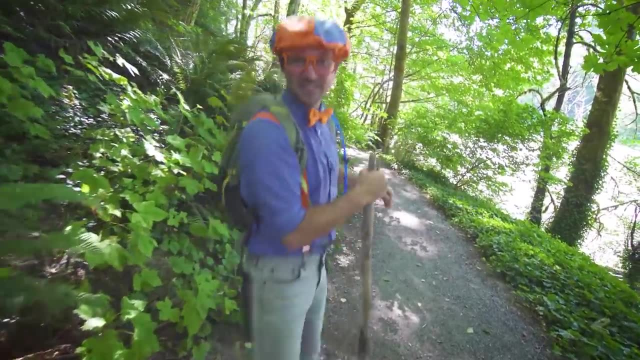 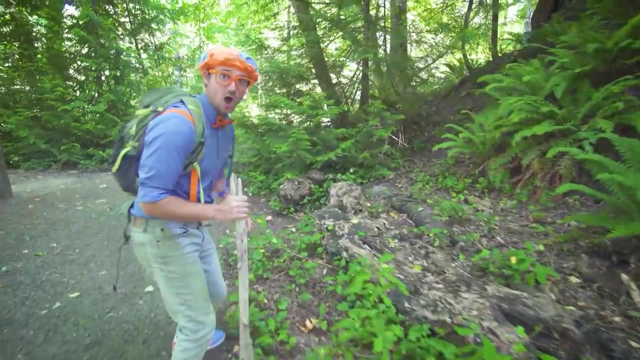 Let me put it in my bag, Just like this, And then I'll show you later. Alright, come on, Let's go. Whoa, Check it out. Whoa, An old tree. Yeah, this tree used to be vertical. 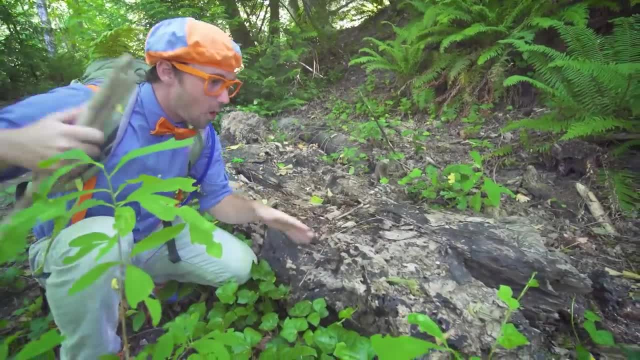 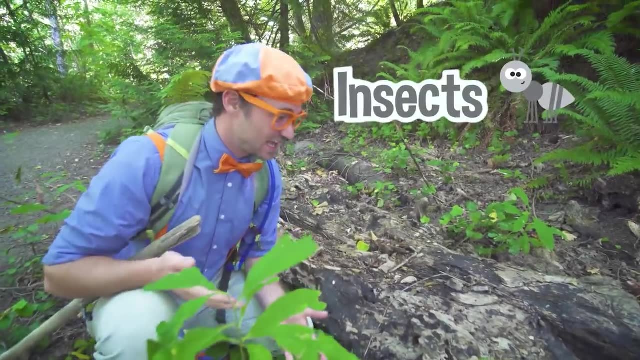 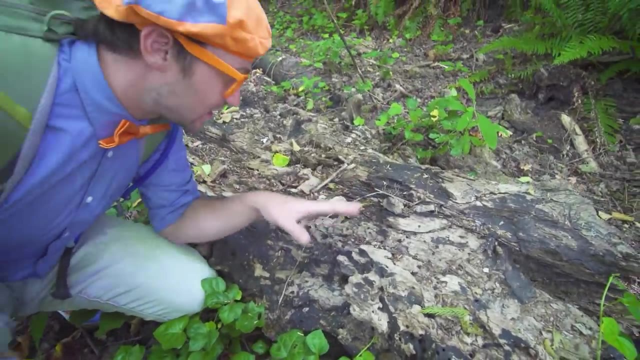 And then it fell down, Whoa. And when trees fall down, they decompose And they allow for great opportunity for insects and animals to have a home. Do you see it? Yeah, Insects love to eat these type of trees. 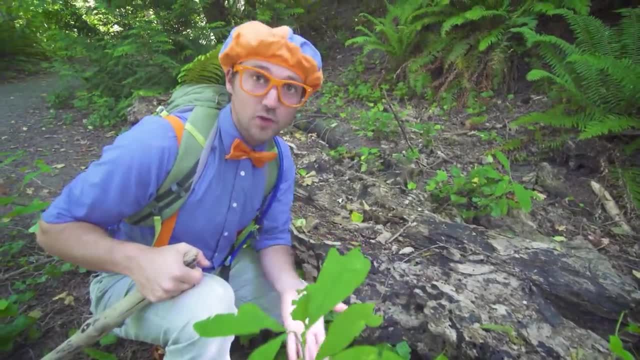 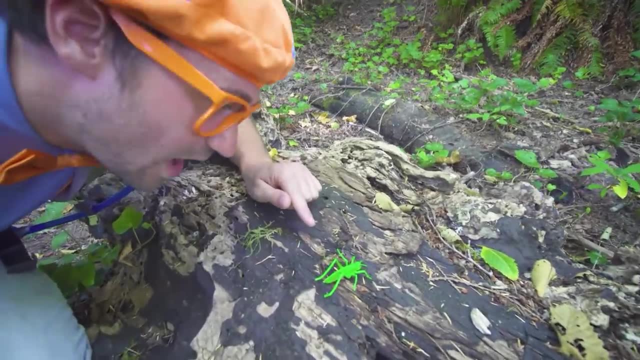 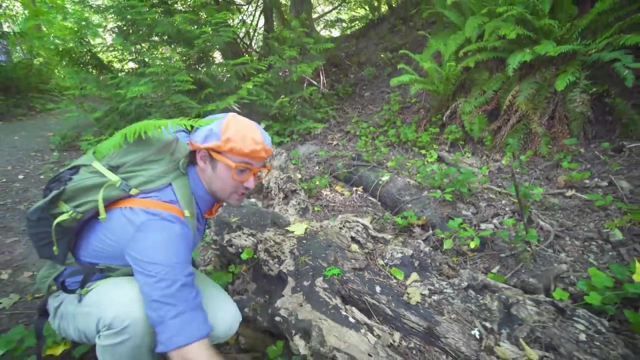 Because then it allows for nutrients to go in the ground. Whoa, Hey, Speaking of bugs, Do you see this? Wow, That is a grasshopper. Hello, grasshopper, Hey, I have something really cool in my backpack. I have. 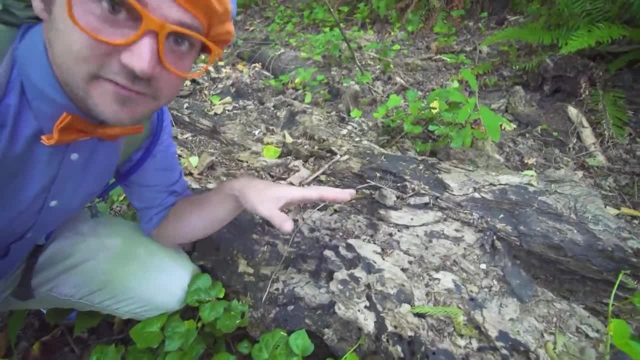 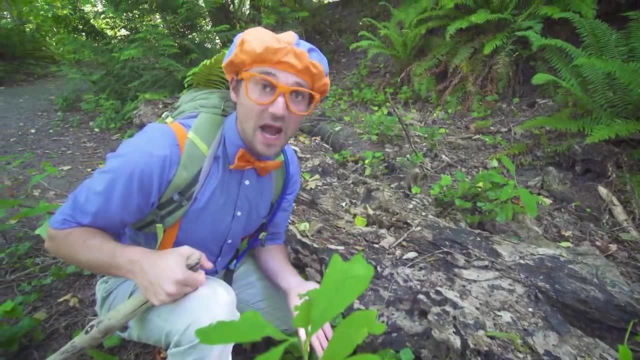 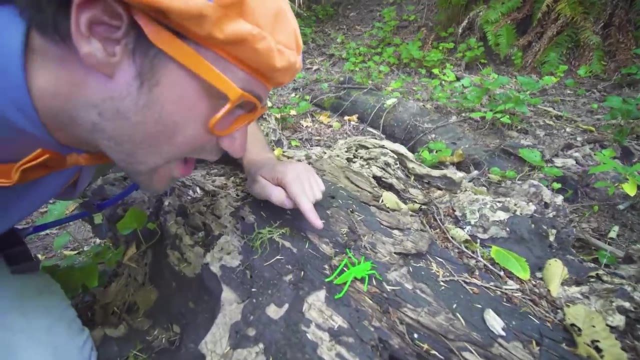 Do you see it? Yeah, Insects love to eat these type of trees. Yeah, because then it allows for nutrients to go in the ground. Whoa, Hey, Speaking of bugs, do you see this? Wow, That is a grasshopper. 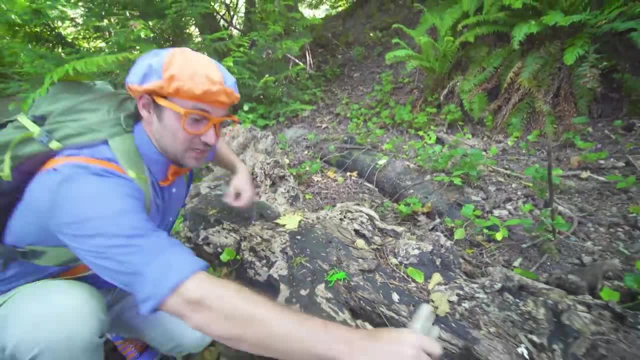 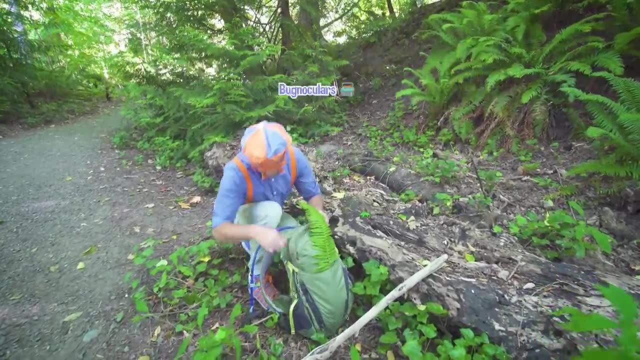 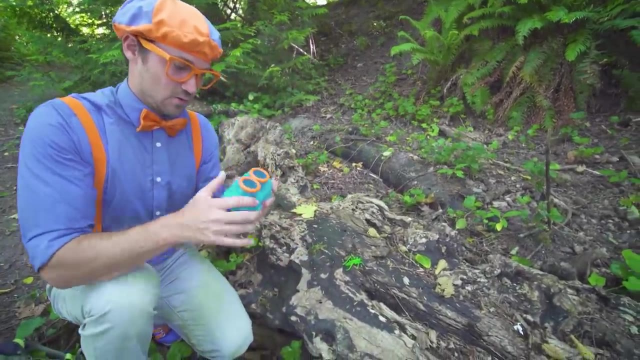 Hello grasshopper. Hey, I have something really cool in my backpack. I have what are called bugnoculars. Let's see here. Bugnoculars are great to use to see bugs up close, So what we're going to do is open them up. 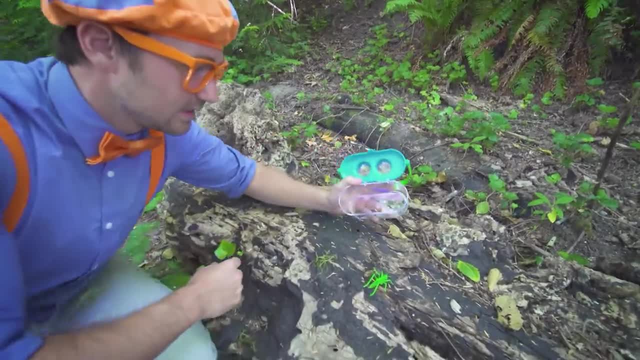 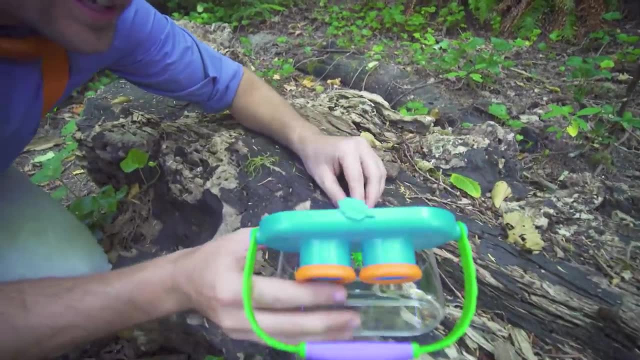 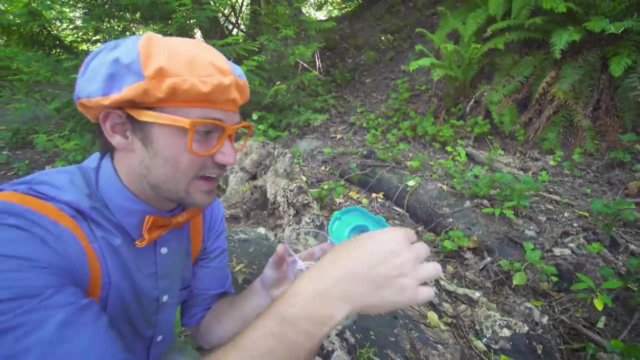 Here we go, And then let the grasshopper jump inside. There you go, There you go, Just get right in there. Yeah, Perfect, Wow, The grasshopper is inside now. So then, if I close this up, I can look through the eyepiece. 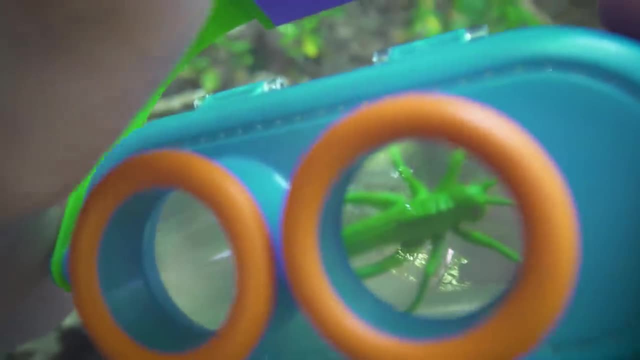 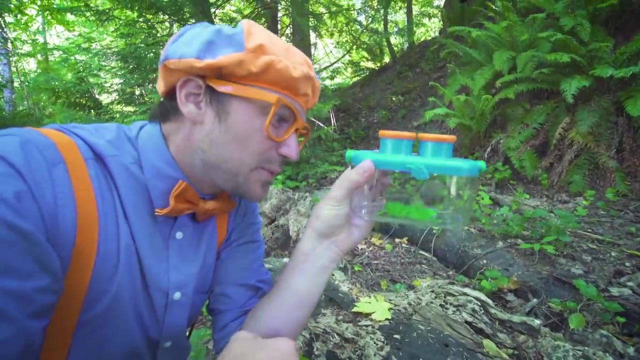 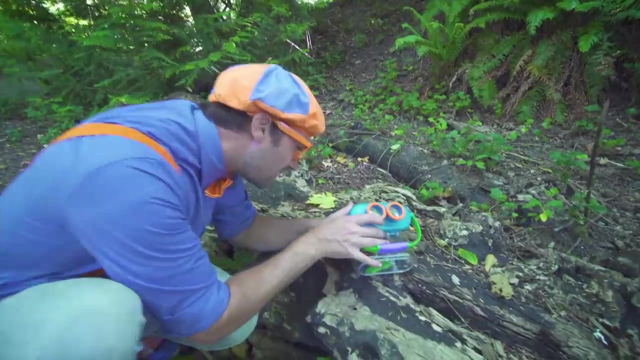 Whoa, And see it really close. Whoa, Check it out. Wow, Wow, What a beautiful little insect. Okay, we should probably let it back. Alright, grasshopper, Go ahead. Oh, Back to your home, you go. 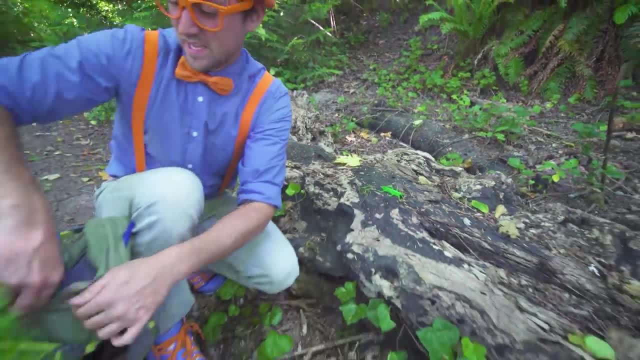 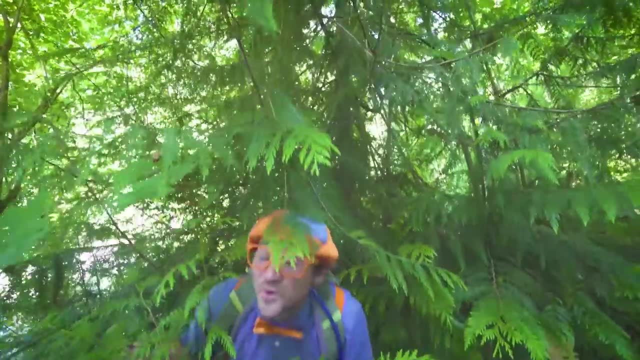 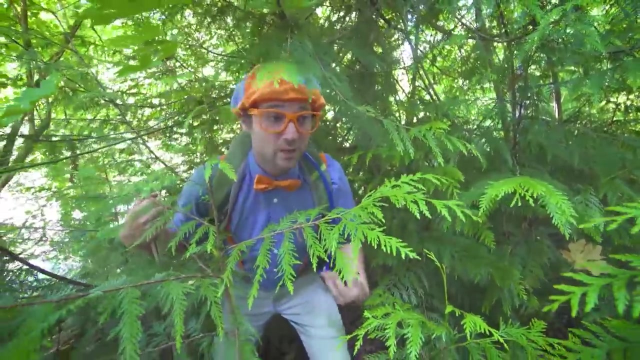 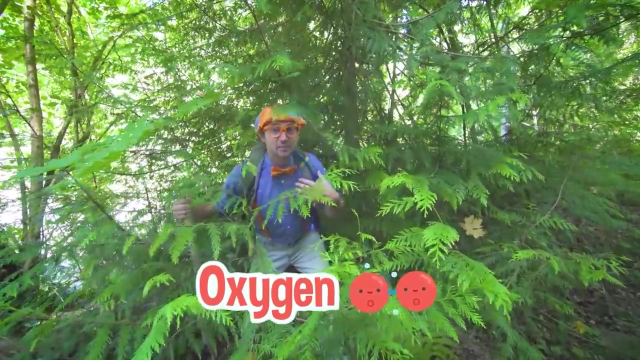 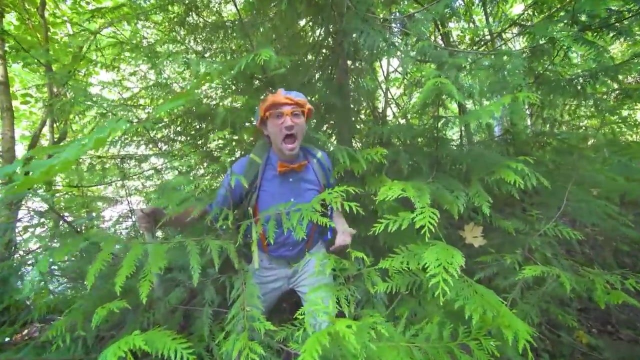 Alright, I'm going to put these back and continue on. See you later, I am getting so tired on my hike. When I breathe in, I breathe in oxygen And I breathe out carbon dioxide In oxygen, out carbon dioxide. But hey, Check this out. 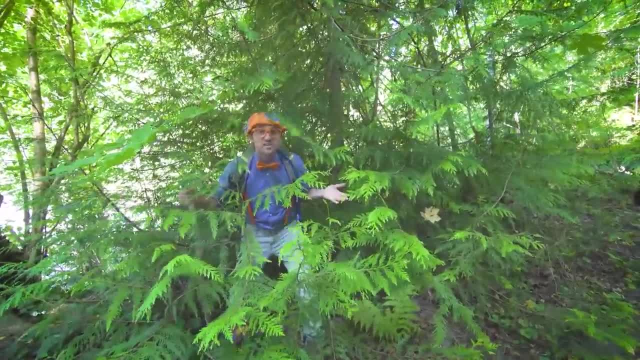 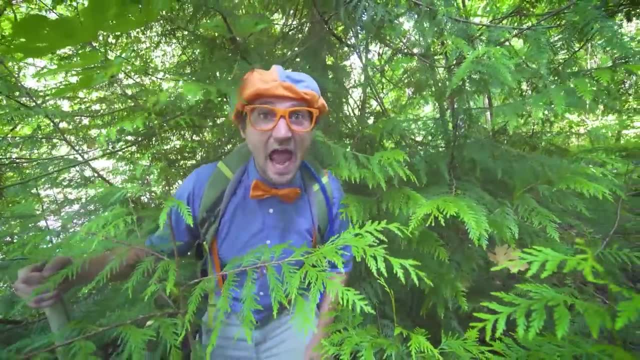 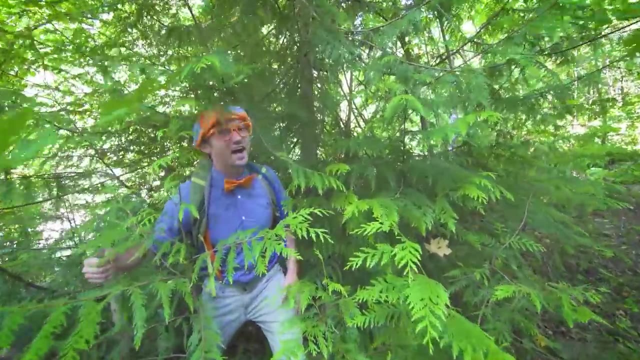 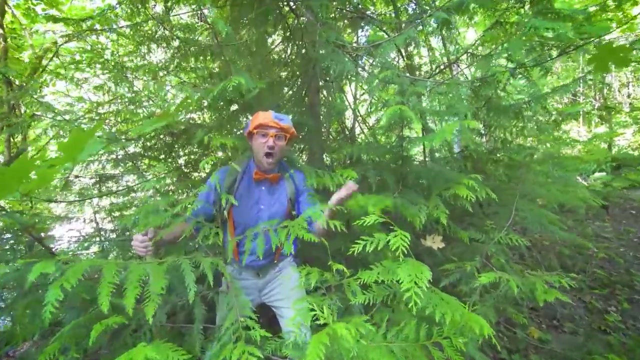 All these plants and trees and bushes and shrubs. they breathe in carbon dioxide and they breathe out oxygen. They breathe in carbon dioxide and they breathe out oxygen. Isn't that cool? Yeah, We're the opposite of them. We breathe out carbon dioxide. 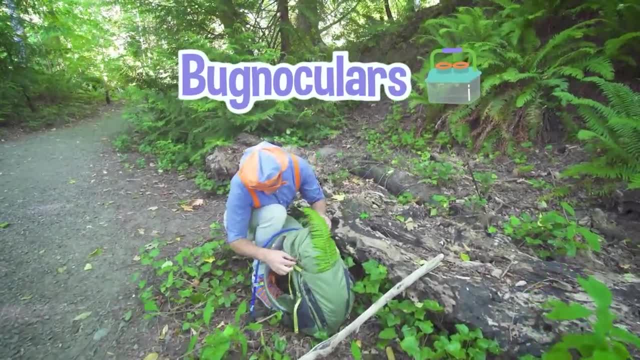 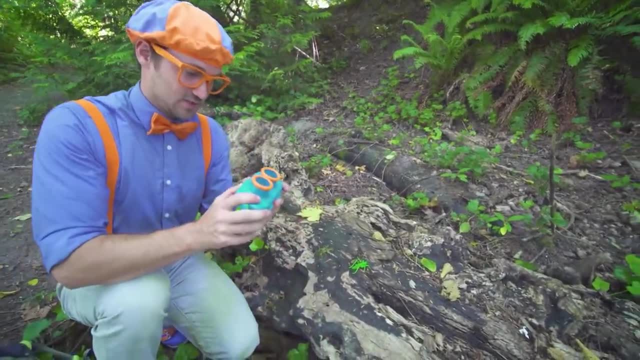 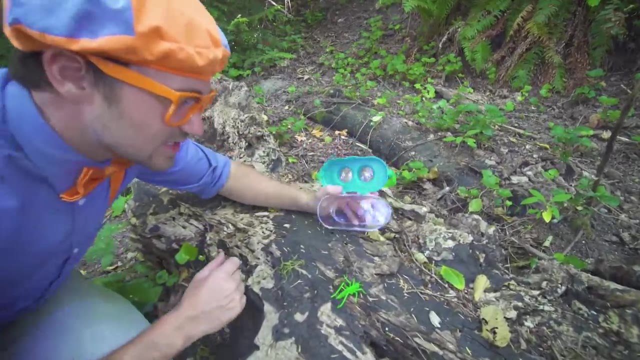 what are called bugnoculars. Let's see here. Bugnoculars are great to use to see bugs up close, So what we're gonna do is open them up. Here we go, And then let the grasshopper jump inside. There you go. 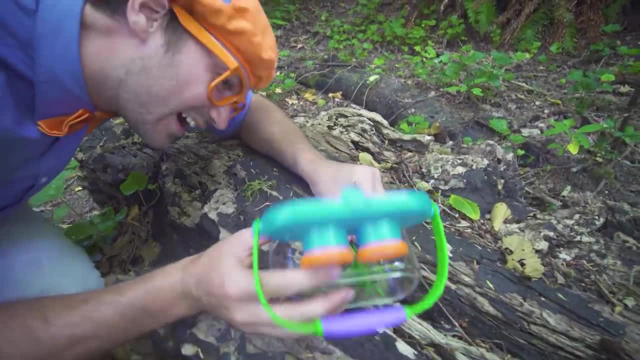 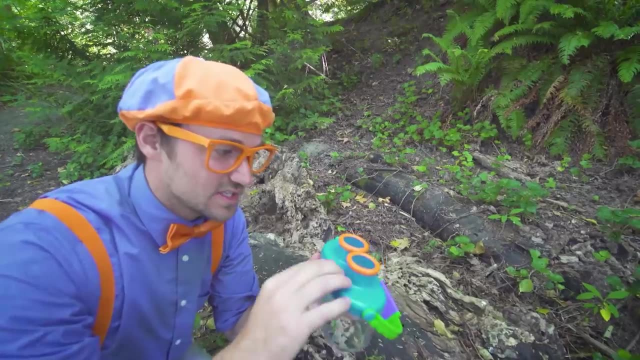 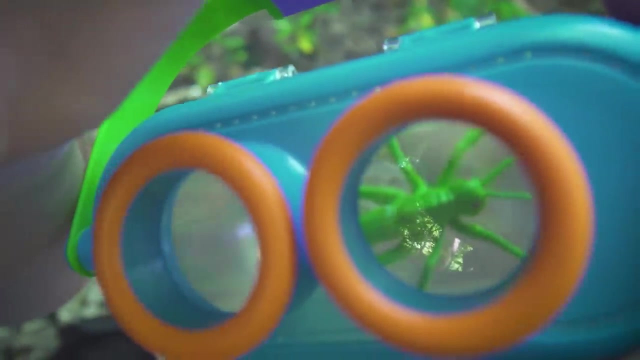 There you go, Just get right in there. Perfect. Wow, The grasshopper is inside now. So then, if I close this up, I can look through the eyepiece Whoa And see it really close. Check it out. 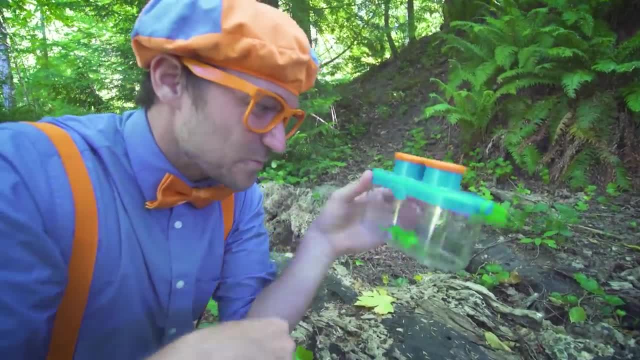 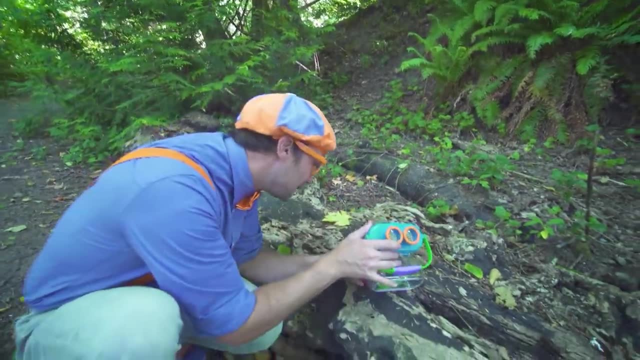 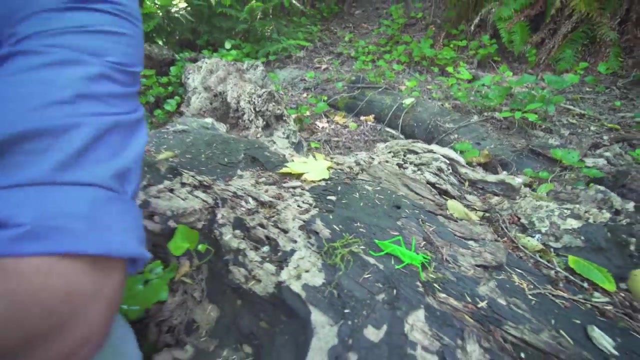 Wow, Wow, What a beautiful little insect. Okay, We should probably let it back, Alright, grasshopper, Go ahead. Oh, Back to your home, you go. Alright, I'm gonna put these back and continue on. See you later. 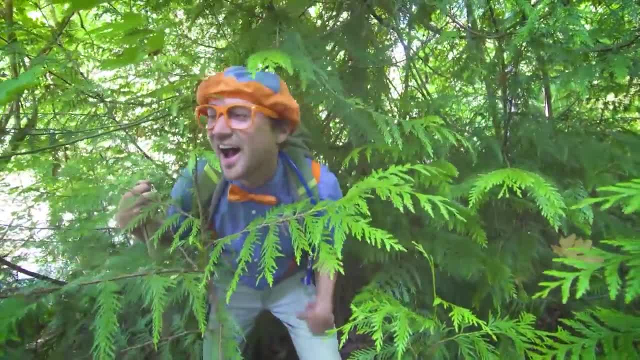 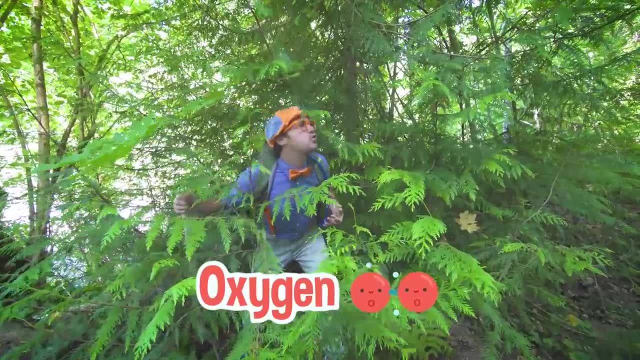 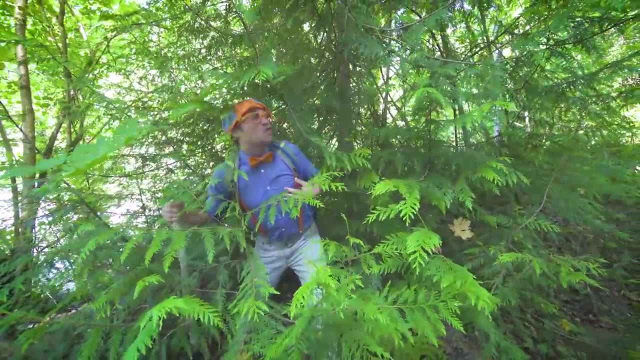 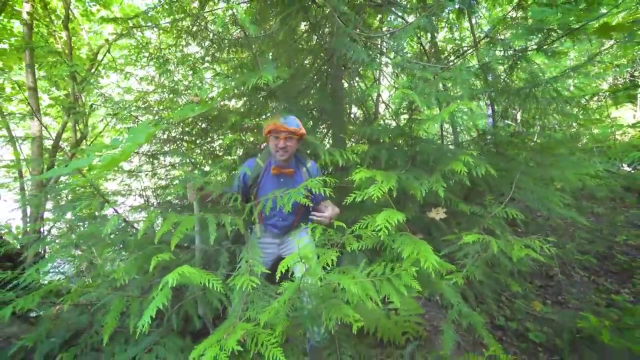 I am getting so tired on my hike. When I breathe in, I breathe in oxygen And I breathe out carbon dioxide In oxygen, out carbon dioxide. But hey, check this out, All these plants and trees and bushes and shrubs, they breathe. 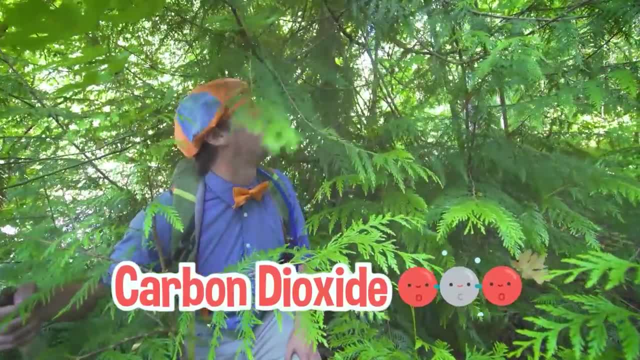 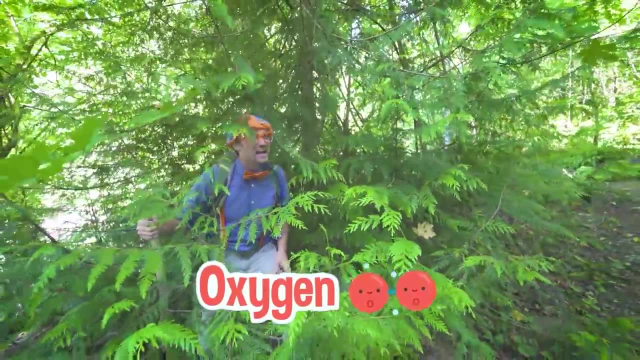 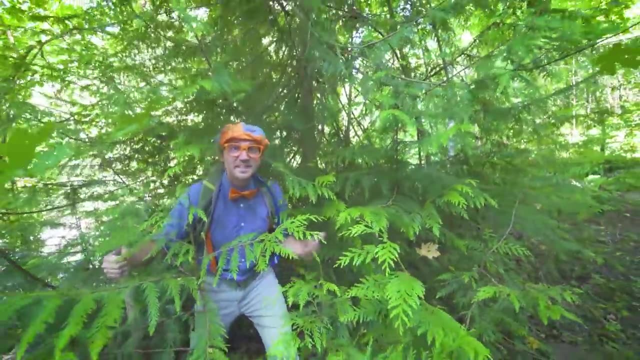 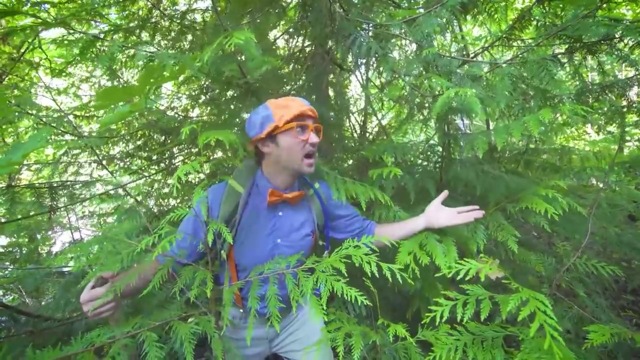 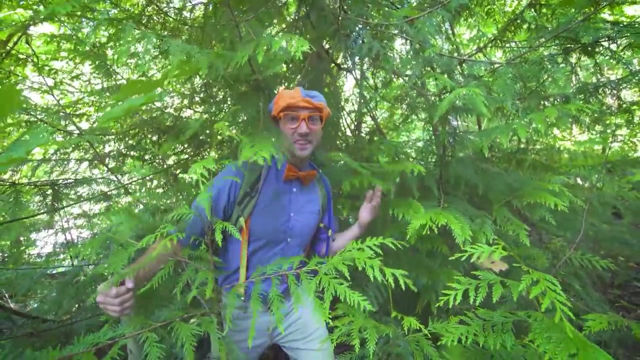 in carbon dioxide and they breathe out oxygen. They breathe in carbon dioxide and they breathe out oxygen. Isn't that cool? Yeah, We're the opposite of them. We breathe out carbon dioxide and that's what they breathe in, And then they breathe. 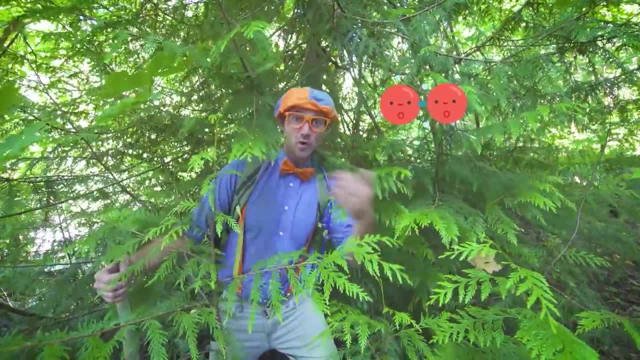 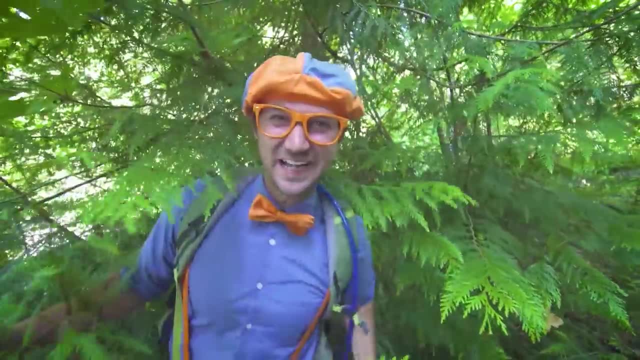 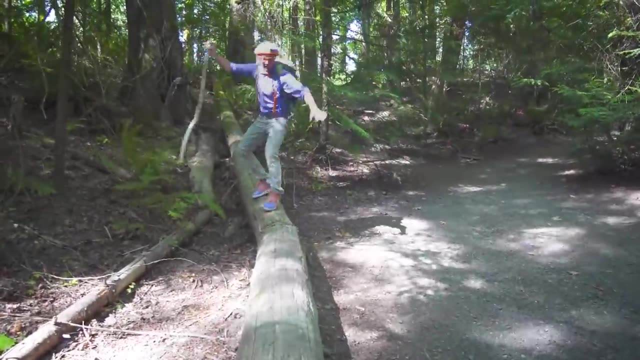 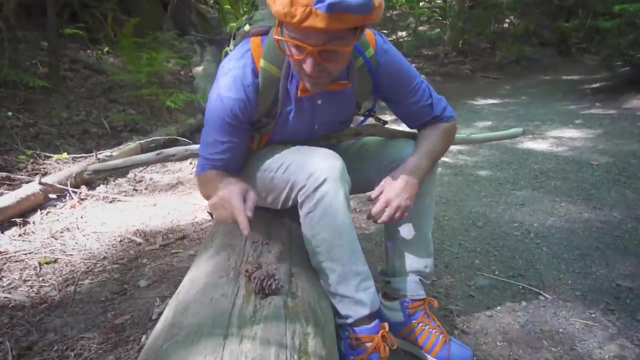 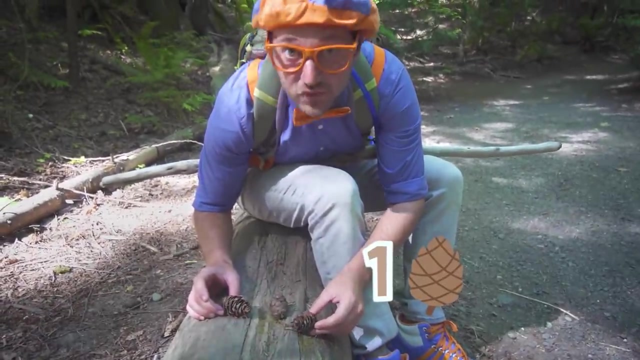 out oxygen and we breathe in oxygen. Yeah, We are a great team. Hey, Check it out. Do you see these? These are pine cones. How many pine cones do you see? One, two, three pine cones? Pine cones are so cool looking. 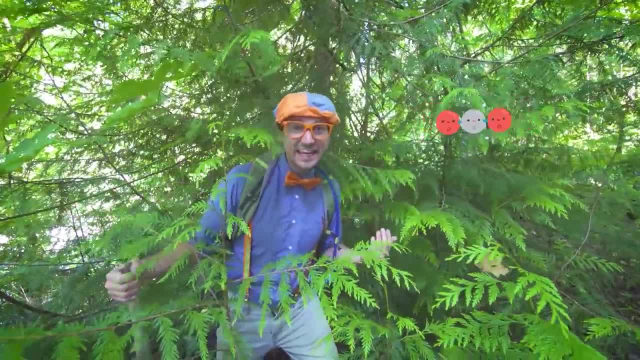 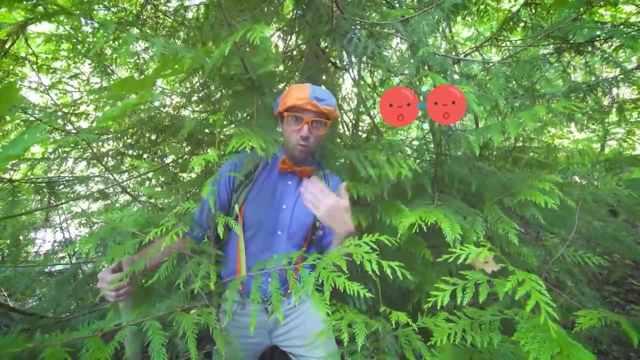 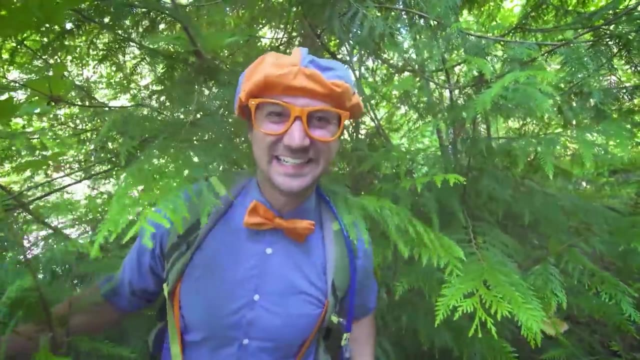 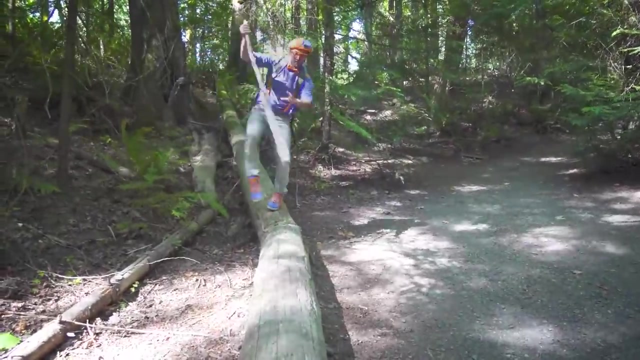 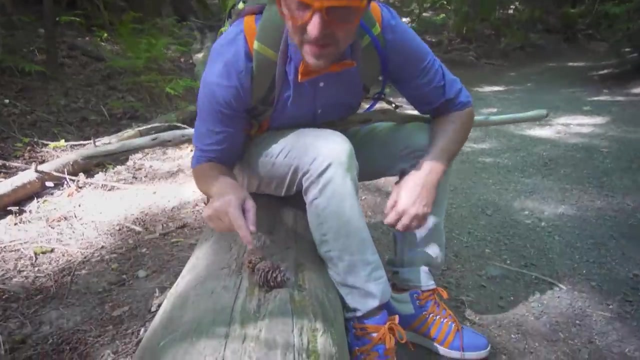 and that's what they breathe in, And then they breathe out oxygen And we breathe in oxygen. Yeah, We are a great team. Hey, Check it out. Do you see these Pinecones? How many pinecones do you see? 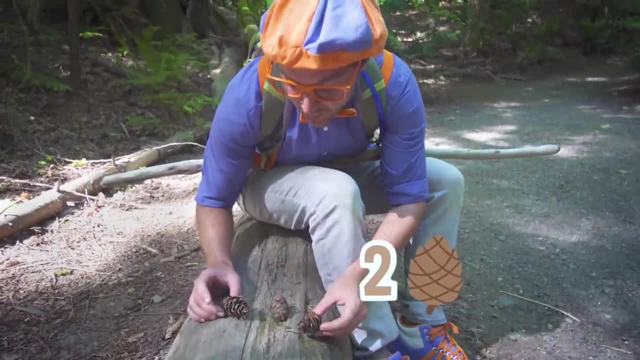 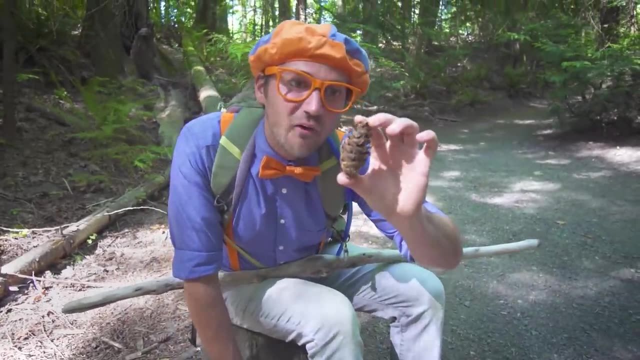 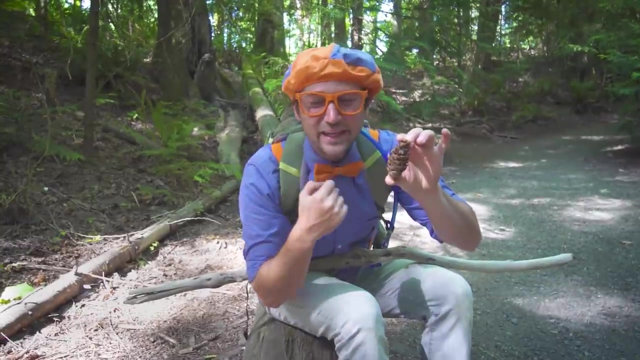 One, Two, Three pinecones. Pinecones are so cool looking, Wow. Hey, Chipmunks love pinecones because there's little seeds in there that they grab and then they eat Pinecone seeds. Okay, I am going to put this. 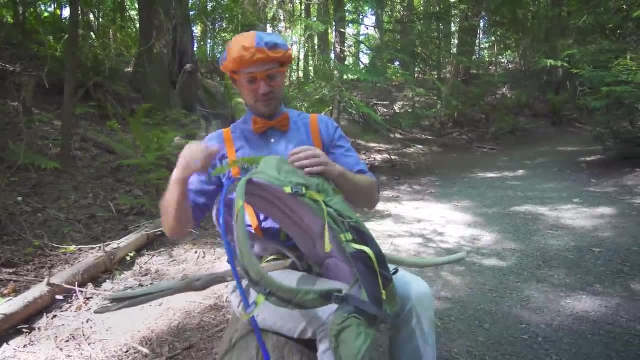 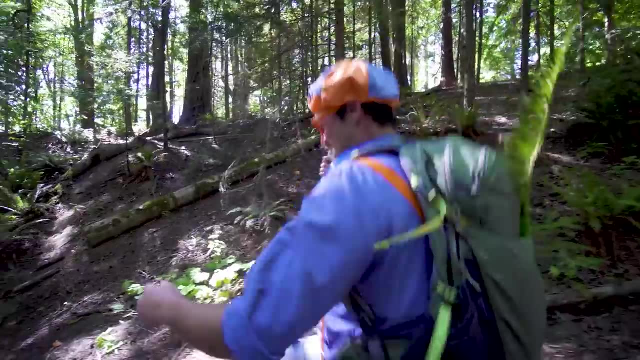 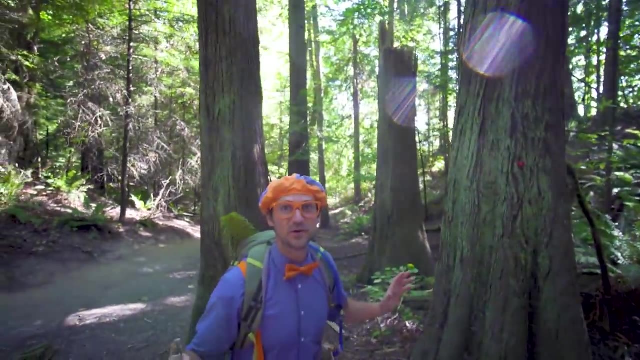 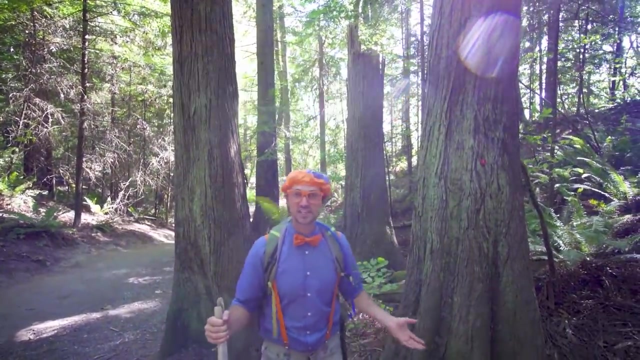 in my bag for later. Yeah, For that special something I was telling you about. Alright, Let's continue on. Woo, I spy something really cool. Let me tell you what it is. I spy a half of a tree, Do you see it? Yeah, 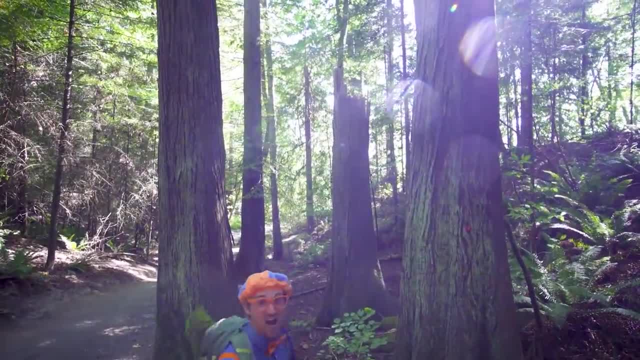 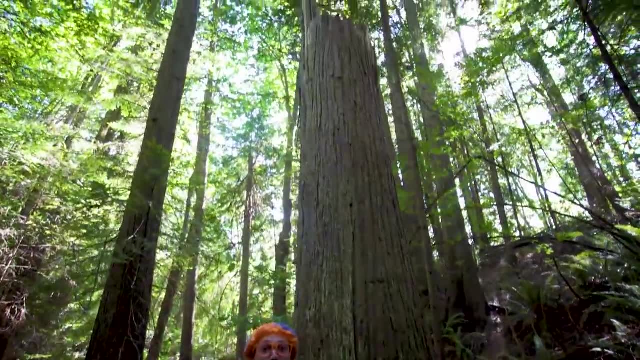 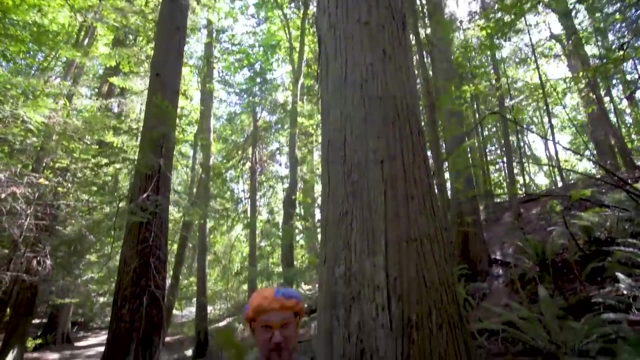 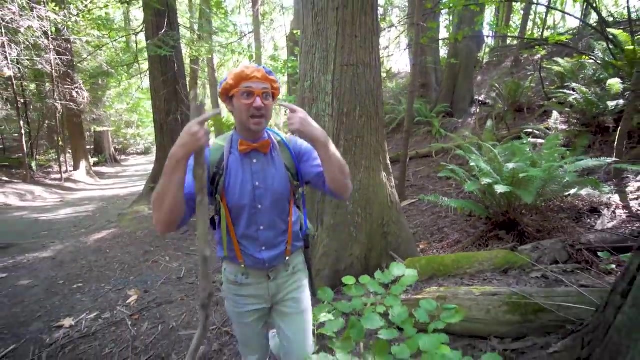 A half of a tree. Yeah, Check it out. This used to be a whole tree, Yeah, But now it's just a half of a tree. Haha, That's cool. Hey, That was actually really fun. Yeah, I got to see something. 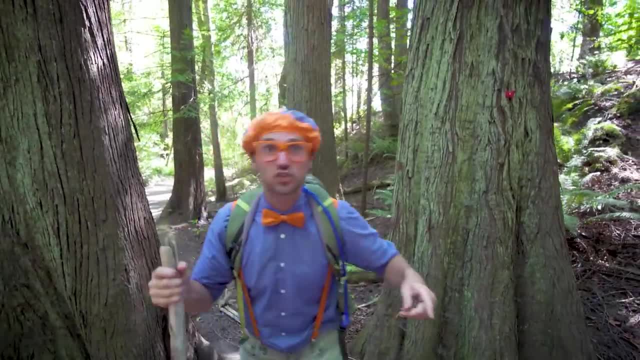 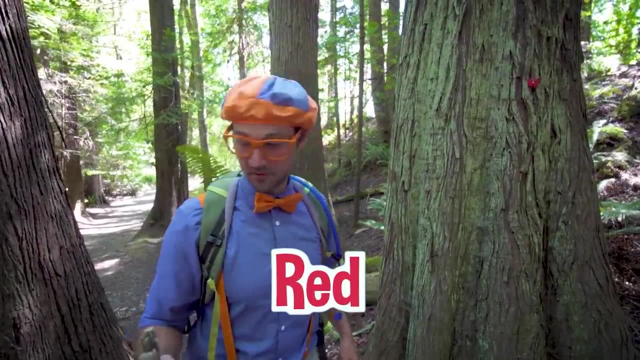 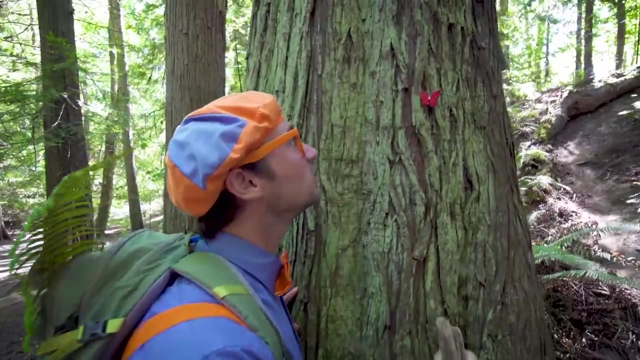 so I say: I spy it, and then you get to look and search and find it. Okay, I'll do another one. I spy something red, Do you see it? Oh yeah, Look. Wow, It's a butterfly, A red butterfly. 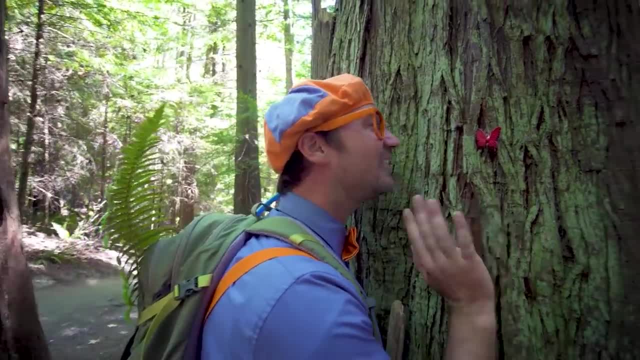 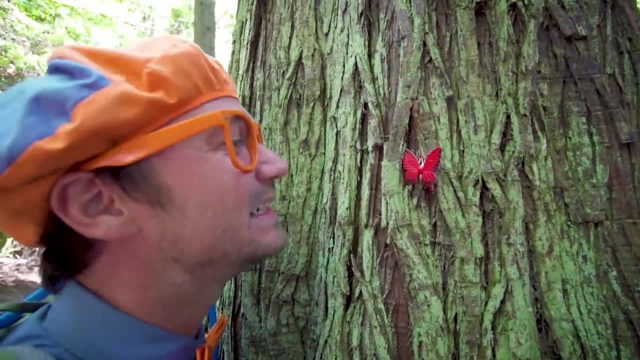 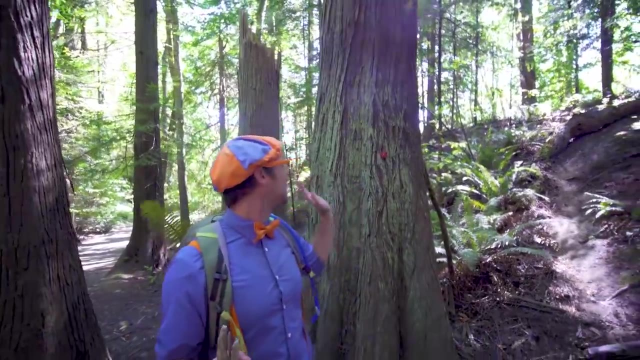 Wow, Hey, red butterfly, How's your day going? Haha, Are you having fun just hanging around? Haha, Butterflies are so beautiful. Okay, We'll just let it be Alright, Bye, bye, butterfly. Okay, We should probably get. 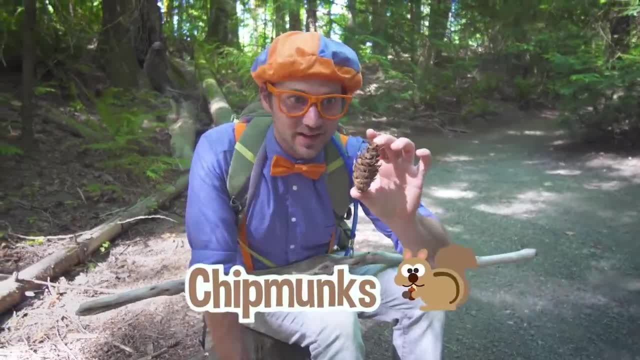 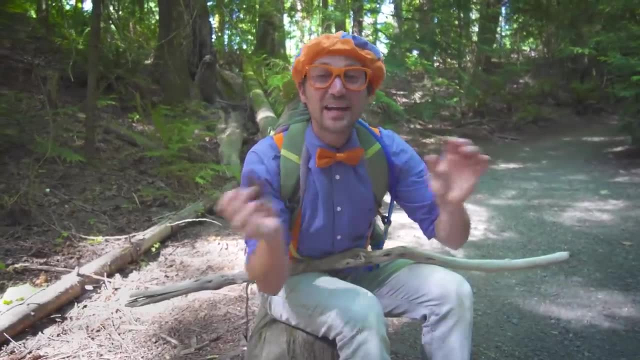 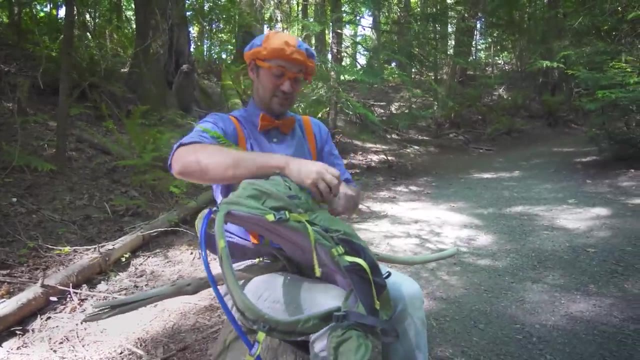 Wow, Hey, Chipmunks love pine cones because there's little seeds in there that they grab and then they eat Pine cone seeds. Okay, I'm going to put this in my bag for later. Yeah, For that special something that I was telling. 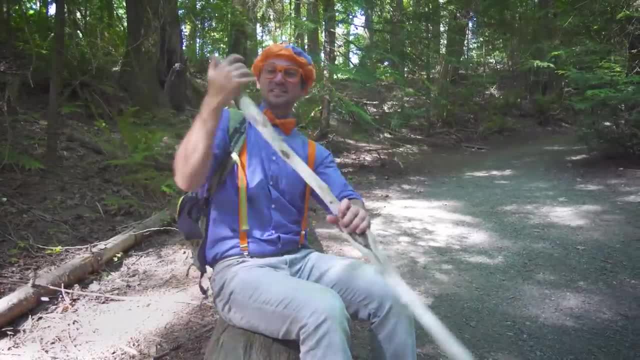 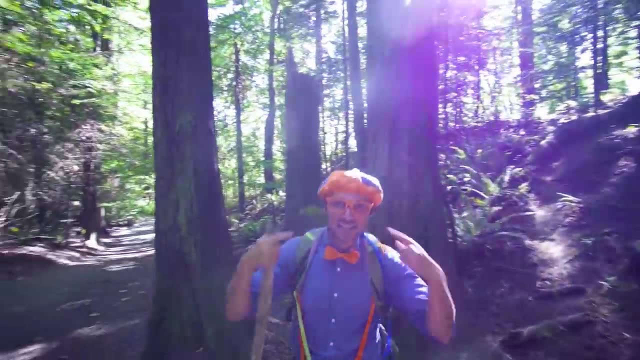 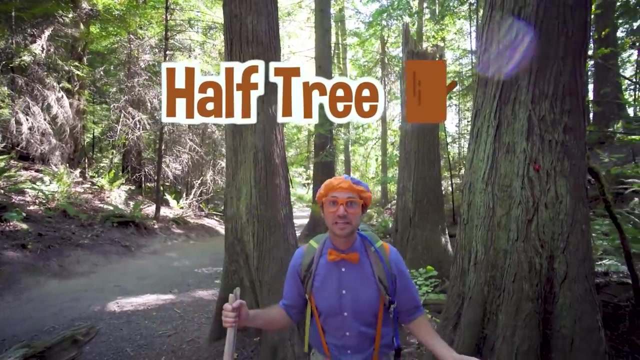 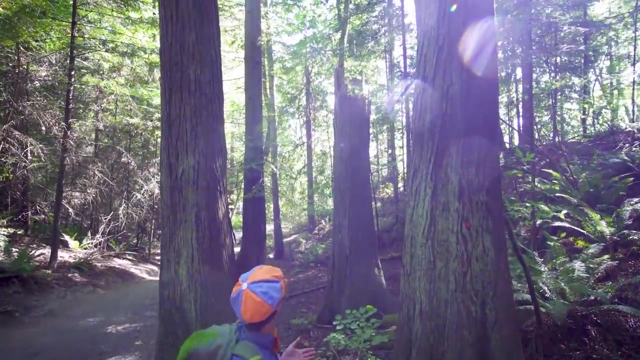 you about. Alright, Let's continue on. Woo Woo, I spy something really cool. Let me tell you what it is. I spy a half of a tree, Do you see it? Yeah, A half of a tree. Yeah, 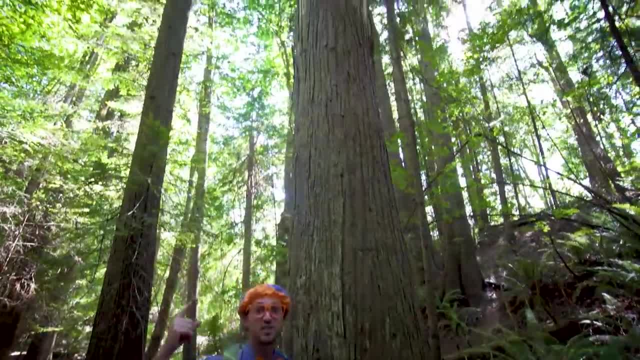 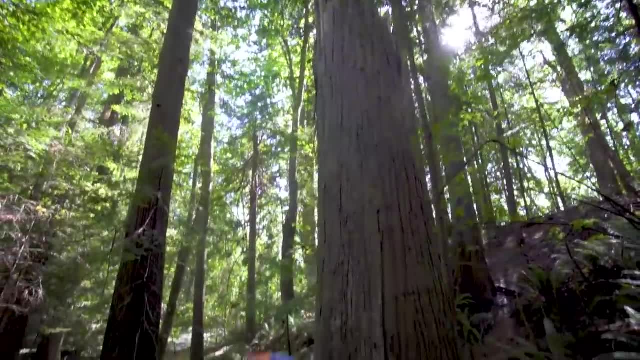 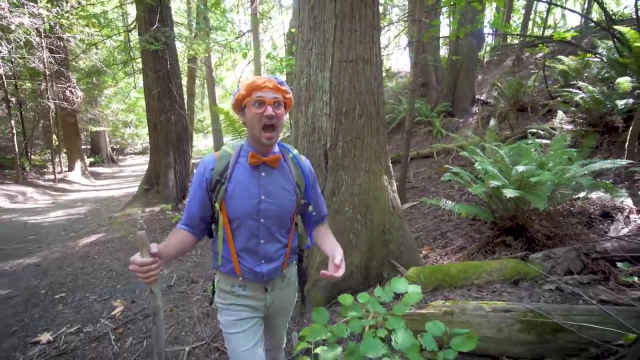 Check it out. This used to be a whole tree, Yeah, But now it's just a half of a tree, Haha. Oh, That's cool. Hey, That was actually really fun. Yeah, I got to see something. So I say: 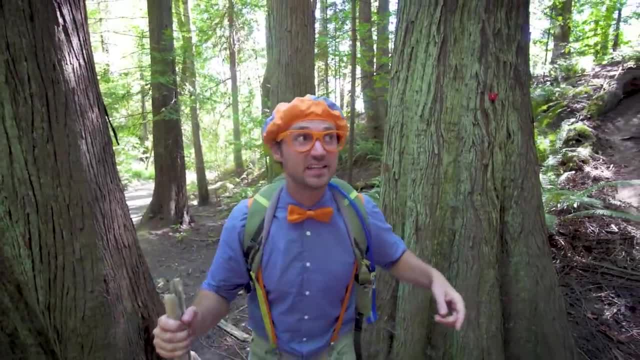 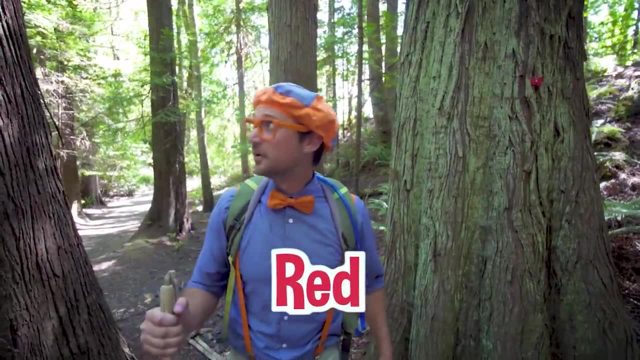 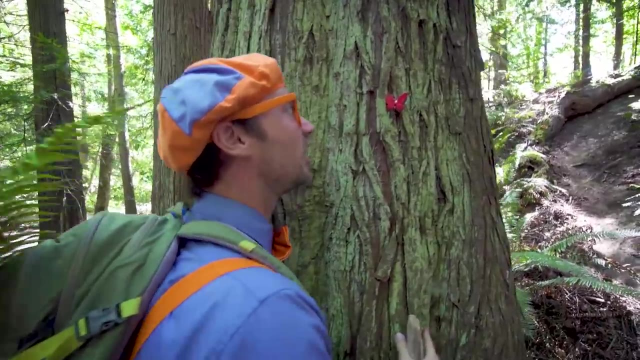 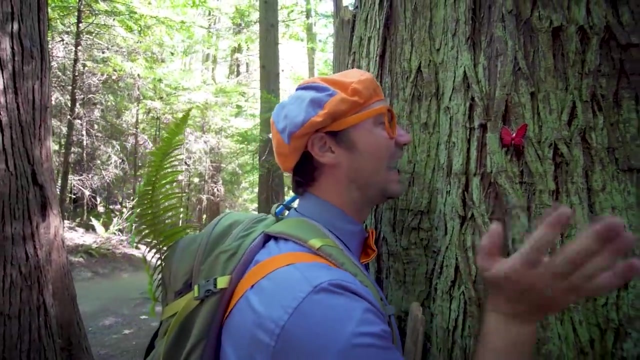 I spy it and then you get to look and search and find it. Okay, I'll do another one. I spy something red, Do you see it? Oh, Yeah, Look, Wow, It's a butterfly, A red butterfly. Wow, Hey, red butterfly. 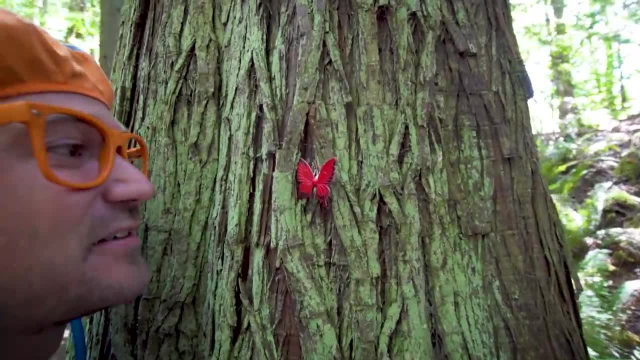 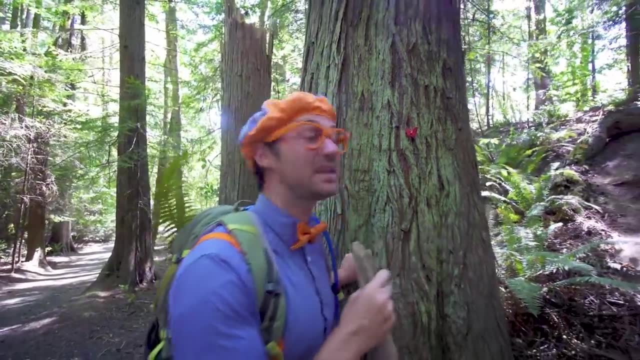 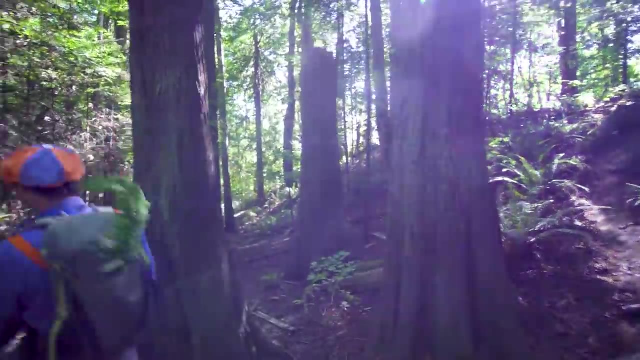 How's your day going? Haha, Are you having fun just hanging around? Butterflies are so beautiful, Wow, Okay, We'll just let it be Alright. Bye, bye, butterfly. Okay, We should probably get continuing on, Haha. 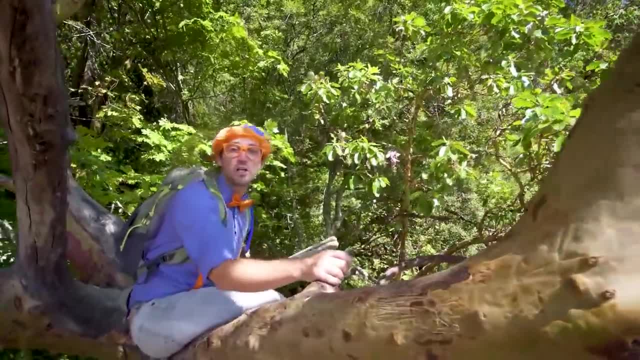 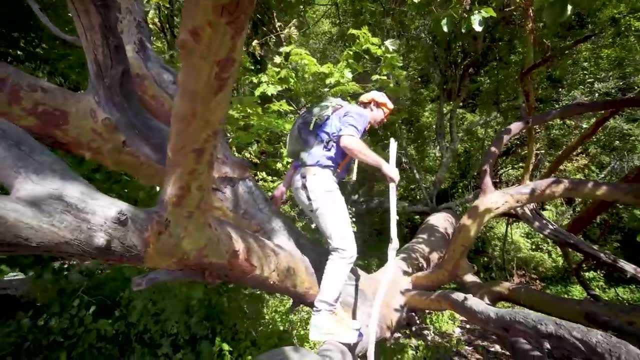 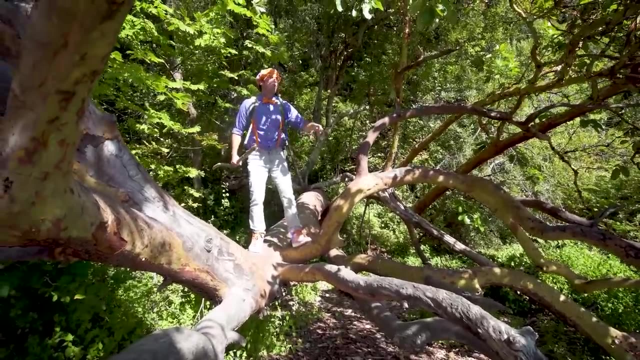 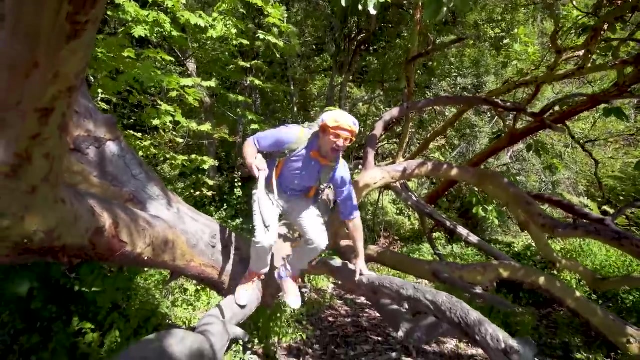 Hey, Check it out. I just found a really good tree to climb on. Wow, You have to be very careful when you're climbing a tree. Wow, Wow, Wow. What's that? I spy something. Haha, I spy the beach. 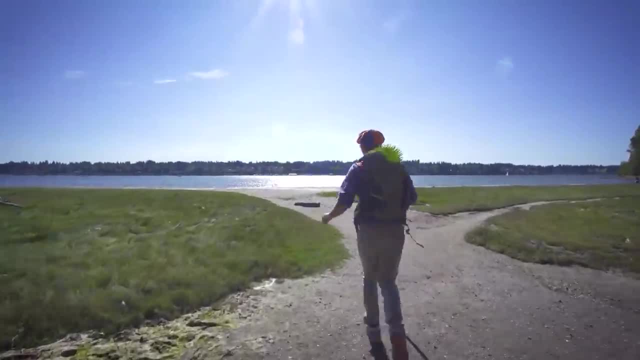 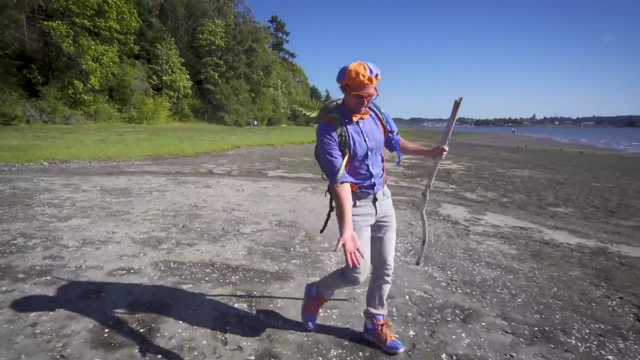 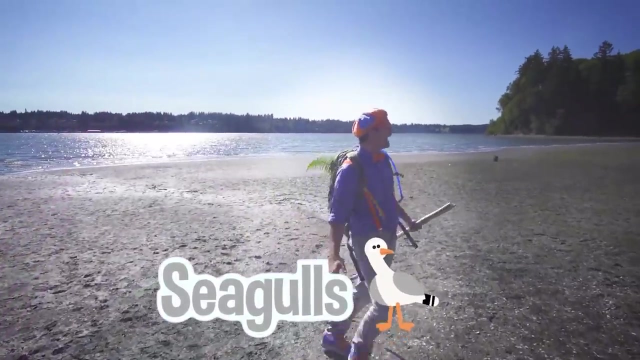 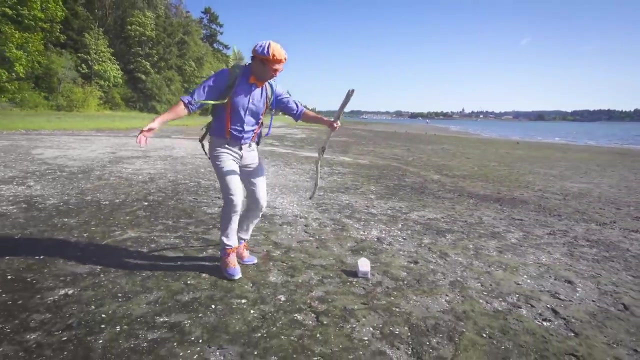 Wow, Wow, I love the beach, Wow, I love the sand, Yeah, And I also love the seagulls, Yeah, Wow, I really enjoy hanging out at the beach all day long, Haha, Wow, Wait a second, What is? 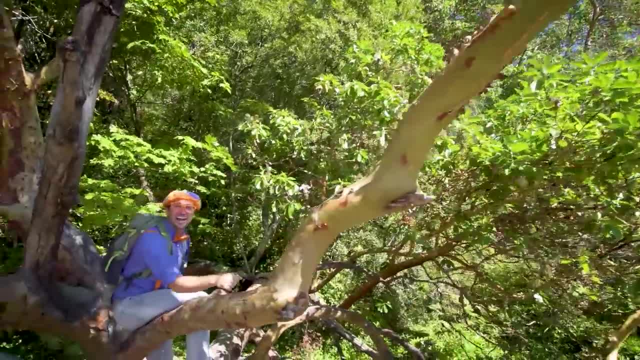 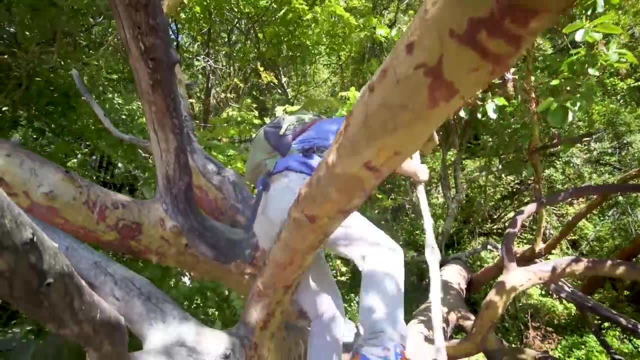 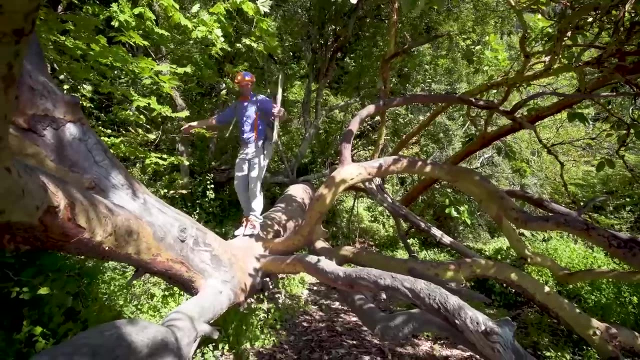 continuing on. Haha, Hey, Check it out. I just found a really good tree to climb on. Whoa Wee. You have to be very careful when you're climbing a tree. Whoa, Whoa, Haha. 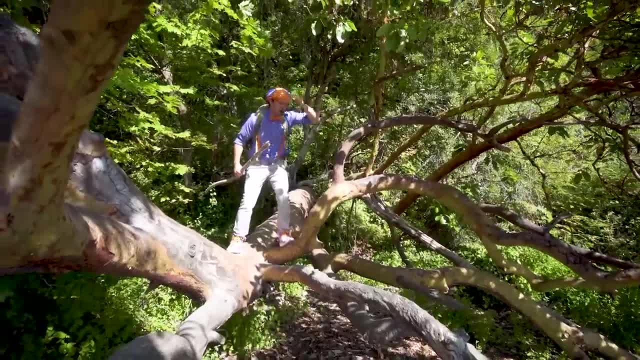 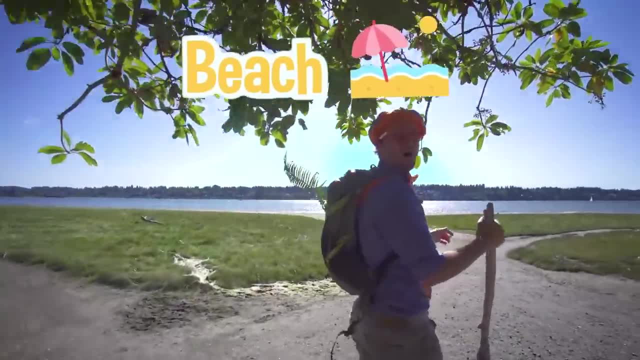 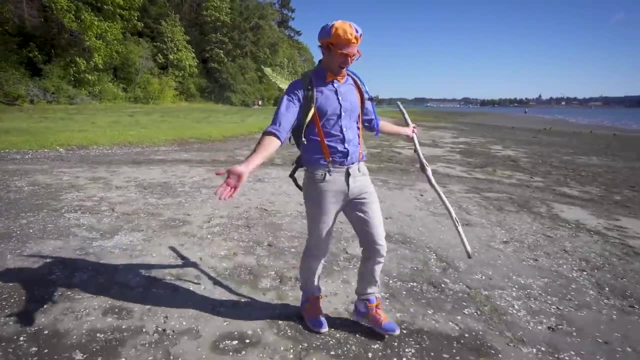 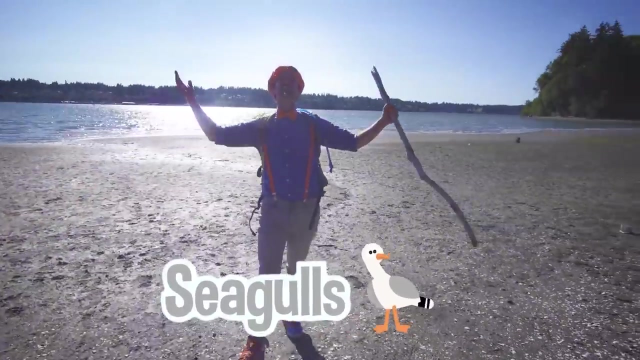 Whoa, What's that? I spy something, Haha. I spy the beach. Whoa, Whoa, I love the beach, I love the sand, Yeah, And I also love the seagulls, Yeah, Wow, I really enjoy hanging out at the beach. 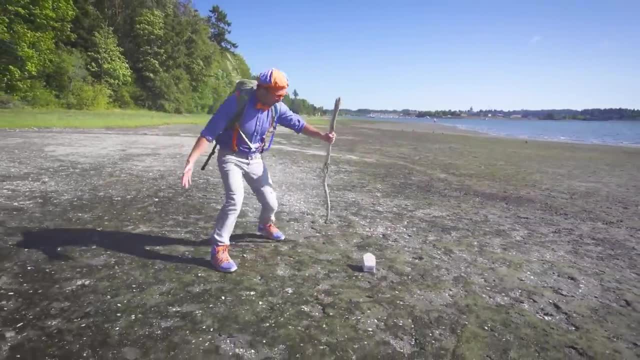 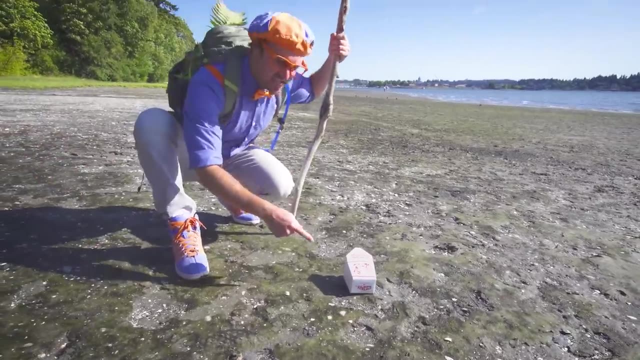 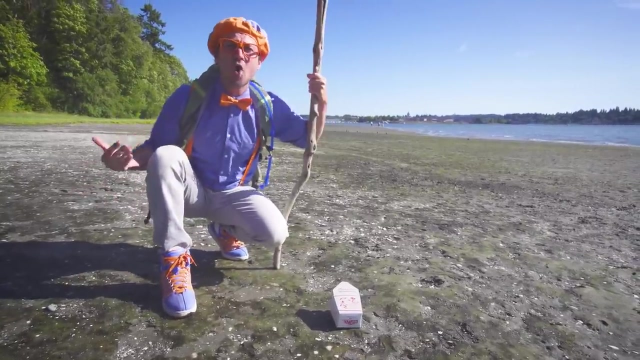 all day long. Haha, Whoa, Wait a second. What is this? This isn't supposed to be here. This is garbage. Boo, Who left this here? I don't even know. I am so mad This beach is home to. 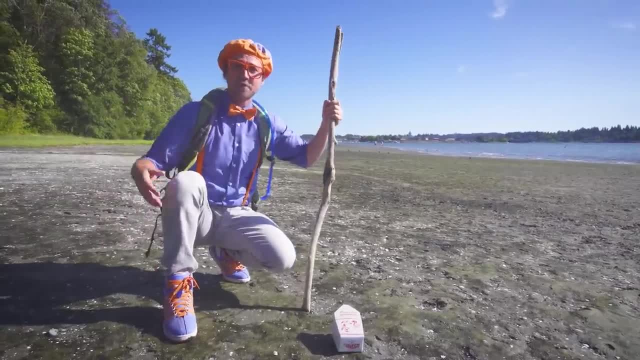 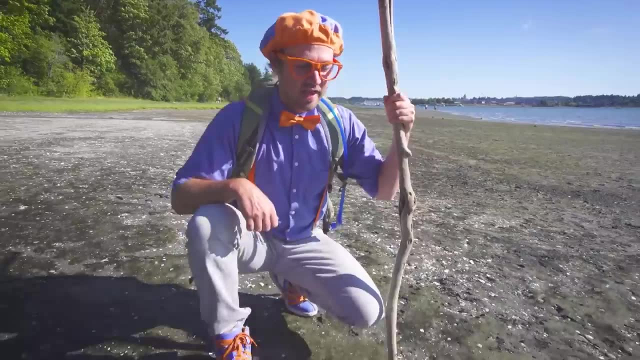 so many critters And it is our duty to keep Earth nice and clean. Yeah, Would you want your home dirty? No, I sure wouldn't. Hey, I have an idea. Why don't you and I clean up the beach? 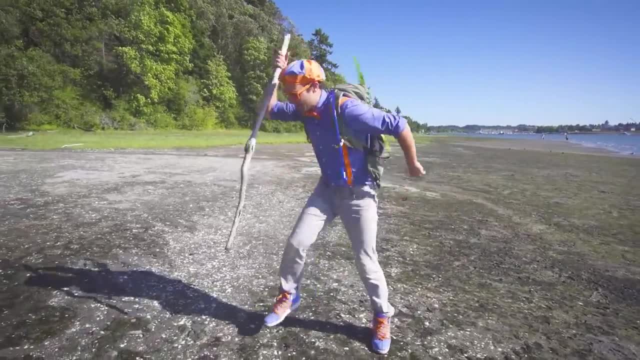 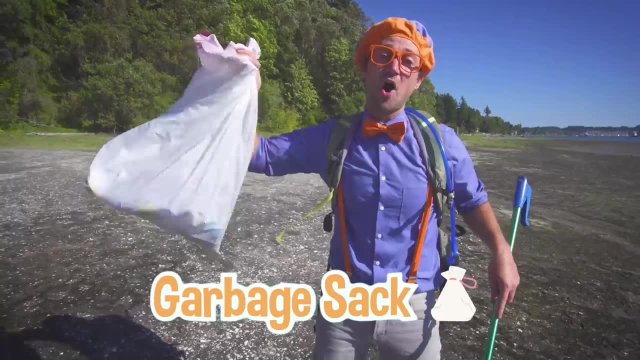 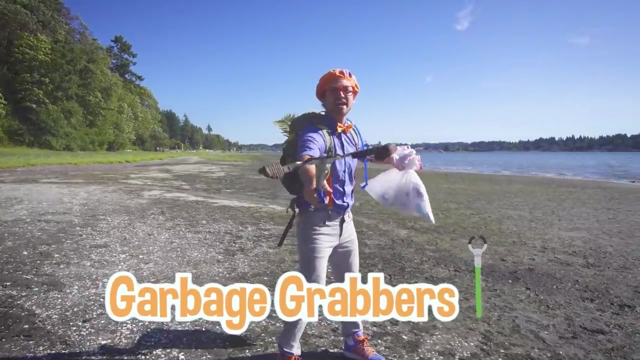 Like fun Ready. Three, Two, One. Whoa, Check it out. I have my garbage sack. Yeah, I'll put all the garbage in here. And then I have, Haha, My garbage grabbers. Yeah, It's like a claw. 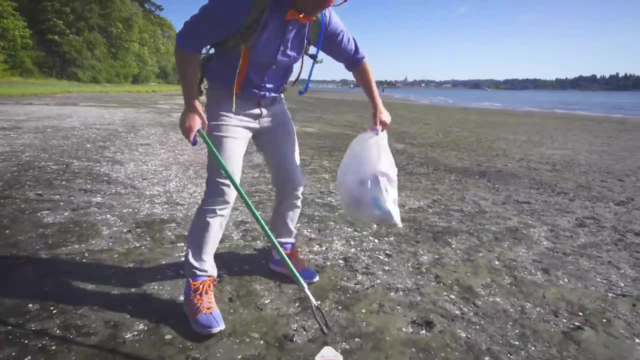 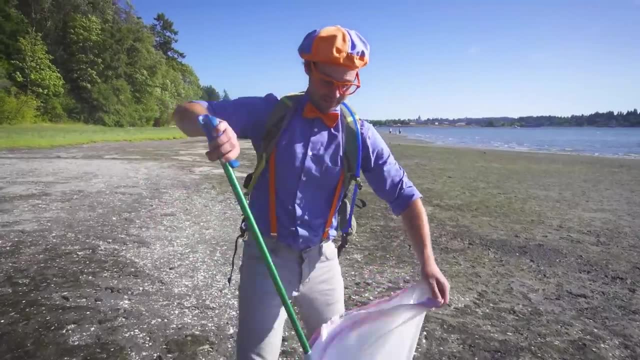 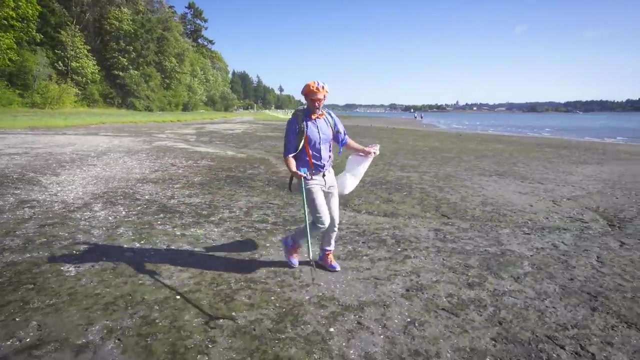 Haha, Alright, Let's pick this piece up. Alright, I'm using these grabbers because I definitely don't want to touch this. I have no idea where that was before. Alright, Haha, Here we go. Okay, I see a shell. That should be there. 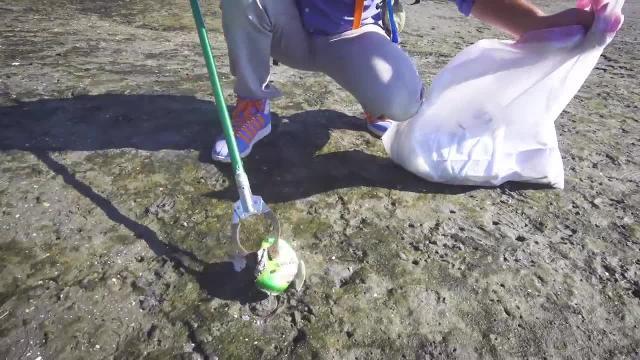 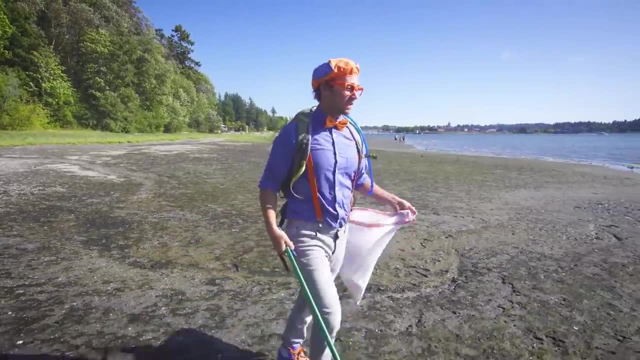 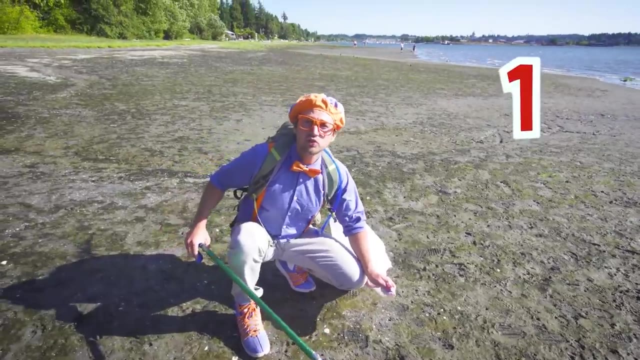 Oh, This should not be here. This looks like a soda can. Yeah, A pop can. Alright, Put it in there. Perfect, We collected two pieces of garbage. Wait a second, Here's another one. One, Two, Three. 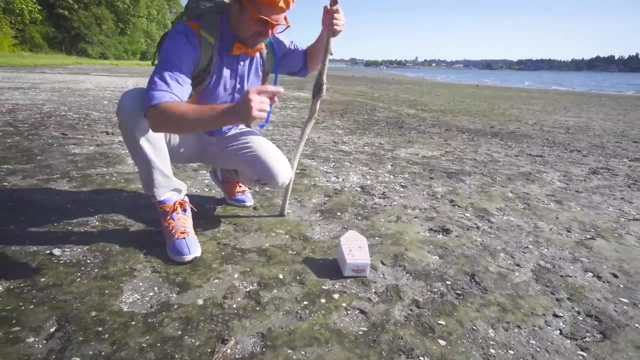 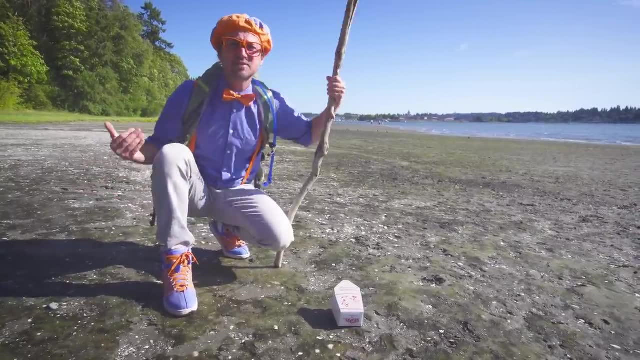 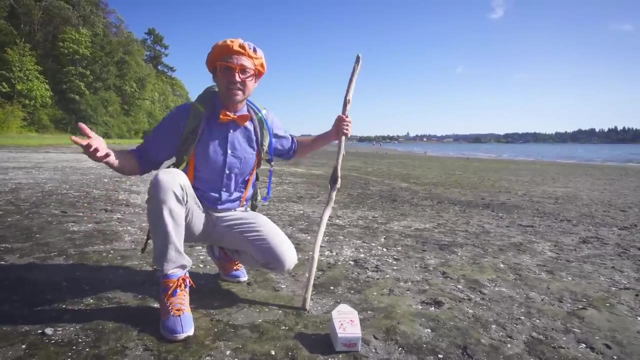 this. This isn't supposed to be here. This is garbage. Boo. Who left this here? I don't even know. I am so mad. This beach is home to so many critters and it is our duty to keep earth nice and clean. 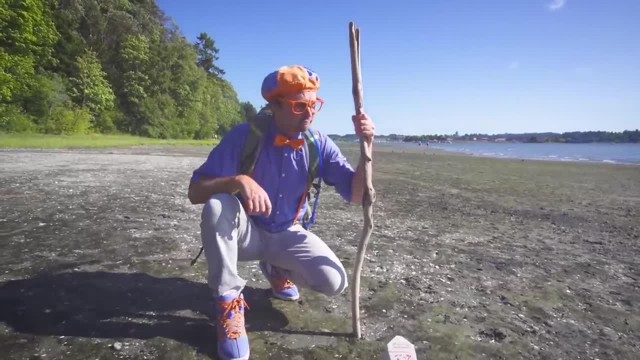 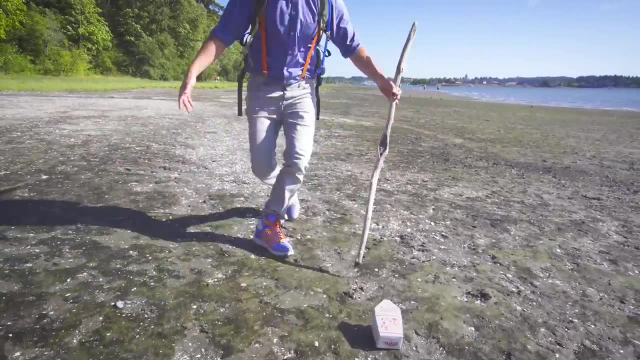 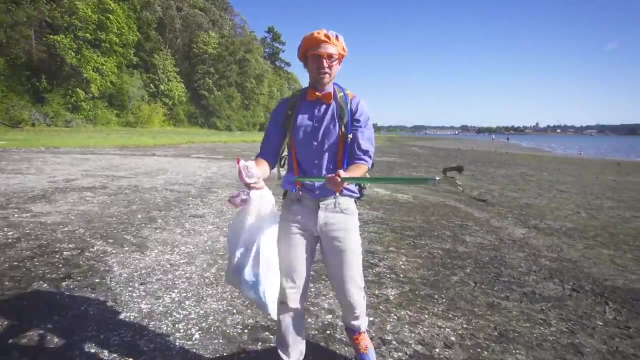 Yeah, Would you want your home dirty? No, I sure wouldn't. Hey, I have an idea. Why don't you and I clean up the beach? That sounds like fun. Ready. Three, two, one. Wow, Check it out, I have my garbage. 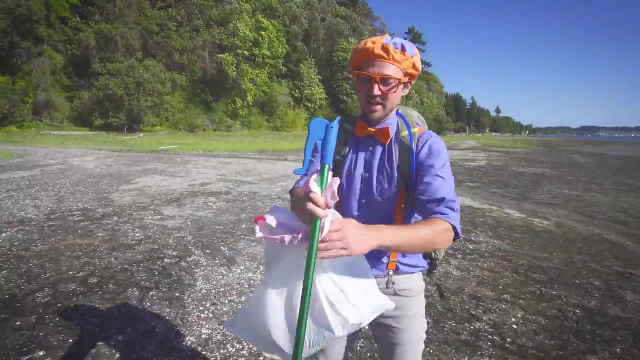 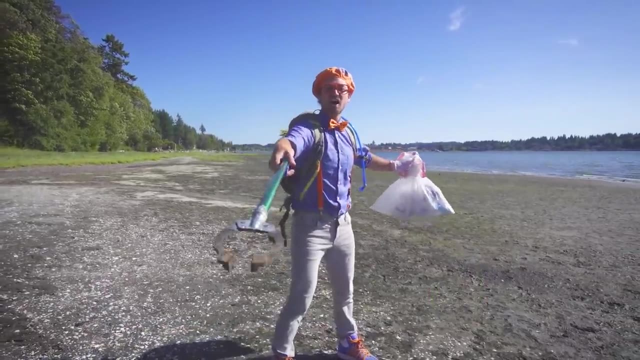 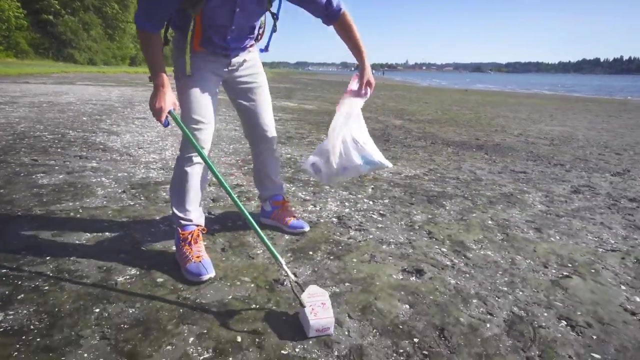 sack. Yeah, I'll put all the garbage in here. And then I have my garbage grabbers. Yeah, It's like a claw. All right, Let's pick this piece up. All right, I'm using these grabbers because I definitely don't want to. 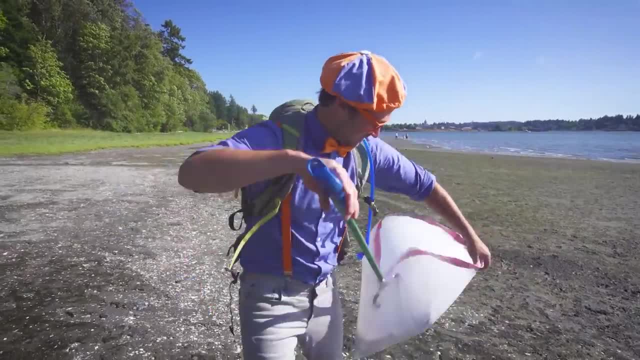 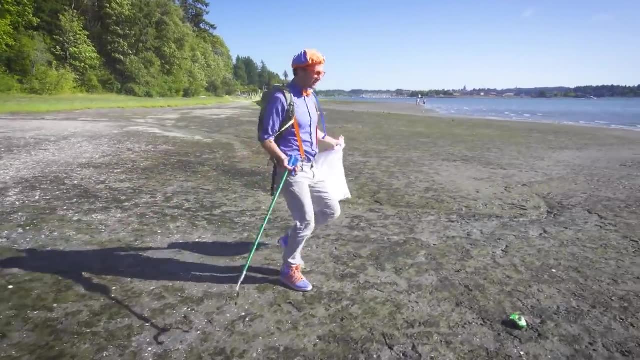 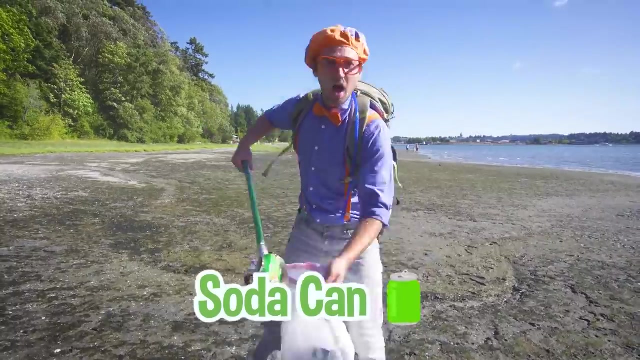 touch this. I have no idea where that was before. All right, Here we go. Okay, I see a shell. That should be there. Oh, This should not be here. This looks like a soda. can, Yeah, A pop? can, All right, Put it. 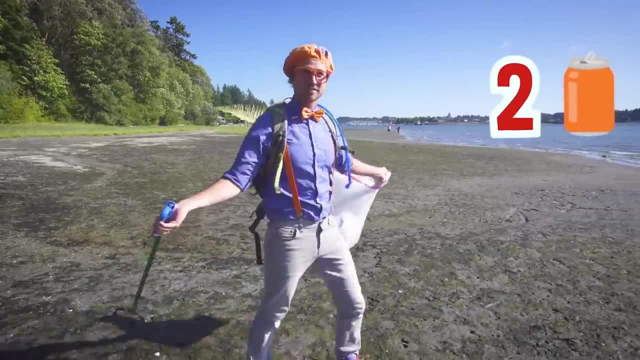 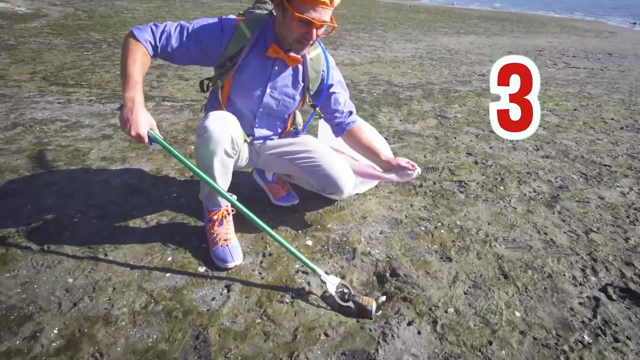 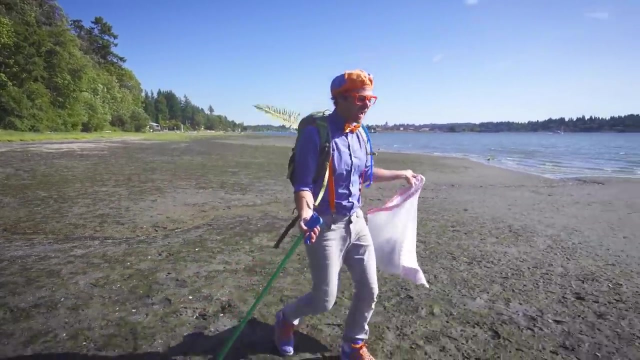 in there. Perfect, We collected two pieces of garbage. Wait a second. Here's another one. One, two, three- Our third piece of garbage. There we go. I am so happy that we're cleaning up this beach. Here's another. 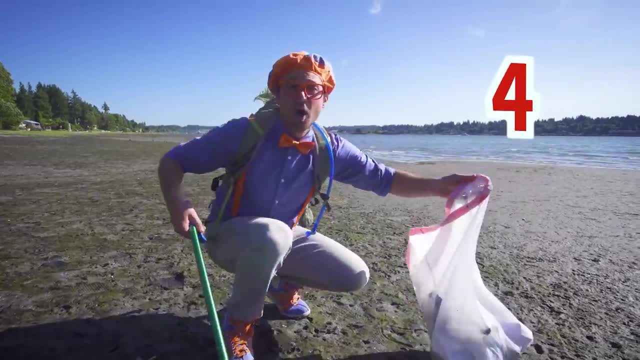 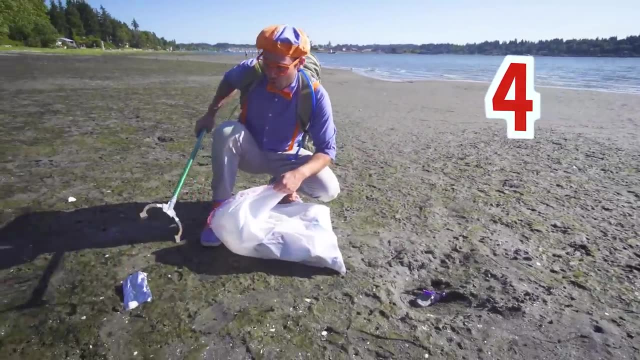 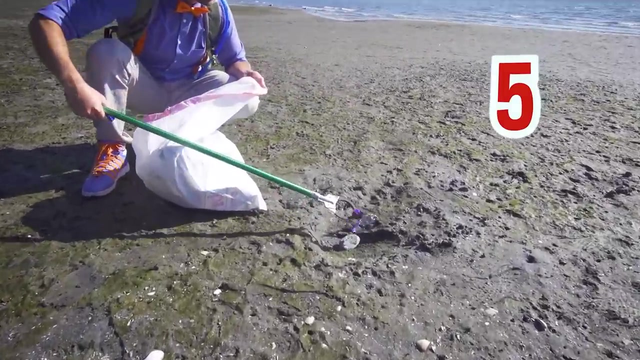 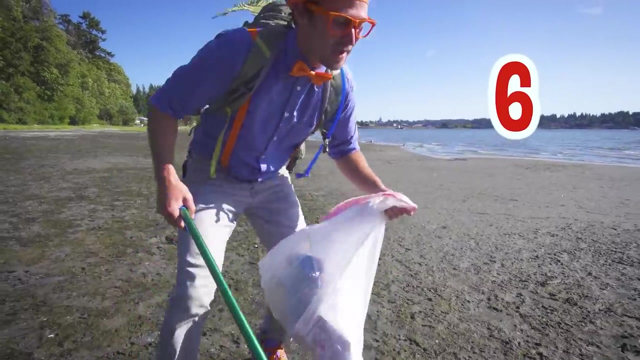 One, two, three, four- The fourth piece of trash is in here- Two more One, two, three, four, five. Right here, Yeah, Six. We collected six pieces of trash. Good job, But we're not done yet. 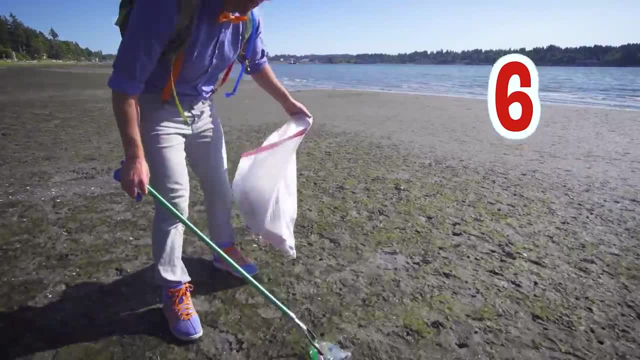 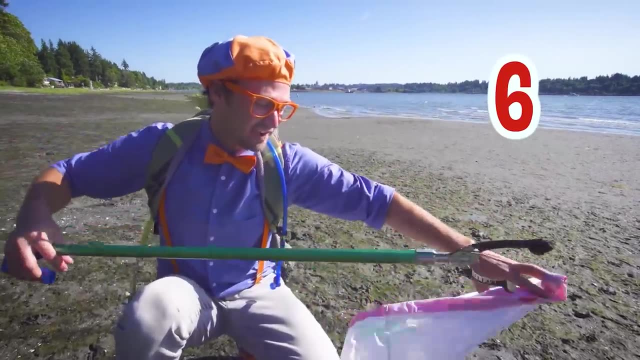 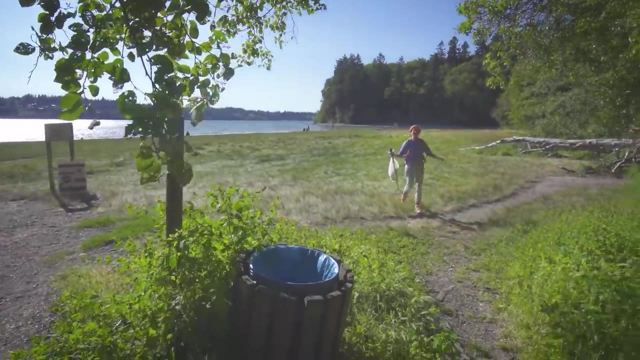 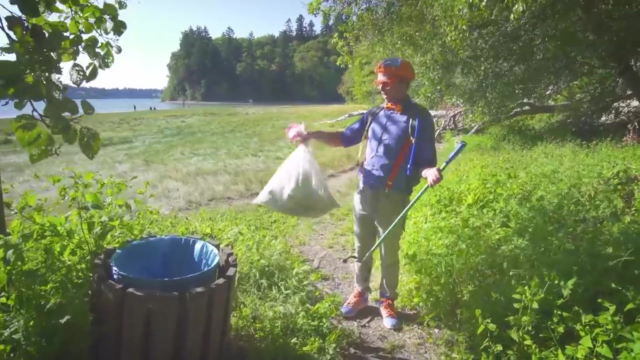 This beach is so dirty. Here's the last piece. All right, One, two, three, four, five, six, seven pieces of trash. Good job, That was so much fun cleaning up the beach with you. All right, I'm going to put this in the trash. 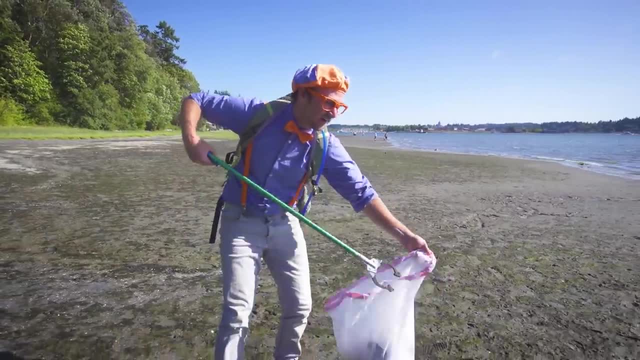 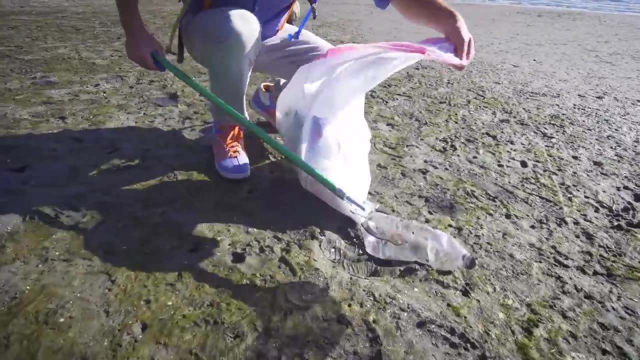 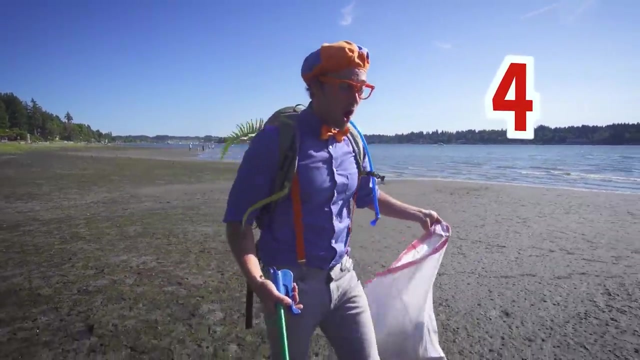 Our third piece of garbage. There we go. Haha, I am so happy that we're cleaning up this beach. Here's another One, Two, Three, Four. The fourth piece of trash is in here. Two more One, Two, Three. 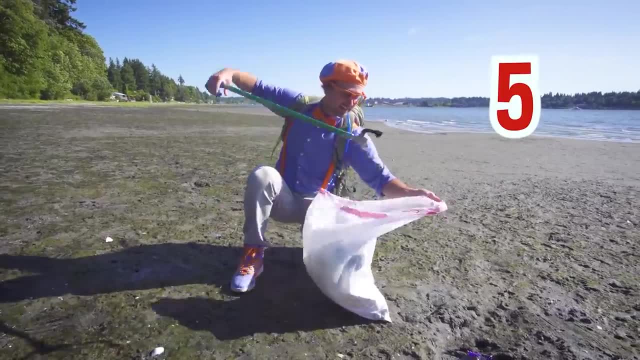 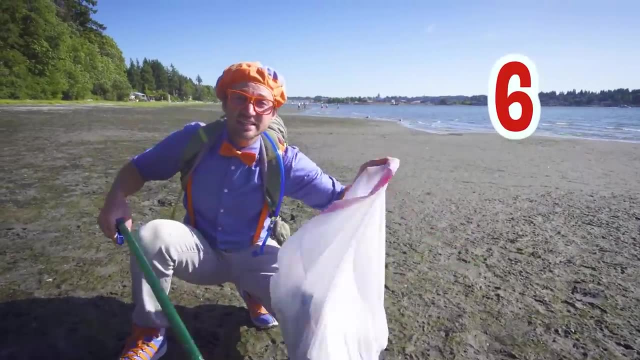 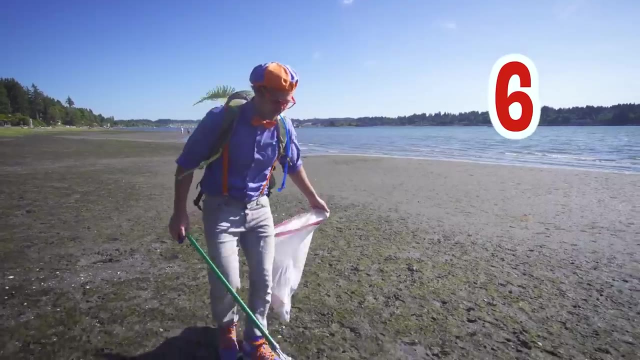 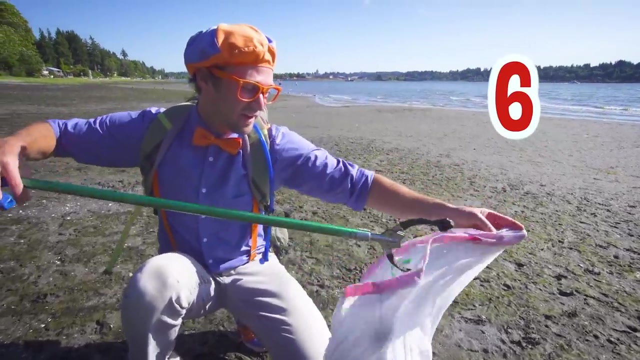 Four, Five, Right here, Yeah, Six. We collected six pieces of trash. Good job, But we're not done yet. This beach is so dirty. Here's the last piece, Alright, One, Two, Three, Four, Five, Six. 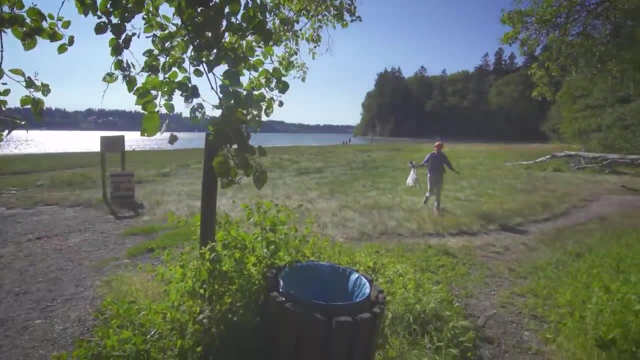 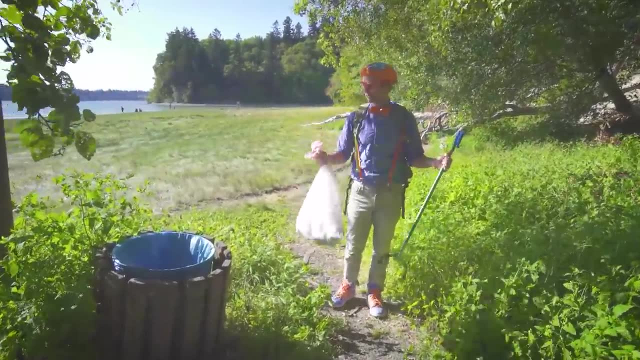 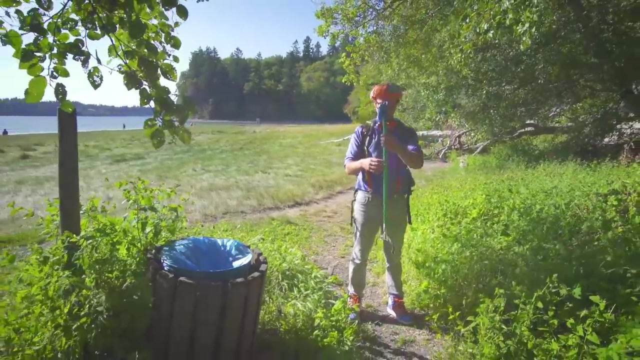 Seven pieces of trash- Good job. Wow, That was so much fun cleaning up the beach with you. Alright, I'm going to put this in the trash can. Bye-bye garbage, Haha, Good job. Well, I should probably get my hiking stick back. 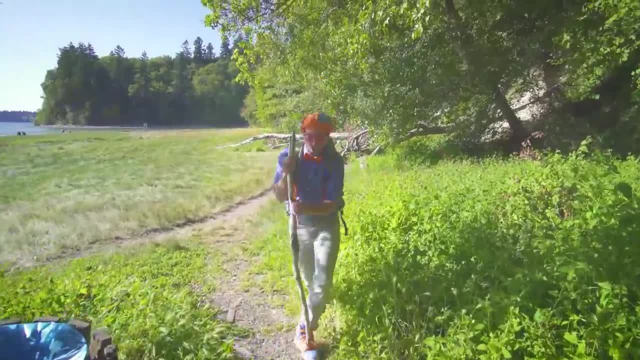 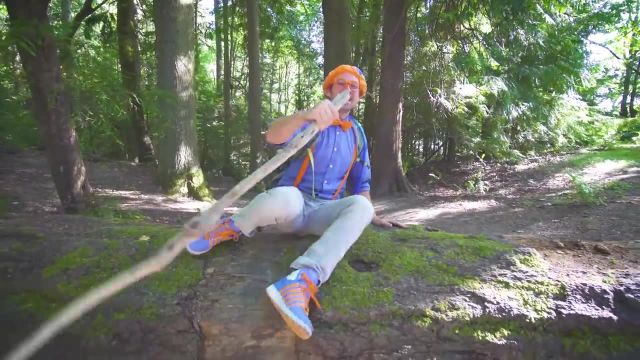 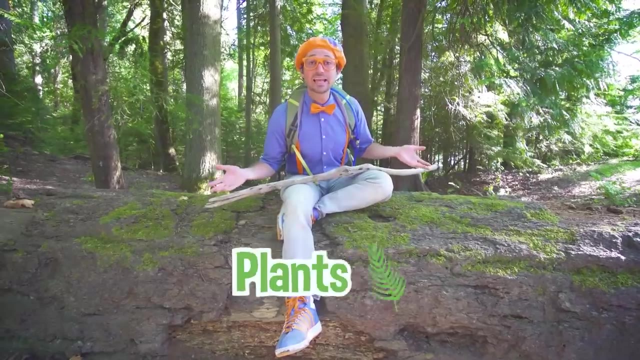 so then we can continue to hike. Woohoo, Got it, I am now ready. Haha, Wee, That was so much fun today going on a hike with you. We learned so much. We got to learn about plants. 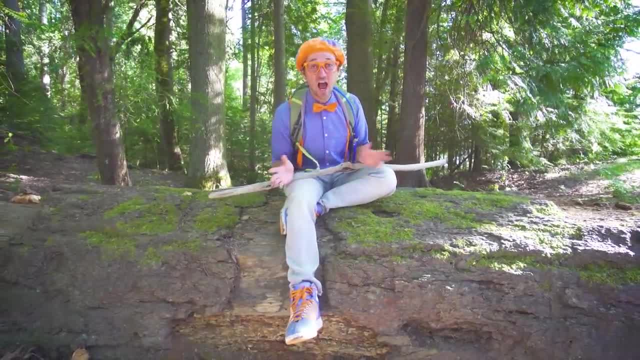 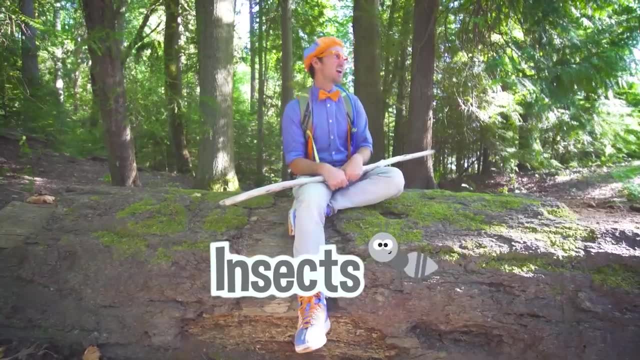 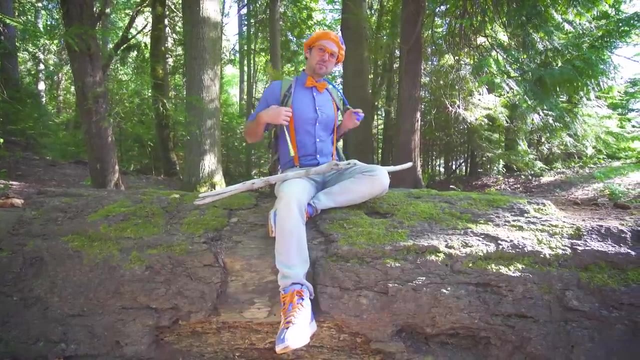 We played some search and find. Yeah, I spy. That was a lot of fun, Hey, We even saw some insects, Haha. Yeah, And probably most importantly, we cleaned up the beach. Good job, Hey, Remember earlier that we found some things. 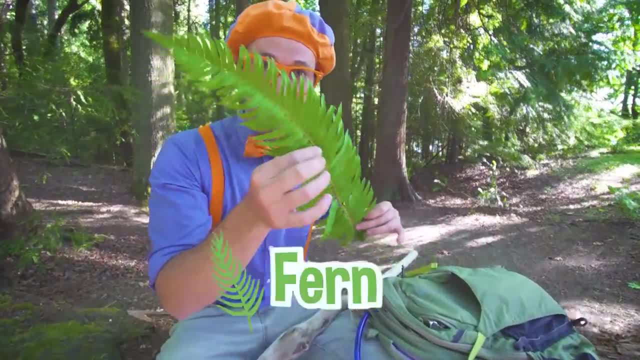 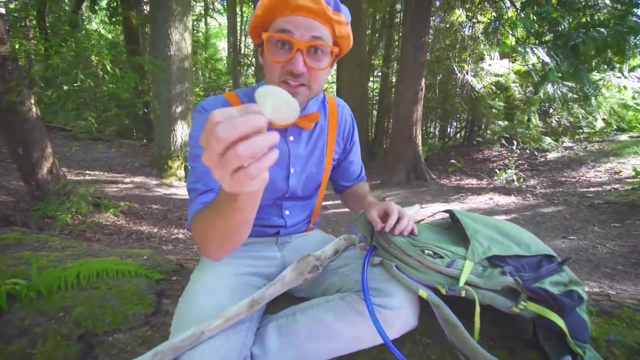 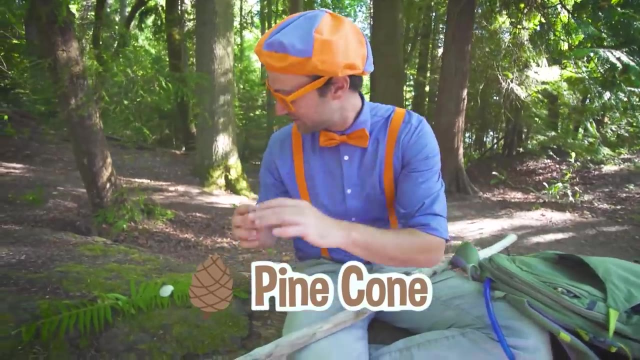 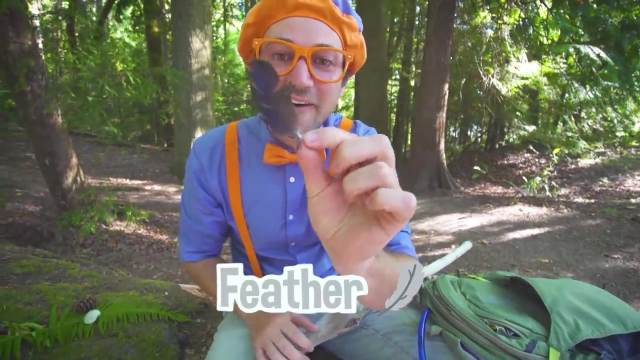 Yeah, We found this fern. Yeah, We're going to do something really cool with it very soon. And then we found this shell. Yeah, We found this pine cone. And we found this bird feather- Wow, Haha. Okay, We'll put that right there. 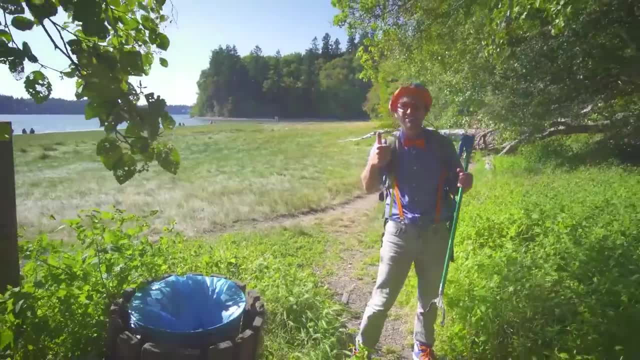 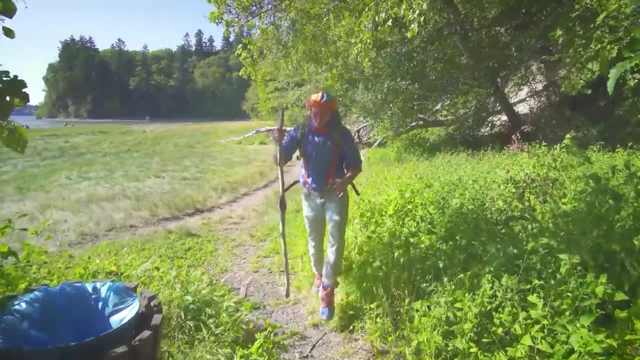 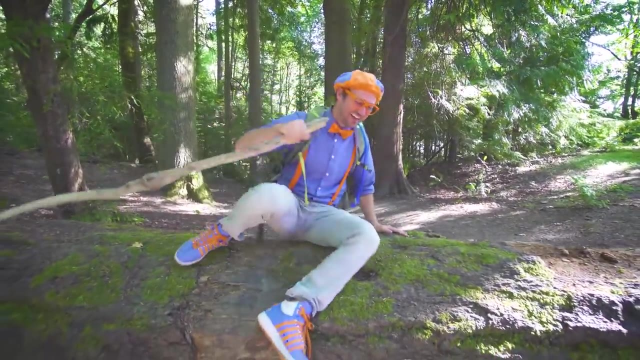 can Bye-bye garbage, Good job. Well, I should probably get my hiking stick back, so then we can continue the hike. Got it, I am now ready. That was so much fun today going on a hike with you. We learned so much. 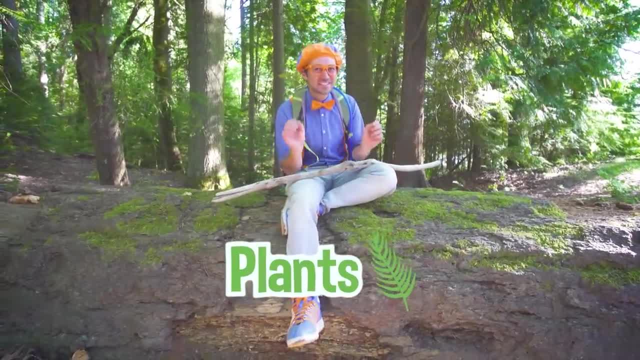 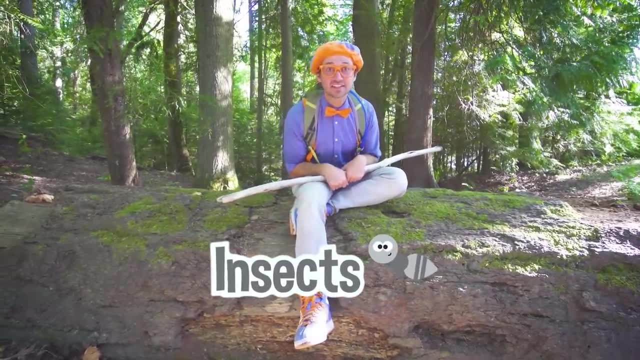 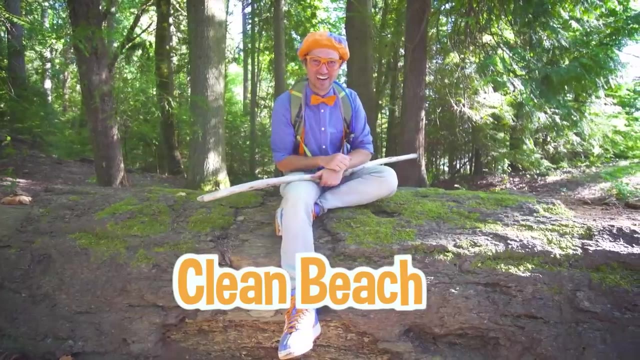 We got to learn about plants. We played some search and find- Yeah, I spy. That was a lot of fun. Hey, we even saw some insects. Yeah, And probably most importantly, we cleaned up the beach. Good job, Hey, remember earlier. 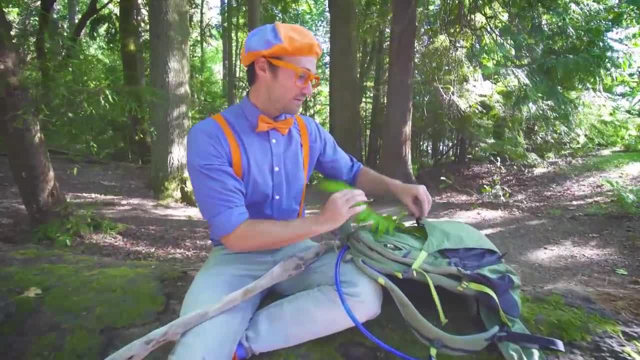 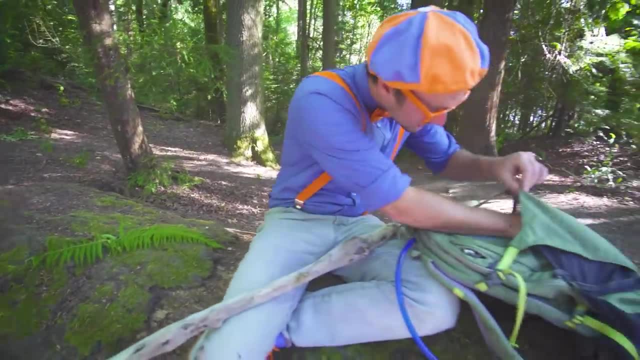 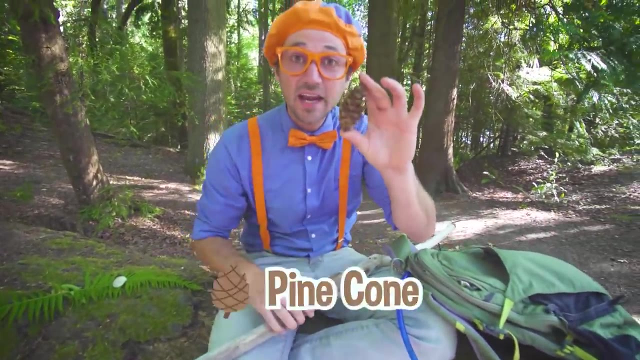 that we found some things. Yeah, We found this fern. Yeah, I'm going to show you something really cool with it very soon. And then we found this shell. Yeah, We found this pine cone And we found this bird feather. 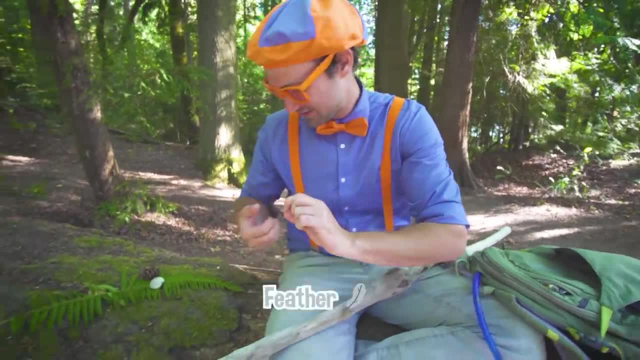 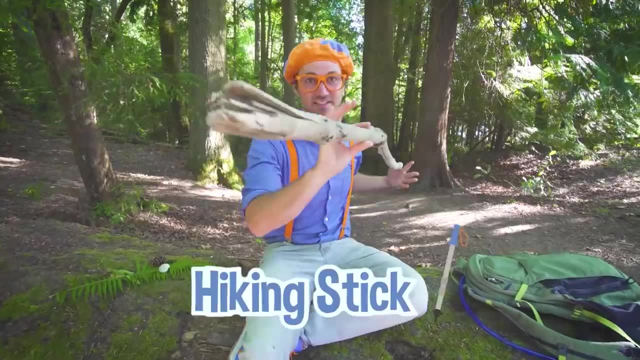 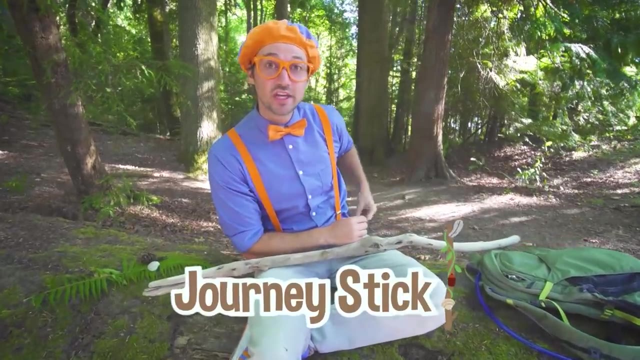 Wow, Okay, We'll put that right there, Okay. Well, this stick used to be a hiking stick that we used all day. That was great, But we're actually going to turn it into what's called a journey stick. Yeah, Indigenous. 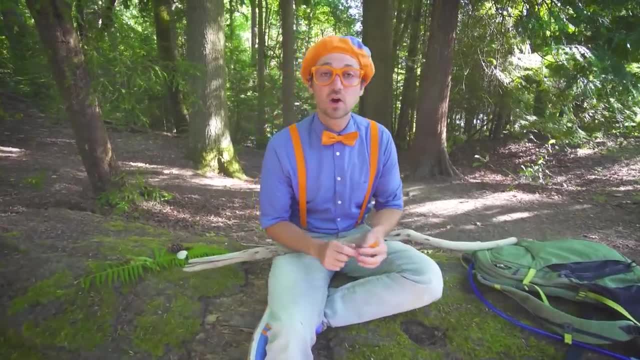 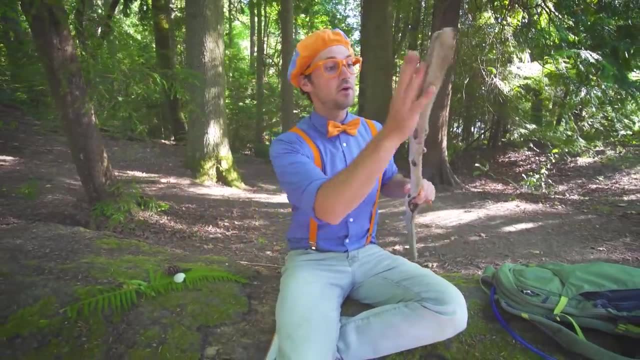 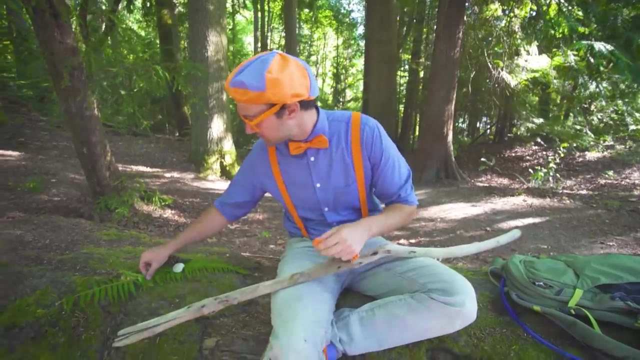 people from different countries used to make what's called journey sticks. They would collect things on their hikes and their journeys and then they would put them on their sticks in chronological order, so then they can remember where they've been. So let's do that now. 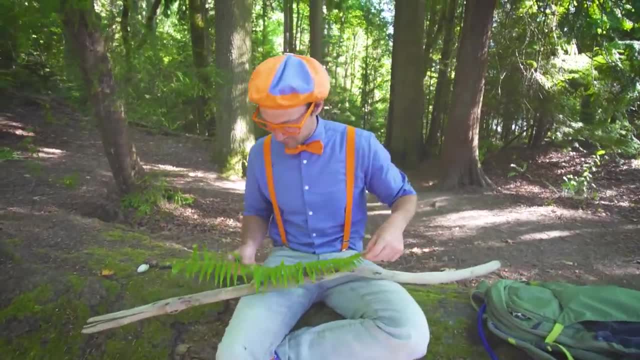 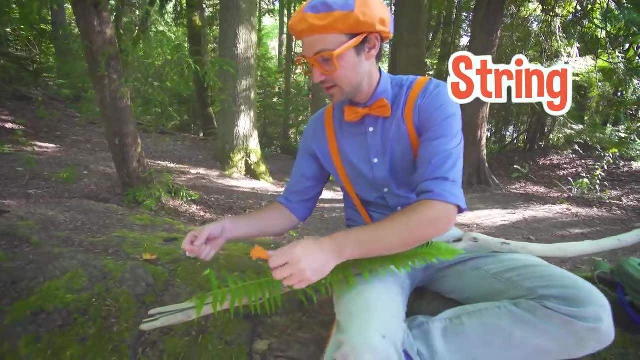 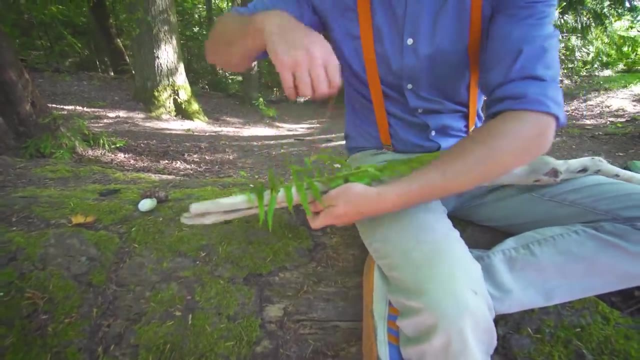 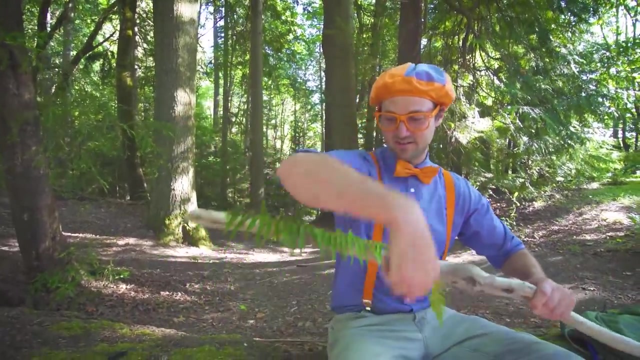 So let's take this big fern and put it right there. I actually have some orange string. Yeah, I'm going to wrap it around. Okay, Perfect, Doesn't that look good? Whoa, Pretty cool, huh, Okay, Wow. 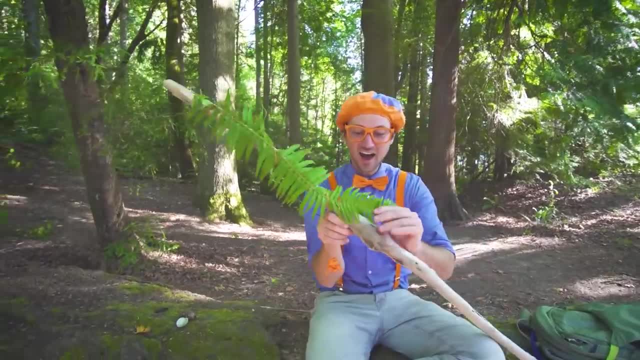 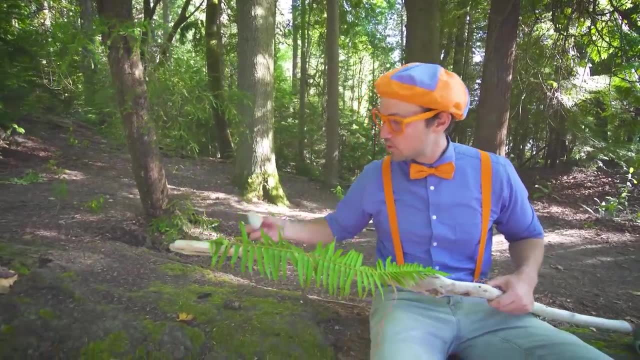 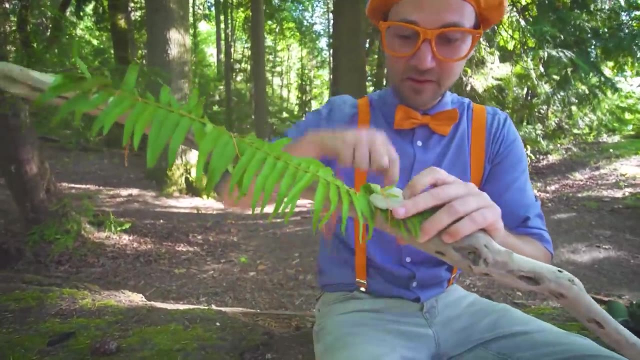 This looks so cool. Yeah, It's like a stick with a fern on it. Okay, What else? Oh, yeah, We have the shell. That's going to be tricky to put on there, But I think we can do it. 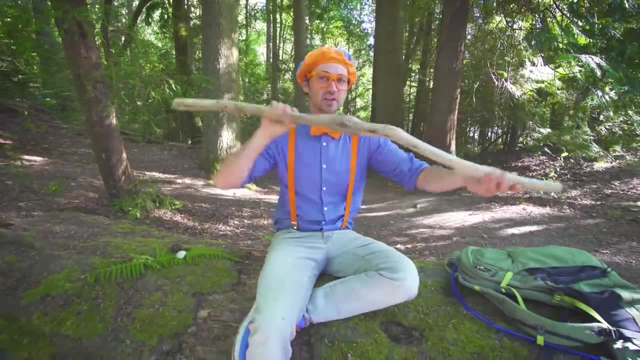 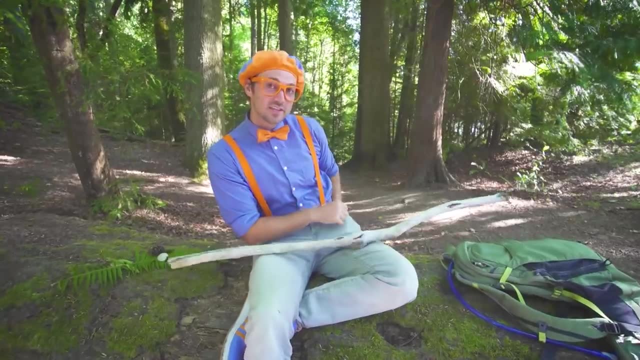 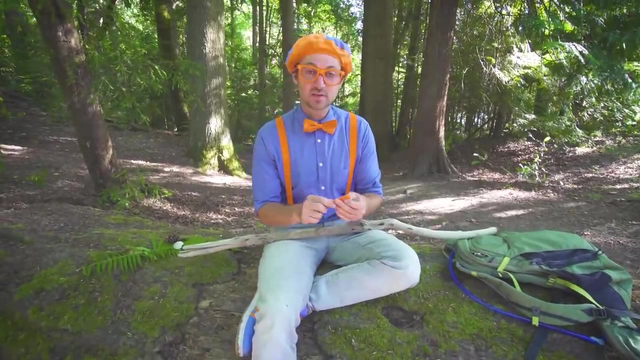 Okay, Well, this stick used to be a hiking stick that we used all day, But we're actually going to turn it into what's called a journey stick. Yeah, Indigenous people from different countries used to make what's called journey sticks. They would collect things on their hikes. 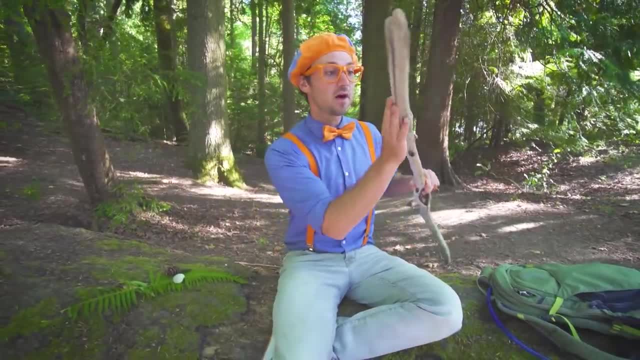 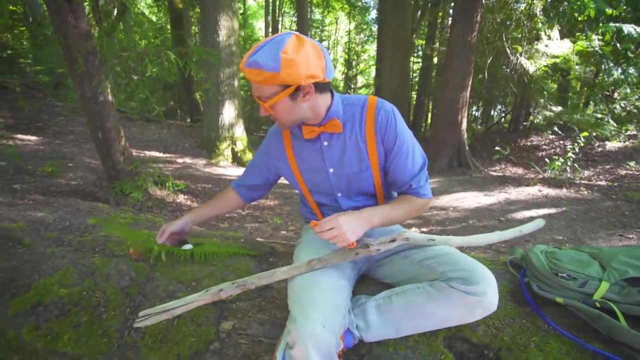 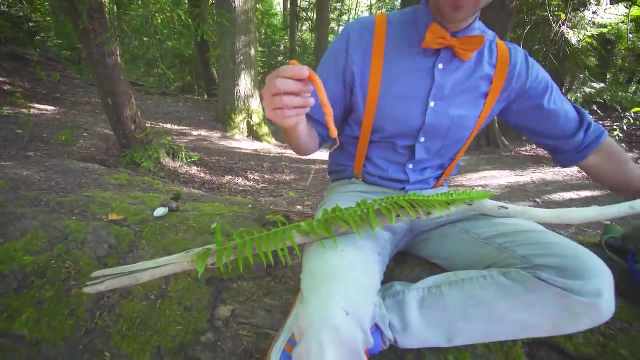 and their journeys, and then they would put them on their sticks in chronological order, so then they can remember where they've been. So let's do that now. So let's take this big fern and put it right there. I actually have some orange string. 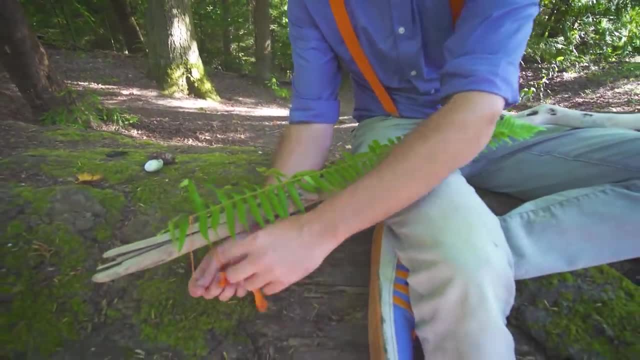 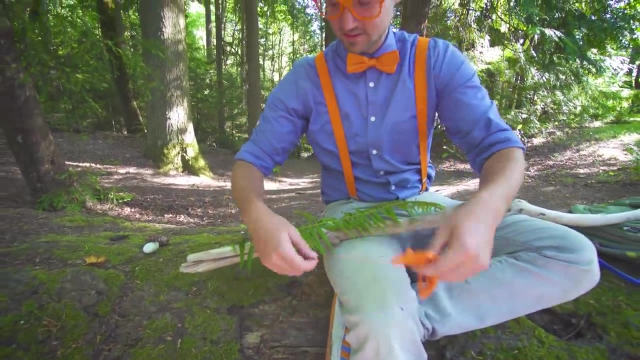 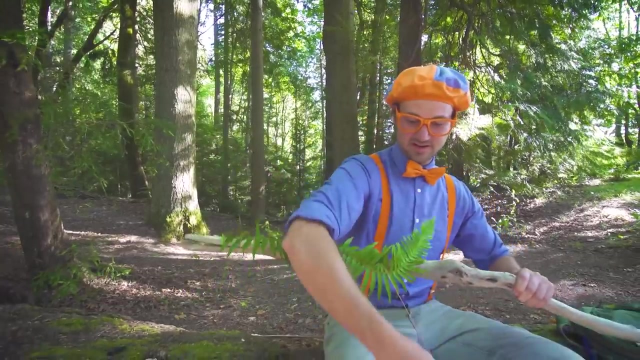 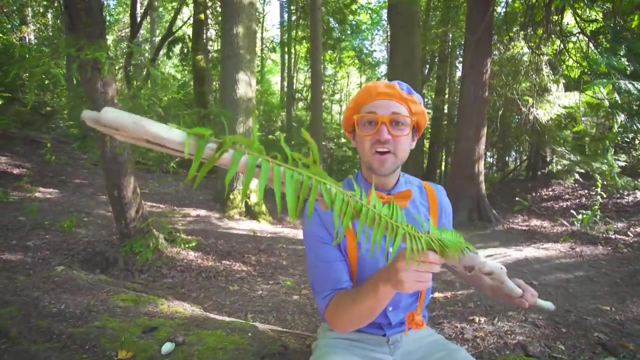 Yeah, I'm going to wrap it around. Okay, Perfect, Doesn't that look good? Whoa, Pretty cool, huh. Okay, Wow, This looks so cool. Yeah, Haha, It's like a stick with a fern on it. 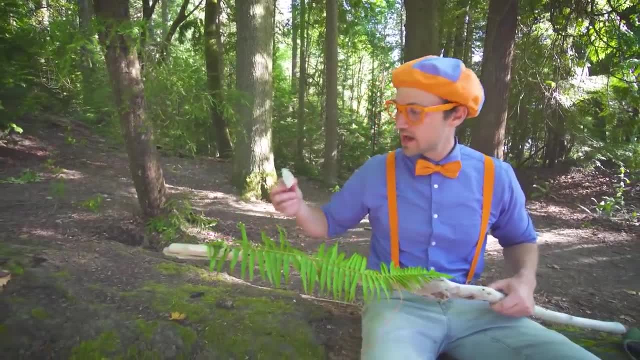 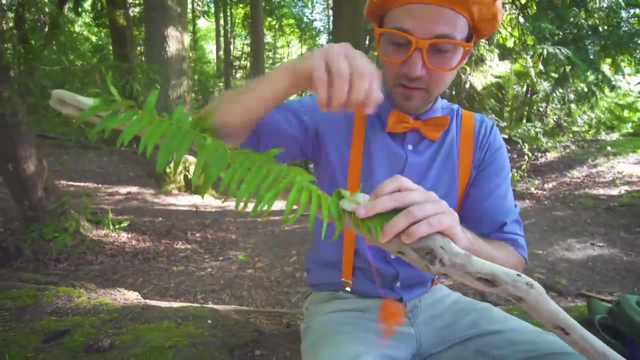 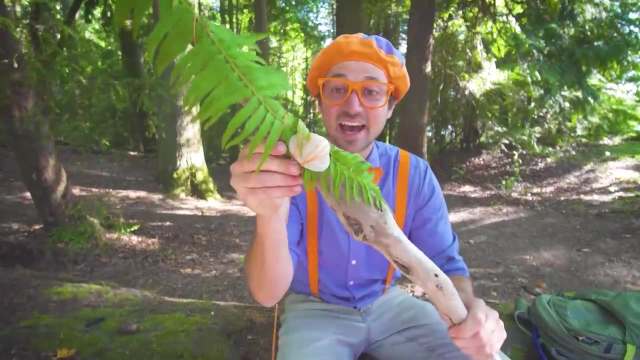 Okay, What else? Oh yeah, We have the shell. That's going to be tricky to put on there, But I think we can do it. There it is. You see that? Yeah, This is looking awesome. And then we have this pine. 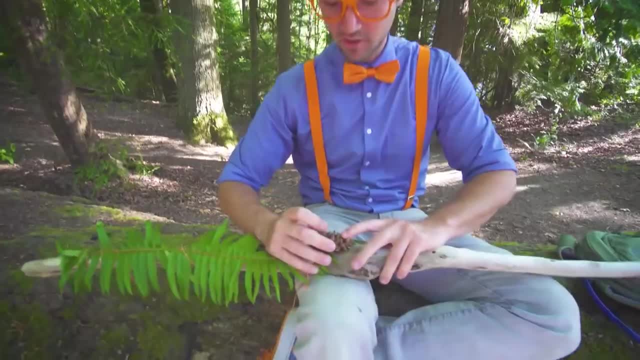 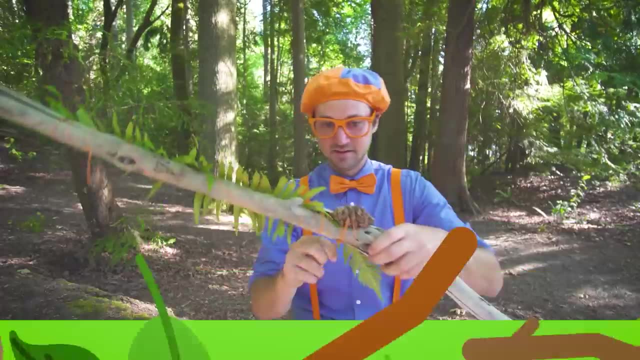 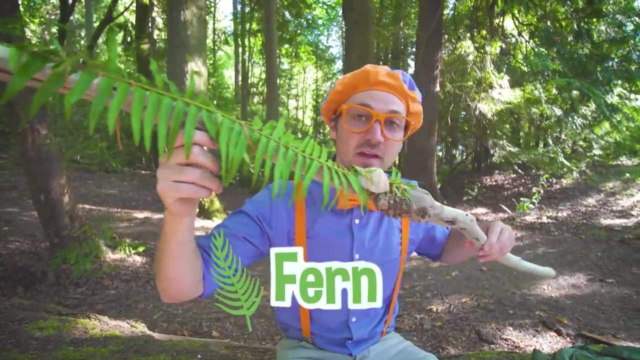 cone that I'll put right below that shell, Just like that, And then I'm going to loop this around, so then it'll hold onto it. Ooh Alright, We are almost done. See, we have the fern, the shell. 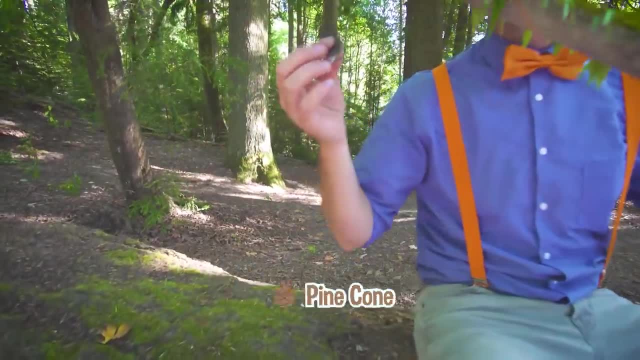 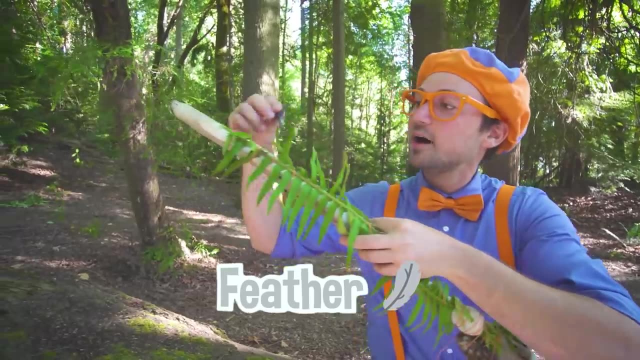 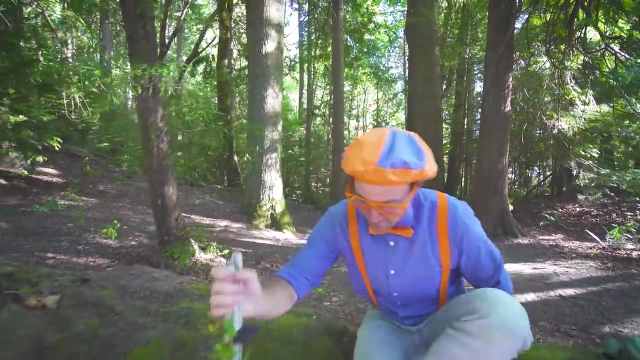 the pine cone and, last but not least, the feather. Okay, I'm going to put it right up top, Right there. See that? Haha? Alright, Check it out. How does this look? Haha, Whoa, Haha. 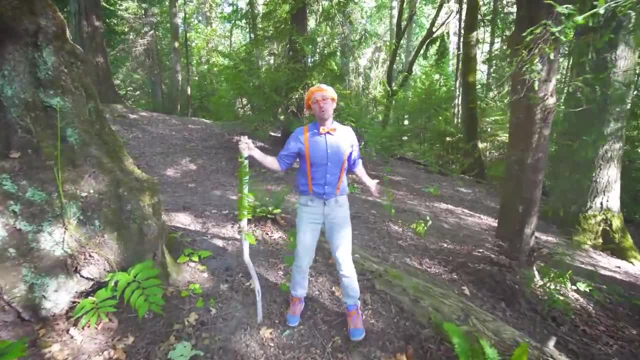 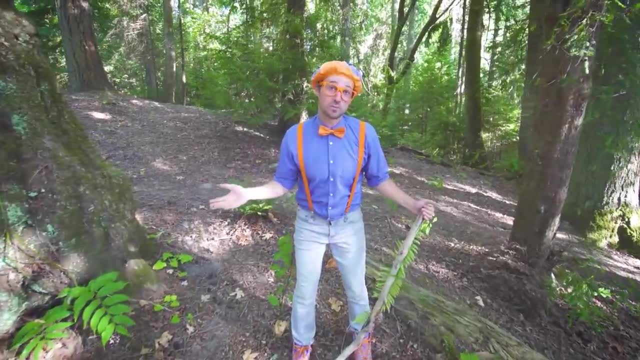 Woo, Haha. Well, this is the end of this video. I had so much fun learning with you, But if you want to watch more of my videos, all you have to do is search for my name. Will you spell my name with me?